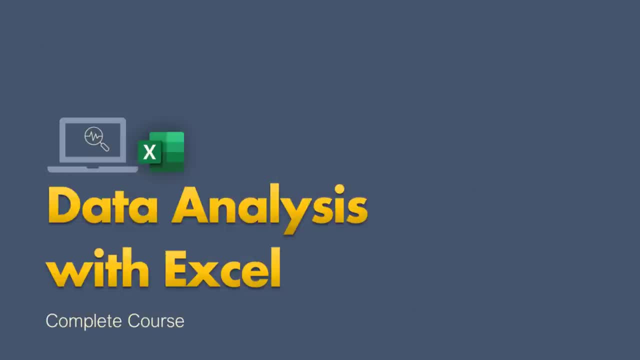 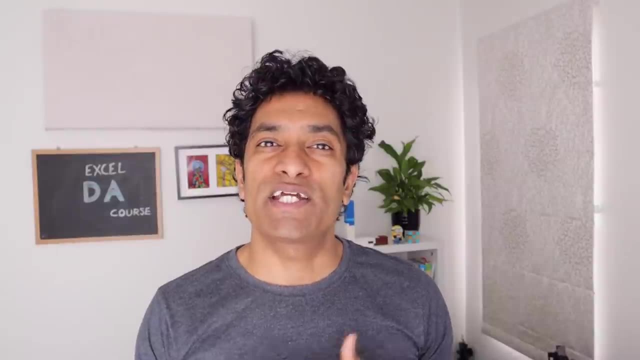 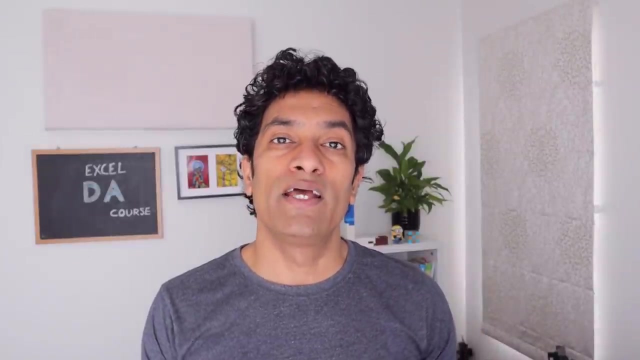 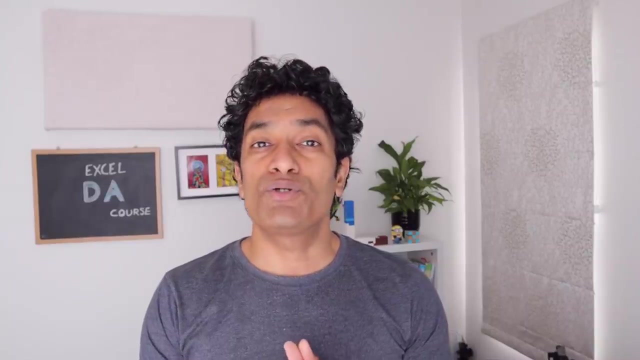 Welcome to Excel data analysis course. This is a completely self-contained data analysis course for people who are just getting started into data analytics with Excel, or people who have been already doing a data analyst role for a while and just want to understand in a more structured manner from an experienced person. In this video, I'm going to show you a sample data. 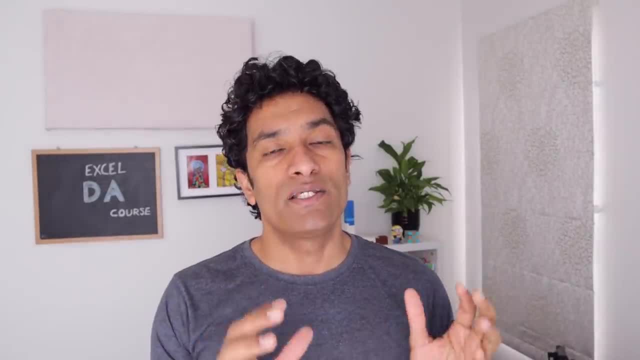 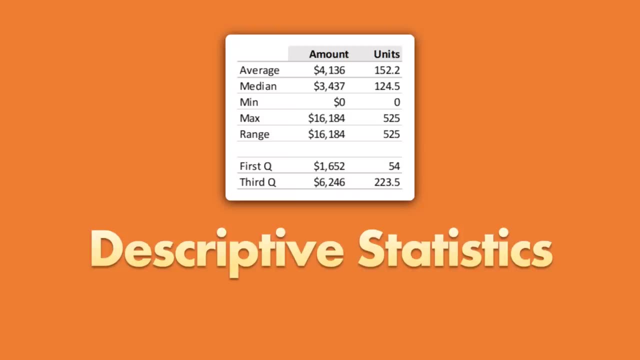 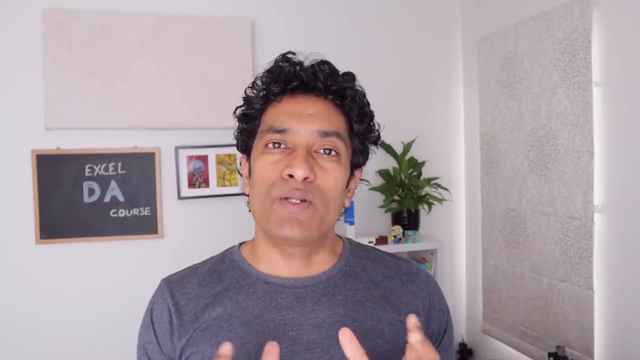 and then 10 ways to analyze the data using Excel. We are going to look at seven key different techniques. We'll talk about descriptive statistics and then we will look at how to use Excel to do exploratory data analysis, and then we are also going to look at formulas, as well as 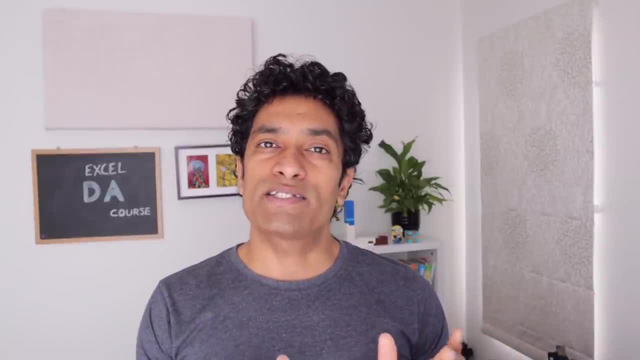 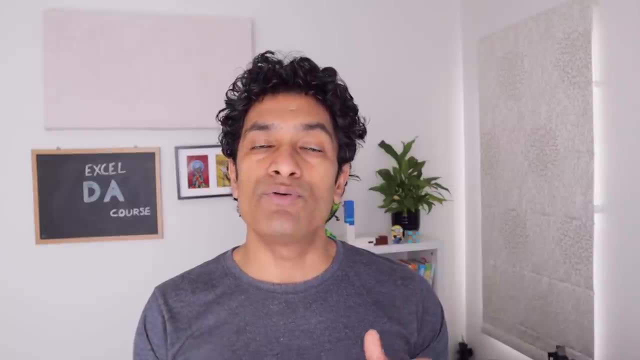 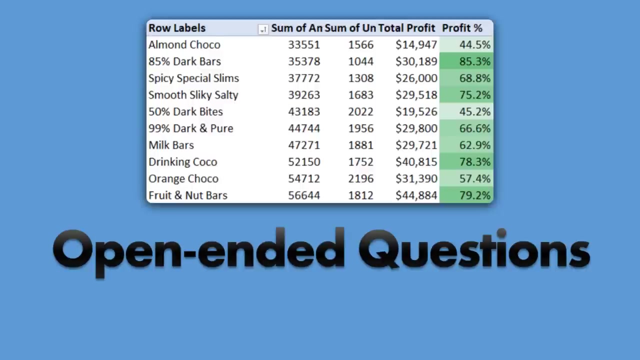 pivot tables to analyze the data. We will also understand how to combine the data that is in separate tables to get a consolidated view when you are analyzing the data. We will also understand how to answer open-ended questions that are: there is no specific question there, but you need to figure. 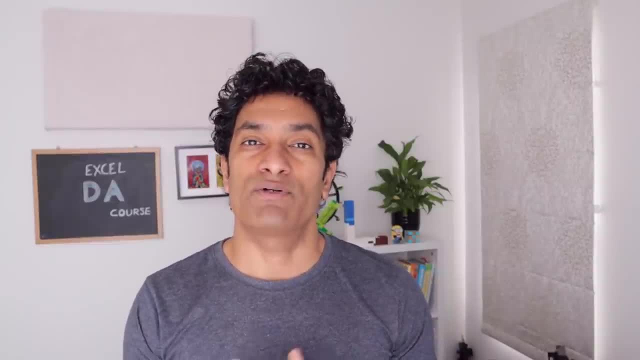 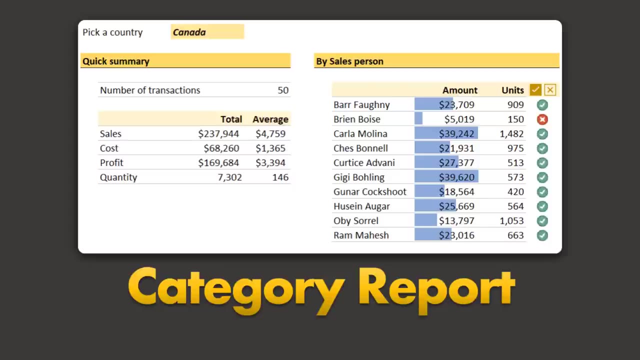 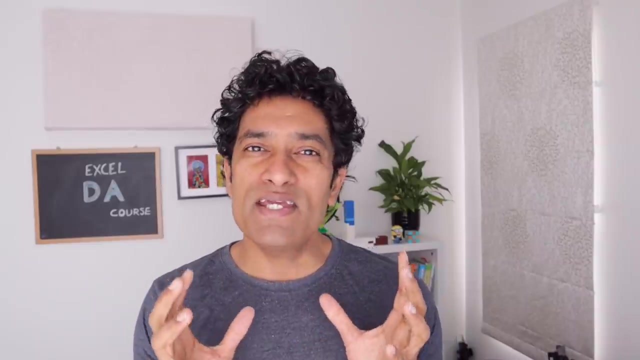 out the answer using data analysis. how to answer those kinds of questions in this video. Finally, you are going to learn how to present the analysis using various types of charts, conditional formatting and other visualization techniques that are available in Excel. This video is really. 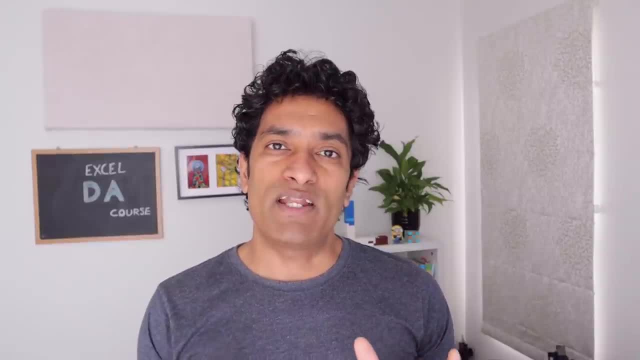 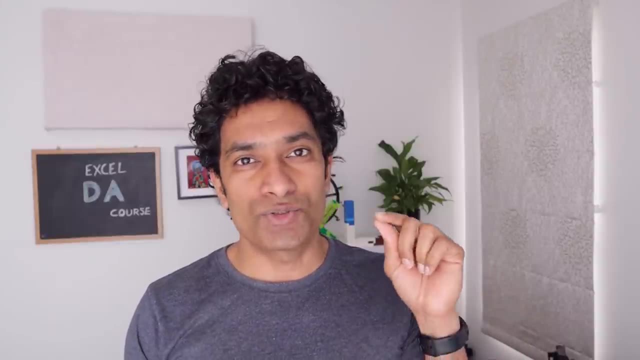 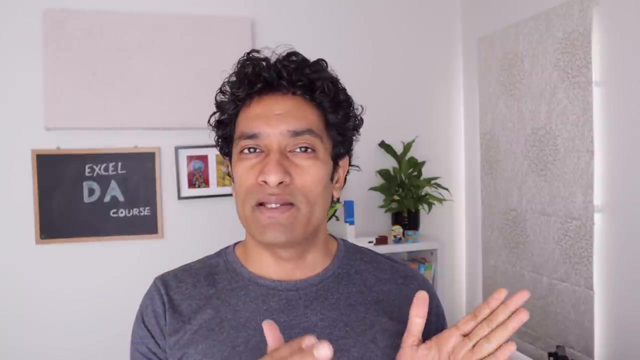 jam-packed with a lot of detail. So what I've done is I have provided you with two workbooks. One is a blank data file. So if you are up for a challenge, I suggest you to download the blank data file and then just use it to go through the material and then try to replicate the steps on. 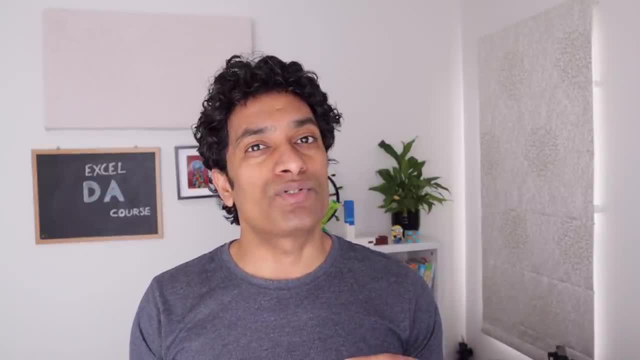 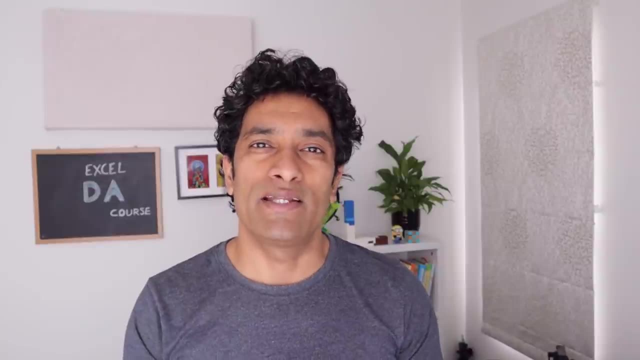 the blank file, But there is also a completed workbook so that you can actually use it as inspiration or take that if you are feeling stuck or if you want just a hand-drawn workbook. So once again, thanks for your patience. If you are interested in learning more about data analysis, 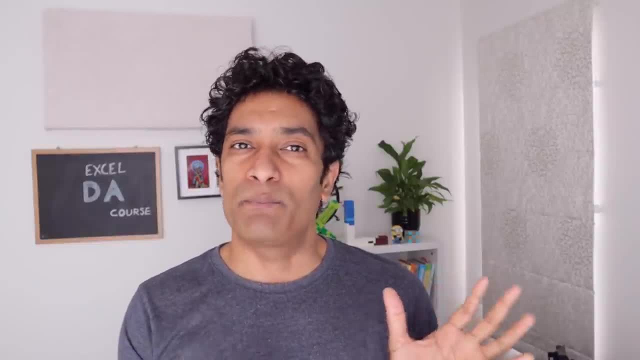 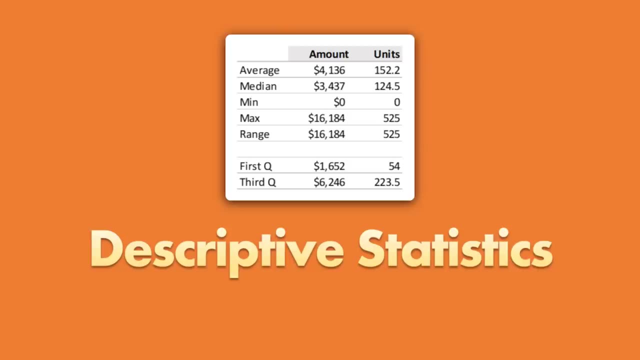 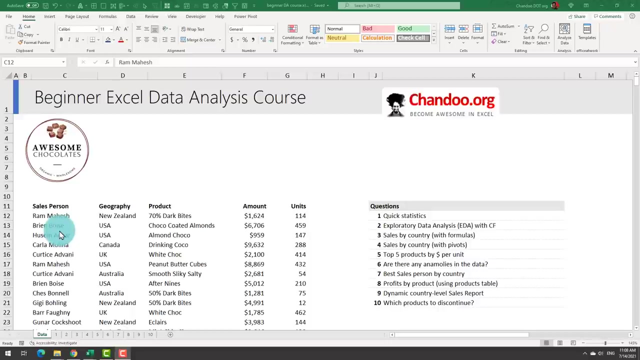 please consider subscribing to our channel and clicking the bell icon to get the latest updates. So let's get started. So first of all, let's start our analysis with preparing some quick statistics on the sample data set here Now. a good practice when you are doing this in Excel data is to turn your raw data into 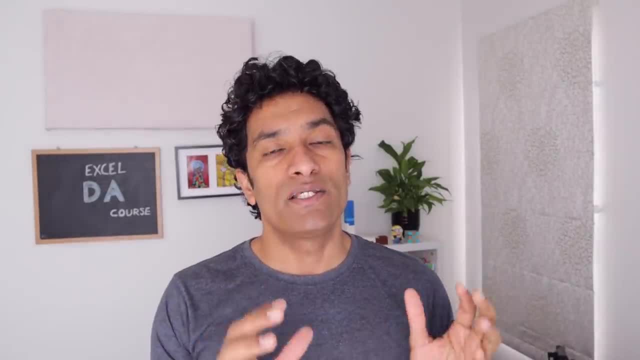 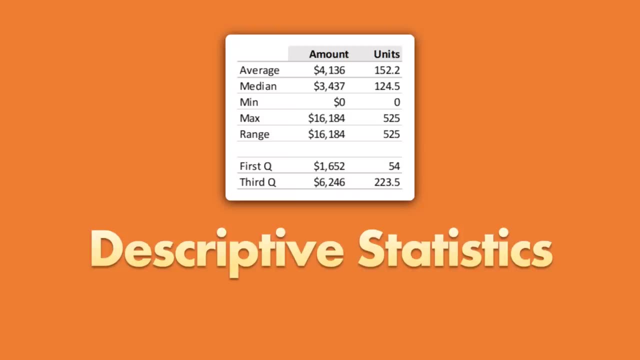 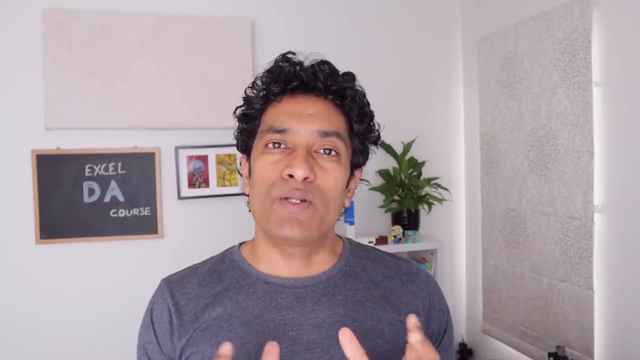 and then 10 ways to analyze the data using Excel. We are going to look at seven key different techniques. We'll talk about descriptive statistics and then we will look at how to use Excel to do exploratory data analysis, and then we are also going to look at formulas, as well as 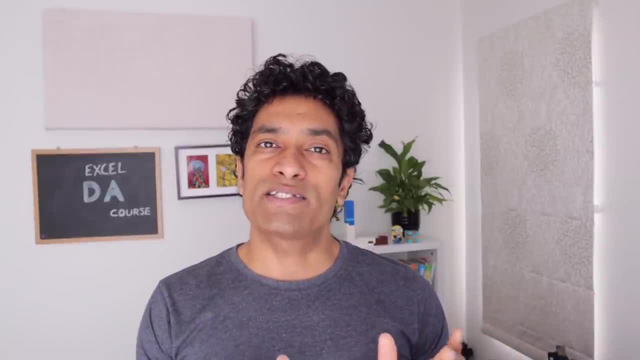 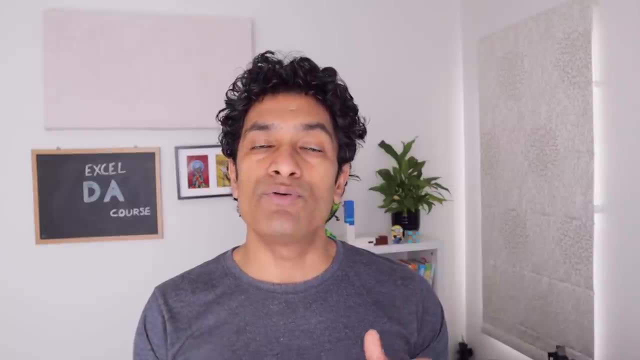 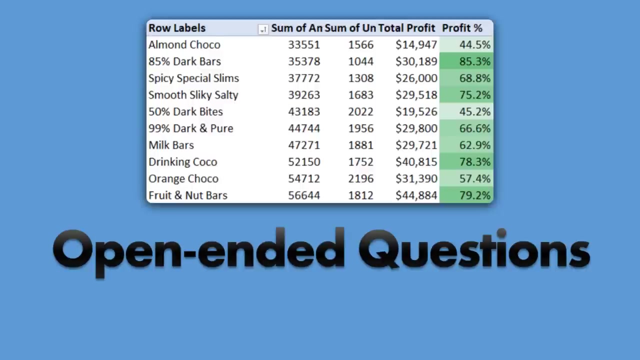 pivot tables to analyze the data. We will also understand how to combine the data that is in separate tables to get a consolidated view when you are analyzing the data. We will also understand how to answer open-ended questions that are: there is no specific question there, but you need to figure. 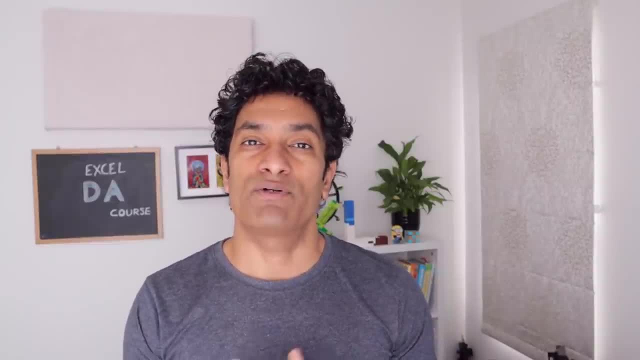 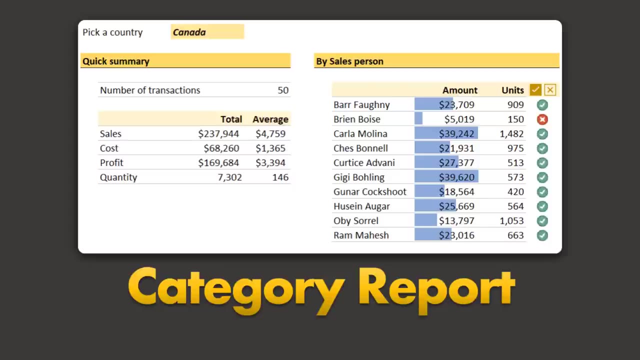 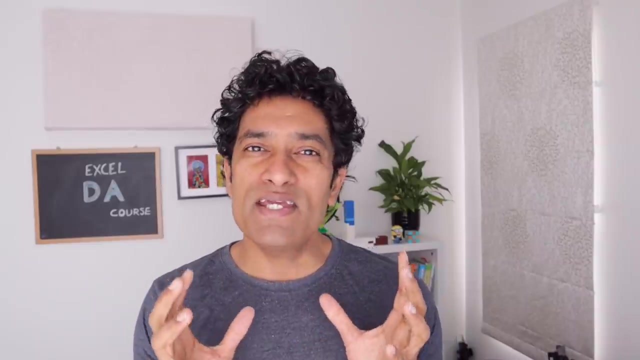 out the answer using data analysis. how to answer those kinds of questions in this video. Finally, you are going to learn how to present the analysis using various types of charts, conditional formatting and other visualization techniques that are available in Excel. This video is really. 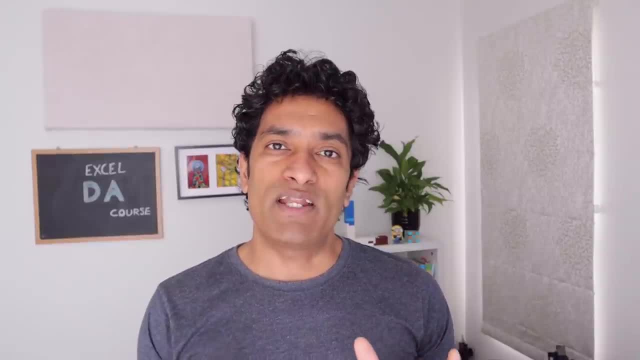 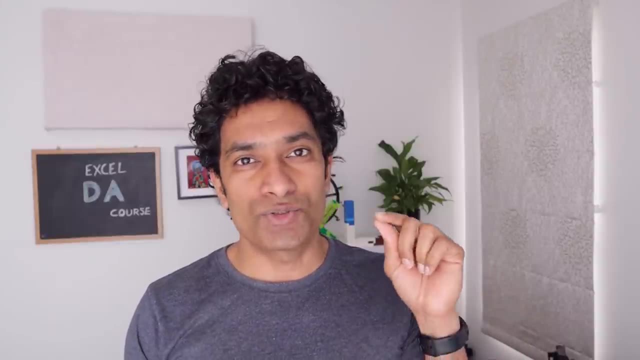 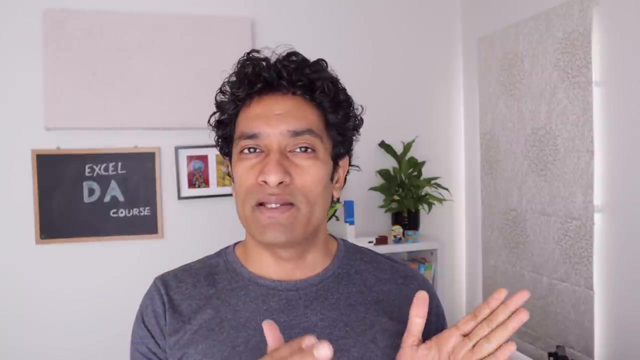 jam-packed with a lot of detail. So what I've done is I have provided you with two workbooks. One is a blank data file. So if you are up for a challenge, I suggest you to download the blank data file and then just use it to go through the material and then try to replicate the steps on. 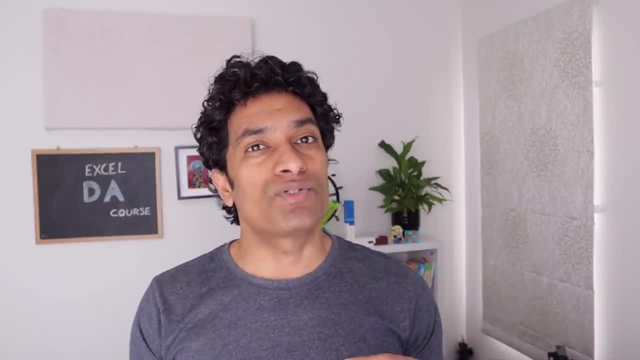 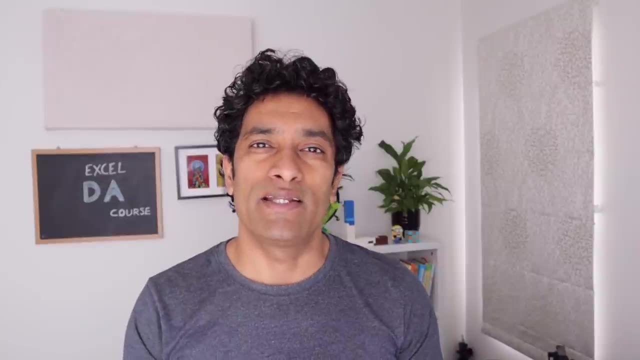 the blank file, But there is also a completed workbook so that you can actually use it as inspiration or take that if you are feeling stuck or if you want just a hand-drawn workbook. So you can use that as inspiration or take that if you are feeling stuck or if you want just a hand-drawn. 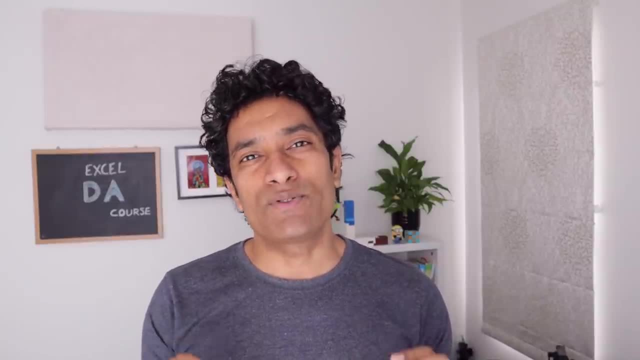 workbook, So you can use that as inspiration. or take that if you are feeling stuck, or if you want just a hand-drawn workbook, So you can use that as inspiration, or take that as inspiration. or, finally, I highly recommend that you set aside time and watch this whole video entirely. 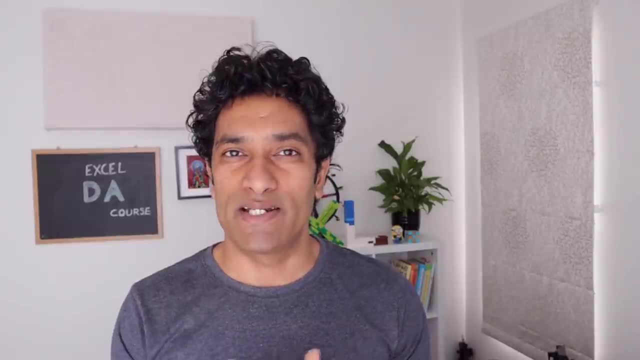 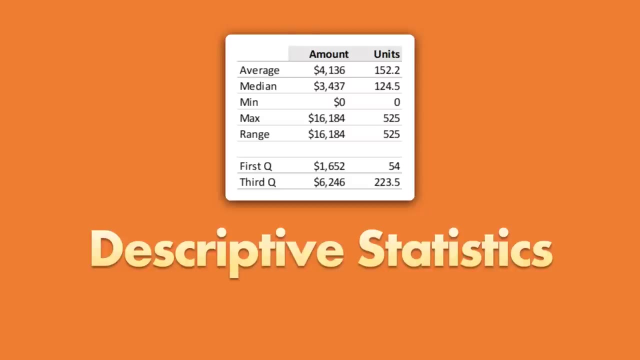 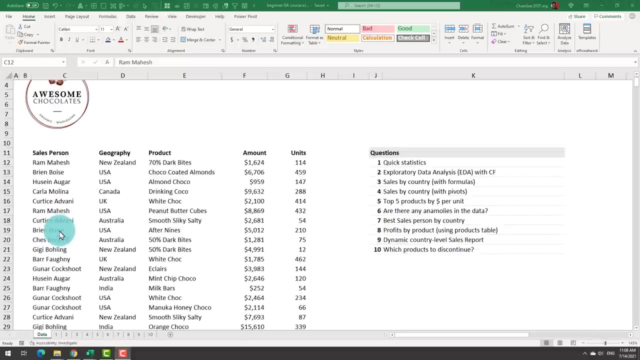 and practice the concepts. if you are really serious about your data analyst skills, Let's jump in. We'll start our analysis with preparing some quick statistics on the sample data set here Now. a good practice when you are doing this in Excel data is to turn your raw data into a table. 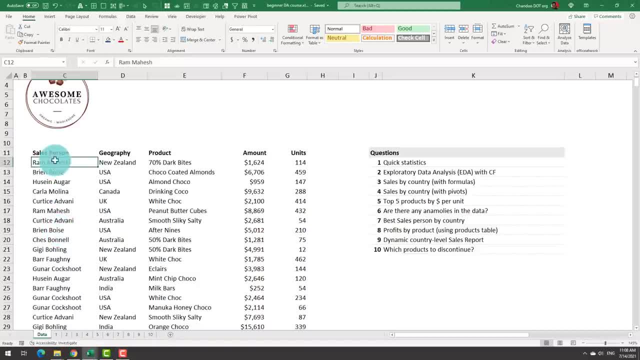 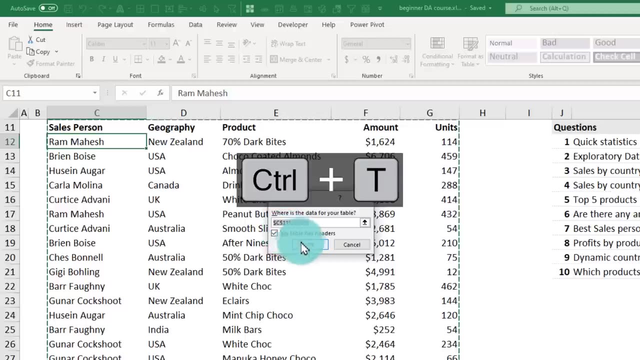 format. This way you don't have to remember where your data begins. In this case you'll have to start from C12 and then it goes all the way up to G12 in the columns and then several rows down. To do this, just select any cell and press control T. T for table to insert a table. 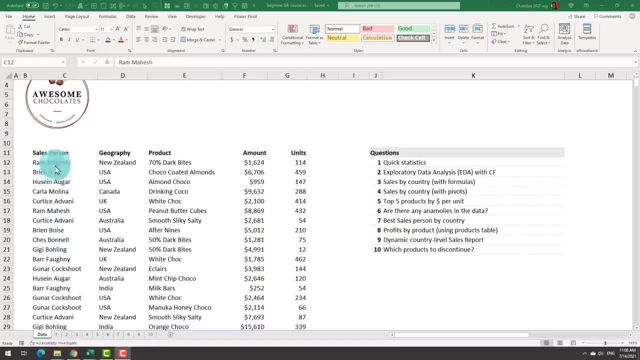 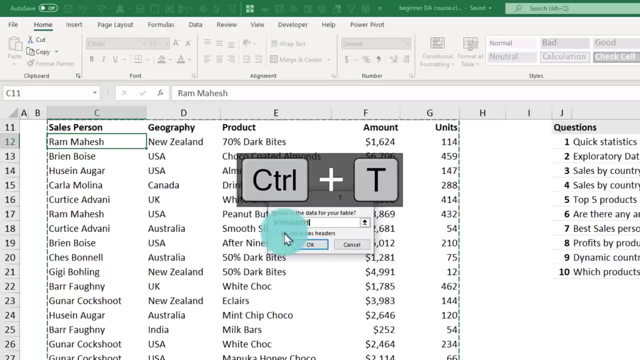 a table format. This way, you don't have to remember where your data begins, In this case from C12, and then it goes all the way up to G12 in the columns and then several rows down. To do this, just select any cell and press control T, T for table to insert a table. and. 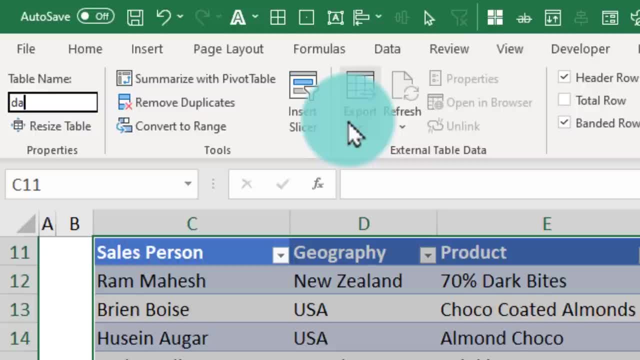 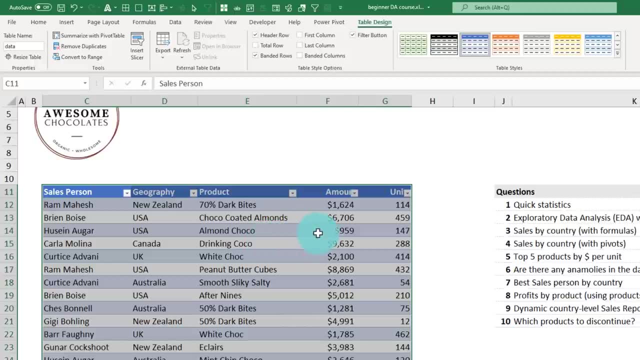 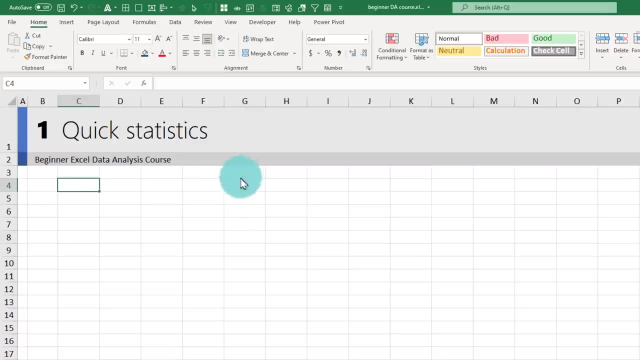 then I'm going to give my table a name. We will call this as data. From here on we'll simply refer to the data table for all our analysis. So let's go and calculate some quick statistics. We could start off with some of the most basic ones on the number column. So we got our amount. 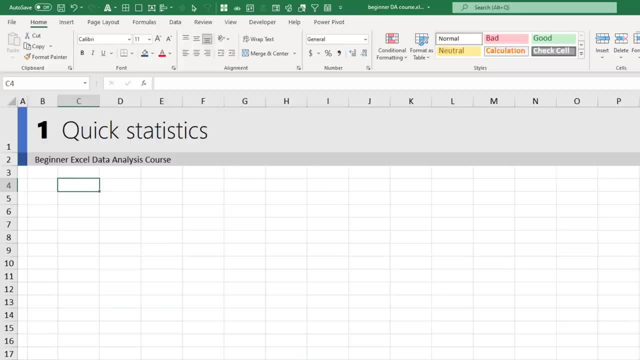 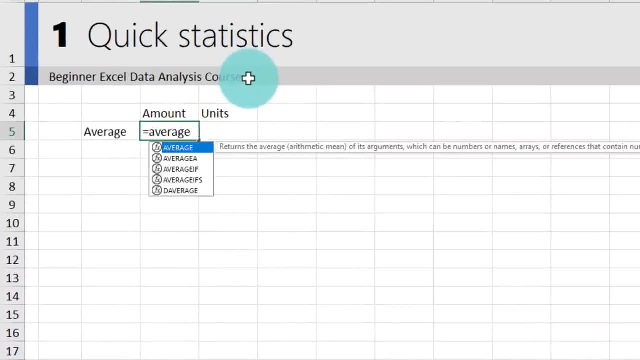 and unit columns. Let's calculate both average amount, average units, as well as median amounts and median units, And here we can use the average formula like this: average data table: amount column. Then we will get the answer as $4,136.. When you drag this formula sideways, 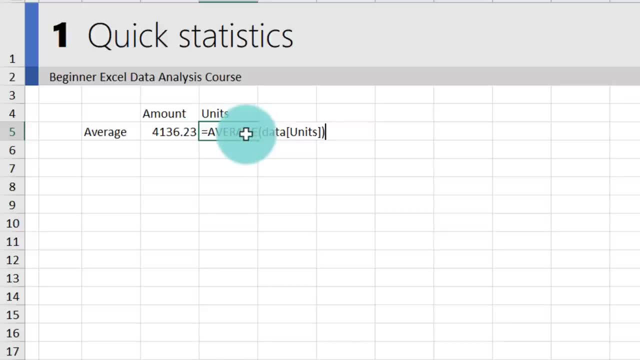 the amount column becomes unit number columns that we can change from beginning to end, or it become a number column. I'm going to be using both of the formulas in this example here, and then we can schedule column and we will get average units as well. Let's do the same for median. We can use the. 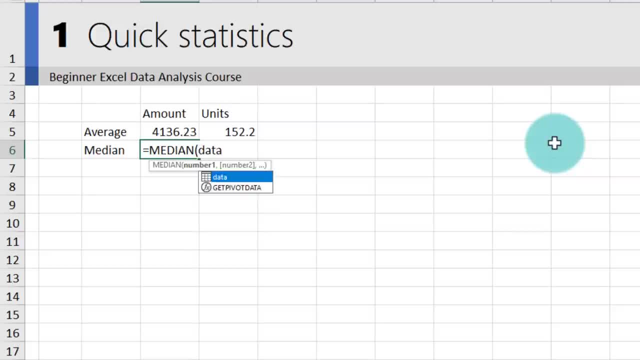 median formula for this median data amount. Now, when you're typing the formulas, one quick way to do this very fast- the way I'm doing- is type equal to type the first few letters and when you see the highlighted value in blue color, press the tab key and Excel will auto fill that for you. So you say: 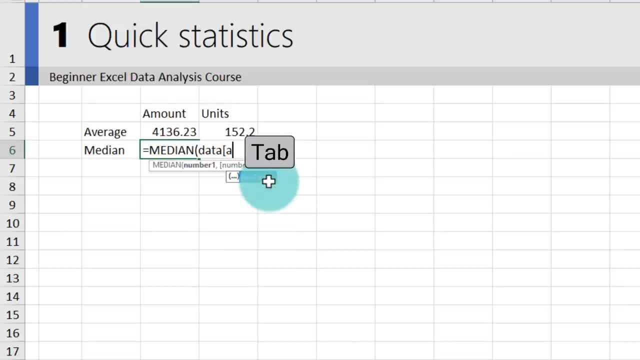 DA tab- open bracket. amount tab- close bracket- close bracket. and then we can just drag this sideways to see the units. Many times when we are analyzing the data, people often confuse between average and median and they try to calculate only one of them. But it's a good idea to calculate. 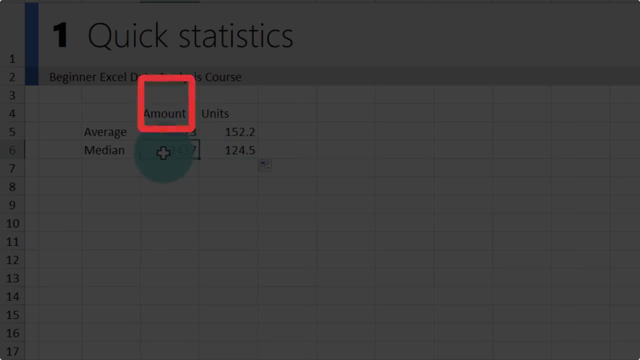 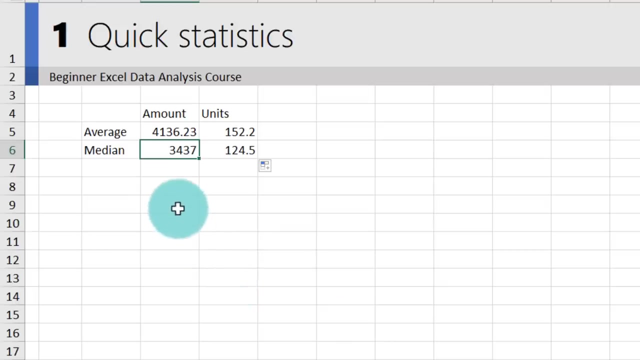 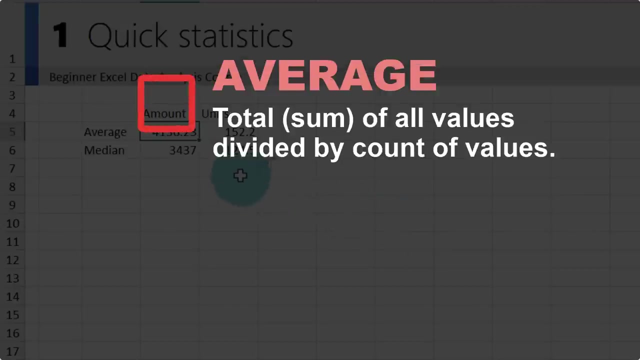 both to understand what's happening in the data. Median refers to the midpoint of the amount, So all the amounts are arranged in ascending order. the middle value will be 3437, whereas average is nothing but sum of all the values divided by count of the values. As you could see from here, our average is slightly higher than the median. that 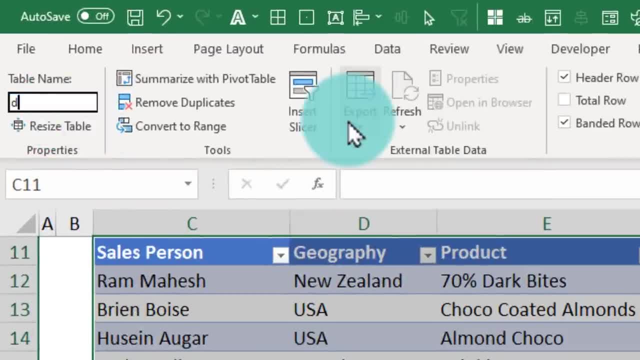 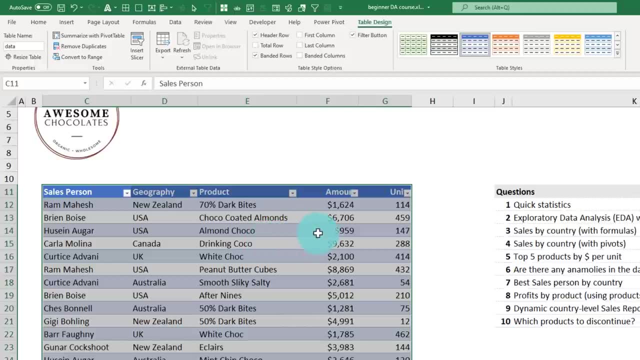 And then I'm going to give my table a name. We will call this as data. From here on, we'll simply refer to the data table for all our analysis. So let's go and calculate some quick statistics. We could start off with. 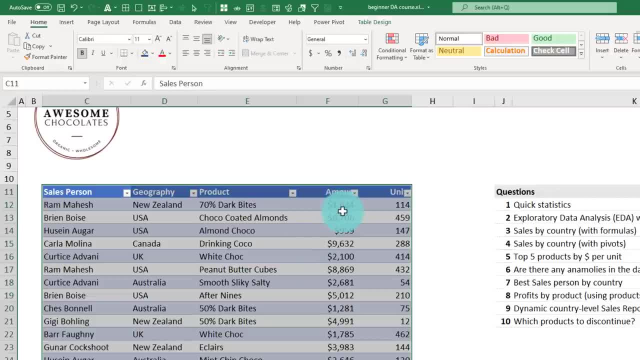 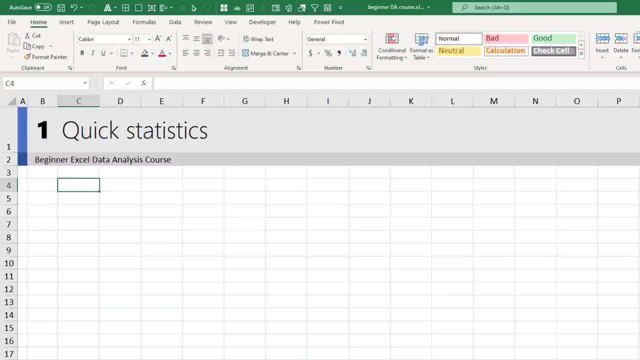 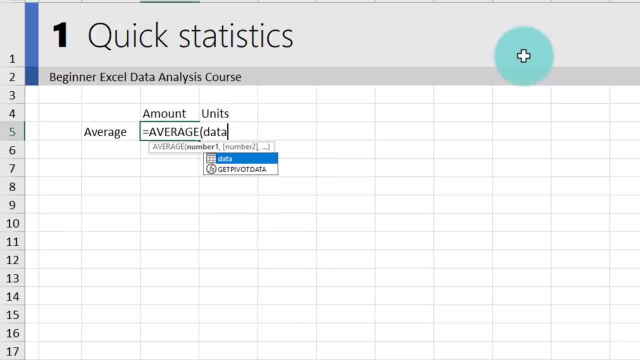 some of the most basic ones on the number column. So we got our amount and unit columns. Let's calculate both average amount and average units, as well as median amounts and median units, And here we can use the average formula like this average data table: amount column. 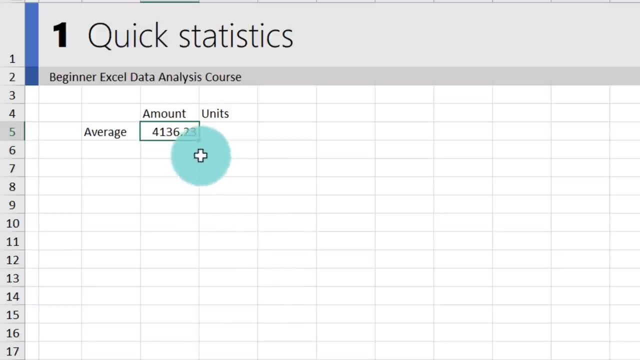 and then we will get the answer as $4,136.. When you drag this formula sideways, the amount column becomes units column and we will get average units as well. Let's do the same for median. We can use the median formula for this median data amount. 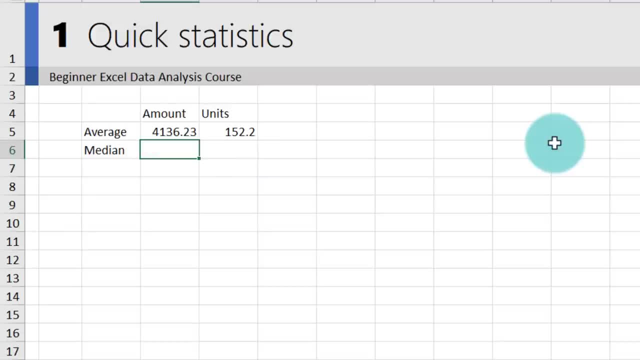 Now when you're typing the formulas. one quick way to do this very fast- the way I'm doing- is type equal to type the first few letters And when you see the highlighted value in blue color, press the tab key and Excel will autofill that for you. So you say DA tab, open bracket. 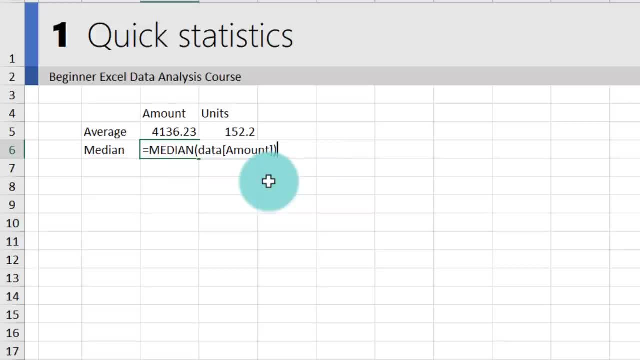 amount tab- close bracket, close bracket, And then we can just drag this sideways to see the units. Many times when we are analyzing the data, people often confuse between average or median and they try to calculate only one of them. But it's a good idea to calculate both to 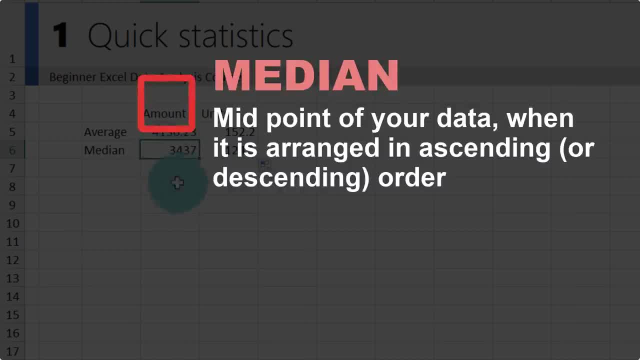 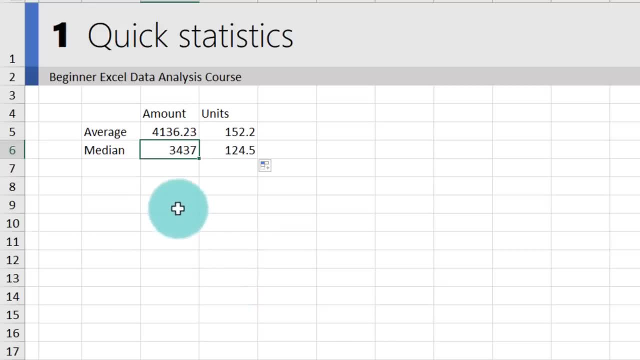 understand what's happening in the data. Median refers to the midpoint of the amount. So if all the amounts are arranged in ascending order, the middle value will be $3,437,, whereas average is nothing but sum of all the values divided by count of three. 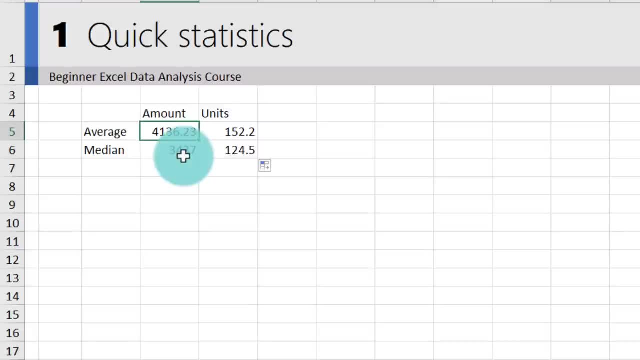 As you could see from here, our average is slightly higher than the median. That means there is probably more higher amounts in the data than there are lower amounts. It's a good practice to also calculate some of the other statistics when you're doing this. So 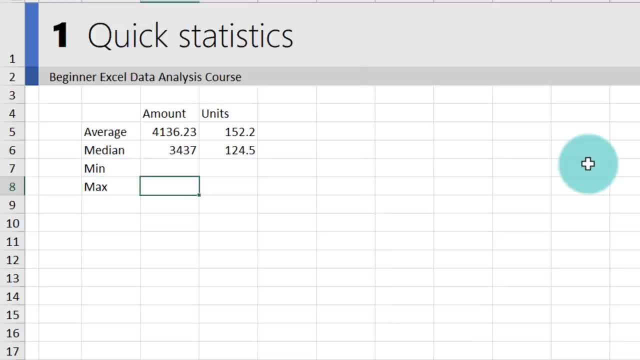 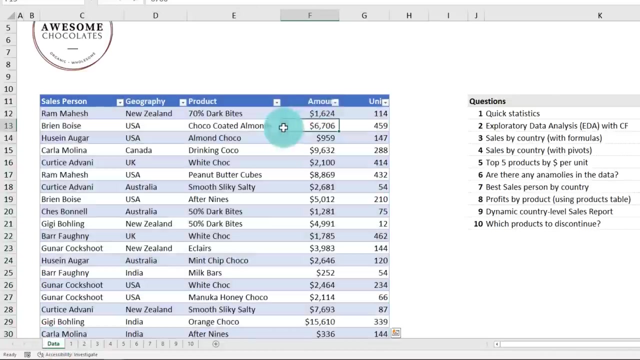 for example, you could calculate minimum and maximum values to see how these values are spread. We can use the similar formulas min, data amount and you could see that the minimum amount is $0.. This looks a bit suspicious, so I'm going to go and check this. I can go to my amount table and 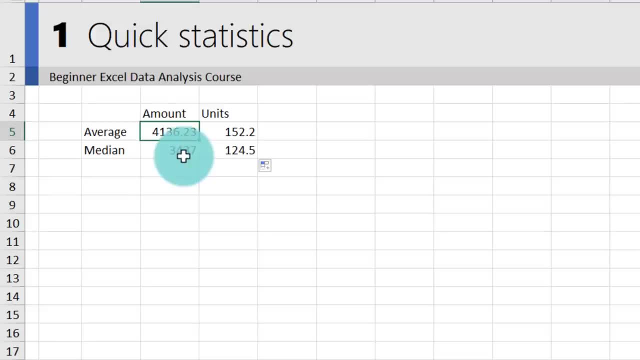 means there is probably more higher amounts in the data than there are lower amounts. It's a good practice to also calculate some of the other statistics when you are doing this, So, for example, you could calculate minimum and maximum values to see how these values are spread. We can use the 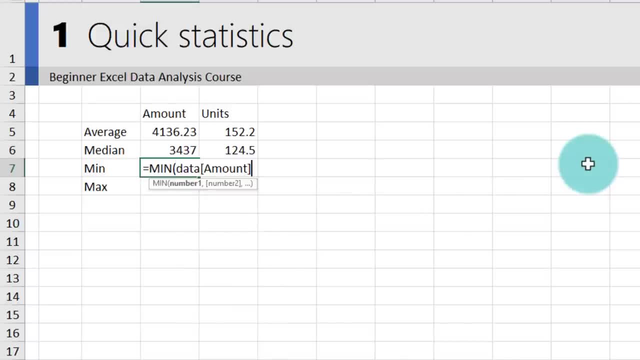 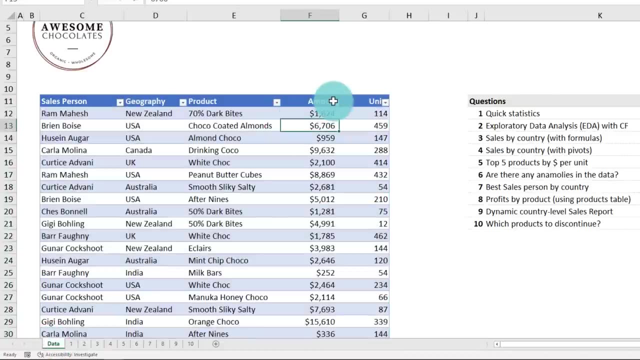 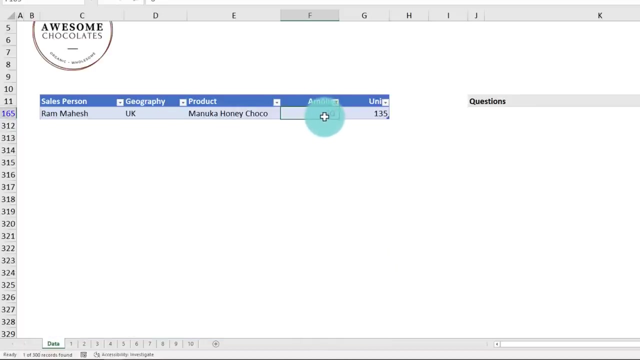 similar formulas- min data, amount- and you could see that the minimum amount is zero dollars. This looks a bit suspicious, so I'm going to go and check this. I can go to my amount table and then filter for the zero dollars to see that there is actually indeed one row where we made zero dollars. 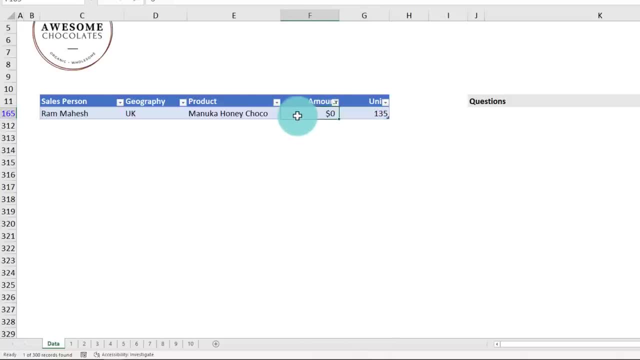 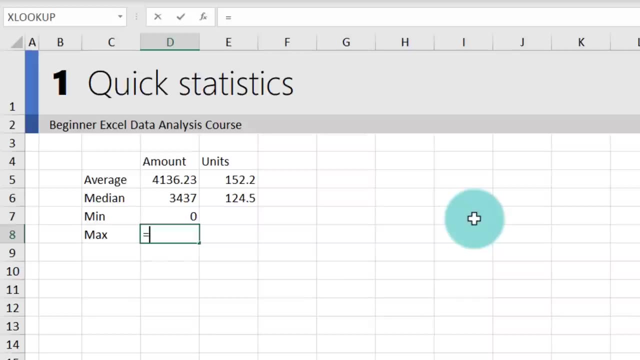 selling 135 units. At this point you may want to calculate the minimum and maximum values of the data. You may want to go back and check your original data to see if this is actually correct or maybe there is something wrong here. Likewise, max is max of data amount, Another common metric. 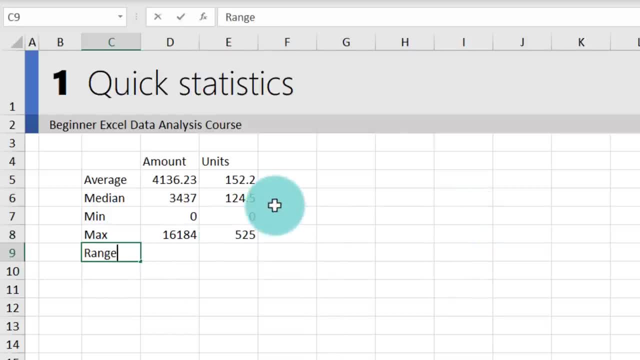 that we calculate in quick statistics is a range. Range is nothing but the distance between minimum and maximum. So we can say max minus min and that will be the range. In this case, because our minimum is zero, range is nothing but max. You can also calculate the quartiles Just as minimum, and 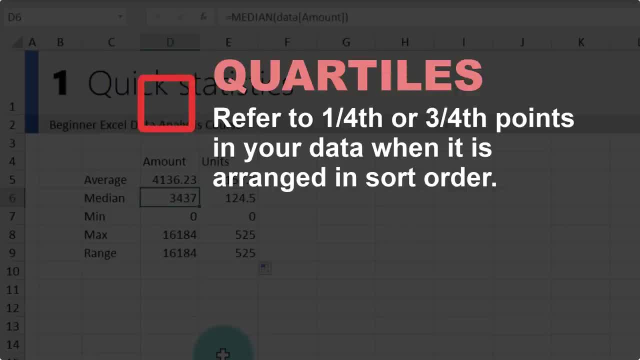 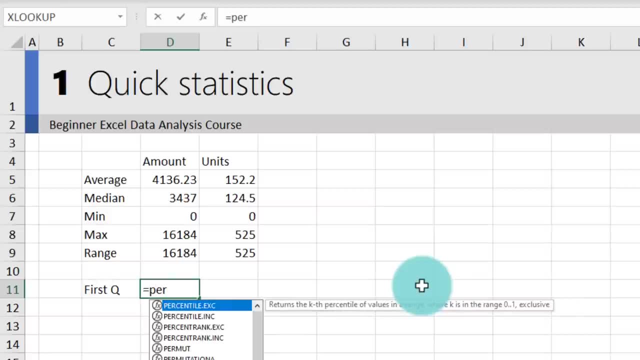 median refers to the middle point of the data. quartile would refer to the one-fourth or the three-fourth points of the data. So first quartile would be: you can use the percentile formula, So we'll say data amount, then the k will be 0.25.. What this number suggests is first one-fourth of 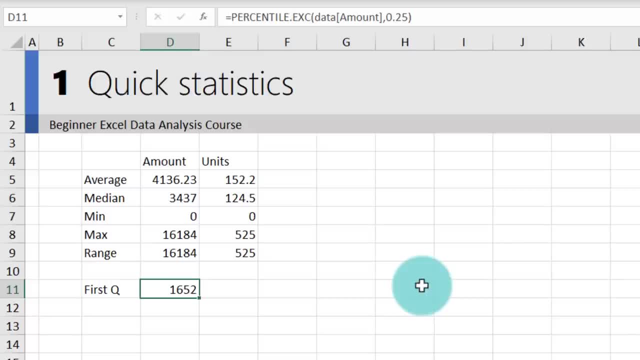 the values are less than or equal to 1652.. You can also calculate the third quartile, which would be a similar formula. So I can copy this formula. and then I can calculate the percentile, So I can copy this formula. To copy the formula from the above cell you can press ctrl c, ctrl v, but because 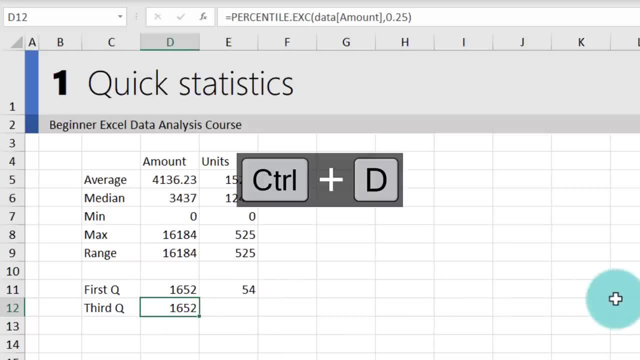 the formula is already in the cell above. I can press ctrl d to copy it down, D for down, and I'll get the same formula here. All I have to do is change this to 75 and we will get that number Again. you can see that what this number suggests is top. one-fourth of the values are above 6245.. 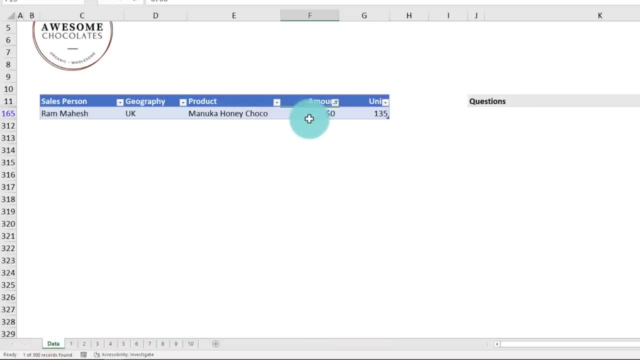 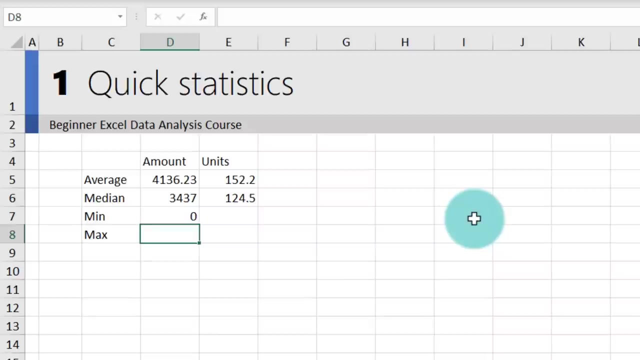 then filter for the $0 to see that there is actually indeed one row where we made $0, selling 135 units. At this point, you may want to go back and check your original data to see if this is actually correct, or maybe there is something wrong here. Likewise, max is max of data amount. 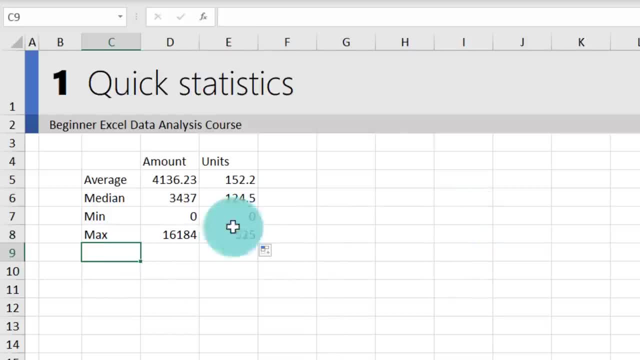 Another common metric that we calculate in statistics is range. Range is nothing but the distance between minimum and maximum. So we can say max minus min and that will be the range. In this case, because our minimum is $0, range is nothing but max. You can also calculate the quartiles, Just as median refers to the middle. 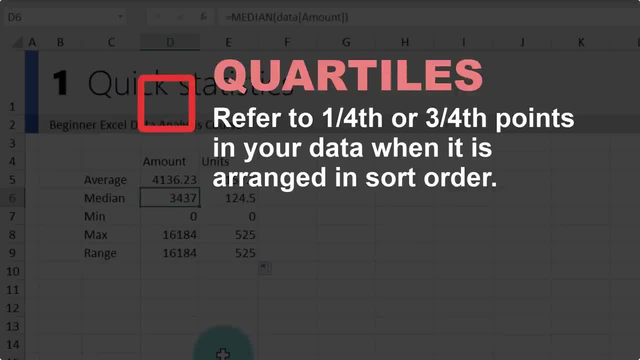 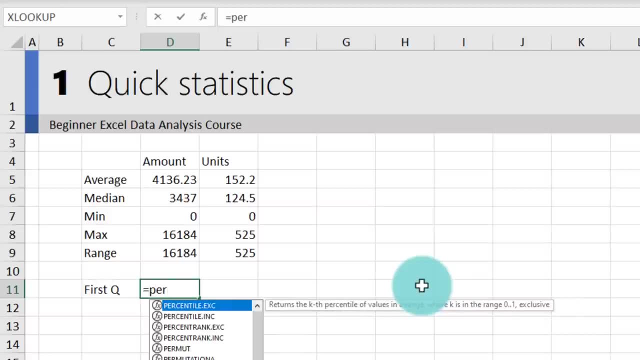 point of the data quartile would refer to the one-fourth or the three-fourth points of the data. So first quartile would be: you can use the percentile formula, So we'll say data amount and then the k will be 0.25.. What this number suggests is first one-fourth of the values. 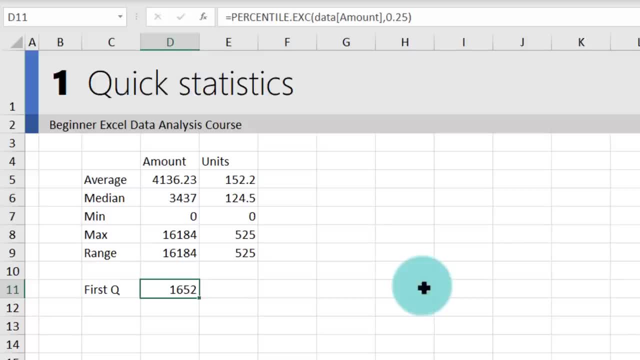 are less than or equal to 1652.. You can also calculate the third quartile, which would be a similar formula. So I can copy this formula. To copy the formula from the above cell, you can press control C, control V, but because the formula is already in the cell above, I can press. 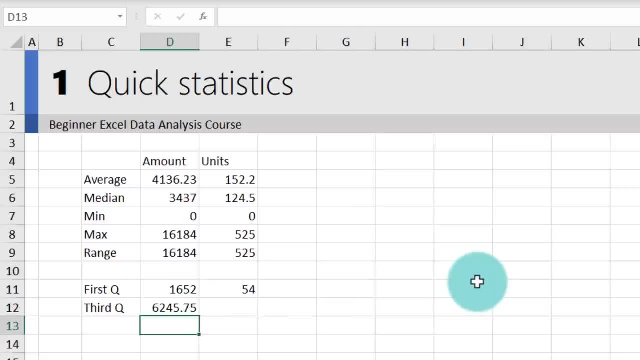 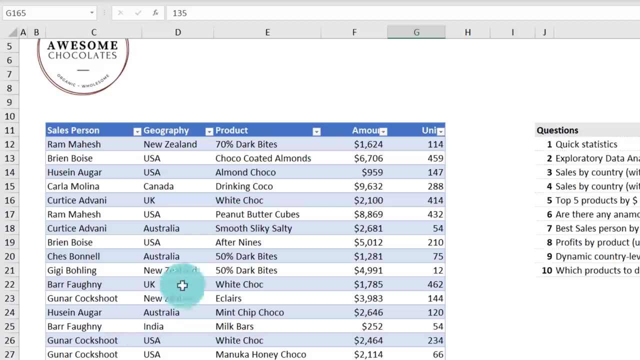 control V, So I can copy this formula Here. all I have to do is change this to 75 and we'll get that number Again. you can see that what this number suggests is top one-fourth of the values are above 6245.. You can also calculate the distinct counts to see how many different salespeople 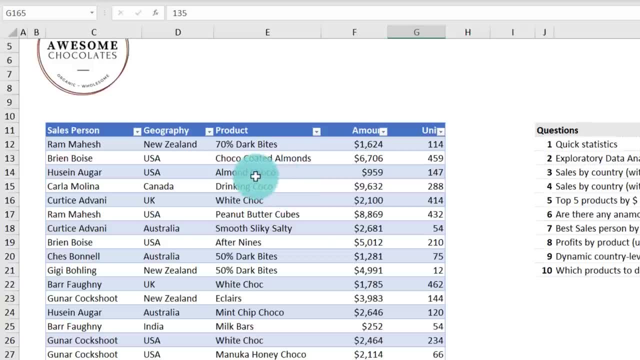 geographies and products are there in the data. I normally don't do that kind of analysis unless I need to specifically look for something. but another quick way of doing this is you can apply. quick shortcut to enable the filters on your data is to select any cell in the table and then press. 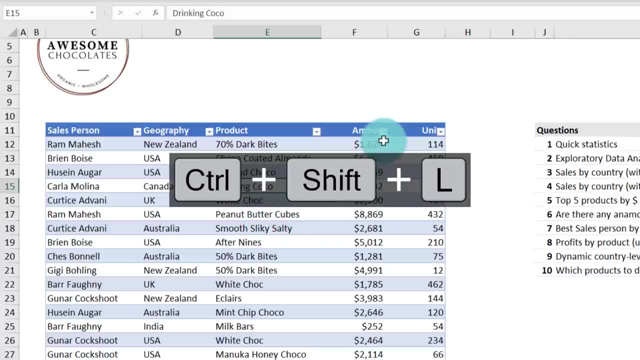 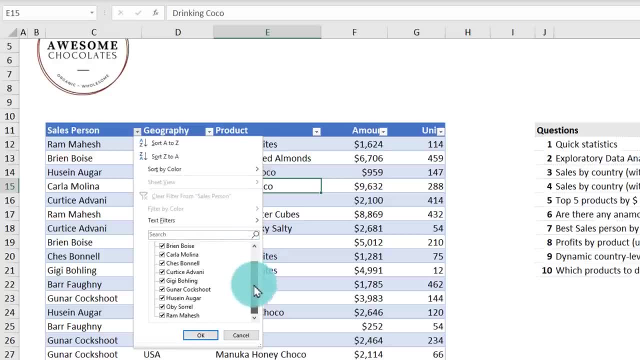 control, shift L. If you press it once, the filters will be added, and then, if you press it again, they will go off. So once you have such filters you can just click on that little arrow to quickly scan and see how many items are there. We seem to be having about 10 salespeople, five or six. 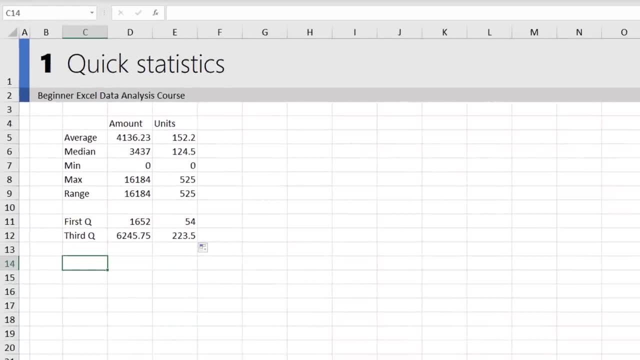 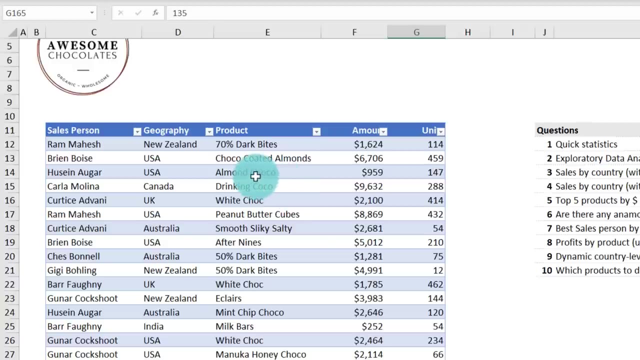 You can also calculate the distinct counts to see how many different sales, people, geographies and products are there in the data. I normally don't do that kind of analysis unless I need to specifically look for something, But another quick way of doing this is you can apply. 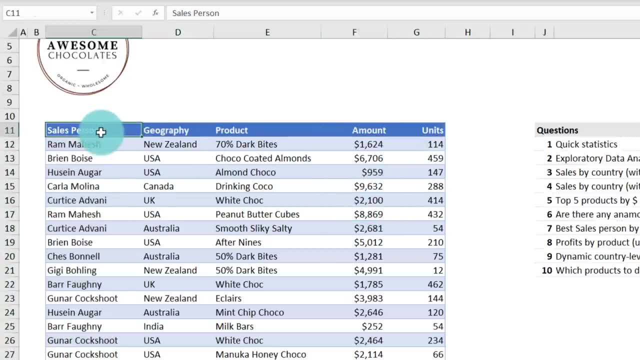 filters on your original table. A quick shortcut to enable the filters on your data is select any cell in the table and then press ctrl shift l. If you press it once, the filters will be added and then if you press it again they will go off. So once you have such filters you can just click on. 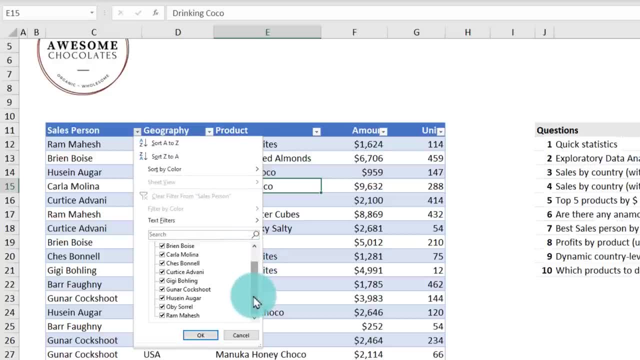 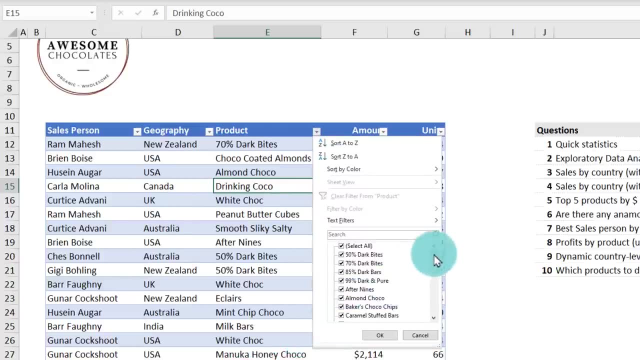 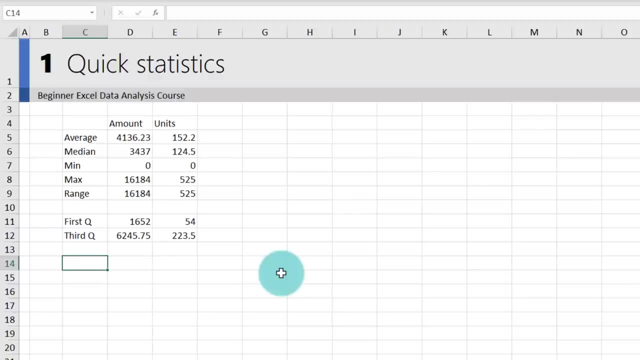 that little arrow to quickly scan And see how many items are there. We seem to have be having about 10 sales people, five or six different geographies, but we have a whole heap of different products. If you simply want to calculate how many products are there using a formula, you can use the unique. 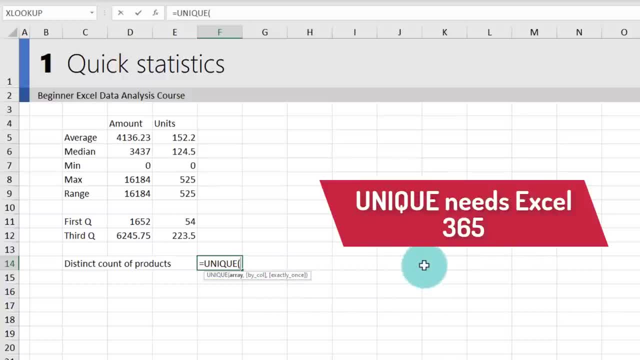 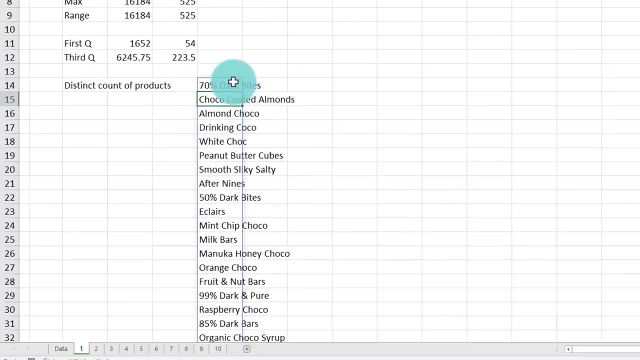 function that is newly introduced into excel. This will only work in excel 365. and then you say unique of data product. What unique will do is it will give you a listing of all the products, one per row. If there is repetitions, it will remove them automatically and it will give you this list. 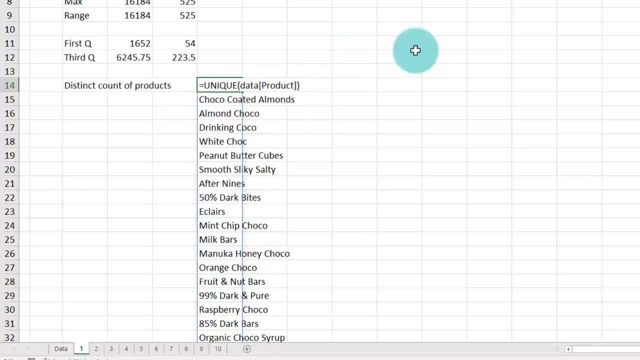 Since we don't want to see the names, we just want to count them. You can then take that and press pass it to the count a function. This will count how many products are there, and then you can see that there are 22 different products that we are selling. So that is how you can do some quick. 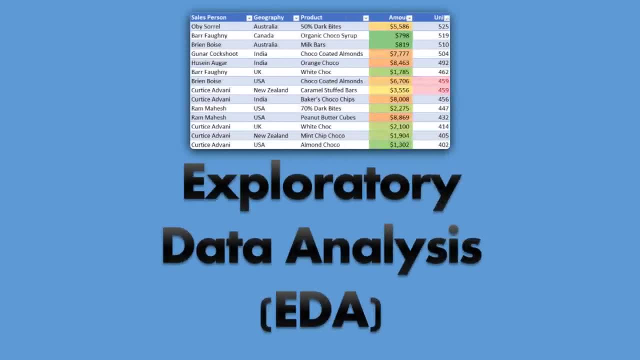 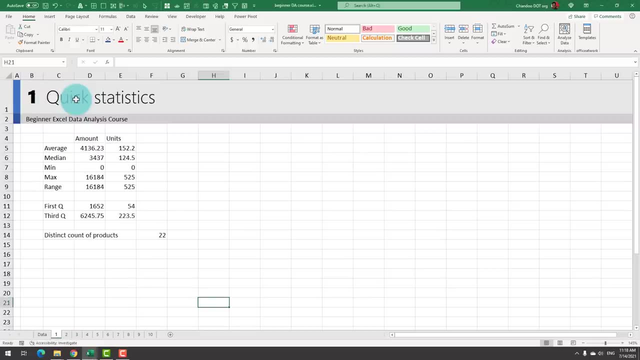 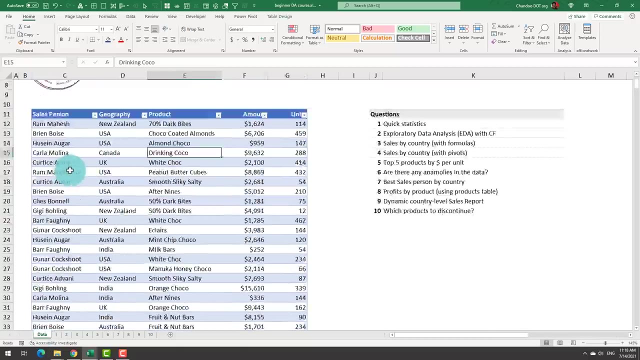 statistical analysis using excel formulas. For our second example, we are going to do exploratory data analysis with conditional formatting, And you normally the exploratory analysis at the start of your data analysis work when you're presented with some data. So here I have some data and I don't really know which way to go. So then what we will do is we: 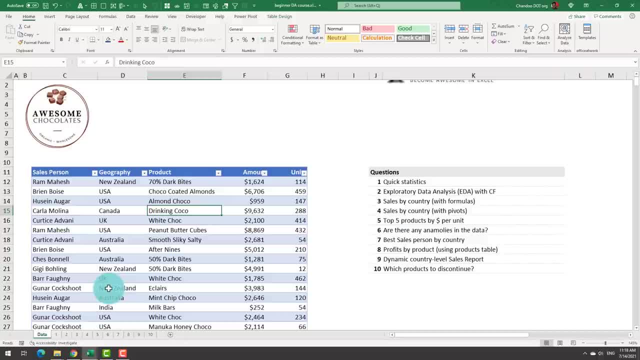 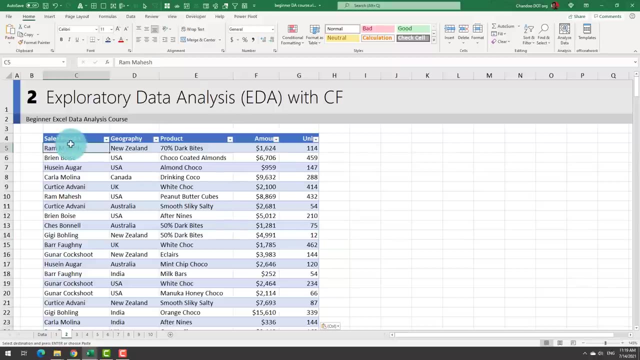 calculate some quick statistics. We will ad hocly explore the data to understand and get a feel of what we have to work with. So I'm going to just quickly copy my data and I'll paste it here So we have a copy of the data to work with. Just quickly adjust column widths and remove the. 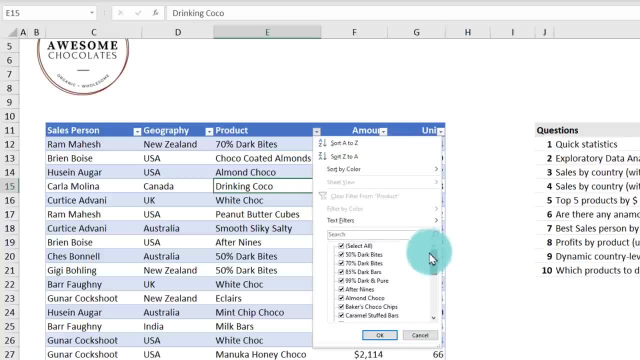 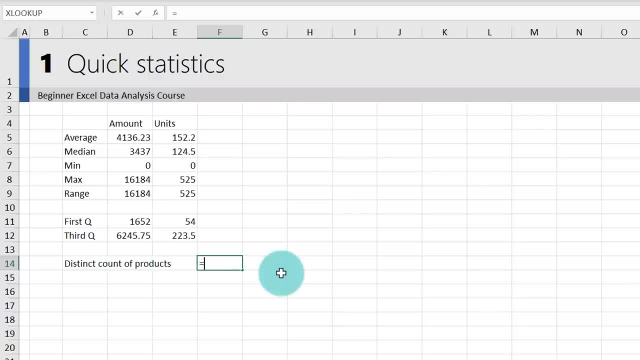 different geographies, but we have a whole heap of different products. If you simply want to calculate how many products are there using a formula, you can use the unique function that is newly introduced into Excel. This will only work in Excel 365. and then you say unique of data. 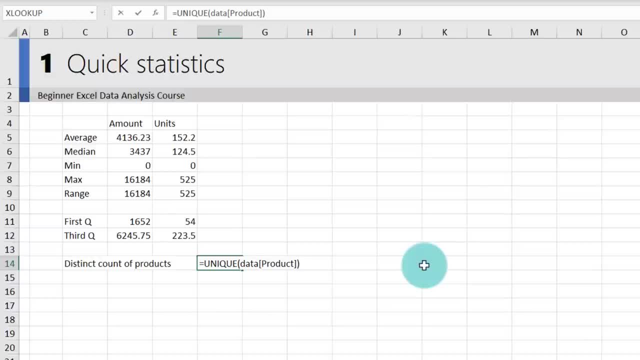 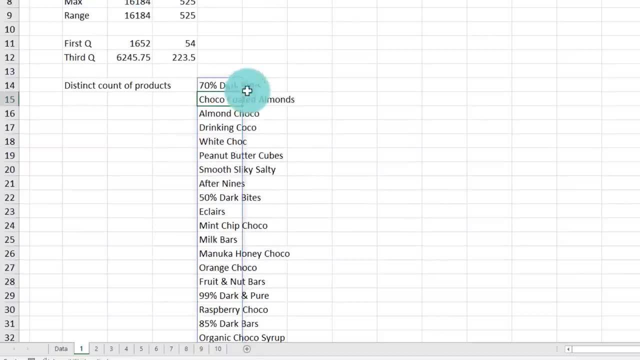 product. What unique will do is it will give you a listing of all the products, one per row. So if there is repetitions, it will remove them automatically and it will give you this list. Since we don't want to see the names, we just want to count them. You can then take that and 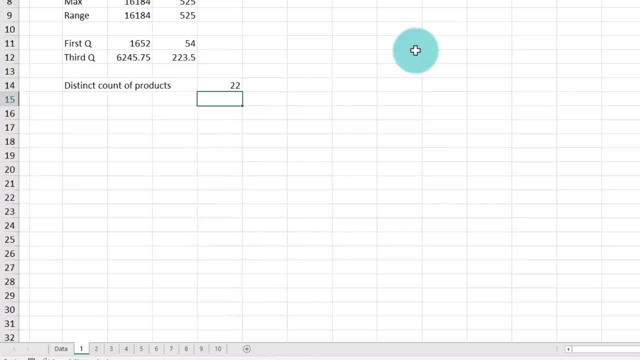 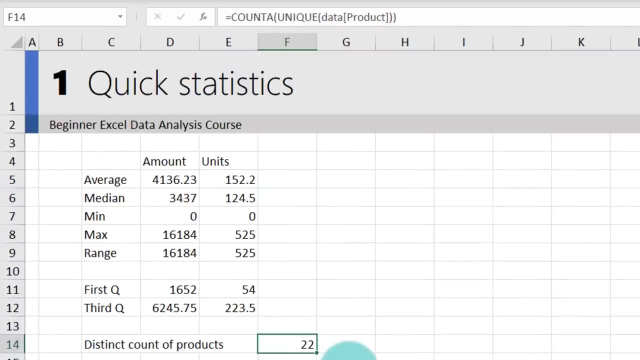 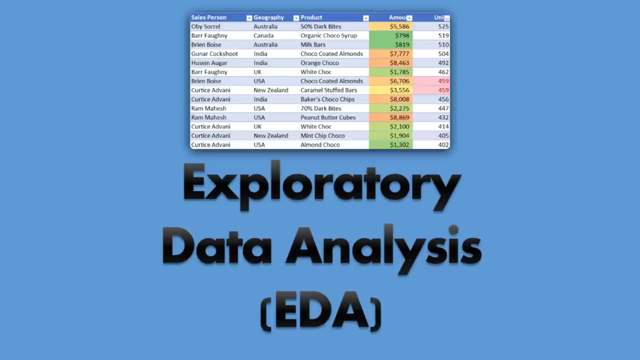 pass it to the counter A function. This will count how many products are there and then you can see that there are 22 different products that we are selling. So that is how you can do some quick statistical analysis using Excel formulas. For our second example, we are going to do exploratory data analysis. 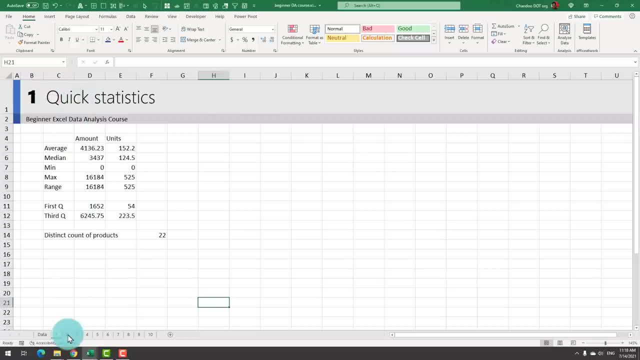 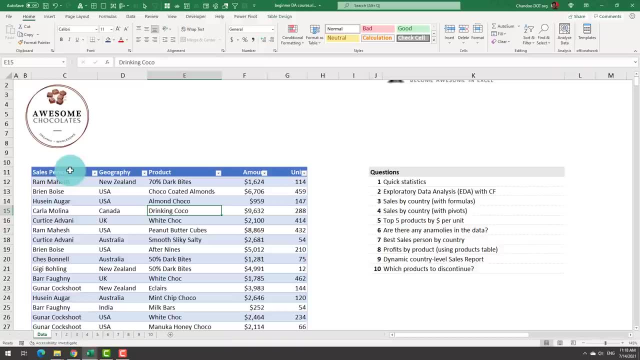 with conditional formatting and you normally do the exploratory analysis at the start of your data analysis work, when you're presented with some data. So here I have some data and I don't really know which way to go. So then, what we will do is we're going to do a little bit of 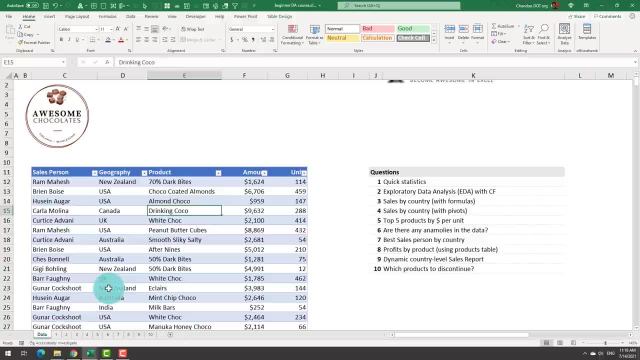 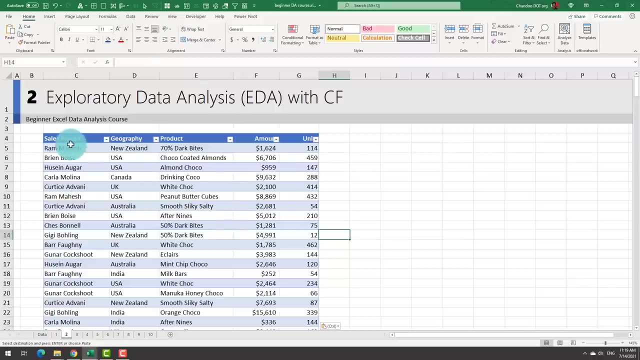 this. We calculate some quick statistics. We will ad hocly explore the data to understand and get a feel of what we have to work with. So I'm going to just quickly copy my data and I'll paste it here So we have a copy of the data to work with. Just quickly adjust column widths and remove the. 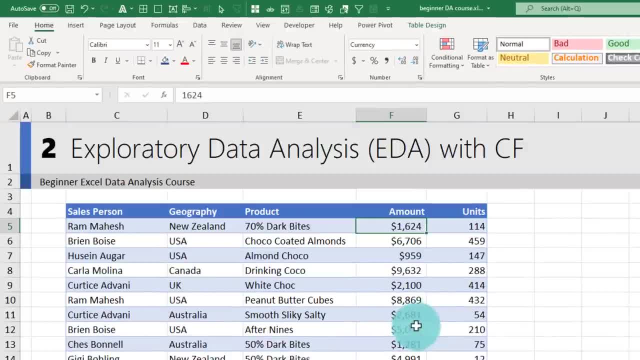 filter. So, first up, I just want to understand how wide or how varied our amounts are, So I can select the entire amount column. You can do this in a few different ways, So I'm going to do a few different ways. You can select the very first cell: press control, shift down arrow. 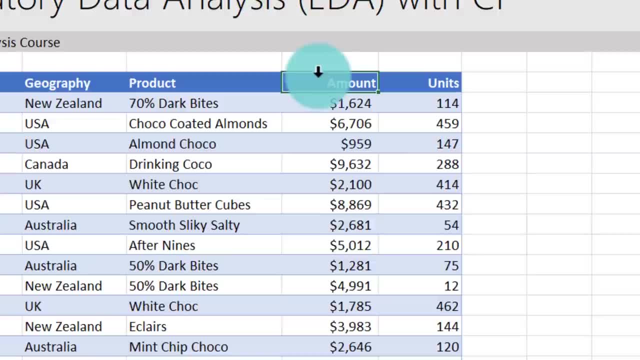 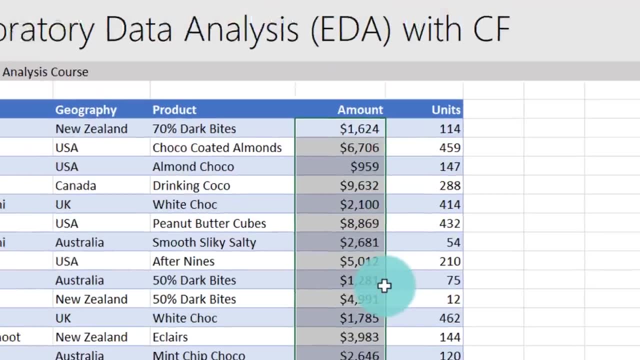 Alternatively, you can place your mouse pointer on the top row of the table And then, when the mouse pointer turns into that black arrow, just click and it will select that entire amount column. However you make that happen, select this entire amount column and then go to conditional. 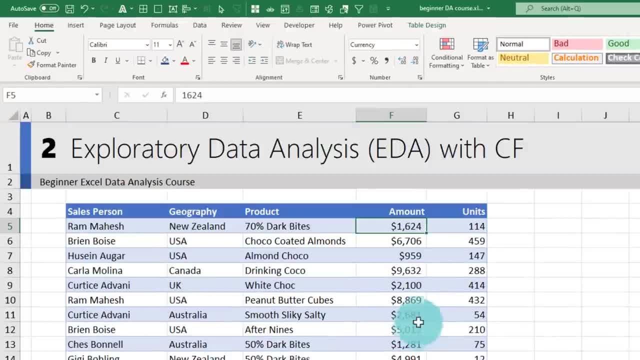 filter. So, first up, I just want to understand how wide or how varied our amounts are, So I can select the entire amount column. You can do this in a few different ways. You can select the very first cell, press ctrl, shift down arrow. Alternatively, you can place your mouse pointer on the top row. 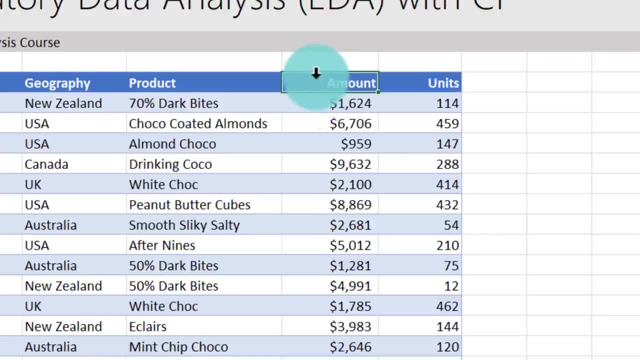 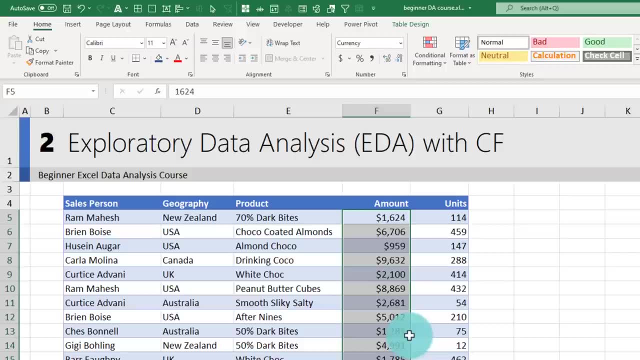 of the table and then, when the mouse pointer turns into that black arrow, just click and it will select that entire amount column. However you make that happen, select this entire amount column and then go to conditional formatting. Let's apply a color scale. Let's go. 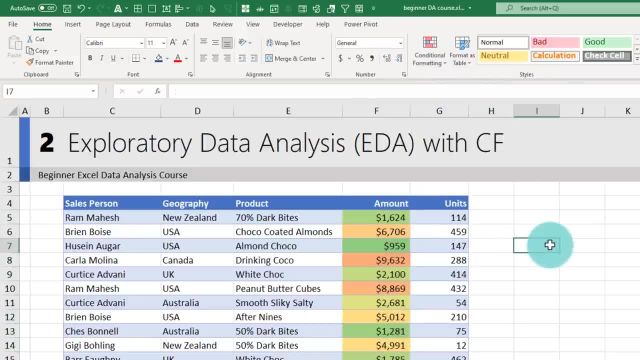 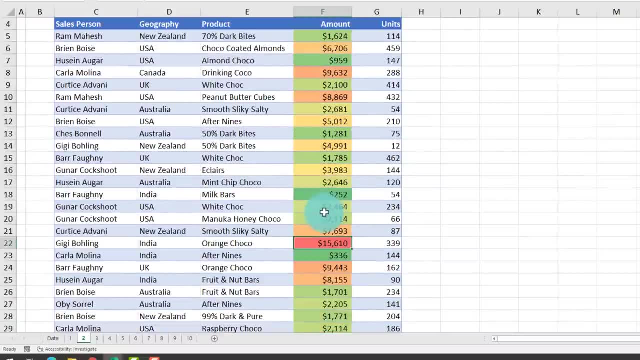 with this option. here and then it will kind of apply different colors depending on the volume of the number, and you can see that higher a number is, the redder this will be, and the lower a number is, the greener it's going to be. So this will give you an instant sense of how varied the values are. 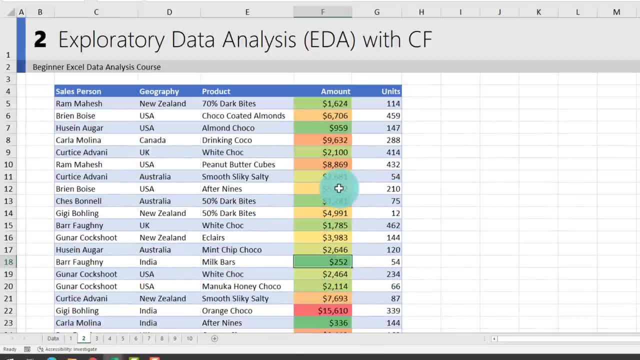 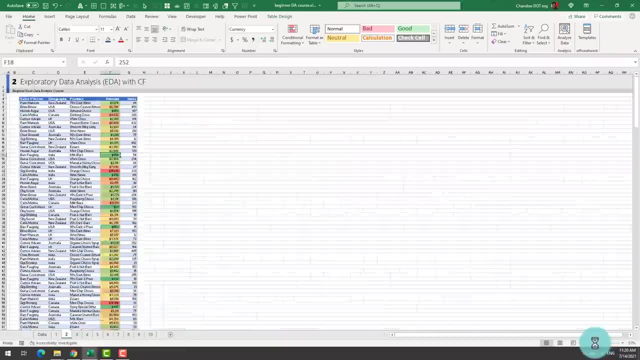 and you can see that they are kind of all over the place. But at this point, normally what I also like to do is I like to zoom down my excel worksheet all the way down so that I can kind of get a bird's eye view of my data. and here you can. 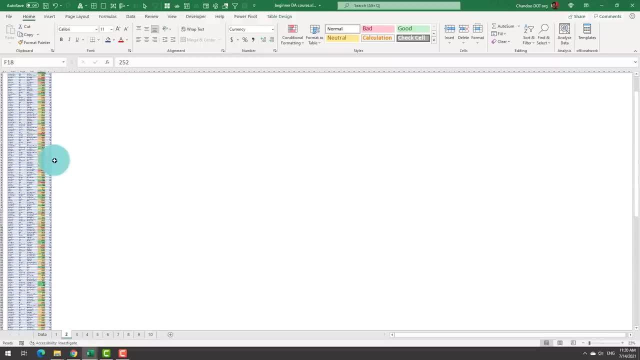 see that of course we can't read anything, but you know, occasionally it is dark red, but we are seeing a lot of green or orange color. so it's kind of like lower and middle values, but some values seem to be skewing that. Another way to analyze the data: 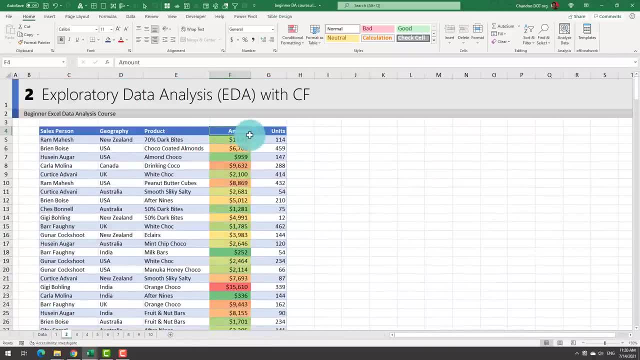 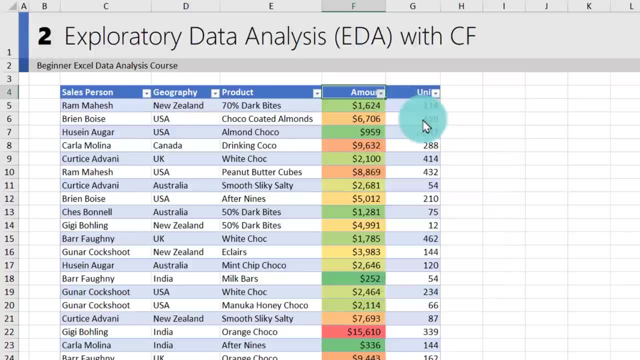 when you have applied these kind of color scale sees, you can enable the filters again. the shortcut is ctrl, shift, l and from there you can just sort it by largest to smallest to kind of get a feel of how high the numbers are, what's happening. So there is a couple of numbers. 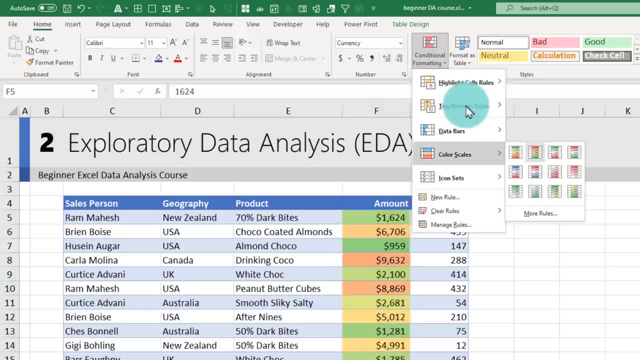 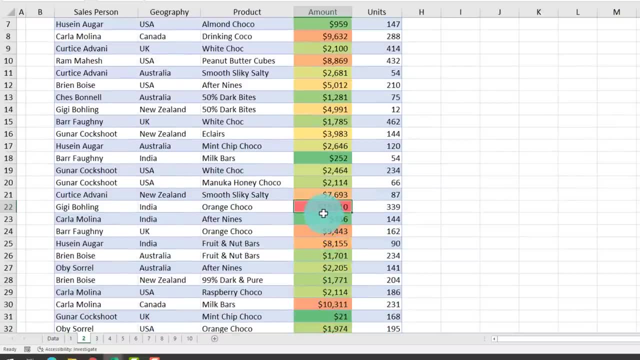 formatting. Let's apply a color scale, Let's go with this option here, And then it will kind of apply different colors depending on the volume of the number, And you can see that higher a number is, the redder this will be, and the lower a number is, the greener it's. 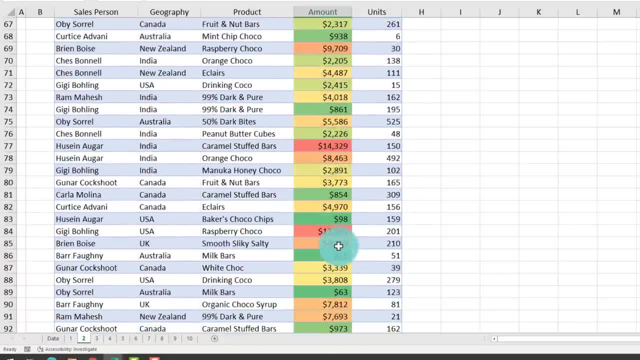 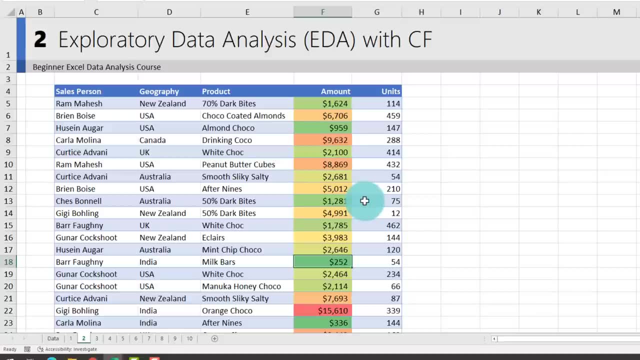 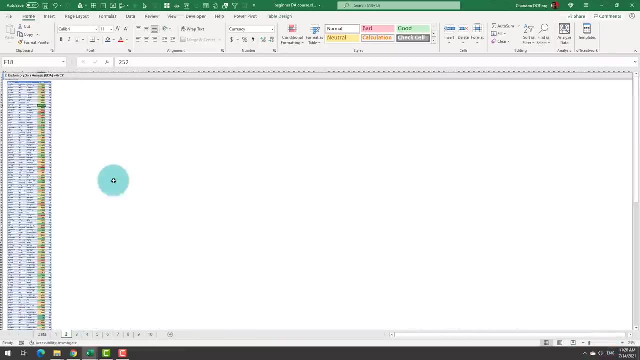 going to be. So this will give you an instant sense of how varied the values are And you can see that they are kind of all over the place. But at this point, normally, what I also like to do is I like to zoom down my Excel worksheet all the way down so that I can kind of get a bird's. 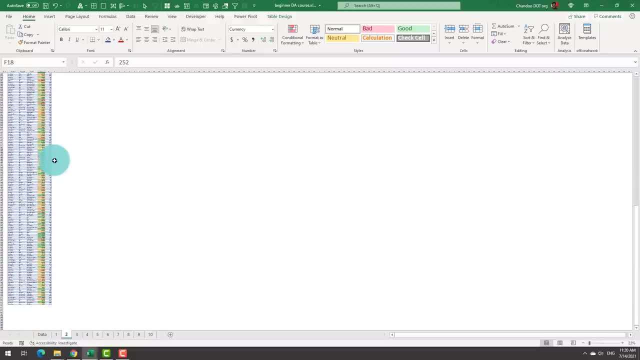 eye view of my data And here you can see that of course we can't read anything. but you know, occasionally it is dark red, but we are seeing a lot of green or orange color. So it's kind of like lower and middle values, but some values seem to be skewing that. 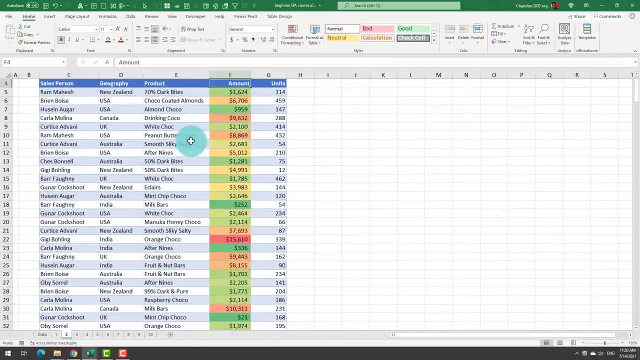 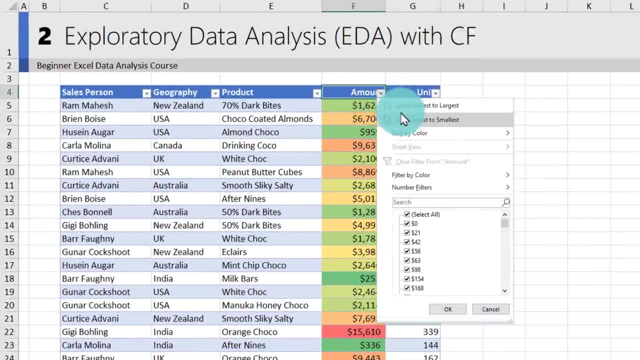 Another way to analyze the data. when you have applied these kind of color scale C's, you can enable the filters Again. the shortcut is control, shift L And from there you can just sort it by largest to smallest to kind of get a feel of how high the numbers are. what's happening? 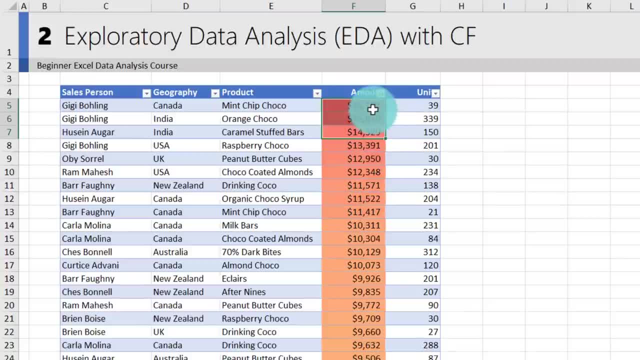 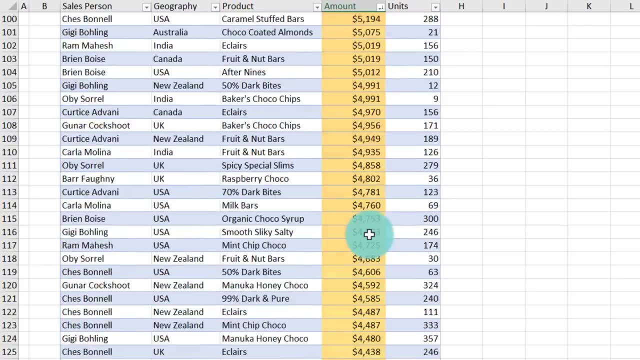 So there is a couple of numbers in the 16 and 15,000 row values, but it quickly falls down to 10,000 and then 9,000. And it seems to be settling in that ballpark of between six and 5,000 before. 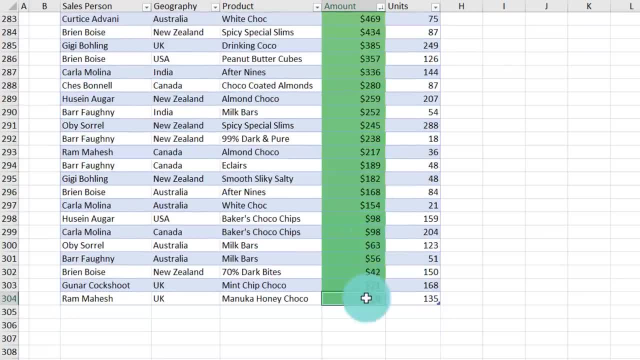 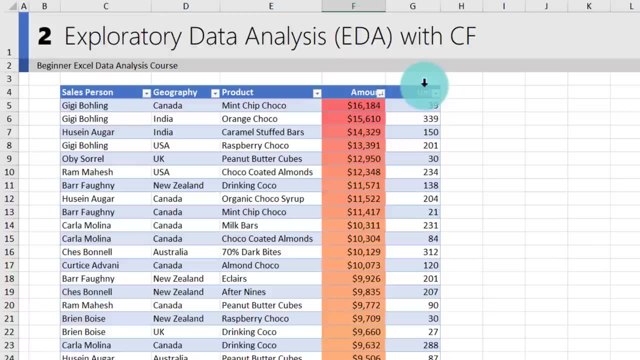 things kind of turn a little bad and go down all the way to zero. So this will also give you a solid indication of how the values are spread. You can do the same for units. For units, we're going to try something else. Select the unit column- conditional format. 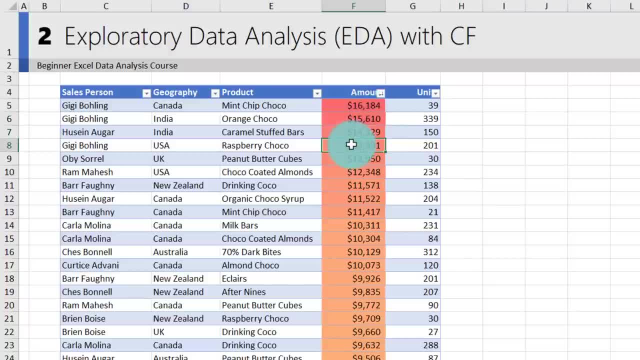 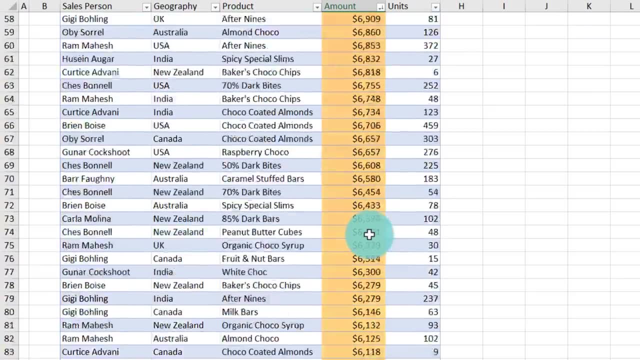 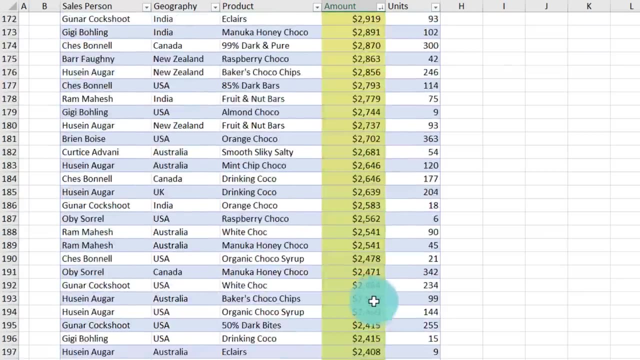 in the sixteen and fifteen thousand row values, but it quickly falls down to ten thousand and then nine thousand and it seems to be settling in that ballpark of between six and five thousand before things kind of turn a little bad and go down all the way to zero. So this will also give you a 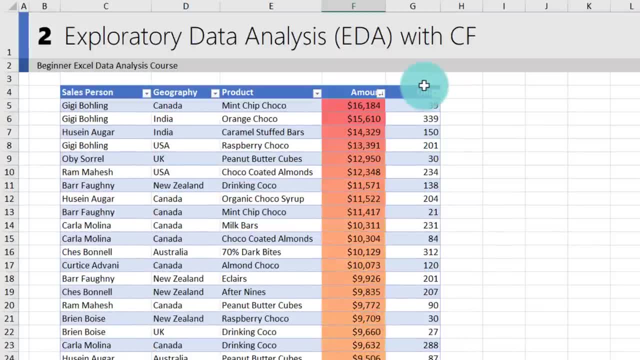 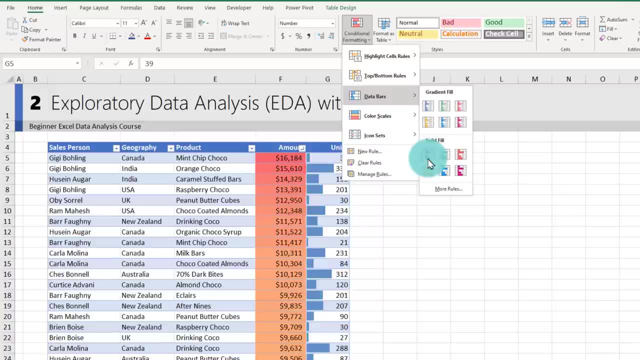 solid indication of how the values are spread. You can do the same for units. For units, we're going to try something else. Select the unit column- conditional formatting. this time let's apply data bars Again. this is also another way to visually explore the data. get a feel of how. 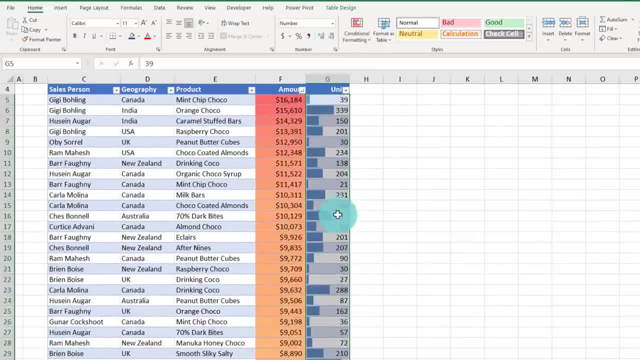 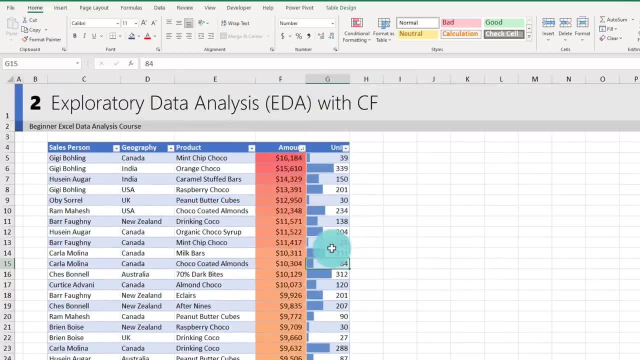 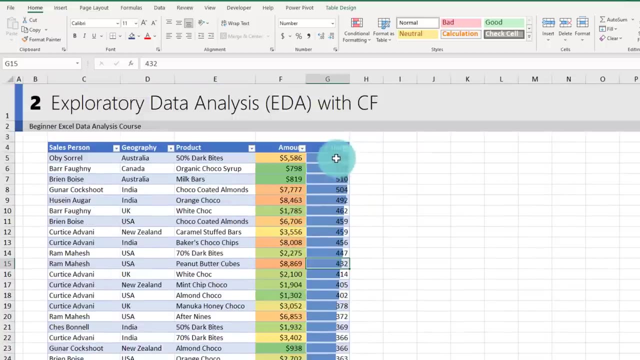 this time let's apply data bars Again. this is also another way to visually explore the data, get a feel of how big or how small these numbers are. And again we are seeing that they are all over the place, And I can apply a similar sorting here to see we are going from 525 all the way to 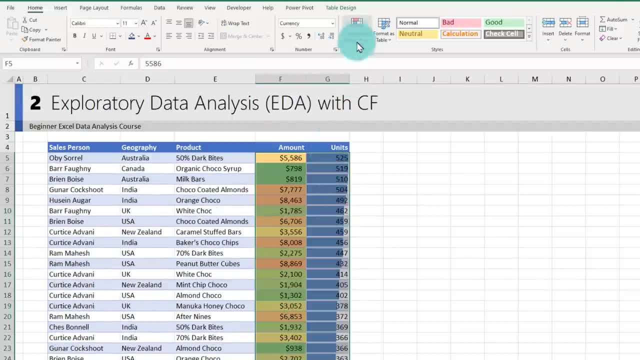 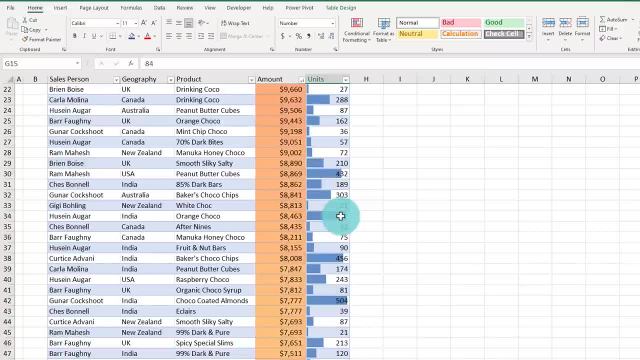 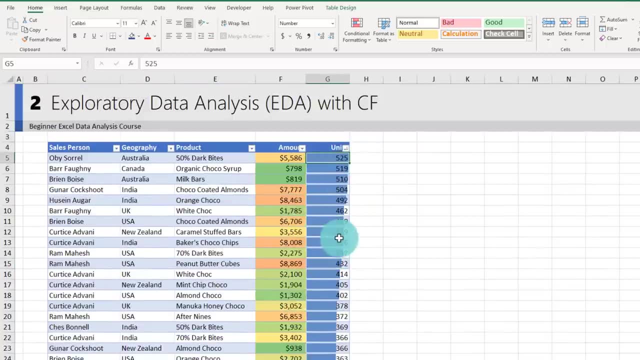 big or how small these numbers are. and again we are seeing that they are all over the place, and I apply a similar sorting here to see we are going from five hundred and twenty five all the way to zero. and let's clear away these rules so we can explore some more ways of looking at the data. 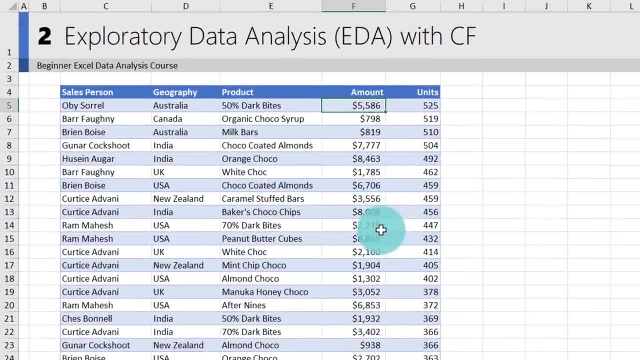 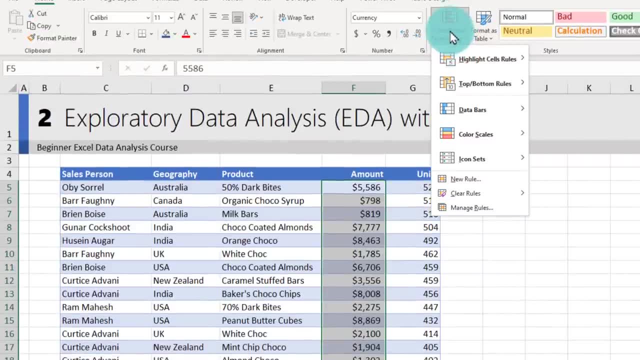 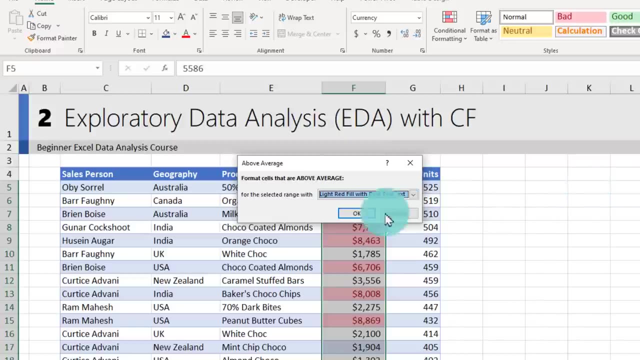 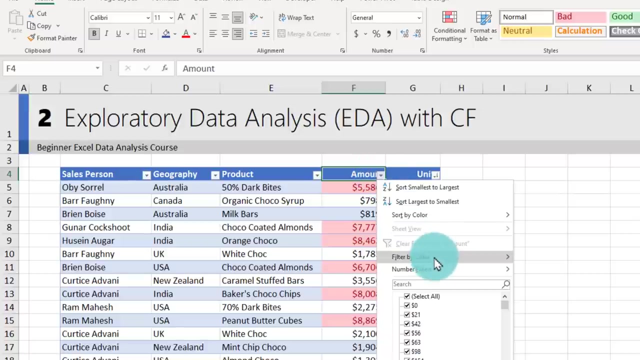 For example, I want to look at all the amounts that are above average, so I can select the amount column, highlight, cell rules- sorry, conditional formatting, top, bottom, and then I can say above average and I can leave the default color and then this will highlight all the above average values and again we can apply the filters. we can kind of filter by the color. 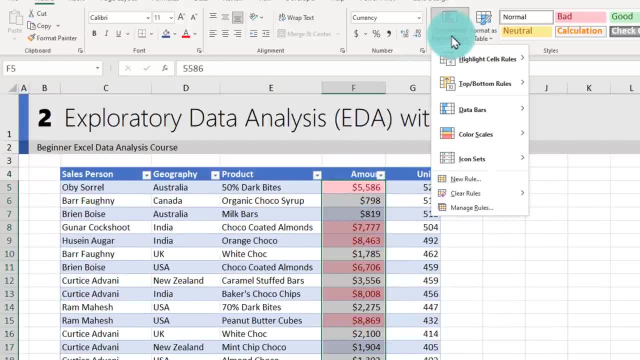 to see all the above, our age values. Another technique that you could also do is you can go high, top, bottom and you can also highlight the top 10 items. So, for example, I'm just going to clear my rule here and then apply top 10 items in the amount and. 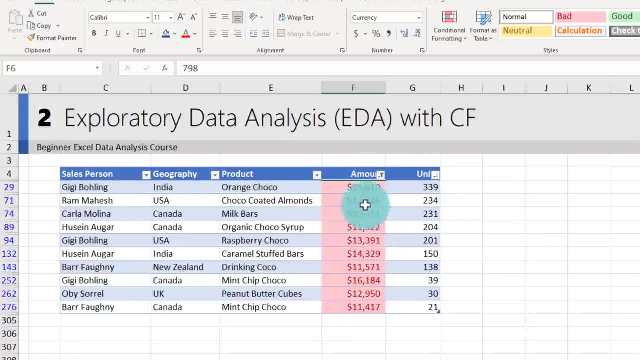 and then just filter them so that I can see who these top 10 items are, and you can see that the name gigi appeared three times. so she's probably one of our top sales person and that's why she- her name- appeared thrice in that list. If you spot any interesting trends, 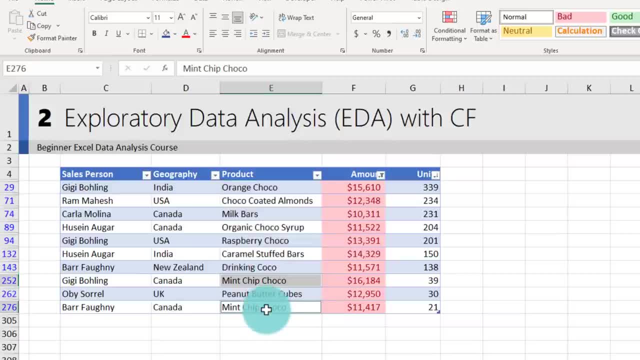 within the product names you can also get a feel like mint chip. choco appeared twice, so it seems to be one of our stronger products, again just based on the intuition that we are at this point in time. Another way to do exploratory data analysis is to see if there is. 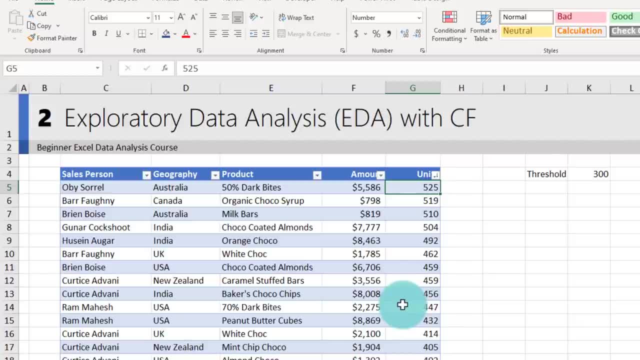 any sort of numbers that are repeating. so, for example, are there any situations where the same number of units are purchased by two different instances? so you can select the unit column, go to highlight and then duplicate values and it will highlight all the duplicate values in color so I can see four, five, nine is duplicated. three, six, six, three, four, eight. 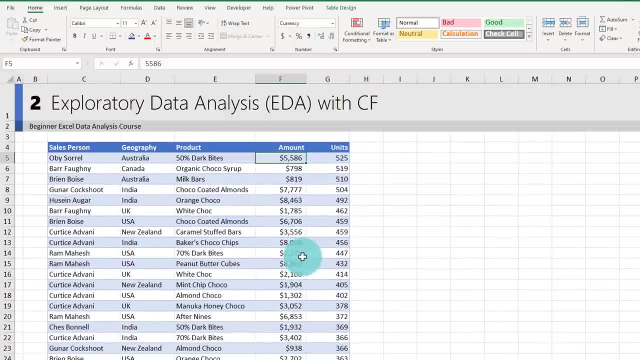 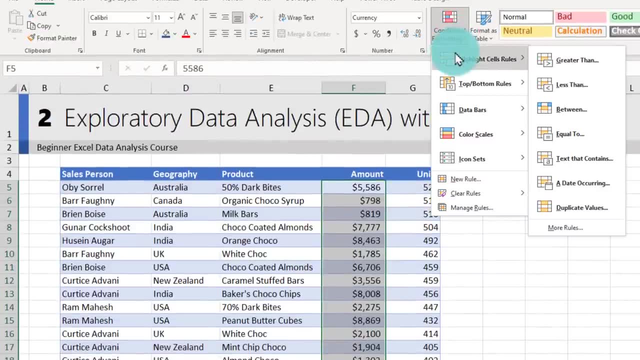 let's go ahead and do that. So let's go ahead and do that. So let's go ahead and get the data. For example, I want to look at all the amounts that are above average, So I can select the amount: column, highlight, cell rules. sorry, conditional formatting top, bottom, and then I can say above. 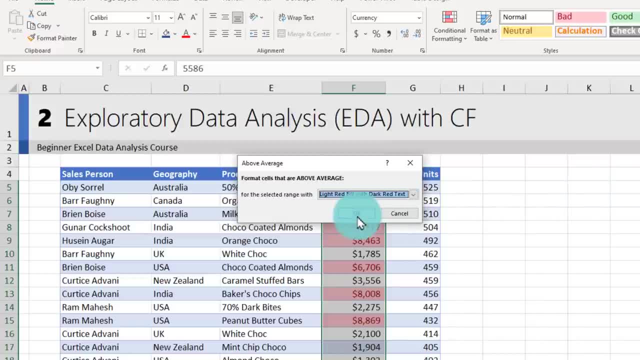 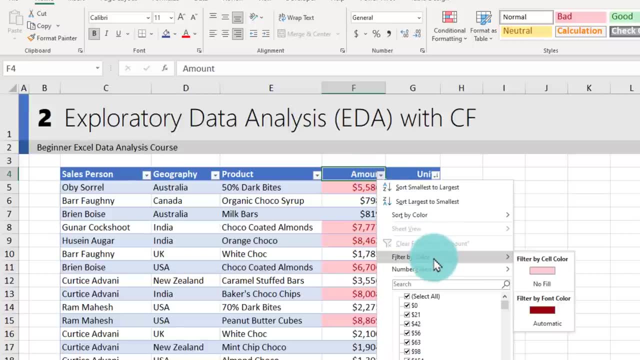 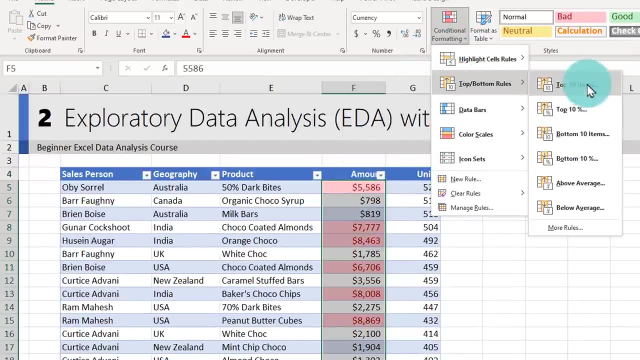 average And I can leave the default color and then this will highlight all the above average values. And again, we can apply the filters. we can kind of filter by the color to see all the above average values. Another technique that you could also do is you can go high, top, bottom and 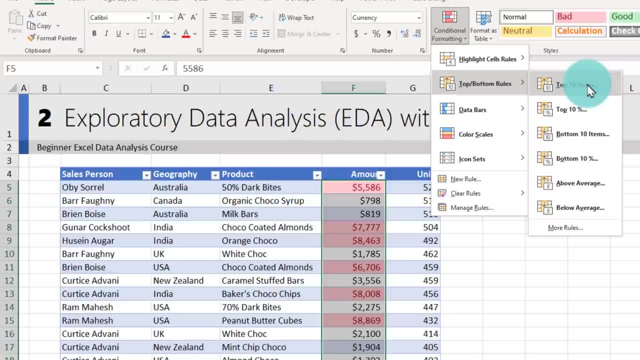 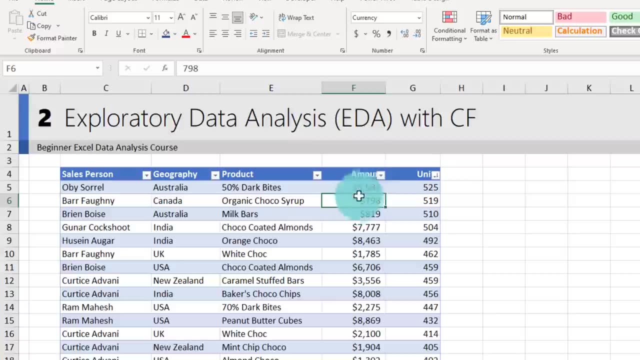 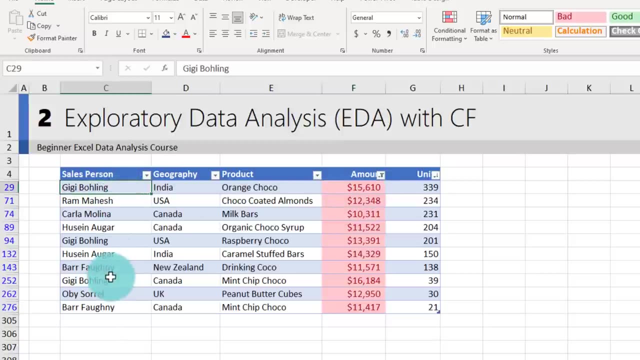 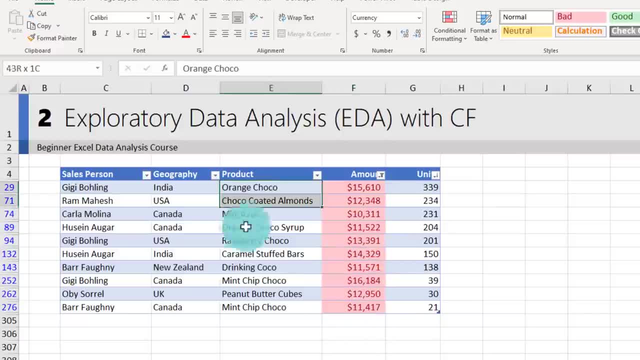 do that. So let's go ahead and do that. So let's go ahead and do that. So let's go ahead and do that. If you spot any interesting trends within the product names, you can also get a feel like mint chip, Choco appear twice, So it seems to be one of our stronger products. 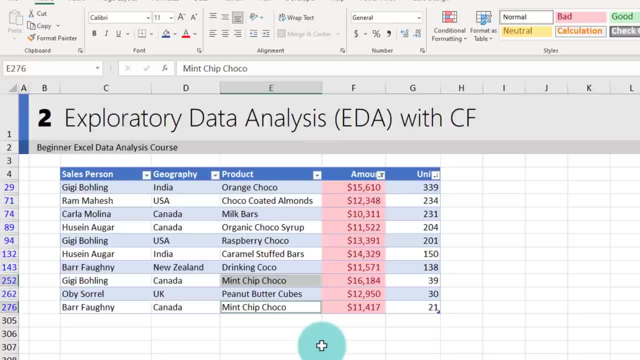 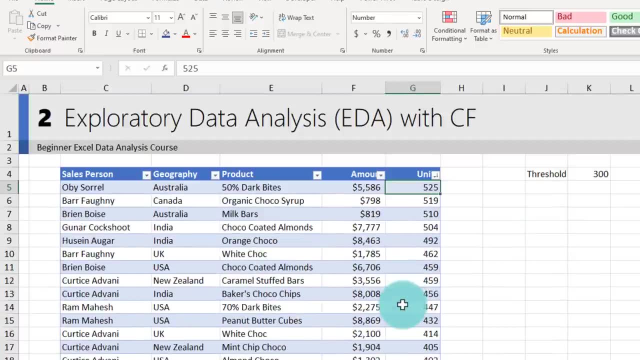 again, just based on the intuition that we are developing at this point in time. Another way to do exploratory data analysis is to see if there is any sort of numbers that are repeating. So, for example, are there any situations where the same number of units are purchased by? 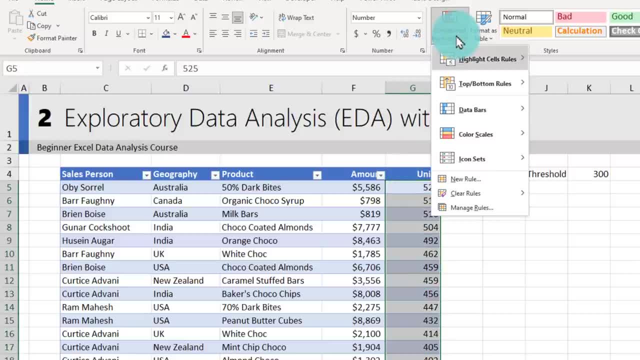 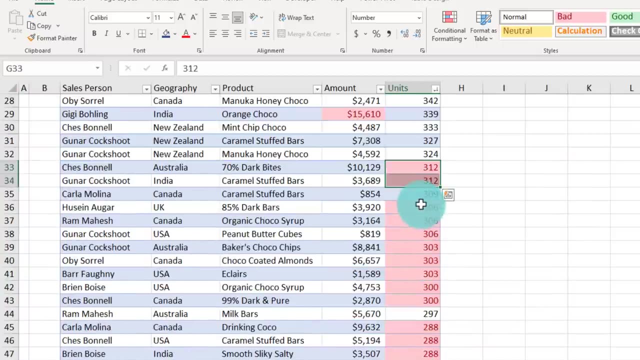 two different instances. So you can select the unit column, go to highlight and then duplicate values And it will highlight all the duplicate values in color. So I can see 459 is duplicated 366348.. And you know you'll get, for example, 306 is fairly popular- 303.. And on all of that, 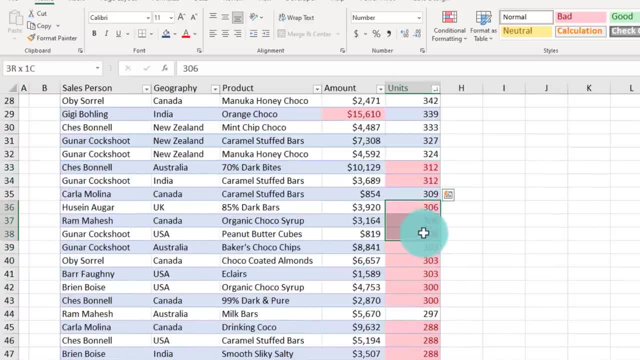 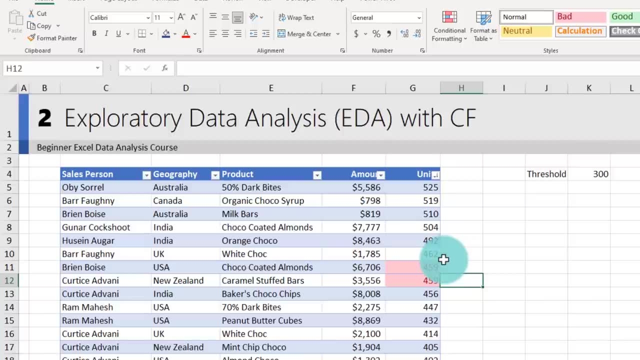 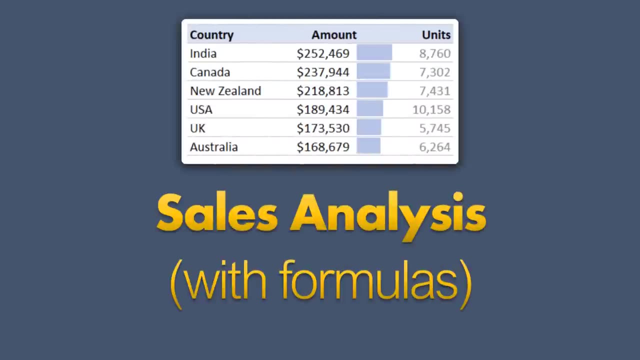 and you know you'll get, for example, 306 is fairly popular, 303 and on all of that, and that will give you a different feel for your data. so that is how you can use conditional formatting to do some exploratory data analysis. our third example: let's analyze the sales by country. so what we want: 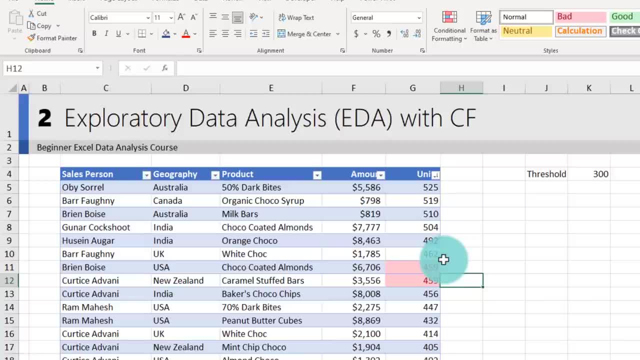 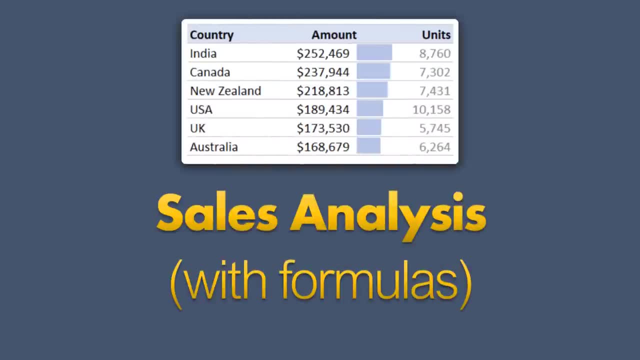 and that will give you a different feel for your data. So that is how you can use conditional formatting to do some exploratory data analysis. Our third example: let's analyze the sales by country. So what we want to do is we want to list all our countries. we just want to see. 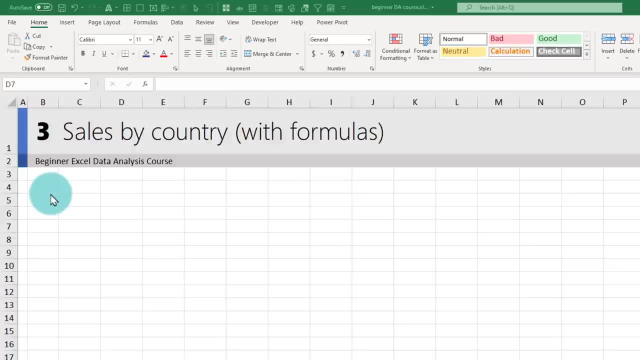 to do is: we want to list all our countries. we just want to see how much is the total amount, how much is the total units, and get a feel of that information. in this particular example, I'm going to show you how to do this with formulas. in the next example I'll show, I'll show you how to do the. 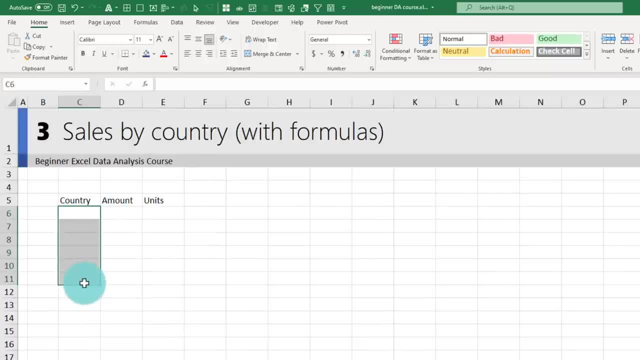 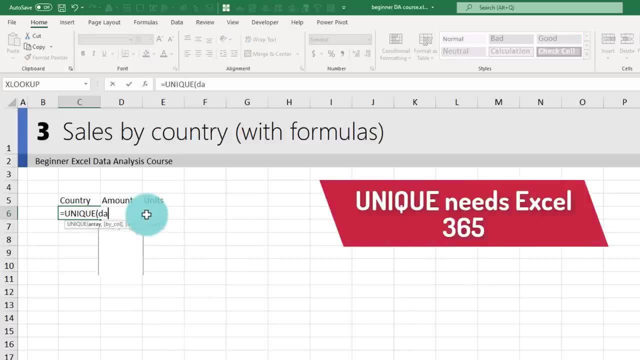 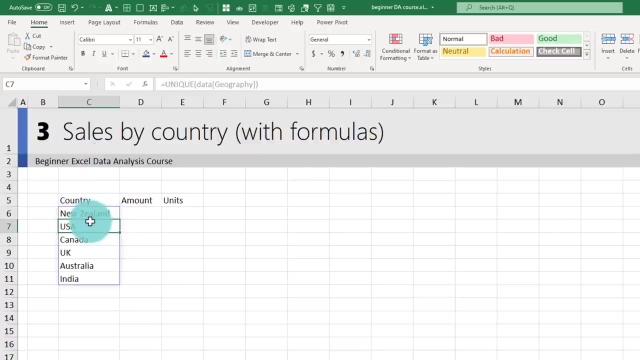 same with pivot tables, so we need to list all the countries here. there are multiple ways to do it. if you have excel 365, you should use the unique function and then say data geography to extract the country names. but if you do not have excel 365, then you are not able to use that. 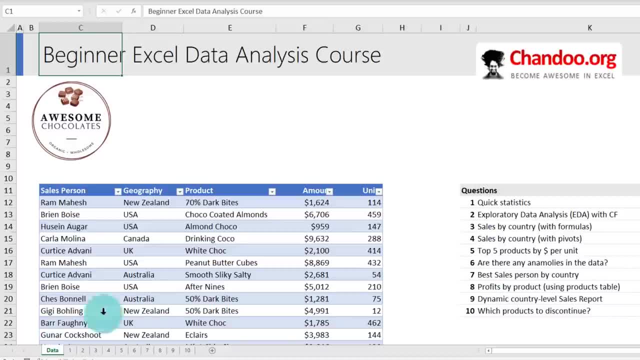 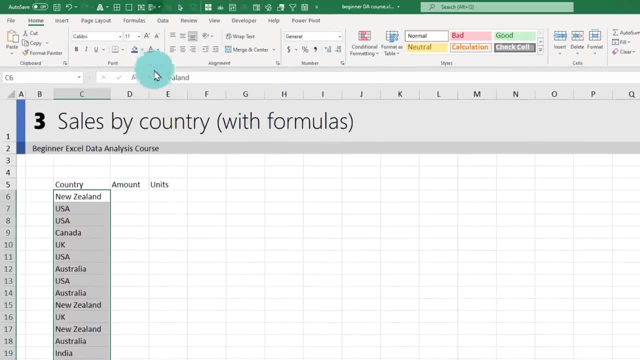 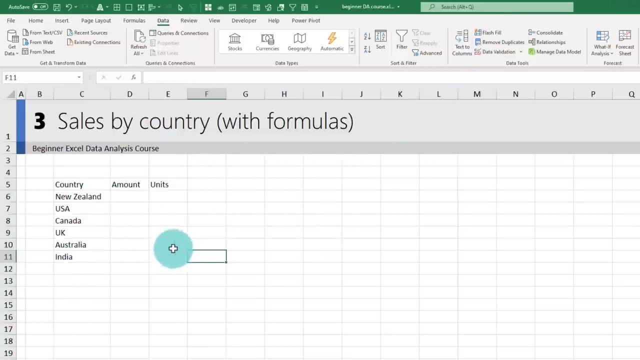 in that case, what you can also do is you can go to your data, click on geography column, copy it back here, paste it as values while keeping the whole thing selected. go to data, click on remove duplicates and it will remove the duplicates and list two items, as is here. this is manual, so if you 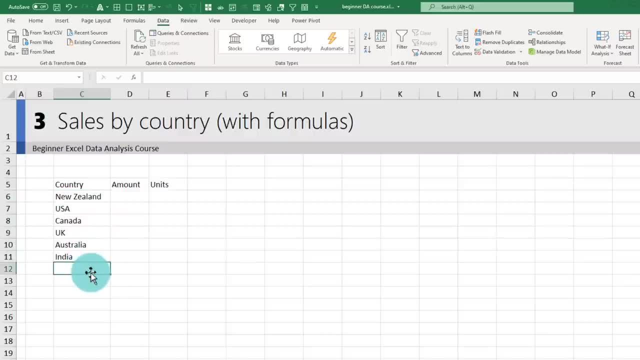 if your data changes and you end up adding one more country, you will have to come back and include that here, whereas with the unique formula it will be completely automatic. so once this is done, we need to use some formulas to find out how much is the total amount by each of these countries. 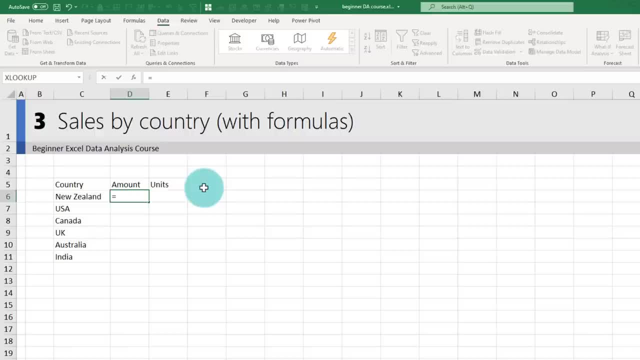 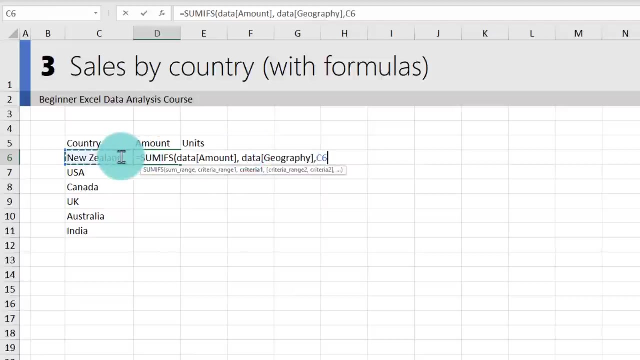 to learn is: this is one of the most important formulas when it comes to data analysis. it is the sum ifs formula. so some ifs. what do you want to sum up? amount column. so that is my data table: amount column. and then my data geography should match new zealand, so we'll say data geography. 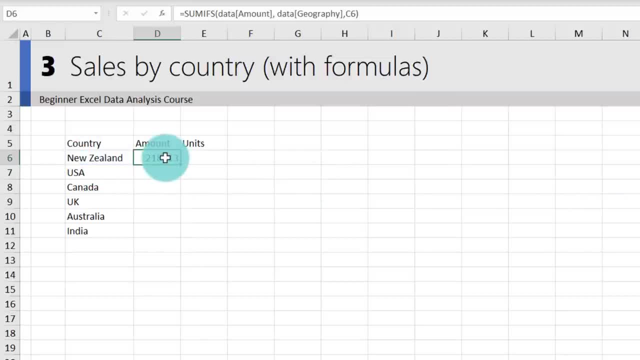 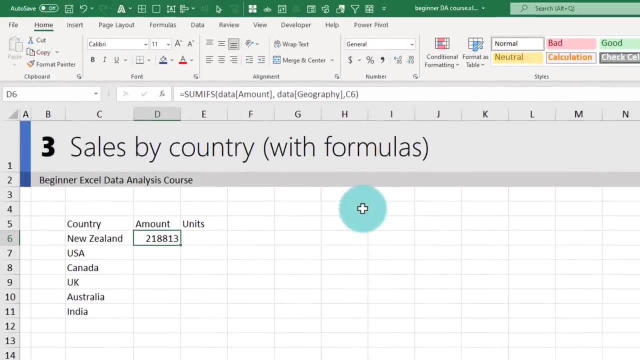 point to c6 and when you close the bracket it will get you that number. let's quickly apply some currency formatting. you can go to home, click on currency. alternatively, you can also ctrl shift 4 to apply the currency formatting with two decimal places. when you are doing analysis at, 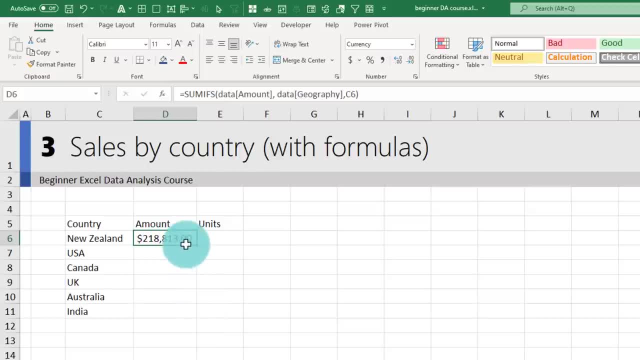 this level where the values are in hundreds and thousands. you don't need to go and show the decimal points unless somebody really asks for them. so it's a good idea to just leave it at that level and then, when you drag this down, it will give you those values. here is a handy tip: you 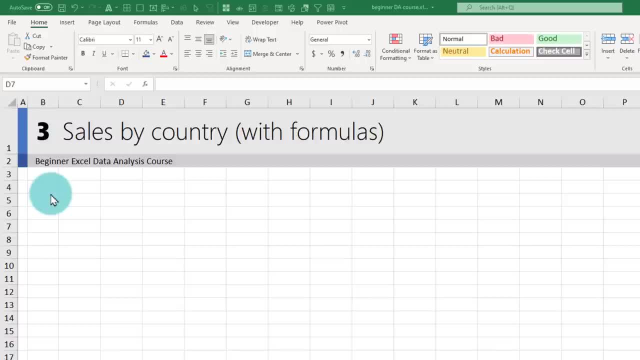 how much is the total amount, how much is the total units, and get a feel of that information. In this particular example, I'm going to show you how to do this with formulas. In the next example I'll show I'll show you how to do the same with pivot tables. So we need to list all 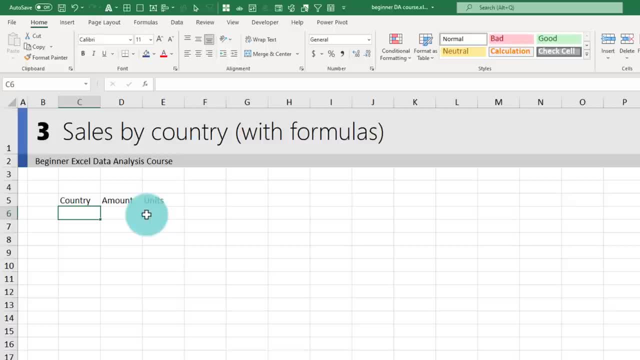 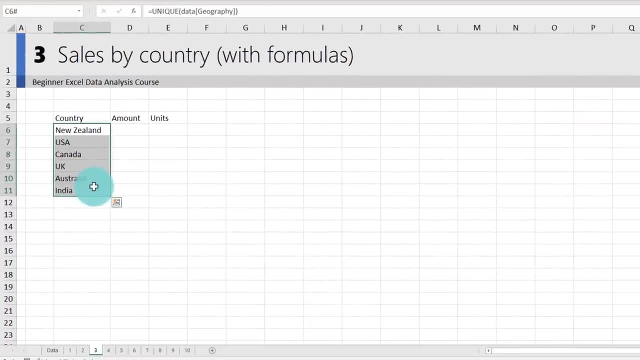 the countries here. There are multiple ways to do it. If you have Excel 365, you should use the unique function and then say data geography to extract the country names. But if you do not have Excel 365, then you are not able to use that. In that case, 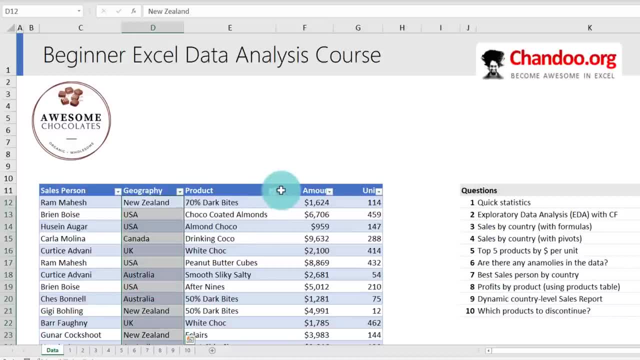 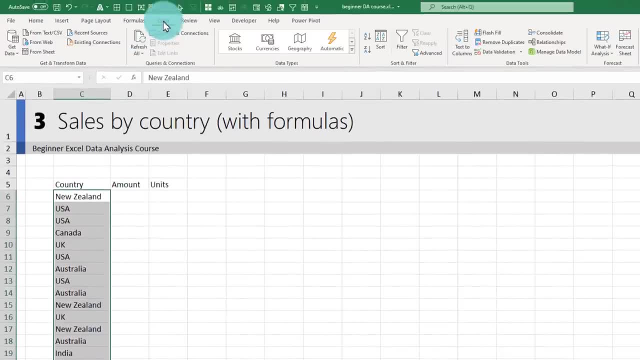 what you can also do is you can go to your data. click on geography column, copy it, come back here, paste it as values, While keeping the whole thing selected. go to data. click on remove duplicates and it will remove the duplicates and the list of items, as is here. 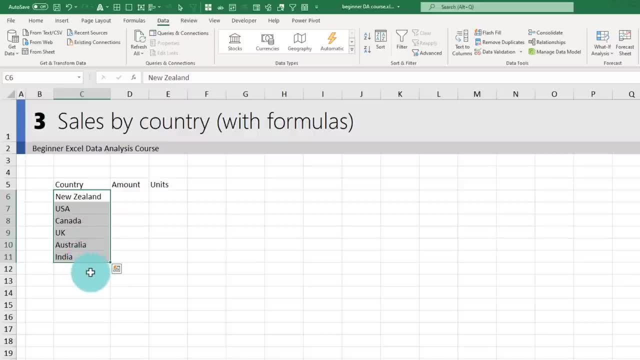 This is manual, So if you, if your data changes and you end up adding one more country, you will have to come back and include that here, Whereas with the unique formula, it will be completely automatic. So once this is done, we need to use some formulas to find out how. 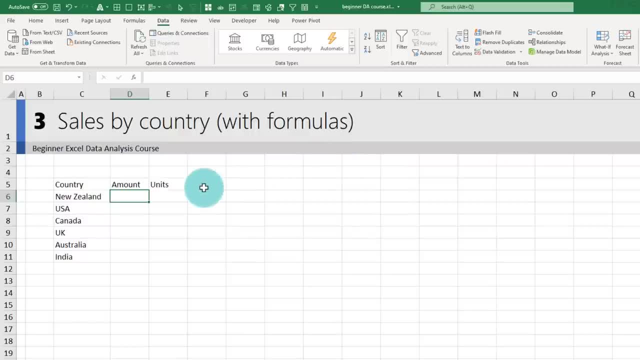 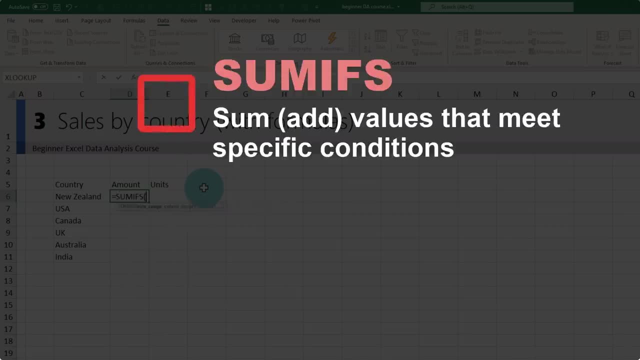 much is the total amount by each of these countries. So the formula that you need to learn is- this is one of the most important formulas when it comes to data analysis- it is the SUMIFS formula. So, SUMIFS, what do you want? to sum up, amount column. so that is my data. 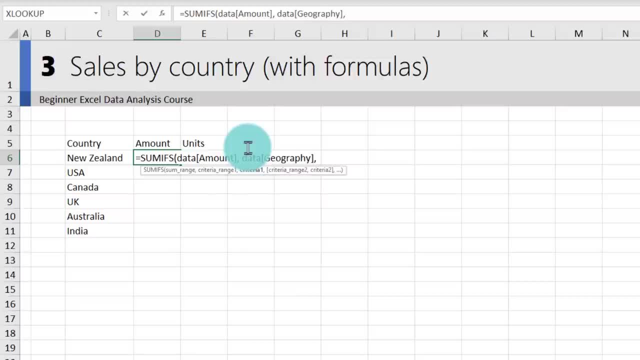 and then my data geography should match New Zealand. So we'll say: data geography point to C6. And when you close the bracket it will get you that number. Let's quickly apply some currency formatting. you can go to home. click on currency. Alternatively, you can also: 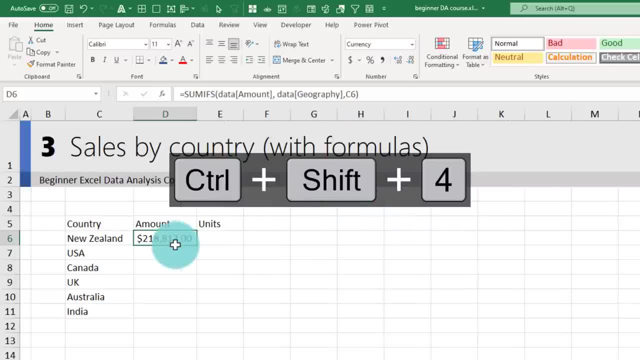 press Ctrl Shift four to apply the currency formatting with two decimal places. When you're doing analysis at this level, where the values are in hundreds and 1000s, you don't need to go and select any of these values unless somebody really asks for them. So it's a good idea to just leave. 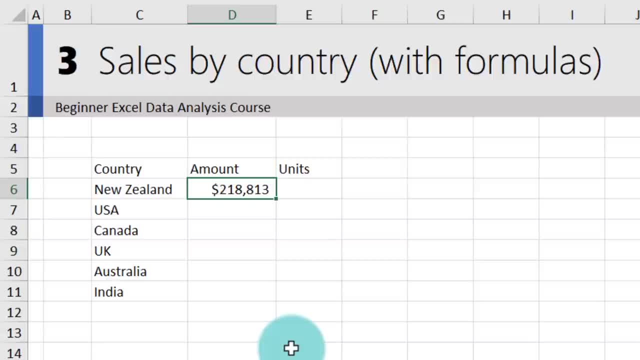 it at that level And then, when you drag this down, it will give you those values. Here is a handy tip: you don't need to drag this down. you can place your cursor at the edge And when it turns into that black plus, double click in Excel will auto fill this for you. Let's do the same for units. 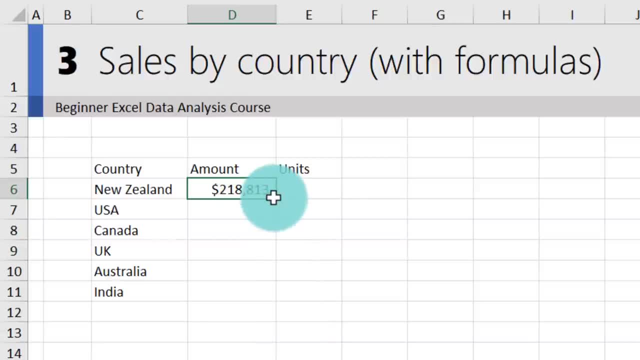 don't need to drag this down. you can place your cursor at the edge and when it turns into that black plus, double click and excel will automatically this for you. let's do the same for units. we'll say some ifs, data units. data geography is new zealand. 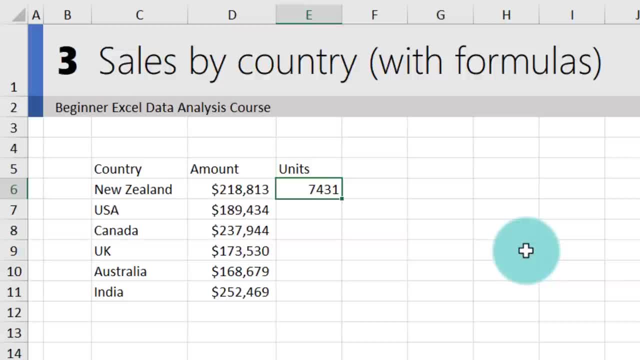 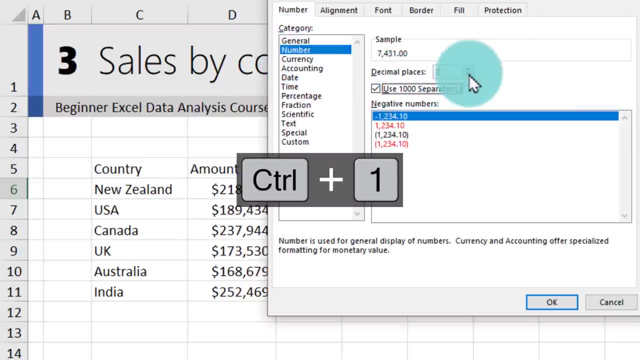 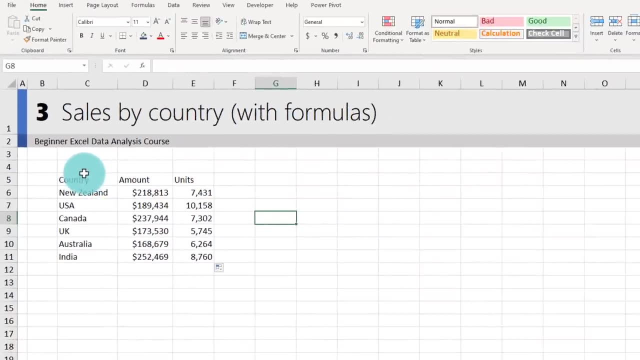 and we will apply some formatting on this. we want to just have a comma so i can select the cell. press ctrl 1 to open the format options from here. number: add a thousand separator zero decimals, click ok and then click down. so at this point this particular analysis gives you the information that 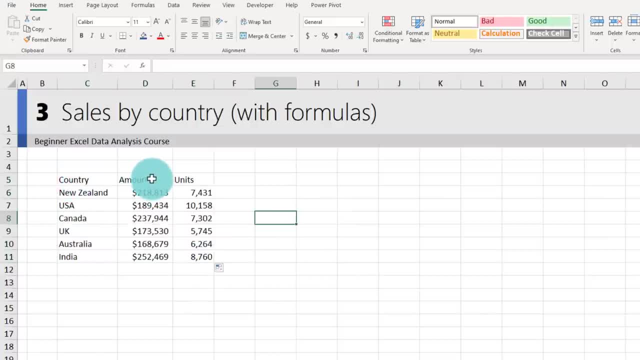 you want. while you may be happy with this, if you are preparing this for somebody else, you may want to also figure out how to present this in a better way. so what i'll do is i'll show you how to make it presentable. first up, we'll select this. we'll make a copy of this so you can see the difference. 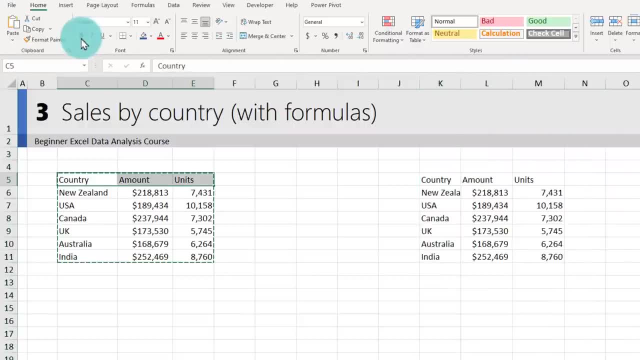 between original and polished format. i'm going to select the headers, make them bold and add a little bit of background color on that. select these two columns right, align them, because that's the numbers and that's how these are aligned. then, most important importantly, apply a sort order that is logical, so you could either sort them in alphabetical order. 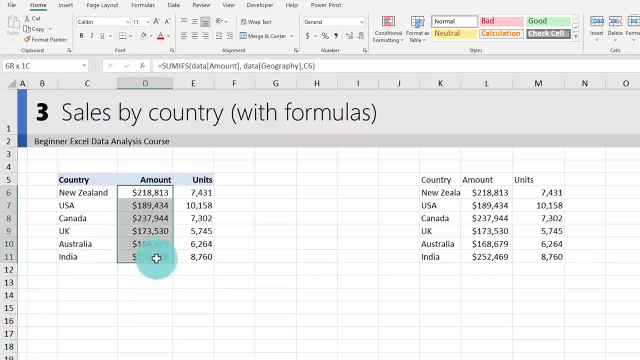 or because we are talking about sales by country. take the amount column and sort this so quickly. add filters largest to smallest and then disable the filters. so now you can see india is our best selling country in this data, followed by canada, and australia is the lowest selling country within. 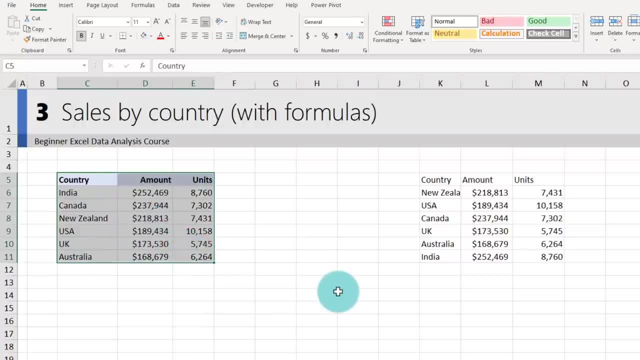 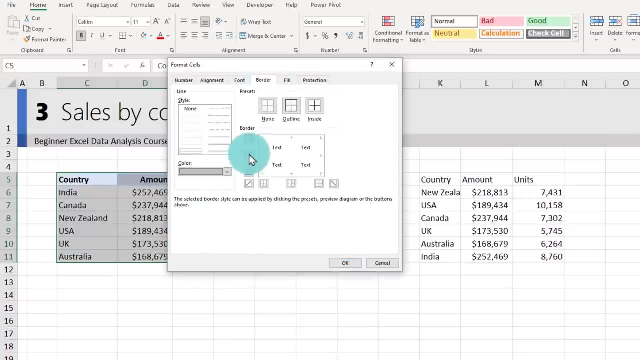 this data set. the next thing that you want to do is select all of this and add some simple borders around it. go to border and just set the color to a dull color and only add horizontal borders. now the border color kind of matches the grid line, so we can't. 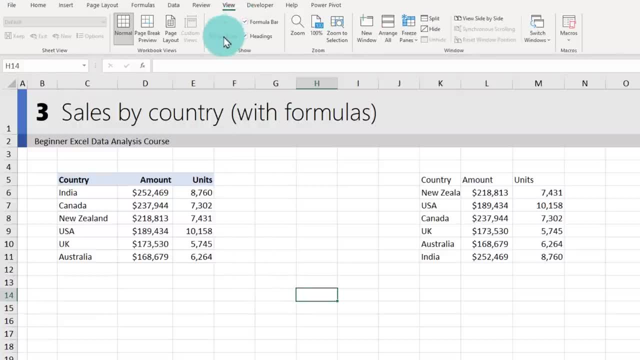 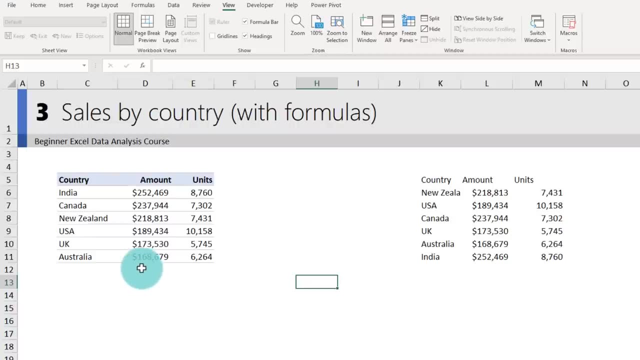 really see what is there. but if i go to view and disable the grid lines, i'll get this nice little thing. the next thing that you may want to consider is adding some additional detail to this so that it looks visually interesting. again, you can do a lot. i'll show you one technique. 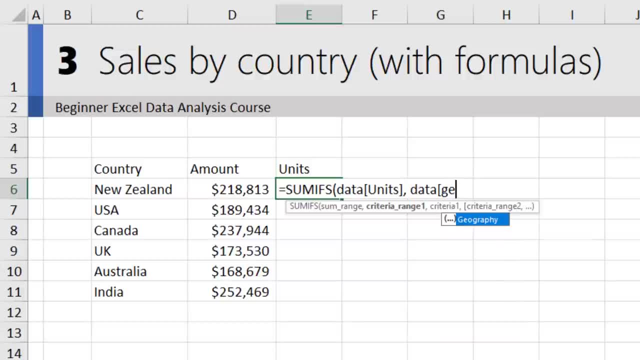 we'll say SUMIFS data units- data geography is New Zealand. we will apply some formatting on this. we will say SUMIFS data units- data geography is New Zealand and we will apply some formatting on this. we will say SUMIFS data units- data geography is New Zealand and we will apply some formatting on this. 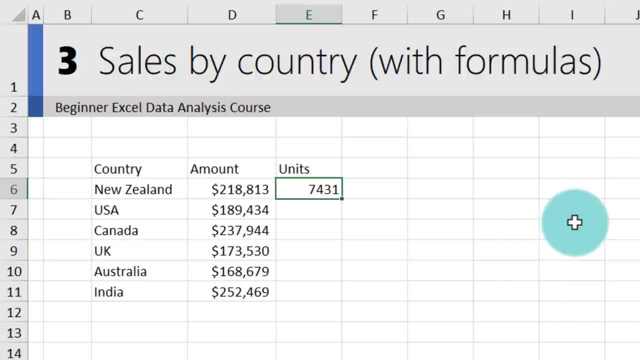 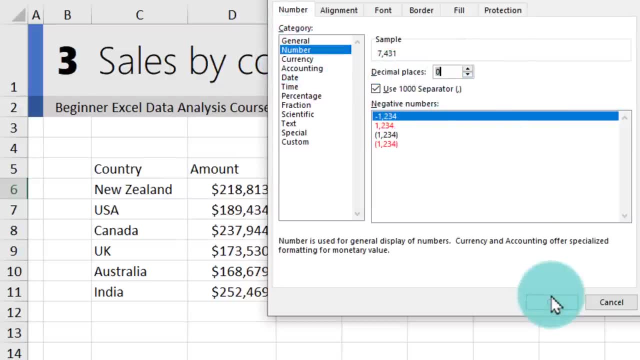 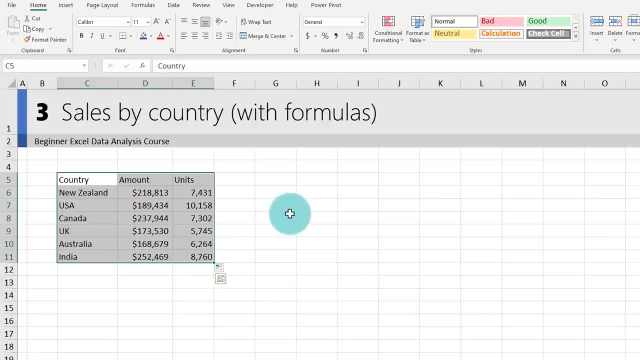 we want to just have a comma so I can select the cell press control one to open the format options from here: number, add a thousand separator zero decimals, click ok and then click down. so at this point, this particular analysis gives you the information that you want. while you may be happy, 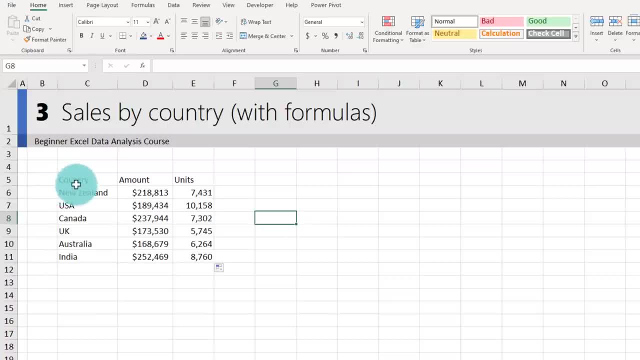 with this. if you are preparing this for somebody else, you may want to also figure out how to present this in a better way. so what I'll do is I'll show you how to make it presentable. first up, we'll select this. we'll make a copy of this so you can see the difference between original and. 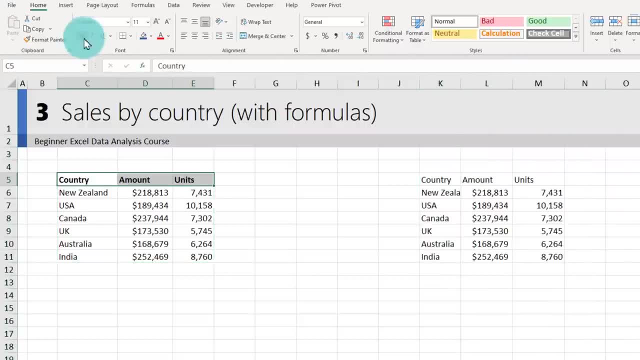 polished format. I'm going to select the headers, make them bold and add a little bit of background color on that. select these two columns right, align them, because that's the numbers and that's how these are aligned. then, most importantly, apply a sort order that is logical. so you could either: 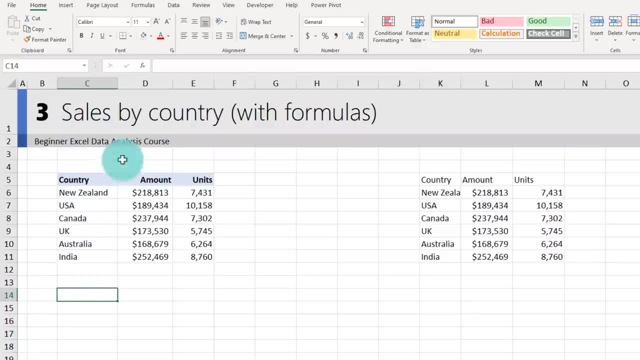 sort them in alphabetical order or because we are talking about sales by country. take the amount column and sort this so quickly. add filters largest to smallest and then disable the filters. so now you can see India is our best-selling country in this data, followed by Canada, and Australia is the lowest selling. 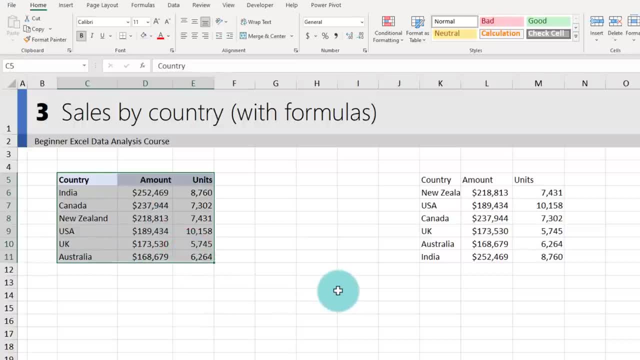 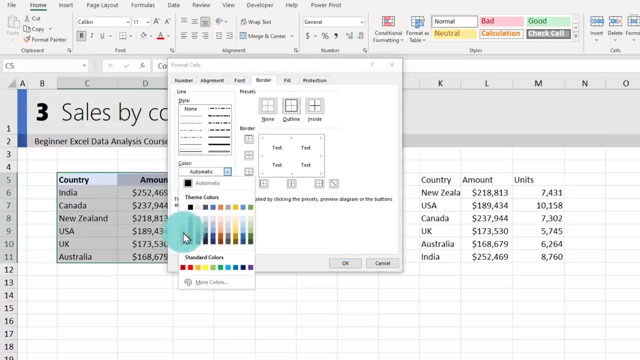 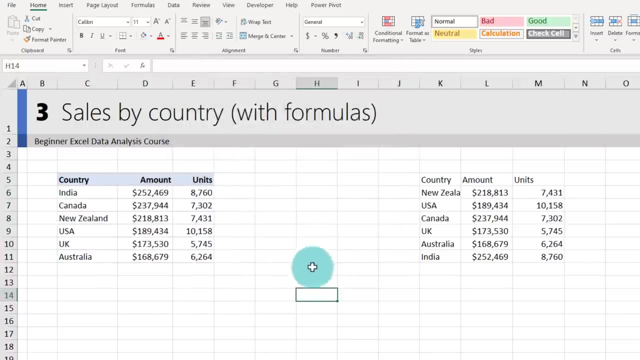 country within this data set. the next thing that you want to do is select all of this and add some simple borders around it. go to border and just set the color to a dull color and only add horizontal borders. now the border color kind of matches the grid line so we can't really see what is there. but if I go to view and disable, 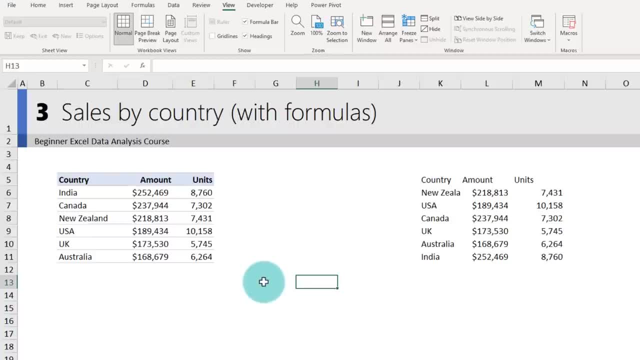 the grid lines, I'll get this nice little thing. the next thing that you may want to consider is adding some additional detail to this so that it looks visually interesting. again, you can do a lot. I'll show you one technique, which is, rather than having amount and units like this, I'll just 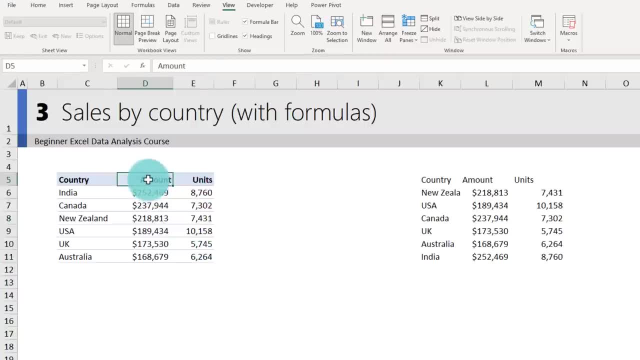 is, rather than having amount and units like this, i'll just take my amount units and then drag them sideways so that there is some space in the middle and in this cell i'll say equal to that value. so we'll get a copy of that value here. notice that we are not writing a formula, we just reuse the value. 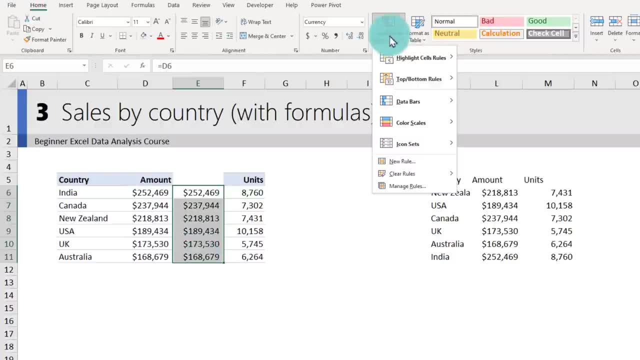 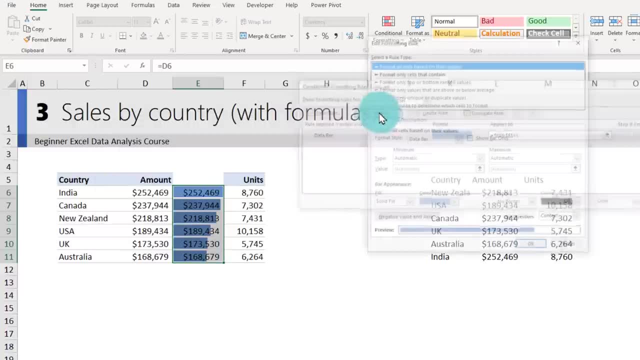 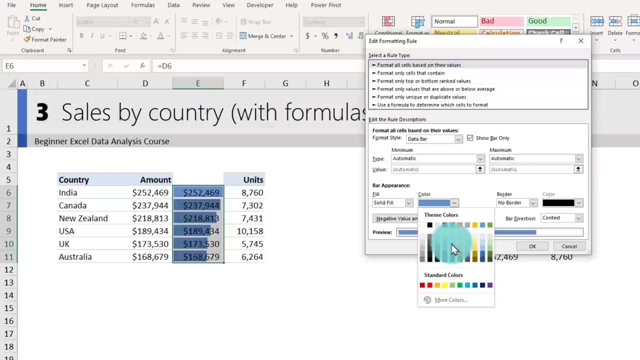 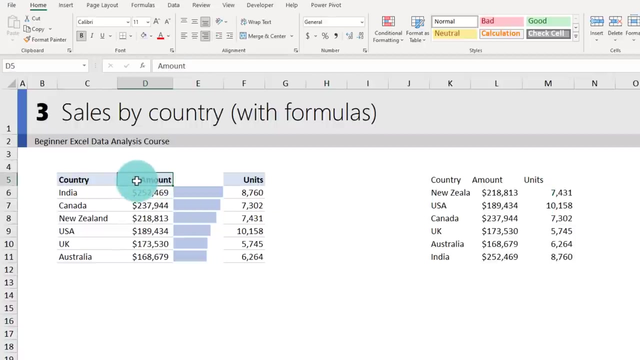 that is already there, select all of these, go to conditional formatting and apply a data bar. we'll go to manage rules, select the data bar and edit it and quickly say we only want the bar and the color need not be so strong. so we'll just go a shade dull like that and click ok, apply, if you think the color kind of matches too. 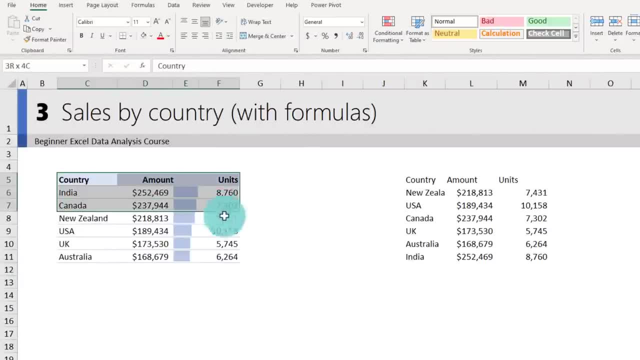 closely with the heading color there. you can readjust it and we'll get a nice little sales report that shows the amount as a bar as well, so that it gives you a visual indication of how high this number is. one last cosmetic touch that you could also do is: 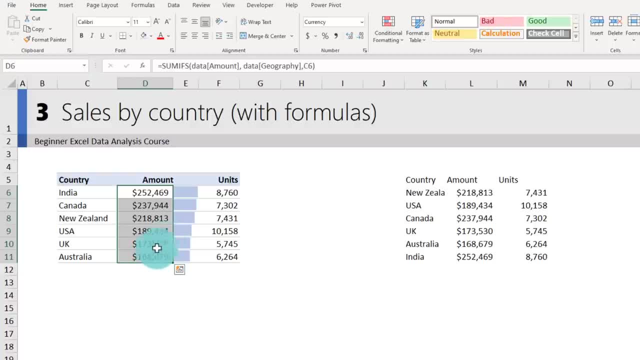 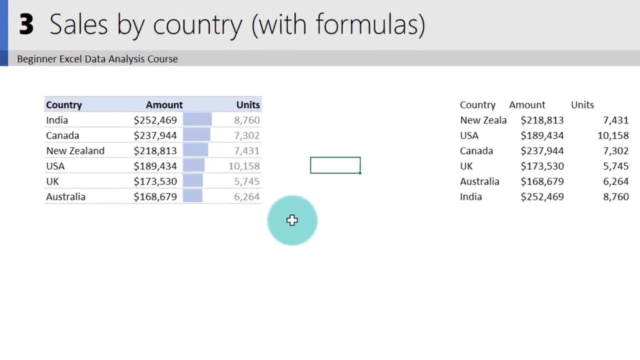 if the focus is on the dollars, then we leave this as it is, but select the units and just make them a different color so that they kind of blend into the background, so that not naturally we read these two and if needed we will read that additional information. so now, if you, 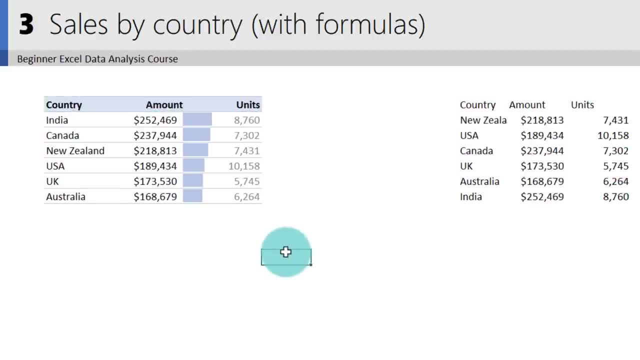 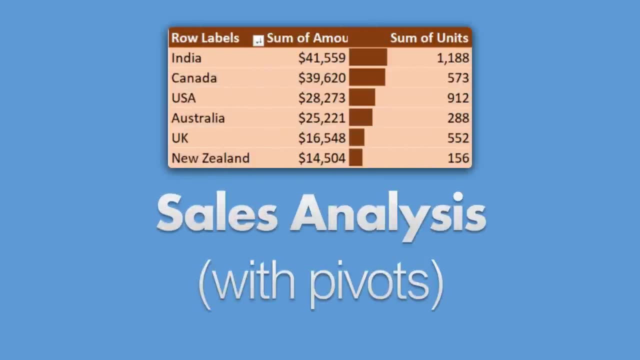 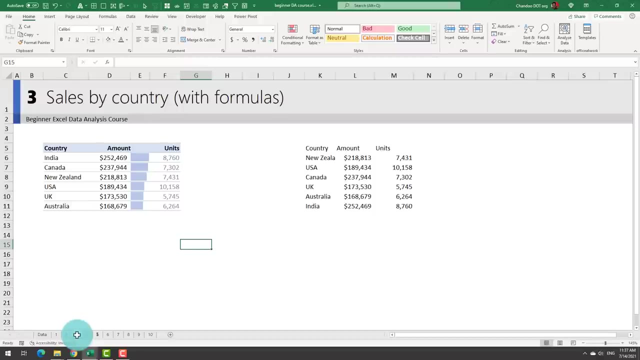 compare this versus that, you will immediately notice how pleasant and informative this left hand side is. in this example, i'm going to show you how to do sales by country using pivot tables. just to do a quick recap: in the previous example we did the same with formulas, so our goal is to replicate most of this by using pivot tables. we go to this page. 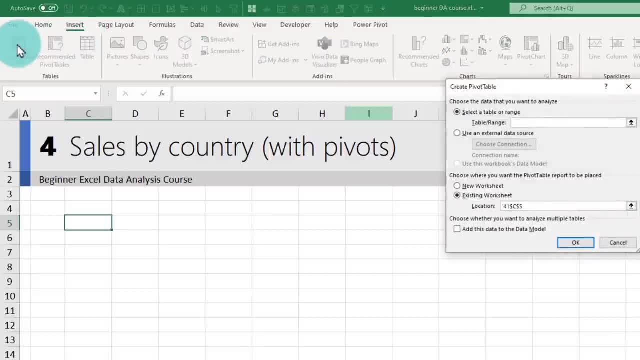 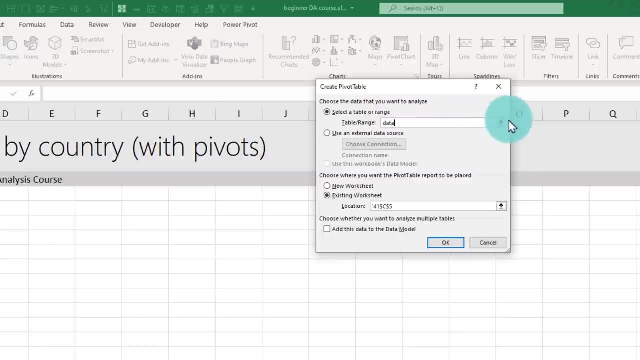 select a blank cell, go to insert pivot table and it will ask you: where is your data? our data is in the table data, so i'm just going to type data here. alternatively, you can go click on that and select the data and when you click ok, you'll get a. 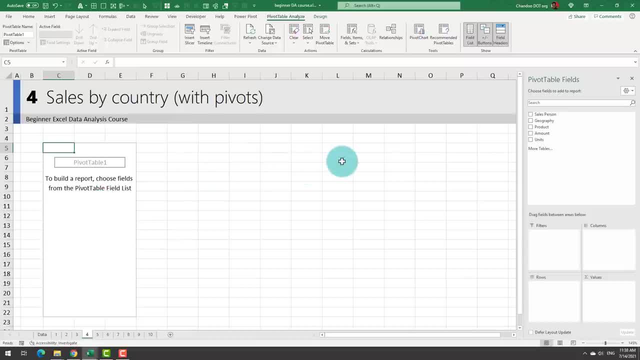 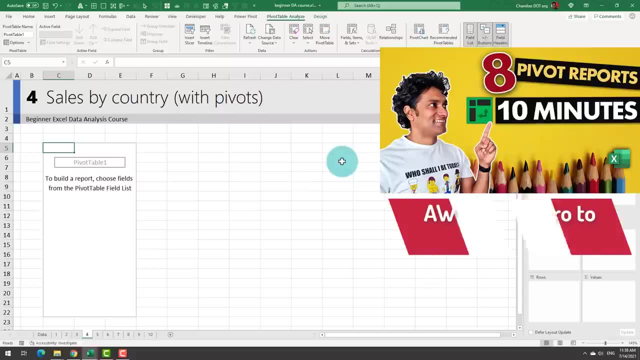 view of your data, and this can be used as a reference to your pivot table, and you can also make a canvas here to build your pivot table. i'm assuming that you are already familiar with pivot tables, but if not, you can watch my video on pivot tables that goes into greater detail on how to 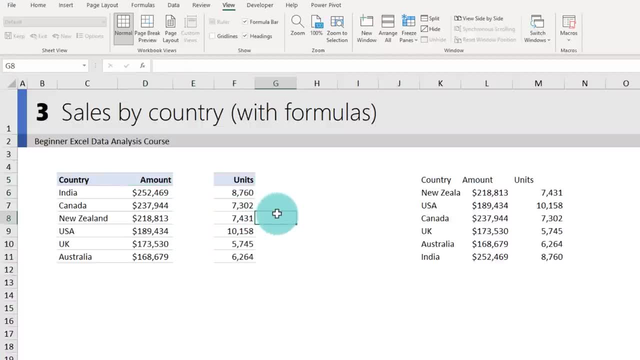 take my amount units and then drag them sideways so that there is some space in the middle and in this cell I'll say equal to that value. so we'll get a copy of that value here. notice that we are not writing a formula, we just reuse the value that is already there. select all of these. 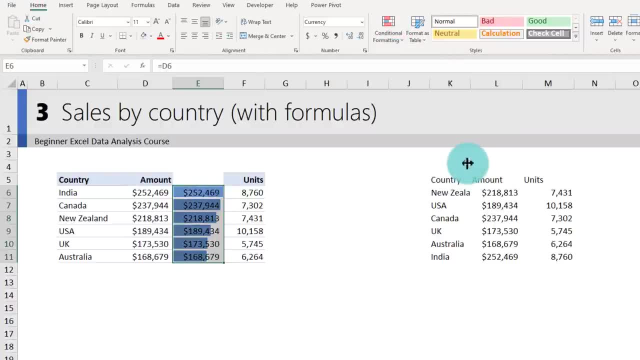 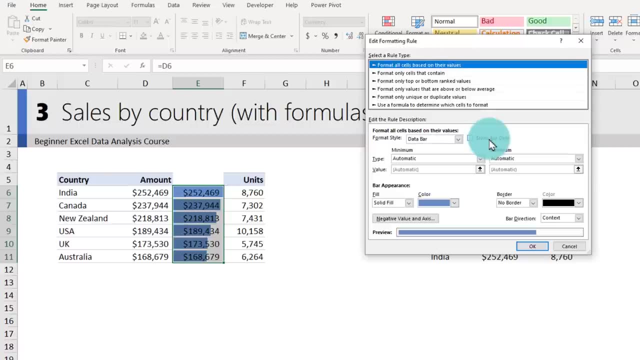 go to conditional formatting and apply a data bar. we'll go to manage rules, select the data bar and edit it and quickly say we only want the bar and the color need not be so strong. so we'll just go a shade dull like that, click ok, apply if you think the color kind of matches too closely with the heading color there. 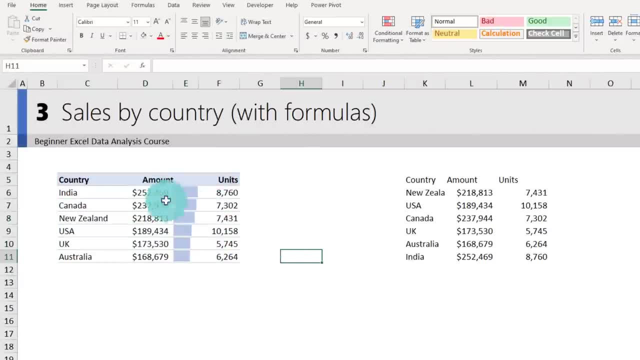 you can readjust it and we'll get a nice little sales report that shows the amount as a bar as well, so that it gives you a visual indication of how high this number is. one last cosmetic touch that you could also do is if the focus is on the dollars, then we leave. 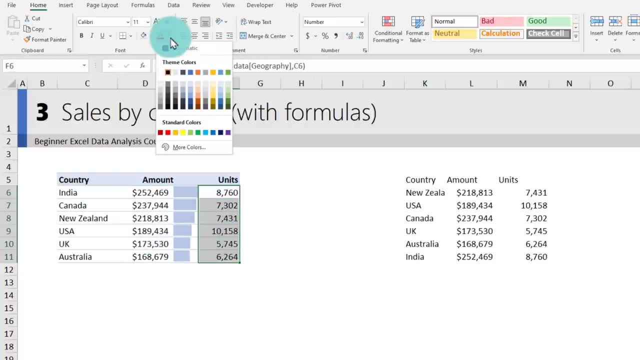 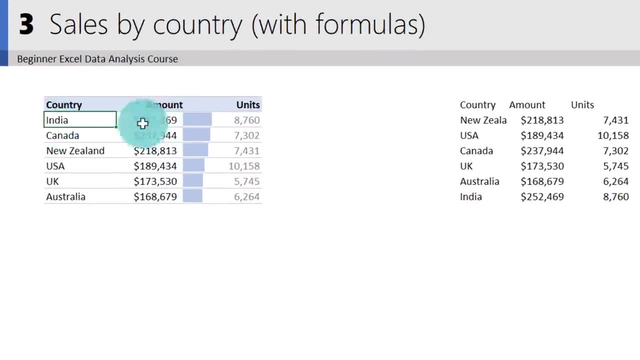 this as it is, but select the units and just make them a different color so that they kind of blend into the background, so that naturally we read these two and if needed, we will read that additional information. So now, if you compare this versus that, you will immediately notice how pleasant and informative 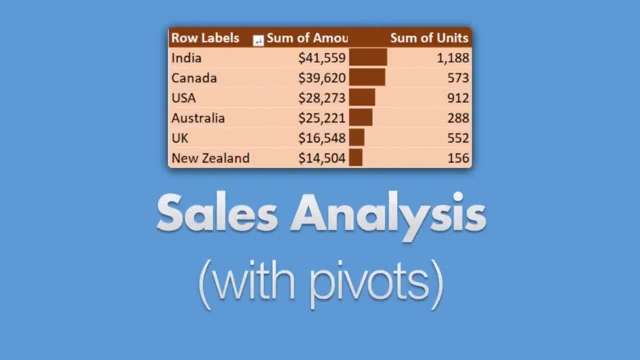 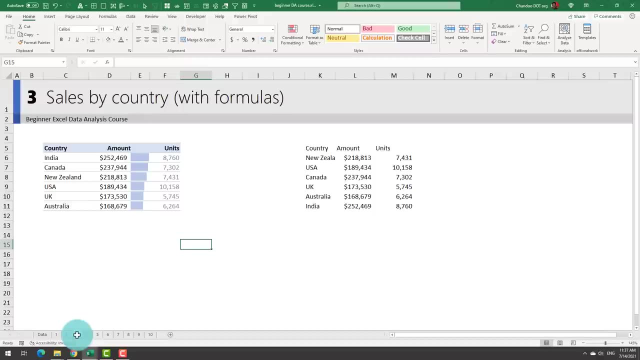 this left hand side is In this example. I'm going to show you how to do sales by country using pivot tables, Just to do a quick recap. in the previous example we did the same with formulas, So our goal is to replicate most of this by using pivot tables. 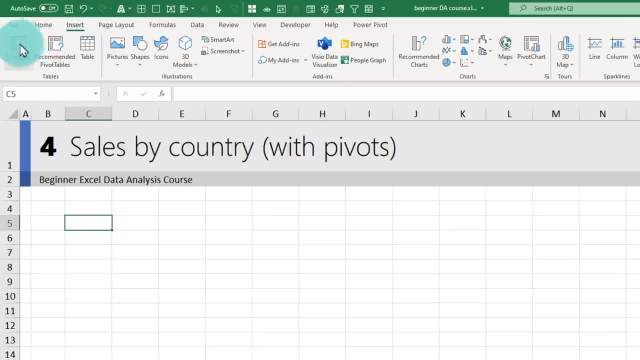 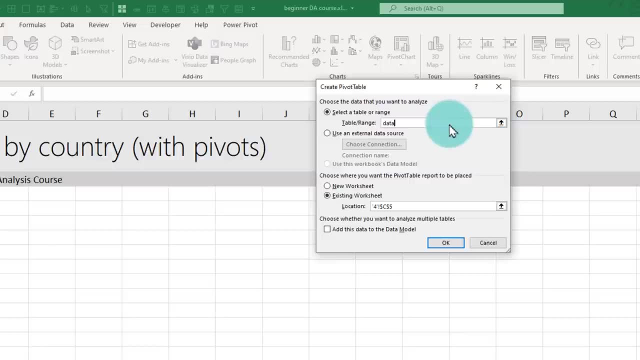 We go to this page, select a blank cell, go to insert pivot table and it will ask you: where is your data? Our data is in the table data, so I'm just going to type data here. Alternatively, you can go click on that and select the data. 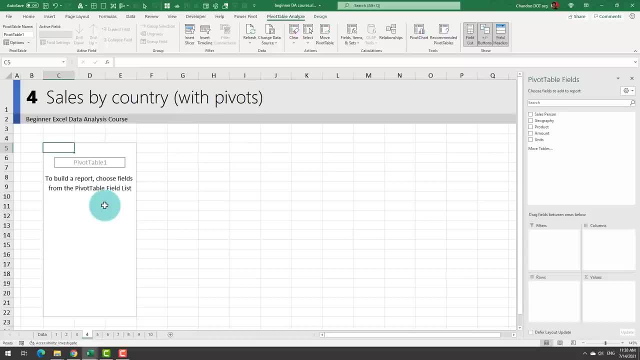 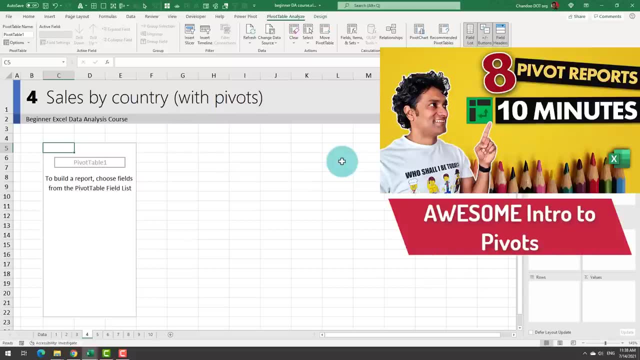 And when you click OK, you'll get a canvas here to build your pivot table. I'm assuming that you are already familiar with pivot tables, but if not, you can watch my video On pivot tables that goes into greater detail on how to construct the pivot tables. 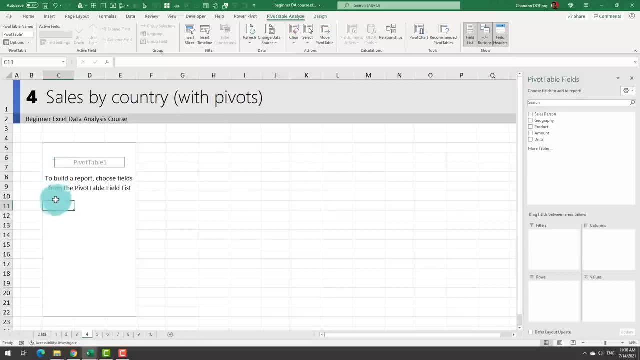 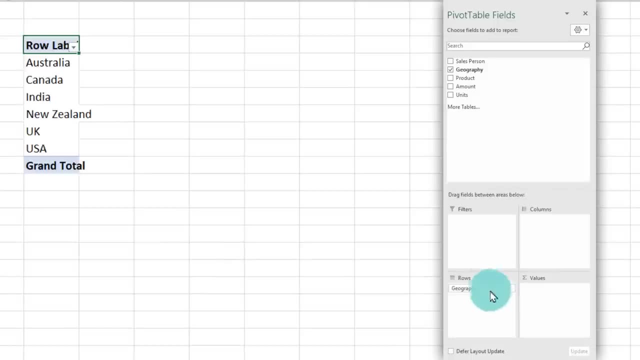 But here what we want to see is we just want to see one country per row and how much amount and how many units they made. So we say, take the geography, put it into the row area, and then take the amount, put it into values, take the units, put it into the values. 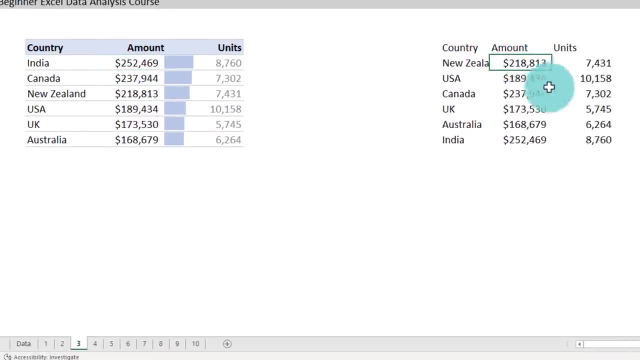 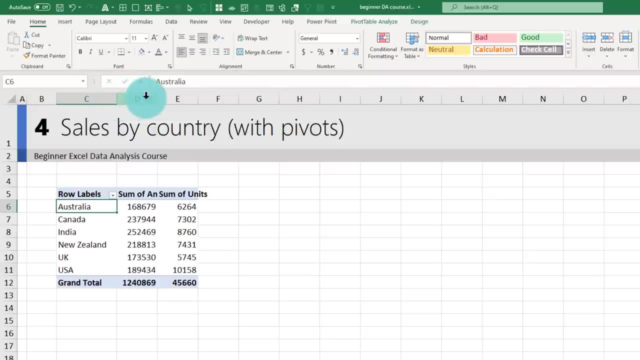 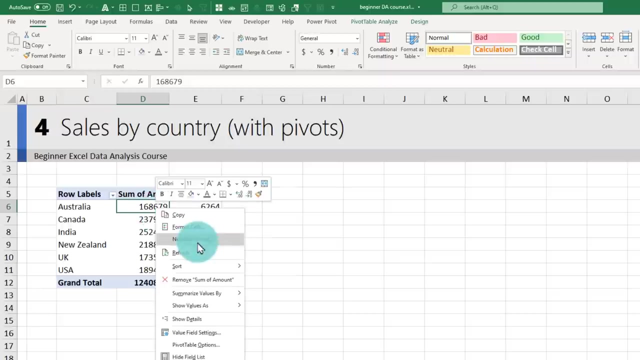 We already have our exact report here. I'm just going to quickly adjust some of these things, Which is make this column wider, select these two, make them wider, and then right click on one of these numbers, go to number format. apply currency formatting. 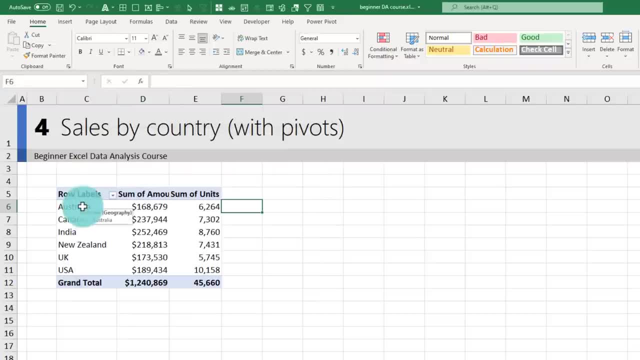 Notice that when you create a pivot table, by default the row labels are in alphabetical order, So they go from A to Z, But if we want to apply that on the amount, you can right click on this. go to sort largest to smallest. 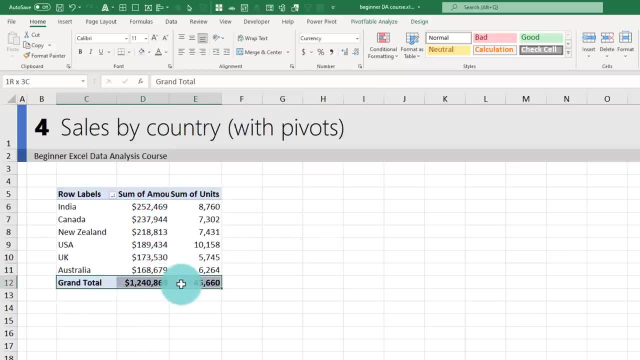 So that we will get again India on the top, Australia at the bottom. We also have this bonus of grand total here at the very bottom in the pivot table. You can adjust the style and color by going to the design ribbon when you have selected. 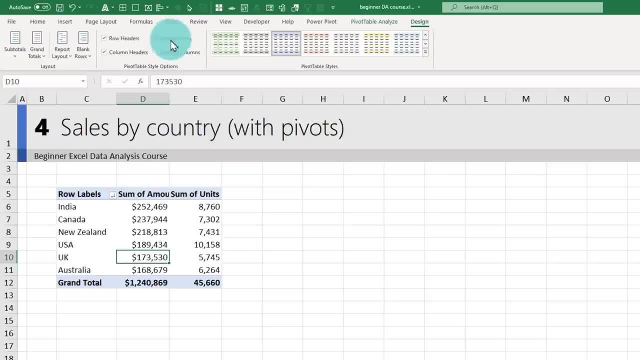 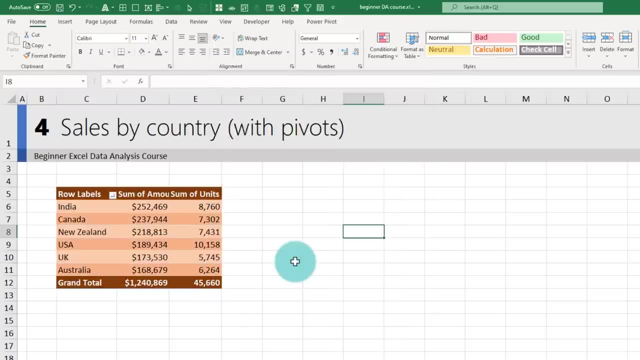 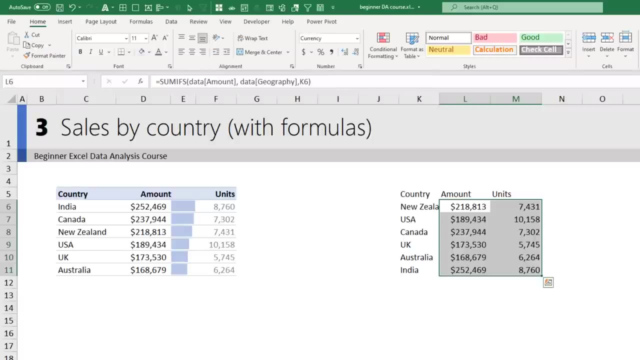 the pivot table And you can, for example, add banded rows. You can change the color scheme and make it like a really strong color, if you prefer. How do we add the conditional formatting data bars here? Because we did this By having a separate column. here I'll try to replicate the same. 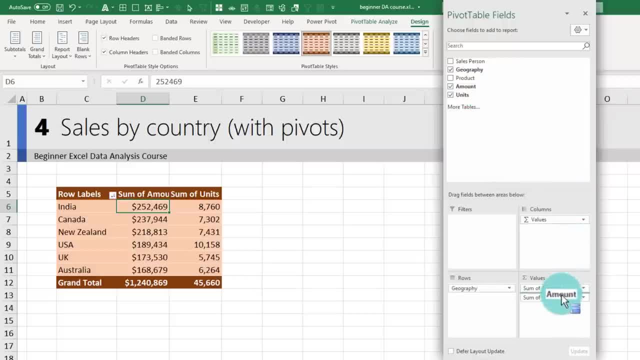 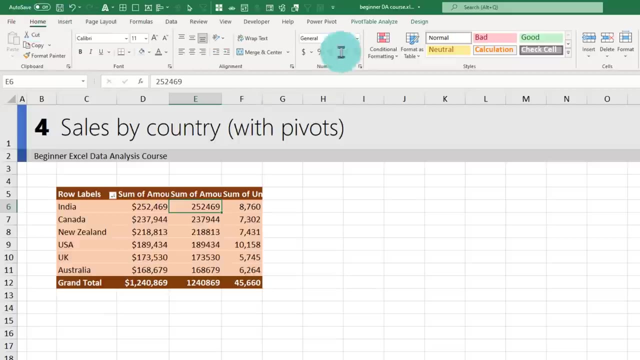 So first up we'll click on the amount, drag and drop it again, not at the bottom but in the middle between the original amount and the units, So we'll get a replica of the same calculation here And then I'll right click on: sorry, I'll select this cell. go to home conditional. 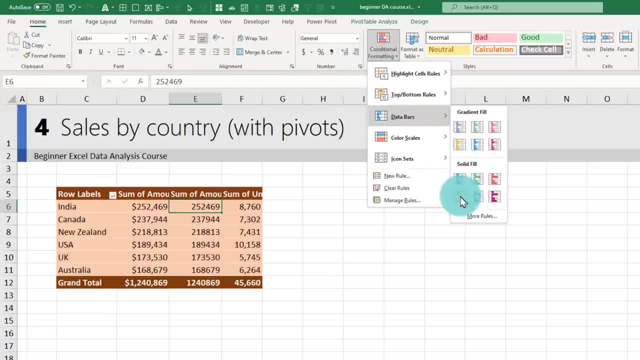 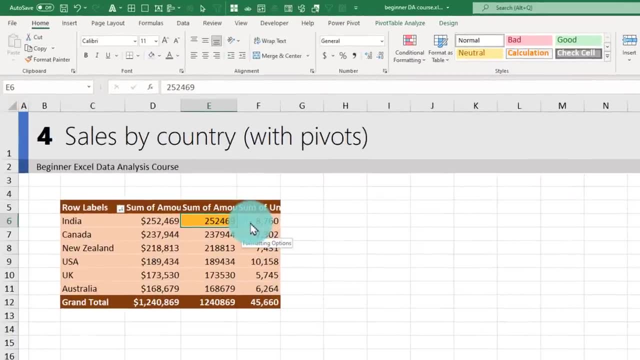 formatting data bar and add the data bar. Let's just go with this color. Then, once you do that, on a single cell you'll get this little pop up box: formatting options. Select the third one. It will add data bar all the way through. 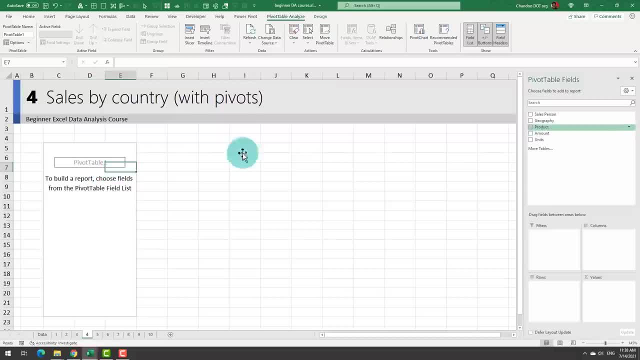 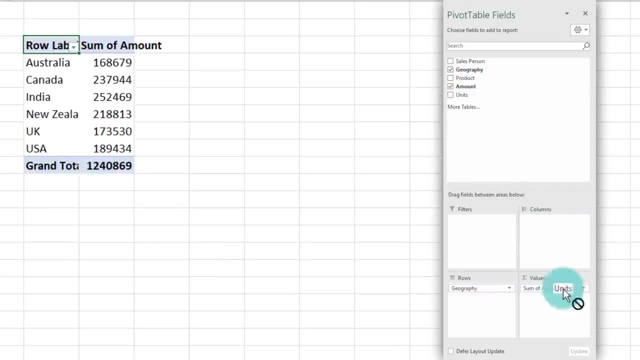 construct the pivot tables. but here what we want to see is we just want to see one country per row and how much amount and how many units they made. so we say, take the geography, put it into the row area, and then take the amount, put it into values, take the units, put it into the values. 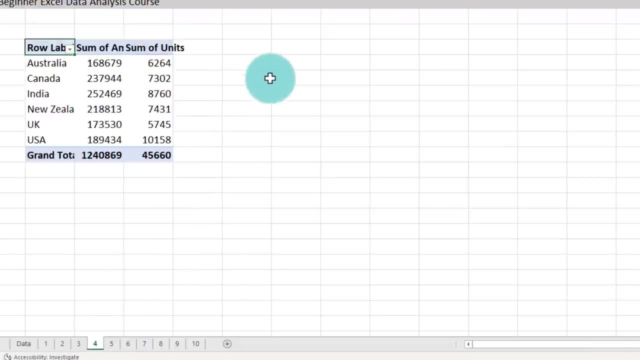 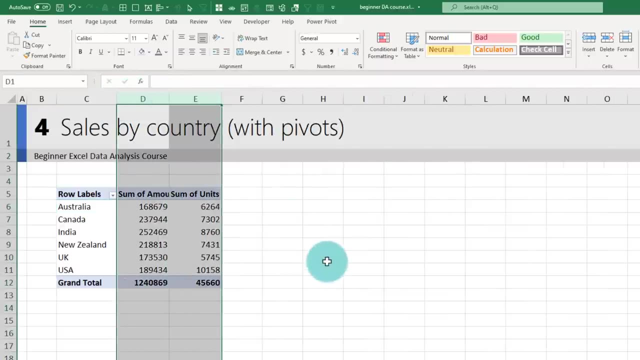 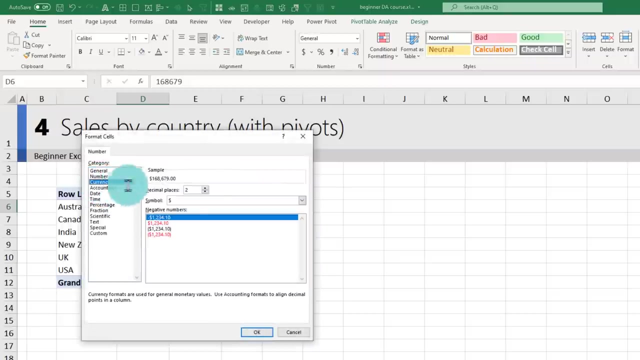 exact report here. i'm just going to quickly adjust some of these things, which is, make this column wider, select these two, make them wider, and then right click on one of these numbers, go to number format, apply currency formatting. notice that when you create a pivot table, by default the row labels: 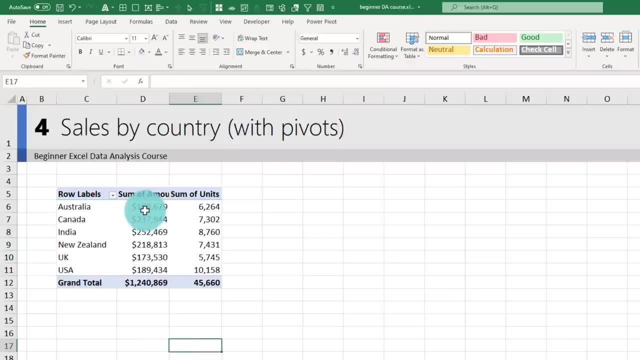 are in alphabetical order, so they go from a to z. but if you want to apply that on the amount, you can right click on this, go to sort largest to smallest so that we will get again india on the top, australia at the bottom. we also have this bonus of grand total here at the very bottom in the 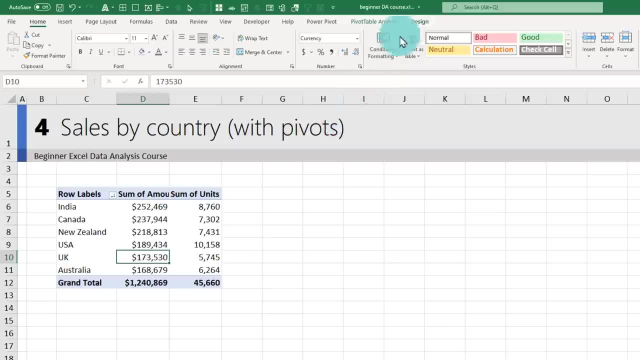 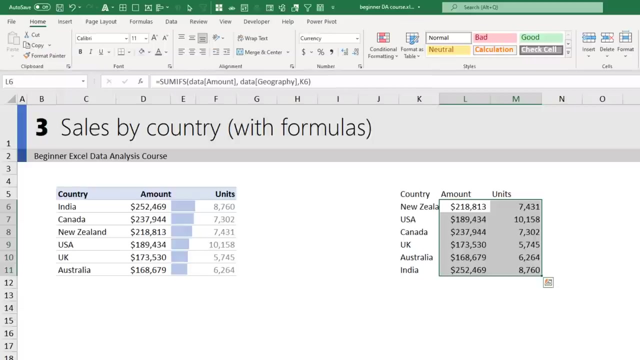 pivot table. you can adjust the style and color by going to the design ribbon when you have selected the pivot table and you can, for example, add banded rows. you can change the color scheme and make it like a really strong color if you prefer how you do. we add the conditional formatting data bars here, because we did this by having a separate. 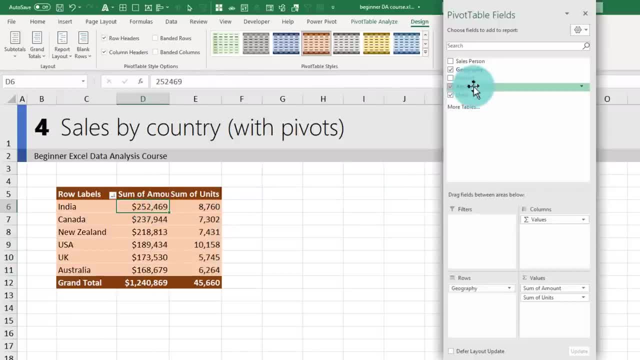 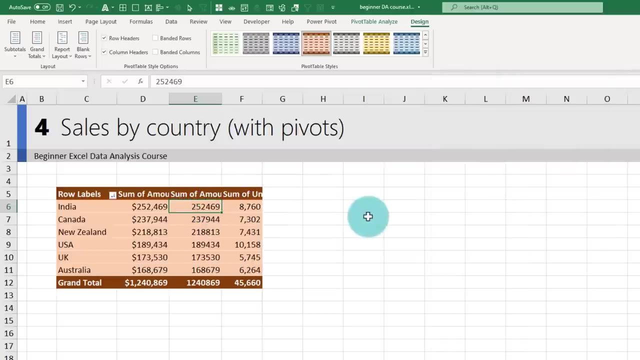 column. here i'll try to replicate the same. so first up we'll click on the amount, drag and drop it again not at the bottom but in the middle between the original amount and the units. so we'll get a replica of the same calculation here and then i'll right click on. sorry, i'll. 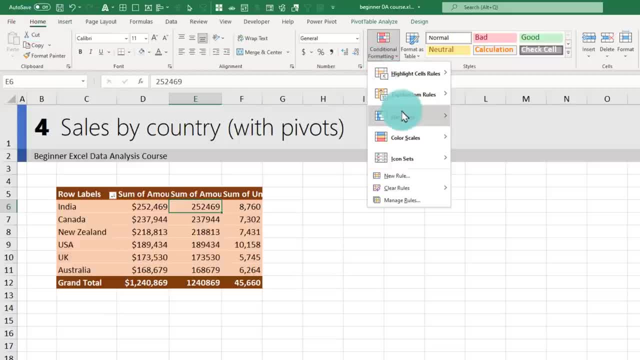 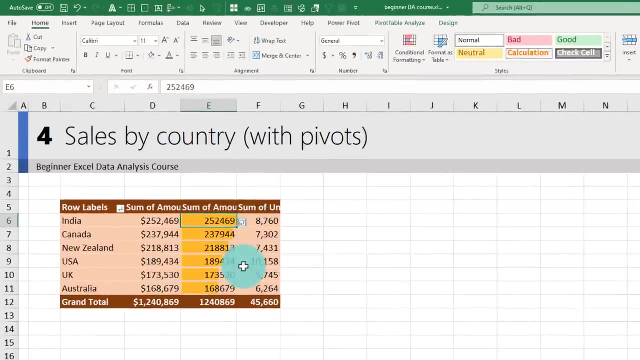 select this cell, go to home conditional formatting data bar and add the data bar. let's just go with this color. then, once you do that on a single cell, you'll get this little pop-up box: formatting options. select the third one. it will add data bar all the way. 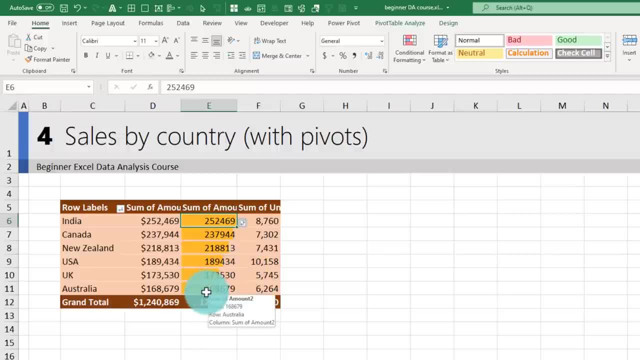 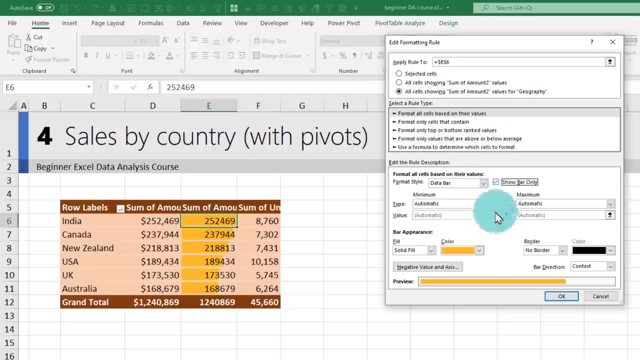 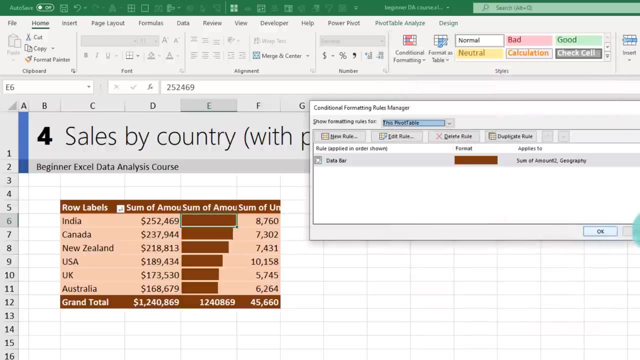 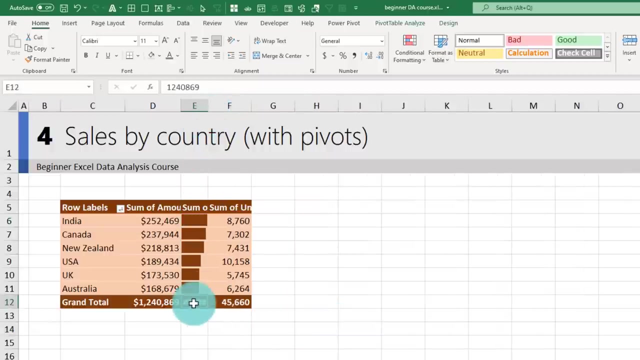 through. the bar is there, but it's not readable. also, the numbers are not required. so we'll go and manage the rule, select this rule, edit it. we'll say show bar. only i'm gonna pick that dark brick color and apply. we'll get that. let's just adjust this. we also don't need the grand total there. so what i'm? 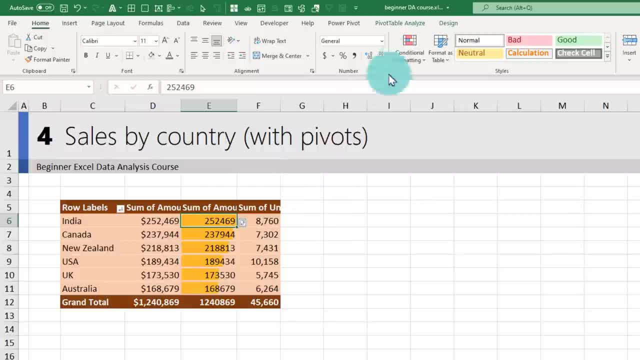 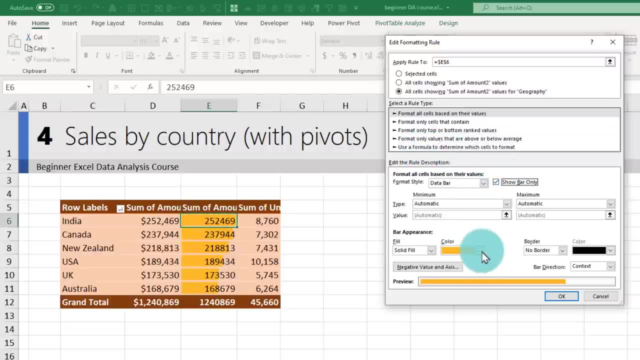 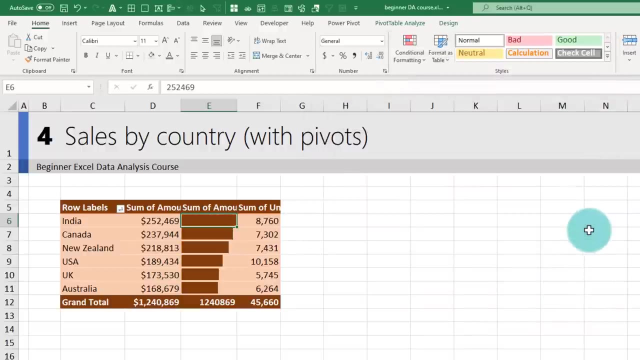 The bar is there, but it's not readable. Also, the numbers are not required. So we'll go and manage the rule. Select this rule, edit it. we'll say show bar. only I'm gonna pick that dark brick color and apply. 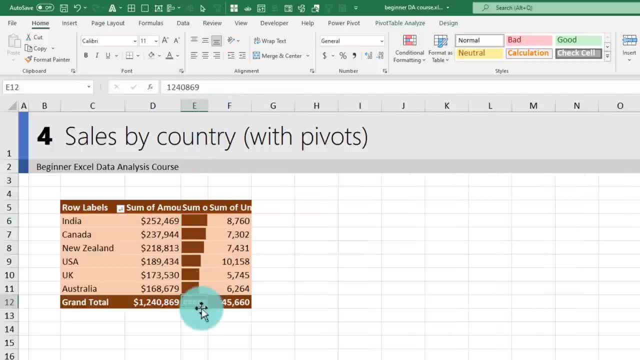 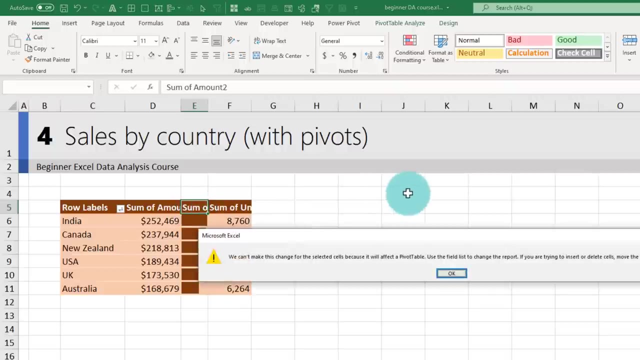 We'll get that. Let's just adjust This. we also don't need the grand total there, So what I'm going to do is I'll just go to the design, turn off my grand totals altogether. select this particular column header on my pivot table. just press the delete key. 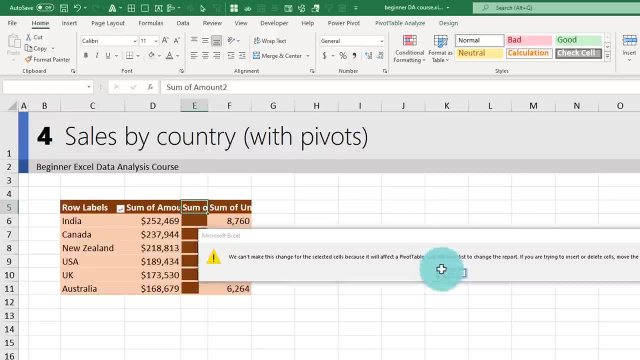 Now you can't really remove it. Excel doesn't like that. So instead of deleting, what we'll do is we'll press the space bar, So we kind of manually set that to space and we get this nice little data bar in the cell. 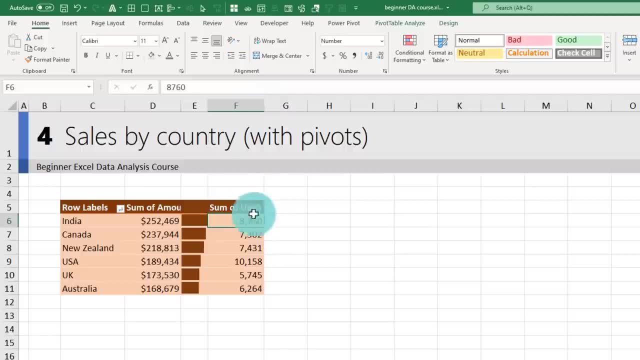 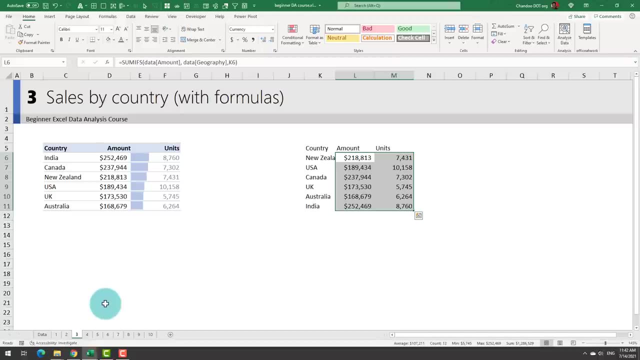 Amounts are there? Units are there? Now, here is a bonus advantage of using pivot tables instead of formulas. Within the formulas I'm looking at all the countries and all the data, But here, because this is a pivot table, I can kind of add some extra layer of filtering. 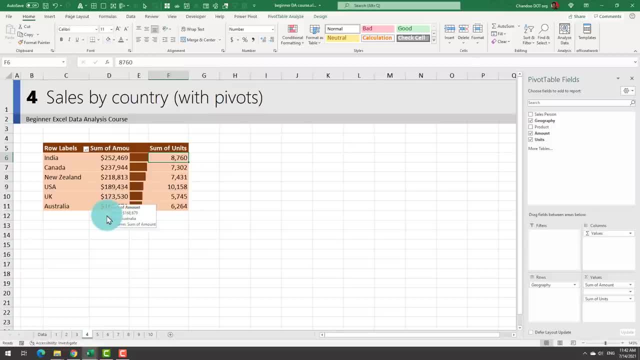 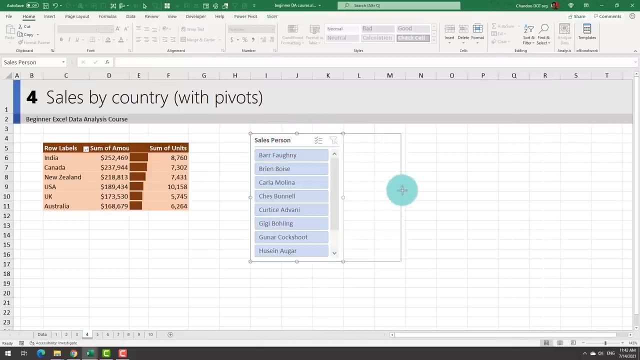 on top so that I can look at this report for an individual salesperson or individual product. So, for example, I'll right click on my salesperson field, add it as a slicer. We'll get all our salespersons here As a box. I'm just going to make this box nice and wide and go to the slicer options. 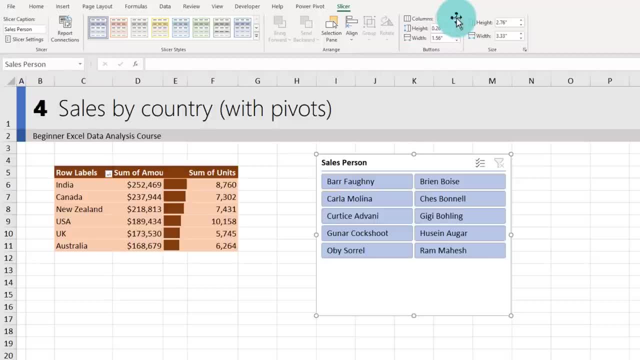 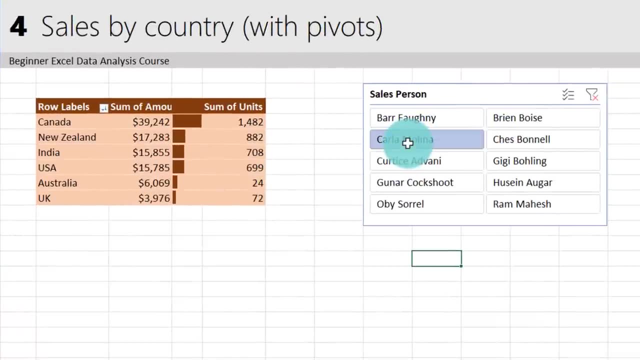 and set this to two columns So we see all the salespeople. Notice what happens if I go into one of our salespeople. So let's look at Carla. I can see how Carla has performed. The numbers graph is updated units and even the sort order is readjusted. 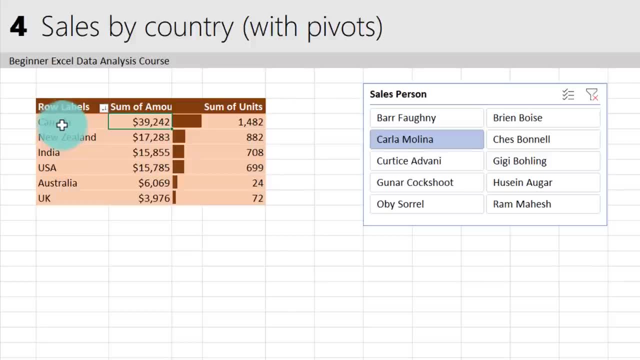 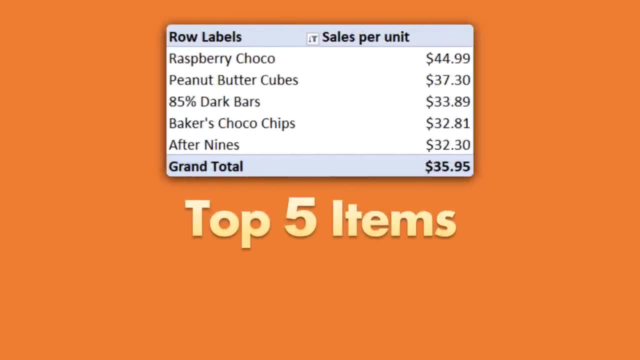 So because Canada is Carla's best country, it goes on the top and UK goes at the bottom. So you can do sales analysis by country using pivot tables. In this example we are going to look at top five products by dollar per unit. 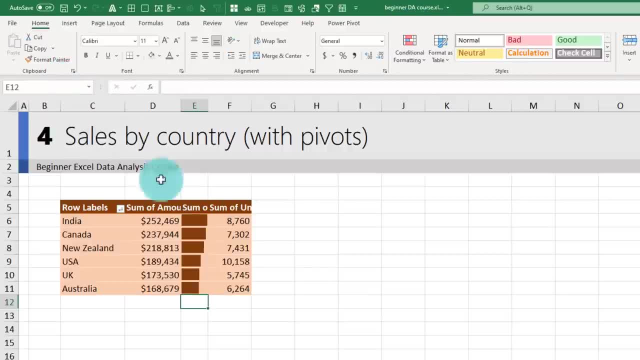 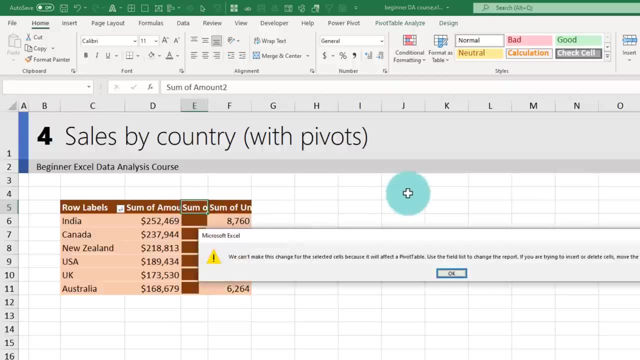 gonna do is i'll just go to the design, turn off my grand totals all together, select this particular column header on my pivot table, just press the delete key. now you can't really remove it, excel doesn't like that. so instead of deleting, what we'll do is we'll press a space bar, so we kind of 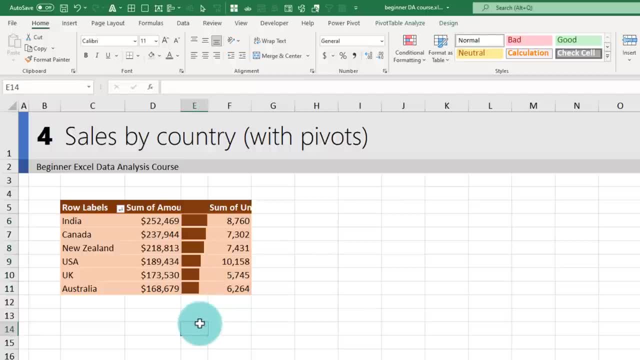 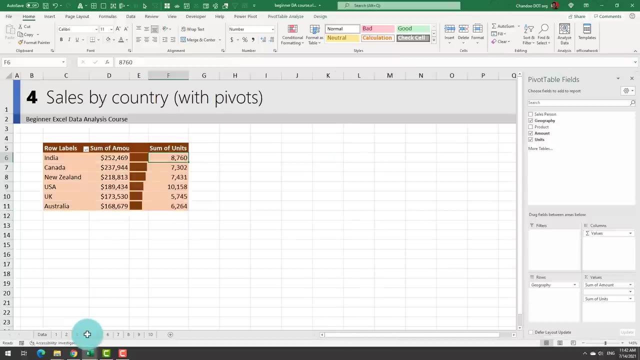 manually set that to space and we get this nice little data bar in the cell. amounts are there, units are there. now here is a bonus advantage of using pivot tables instead of formulas. within the formulas i'm looking at all the countries and all the data, but here, because this is a pivot table, i can kind of add some. 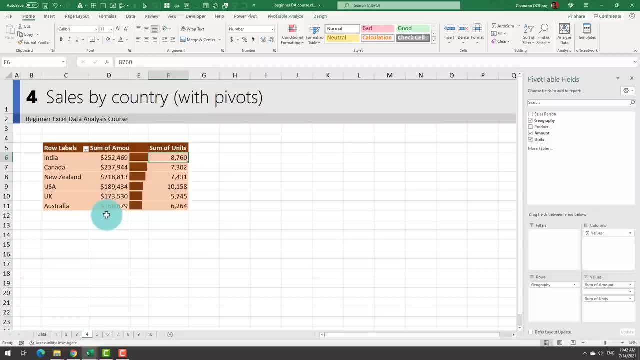 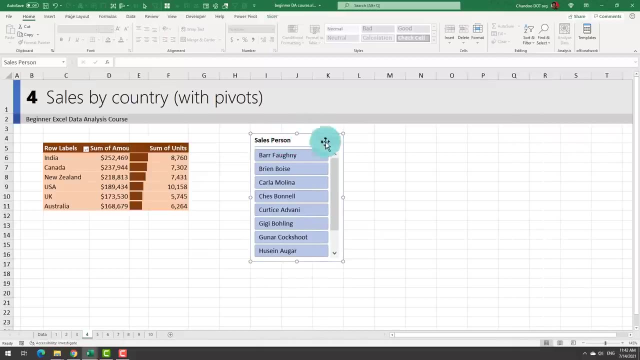 extra layer of filtering on top so that i can look at this report for an individual salesperson or individual product. so, for example, i'll right click on my salesperson field. add it as a slicer. we'll get all our salespersons here as a box. i'm just gonna make this box nice. 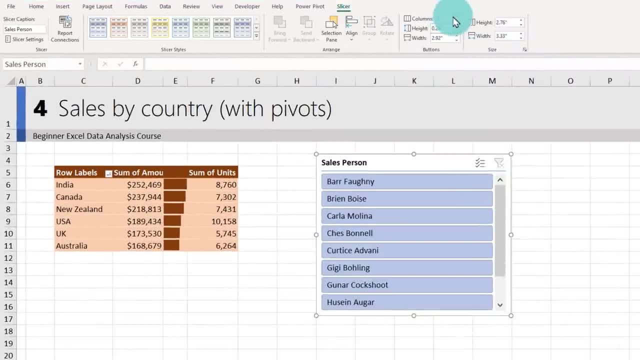 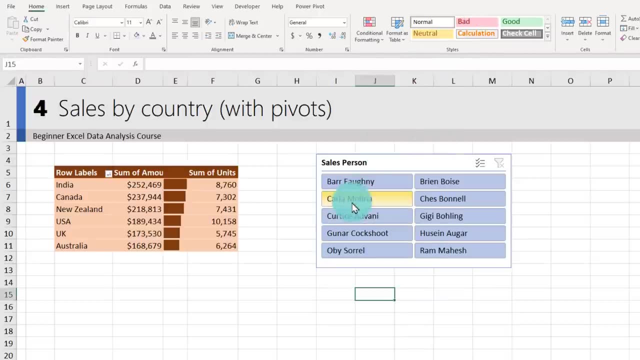 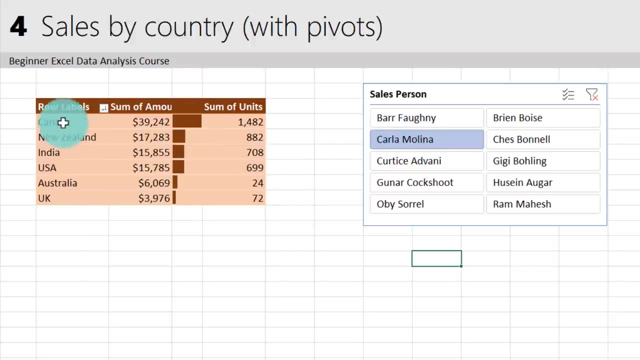 and wide and go to the slicer options and set this to two columns so we see all the salespeople notice what happens if i go into one of our salespeople. so let's look at carla. i can see how carla has performed. the numbers graph is updated units and even the sort order is. 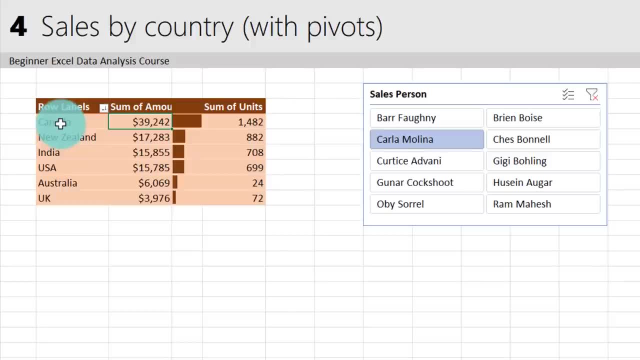 readjusted. so because canada is carla's salesperson field, so i'm going to go to the salesperson field best country, it goes on the top and uk goes at the bottom. so that's how you can do sales analysis by country using pivot tables. in this example we are going to look at top five products. 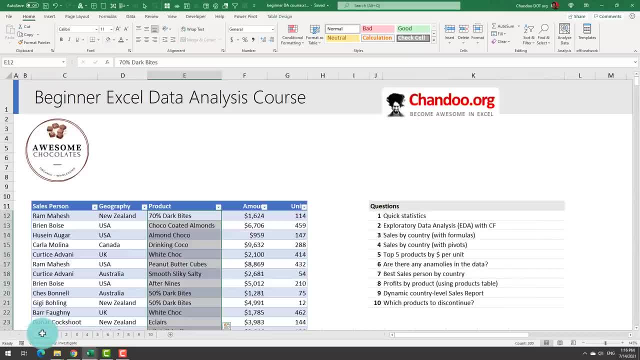 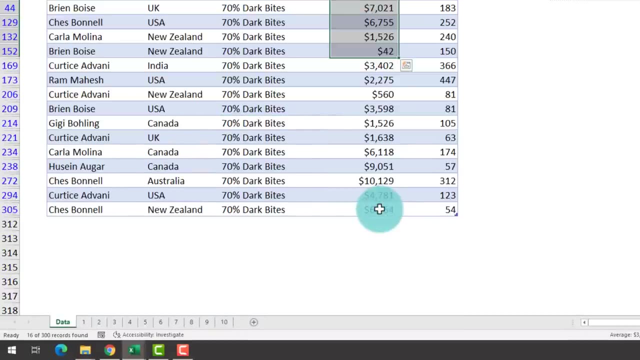 by dollar per unit. now if you go back to the data, you notice that we don't have dollar per unit. we have the amount and unit. so the dollar per unit would be for a product like 70 percent dark bytes. total amounts added up divided by two. 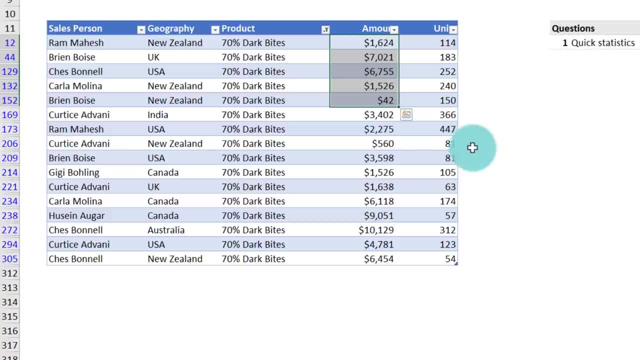 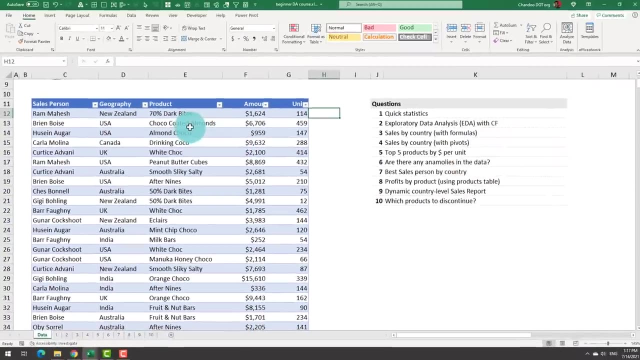 total units, and that's what the dollar per amount would be. so this kind of analysis requires introducing a third item. but we can't really add a column here, because that will only tell you per line item. what we want is at an aggregate level, so i'll show you how to use pivot tables to do such. 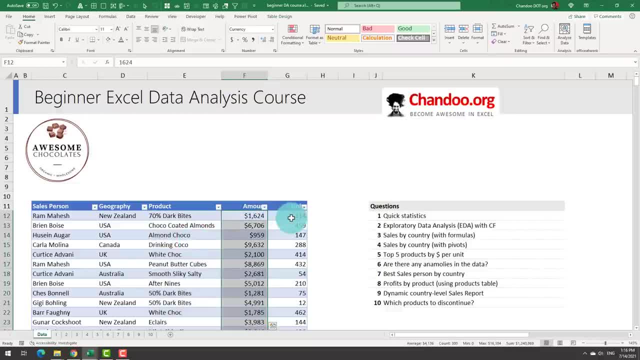 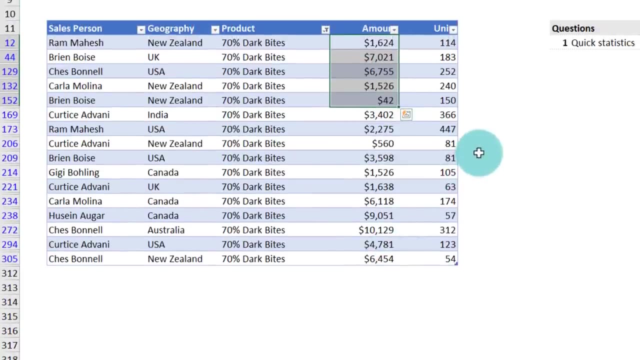 Now, if you go back to the data, you notice that we don't have dollar per unit, We have the amount and unit. So the dollar per unit would be for a product like 70% dark bites, total amount added up divided by total units, and that's what the dollar per amount would be. 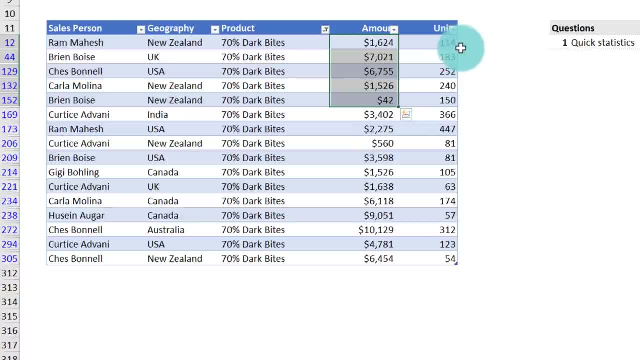 So the analysis requires introducing a third item. but we can't really add a column here, because that will only tell you per line item. What we want is at an aggregate level, So I'll show you how to use pivot tables to do such analysis. 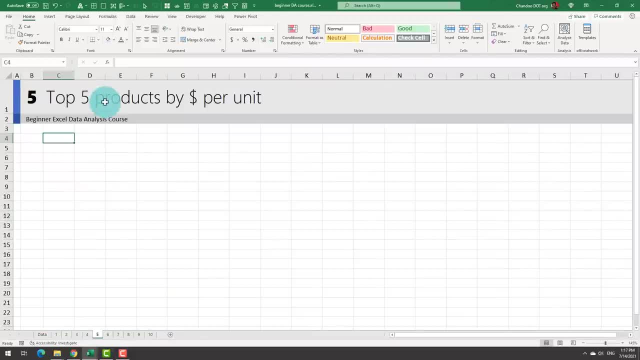 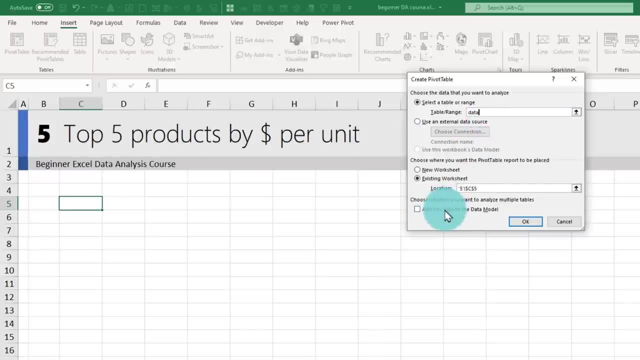 While we can use formulas to answer a question like this, uh, pivot tables provide a more logical and simpler way to do this. So we go to a blank cell here, insert a pivot table. We want the pivot from our data. But here is the critical part. 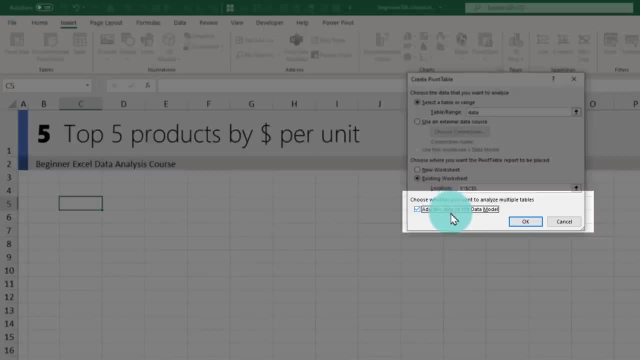 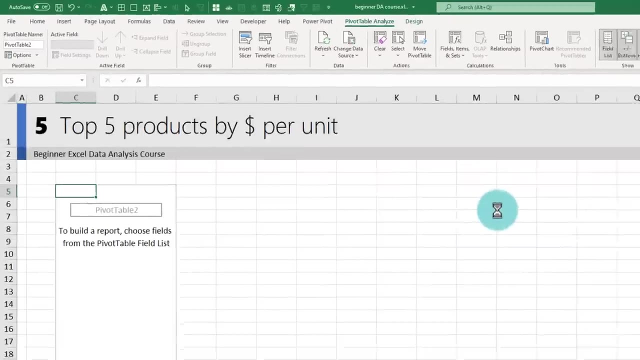 You need to add the data to data model. So enable this option. Only then we will be able to do such extra calculations, And then we click okay. The pivot table that you create is essentially similar to the pivots that we created in the. 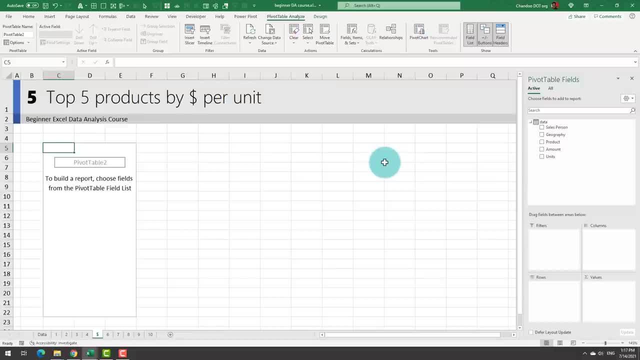 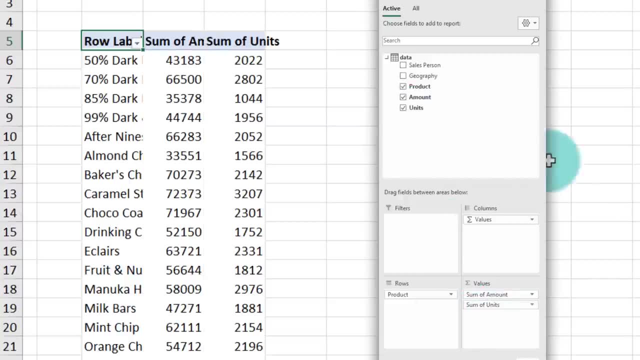 earlier examples. But here there's a bit more convenience. So now I'll take my product put here, let's add amount and units, So we get total amount And total units. So for each of these products that's the total amount and that's the how many units. 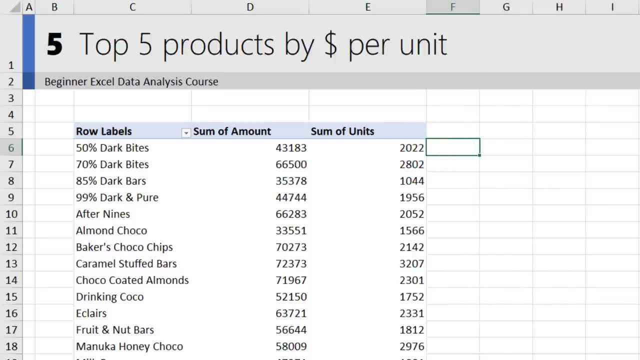 there is. Now we need to calculate a dollar per unit. We could kind of go outside and write a formula to do a D six divided by E six. but that's not what we want. We want to calculate that as part of the pivot and then look at top five products. 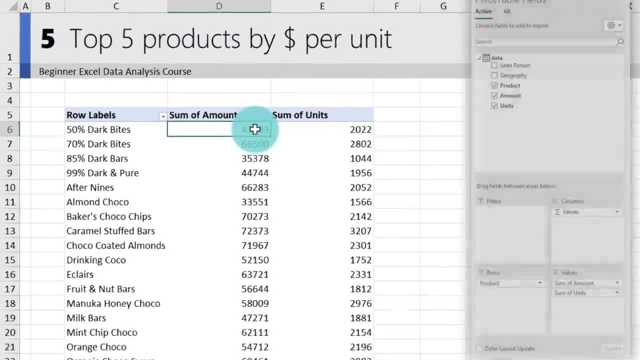 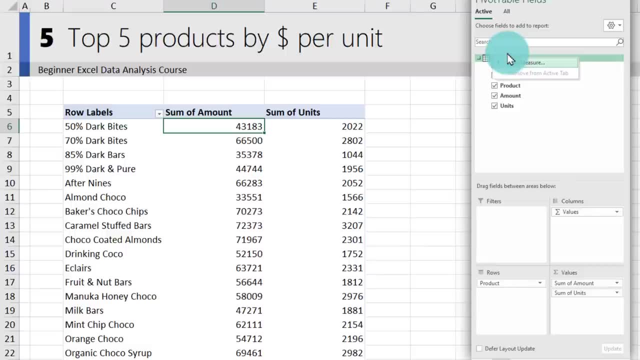 So here, now that the pivot is part of my data model, I can right click on the table in the pivot table field List and use add measure option. This is how you incorporate power pivot, which is a special engine that can be used to add. 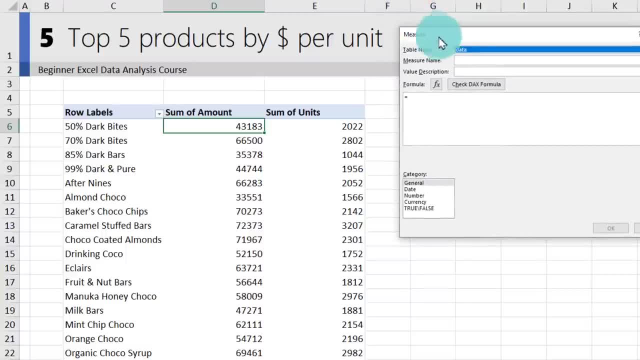 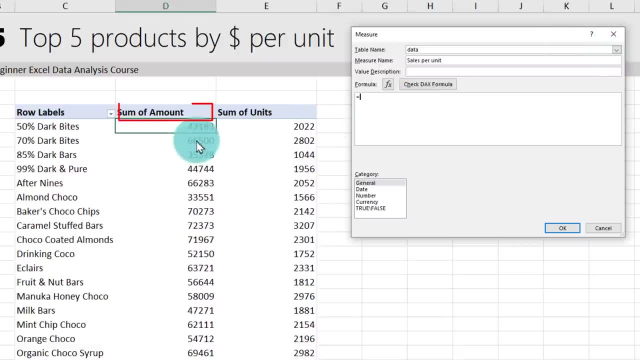 such custom calculations. So we will add a measure. This measure we will call it as sales per unit And this is nothing but this number divided by that number. This number is called sum of amount. So we open the square bracket and say sum of amount. 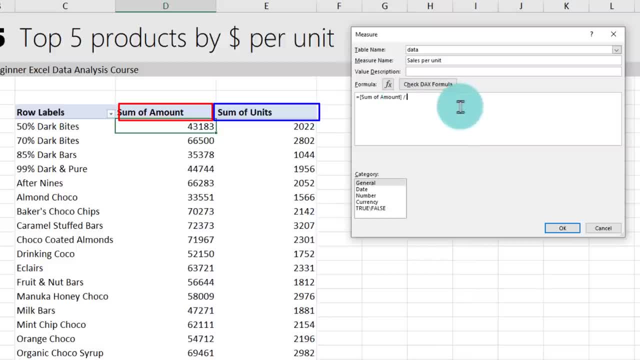 You can already see that it is there. Divide that with sum of units. So we take the first number, divide it with second number to create a third composite number called sales per unit. Let's just quickly make it currency: two decimal points Click okay. 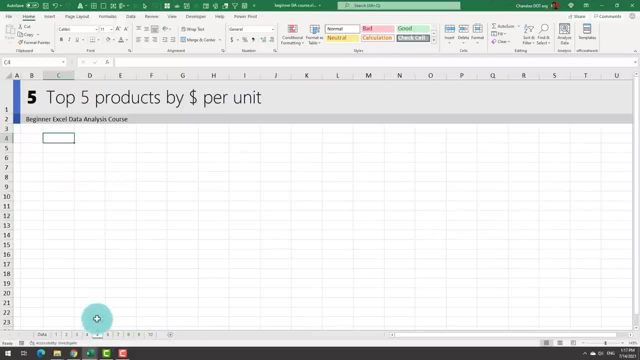 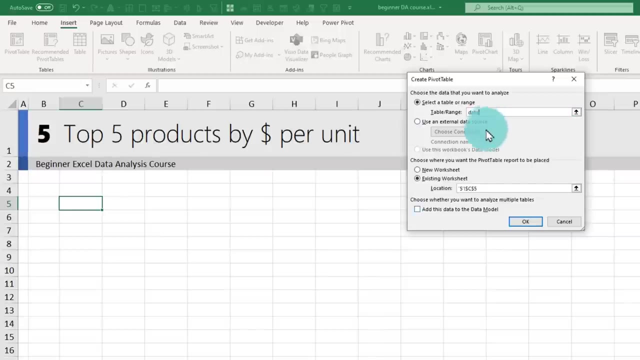 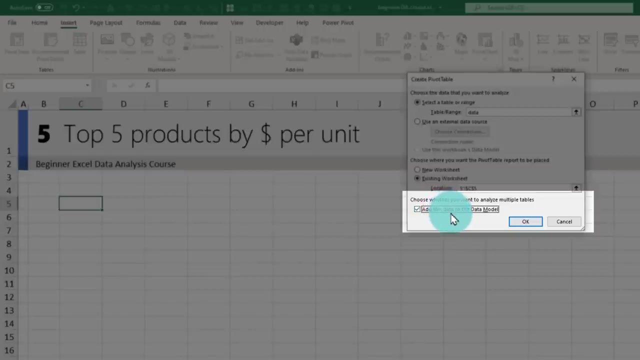 analysis. while we can use formulas to answer a question like this, pivot tables provide a more logical and simpler way to do this. so we go to a blank cell here, insert a pivot table. we want the pivot from our data. but here is the critical part: you need to add the data to data model. so enable this option. only then we will be able to do such extra. 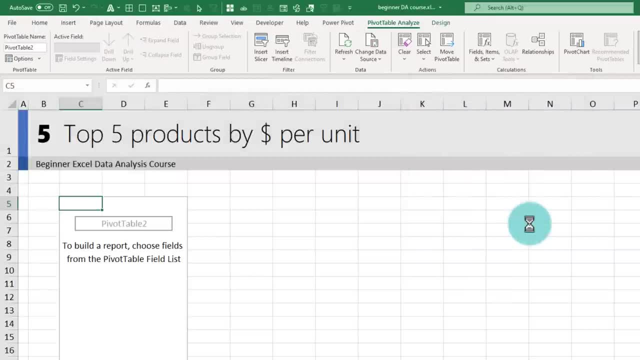 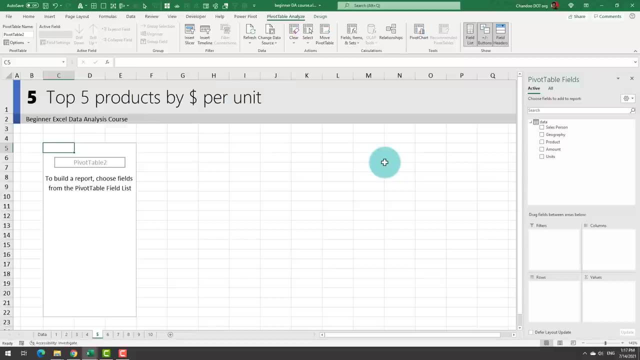 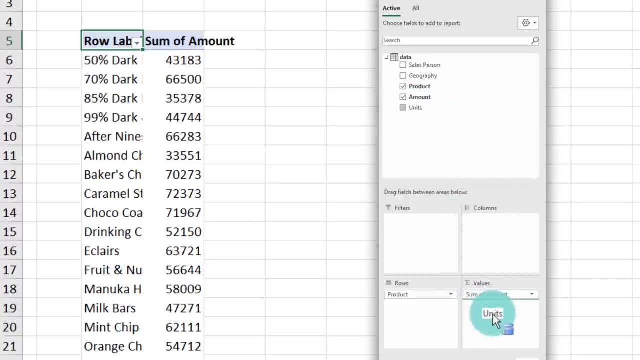 calculations and then we click ok. the pivot table that you create is essentially similar to the pivots that we created in the earlier examples, but here there's a bit more convenience. so now i'll take my product, put here, let's add amount and units, so we get total amount and total units. so for each of these products, that's. 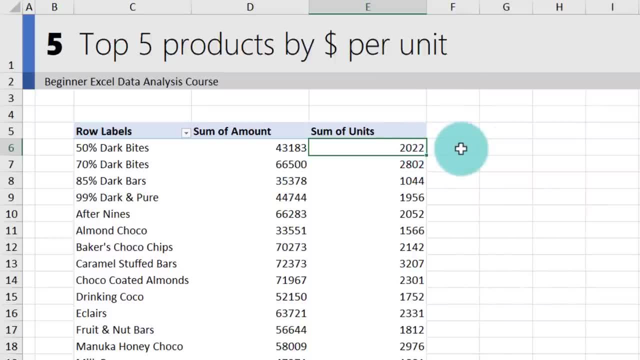 the total amount and that's the how many units there is. now we need to calculate a dollar per unit. we could kind of go outside and write a formula to do d6 divided by e6, but that's not what we want. we want to calculate that as part of the pivot and then look at top five products. 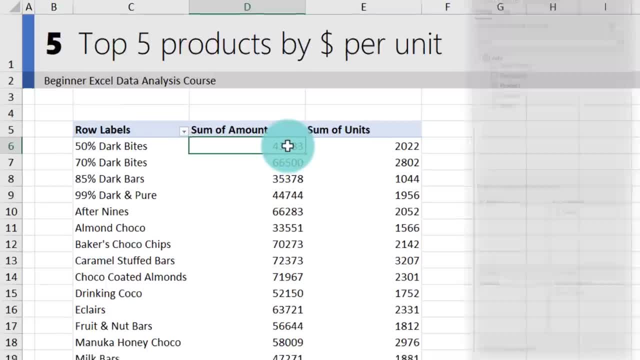 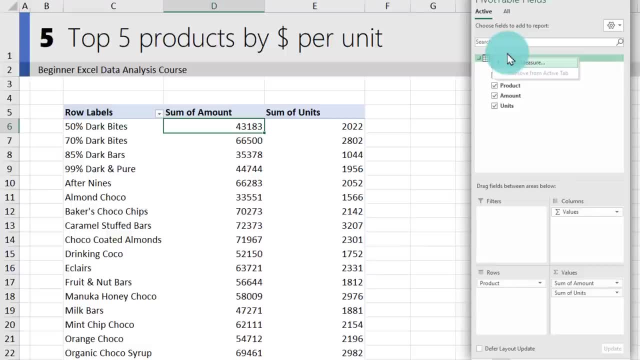 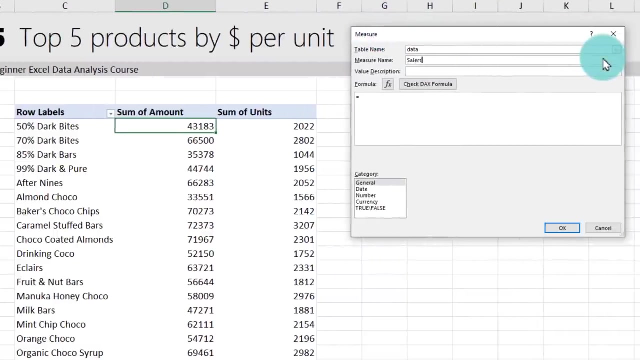 so here, now that the pivot is part of my data model, i can right click on the table in the pivot table field list and use add measure option. this is how you incorporate power pivot, which is a special engine that can be used to add such custom calculations. so we will add a measure. this measure we will call it as sales per unit and this 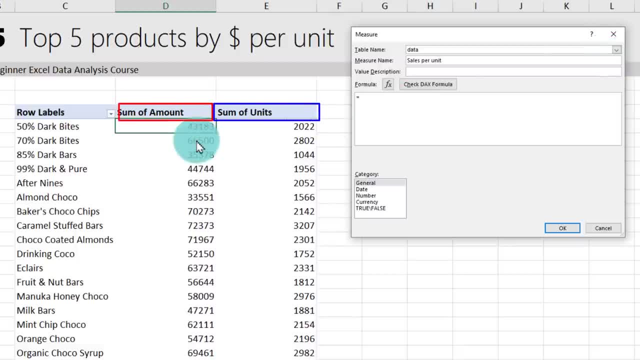 is nothing but this number divided by that number. this number is called sum of amount. so we open the square bracket and say sum of amount. you can already see that it is there- divide that with sum of units. so we take the first number, divide it with second number to create a third composite number called sales. 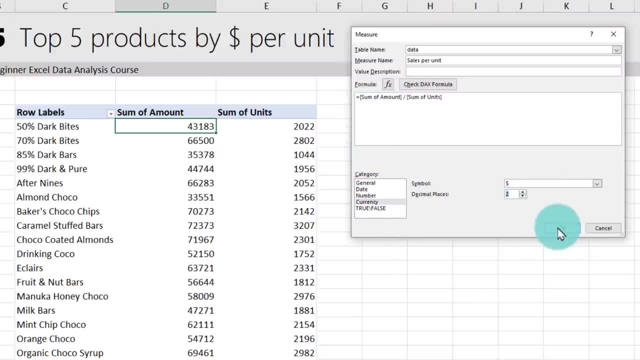 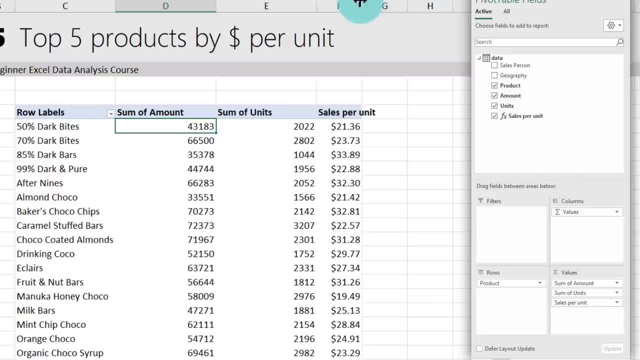 per unit. let's just quickly make it currency: two decimal points, click ok and we get sales per unit as a measure added. i can put it into the pivot table and then i'll see how much is the sales per unit for each of our products. now at this point, because we don't keep 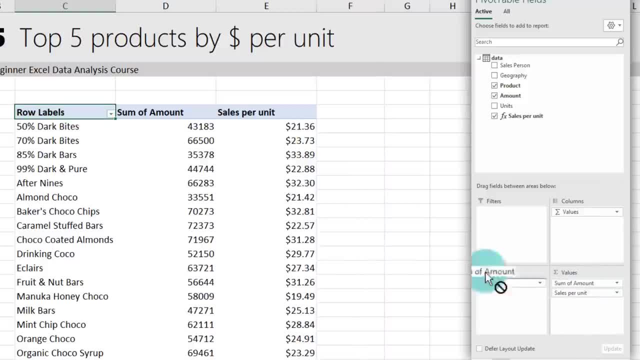 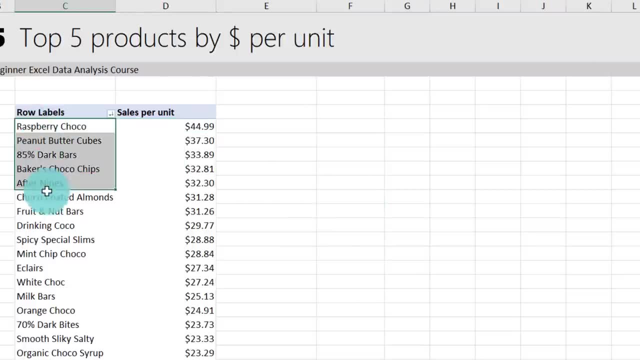 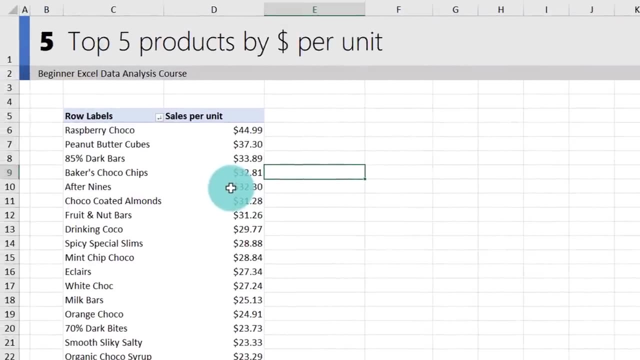 much about any of these other things. i'm going to drop them from my pivot, so we are only looking at this now. right click sort largest to smallest so we can see which products have the highest dollar per unit. remember, we only want to see the top five. we don't need to see everything. 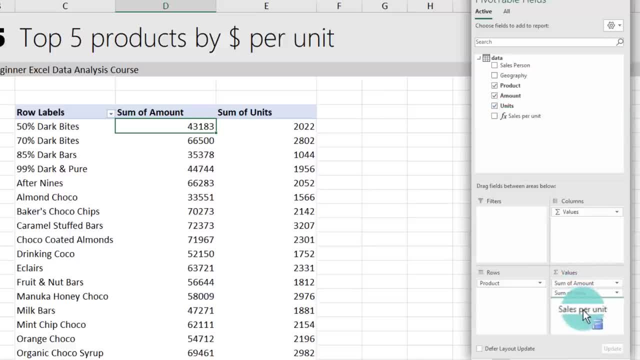 And we get sales per unit as a measure added, I can put it into the pivot table and then I'll see how much is the sales per unit for each of our products. Now, at this point, because we don't care much about any of these other things, I'm going. 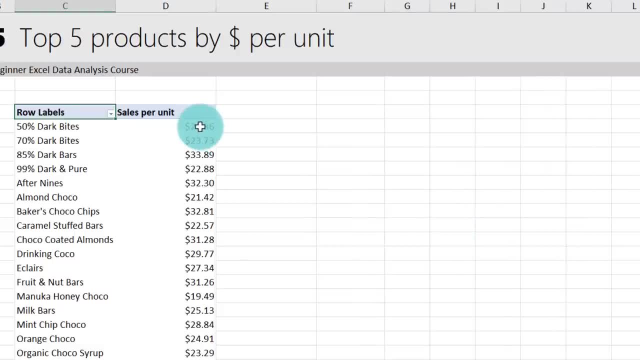 to drop them from my pivot. So we are only looking at this Now. right click sort largest to smallest So we can see which products have the highest dollar per unit. Remember, we only want to see the top five, We don't need to see everything. 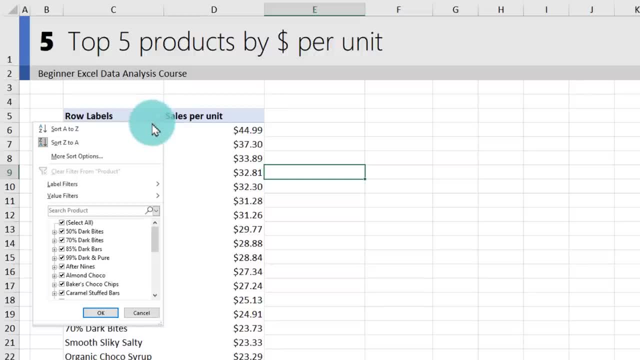 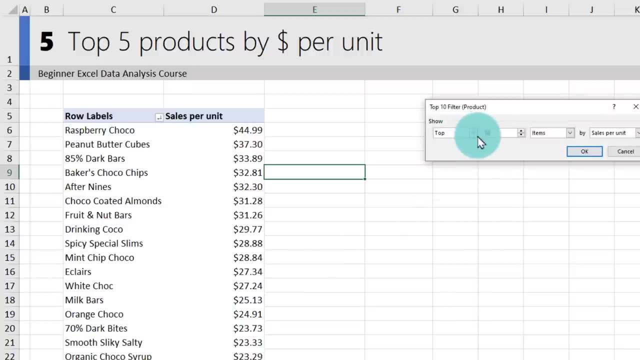 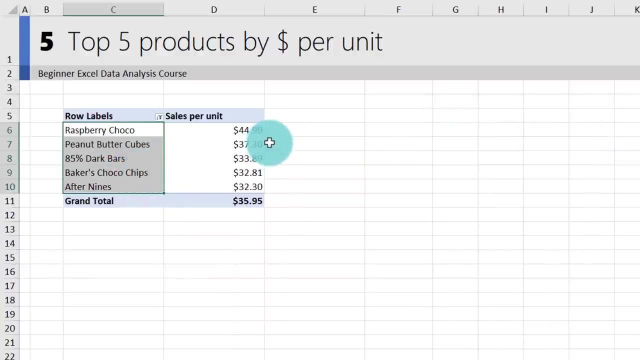 So at this point you can also use row label. Click on that little arrow value, filter top 10 and select five items so that we want to see top five items by sales per unit. So these are my top five items when it comes to making most money per unit sold. 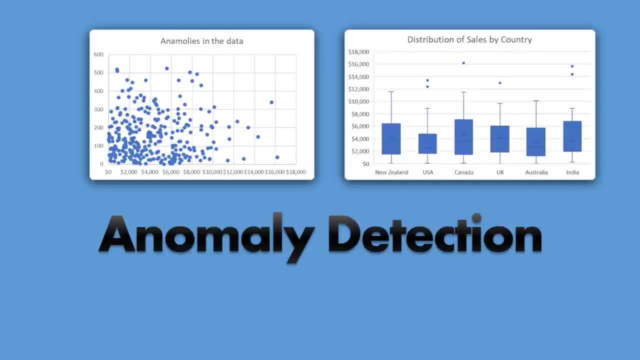 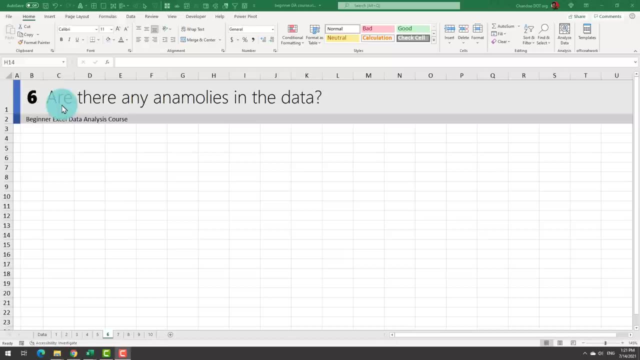 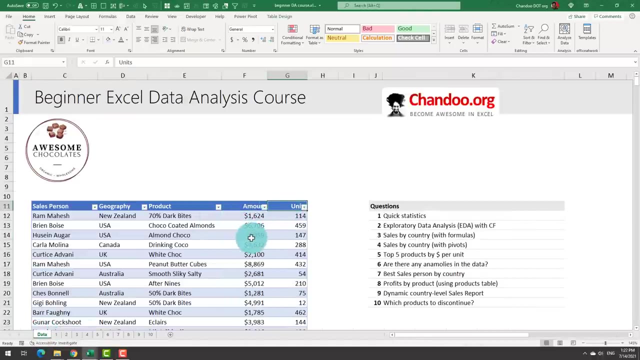 The sixth one is: are there any anomalies in the data? Now, this is kind of like an open-ended question and you can really go any number of ways to get the answer. So I'm going to show you two different techniques. The first one is because we got two columns: amount and unit. I just want to see: are there? 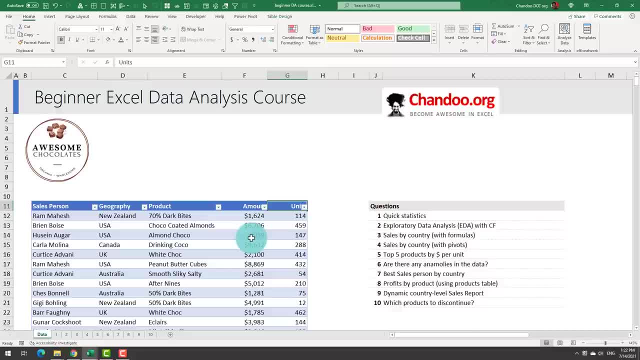 any weird combinations of amount and unit That is So, for example, we're making too much amount but just selling one or two units. or too many units are there but not enough amount. you know those, those could be anomalies. 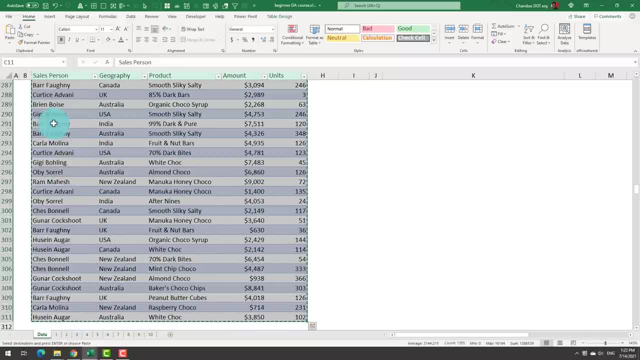 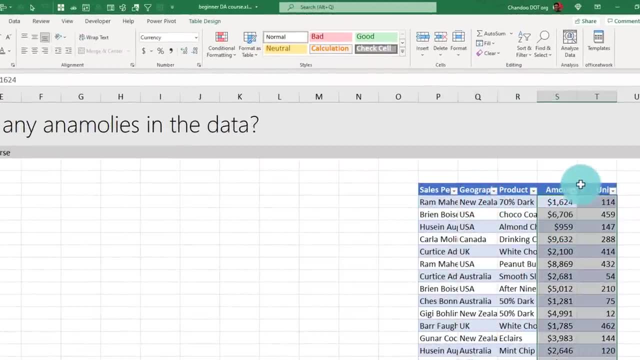 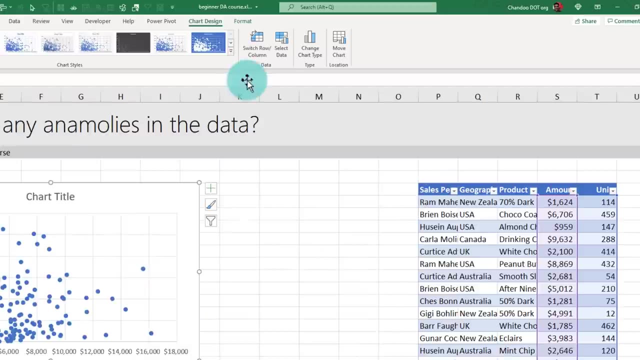 So for the purpose of this exercise, I'm just going to copy this table, control C, paste it here, control V, So we have a copy of the data, And then I'll pick my amount and unit columns and insert a XY scatterplot. 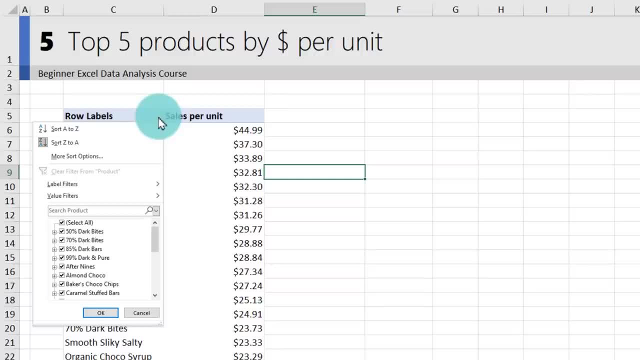 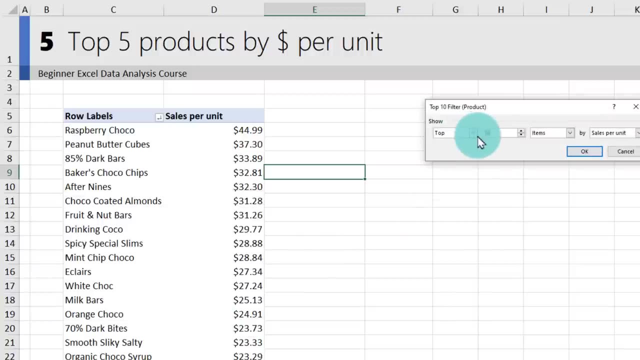 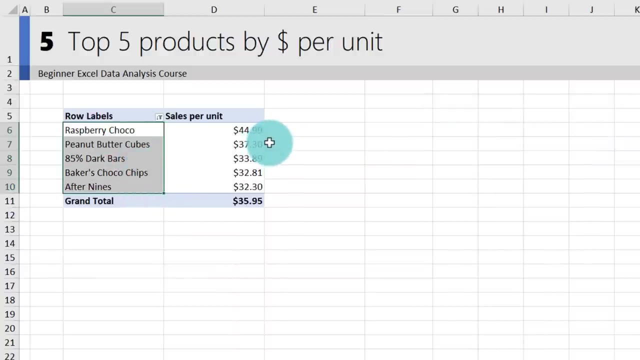 so at this point you can also use row label. click on that little arrow value, filter top 10 and select five items so that we want to see top five items by sales per unit. so these are my top five items when it comes to making most money. 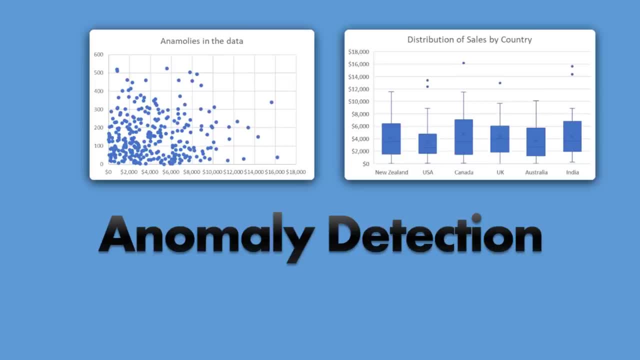 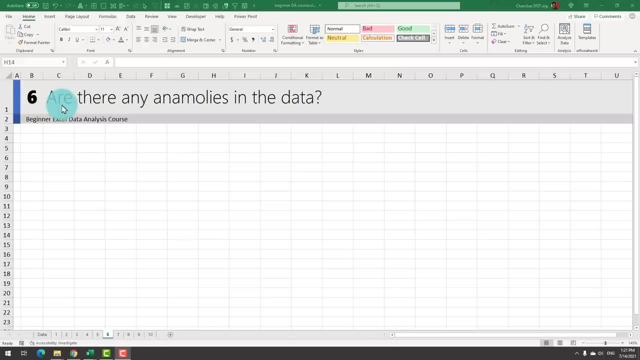 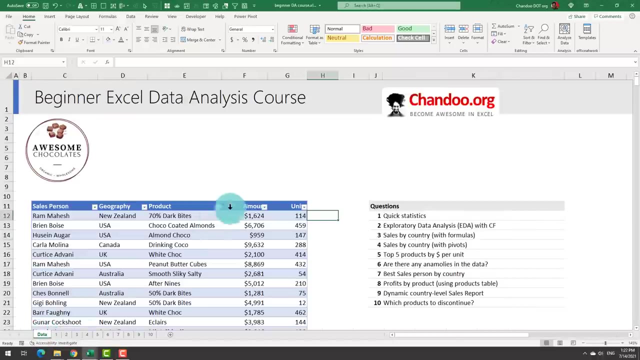 per unit sold. the sixth one is: are there any anomalies in the data? now, this is kind of like an open-ended question and you can really go any number of ways to get the answer. so i'm going to show you two different techniques. the first one is because we got two columns: amount and unit i. 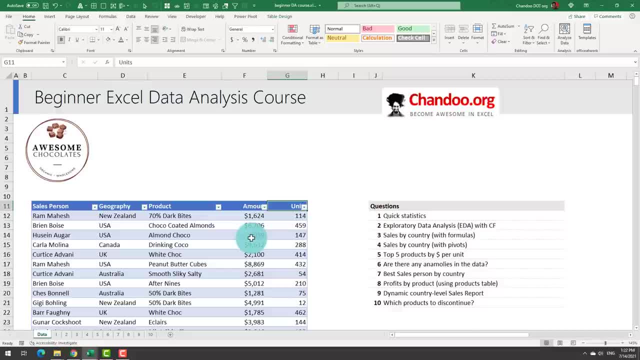 just want to see: are there any weird combinations of numbers that we have to make for the sales per of amount and unit? that is, for suppose we're making too much amount but just selling one or two units, or too many units are there but not enough amount? you know those those could be. 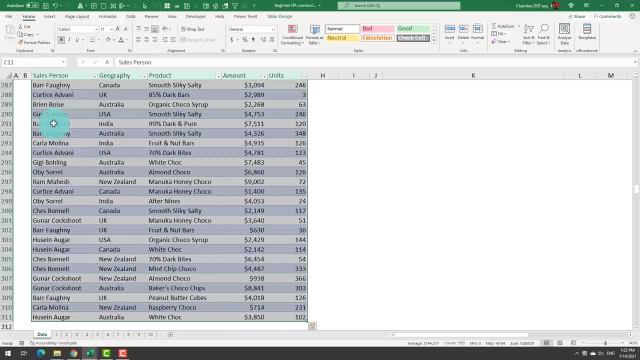 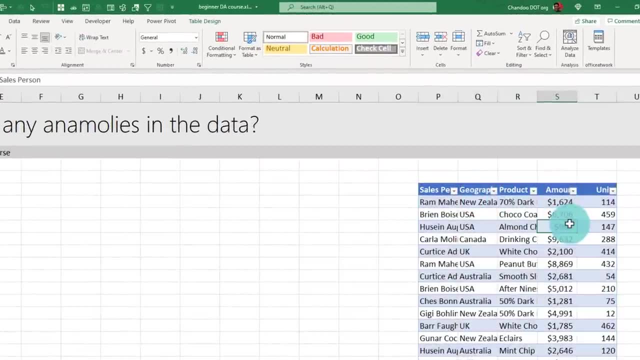 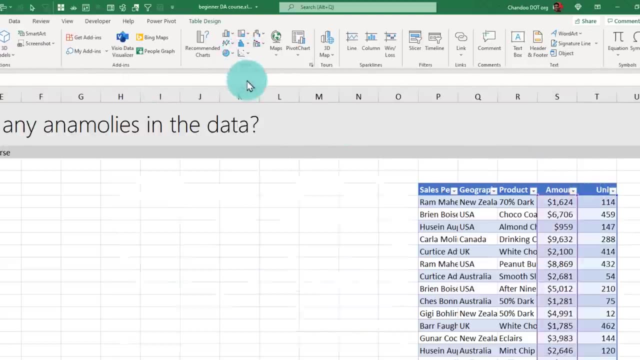 anomalies. So for the purpose of this exercise, I'm just going to copy this table- ctrl c, paste it here, ctrl v, so we have a copy of the data, and then I'll pick my amount and unit columns and insert a x- y scatter plot. what this will do is it will give you a distribution of the data. 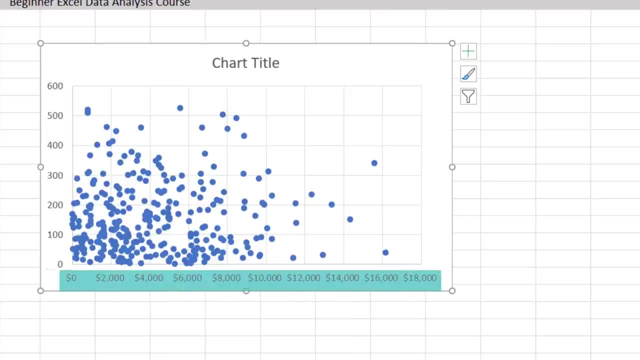 you can see that amount is on the x axis here and on y axis we have the units and you will see that in general they're kind of all over the place, but I would call some of these dots as anomaly like. there is a amount of fifteen thousand six hundred and ten dollars, selling 339 units, so a quite a. 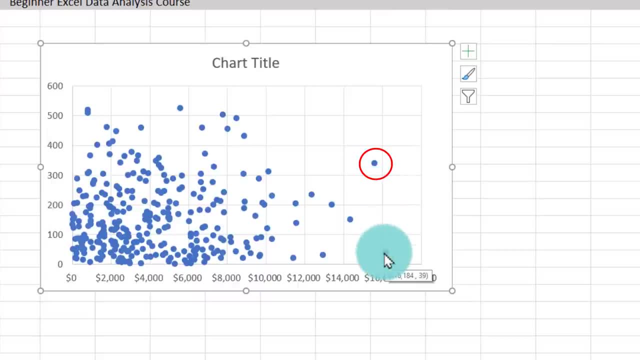 high amount and high amount of data. So for the purpose of this exercise, I'm just going to copy high number of units, whereas this dot is also interesting: sixteen thousand dollars just selling 40 units. So likewise, here are some of the interesting examples. the only problem with 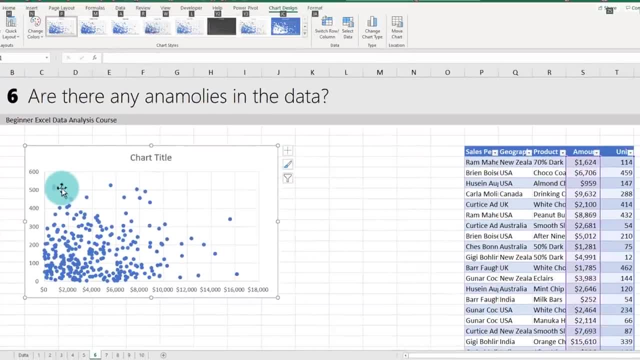 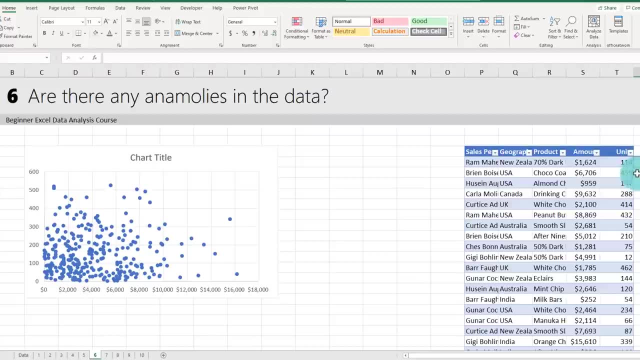 this approach is: you will have to do it manually. like you will examine this, you will say, okay, these look interesting, that looks interesting, that looks interesting. then you will have to go back to your data manually, tag those items for further follow-up. so there is no systematic way to. 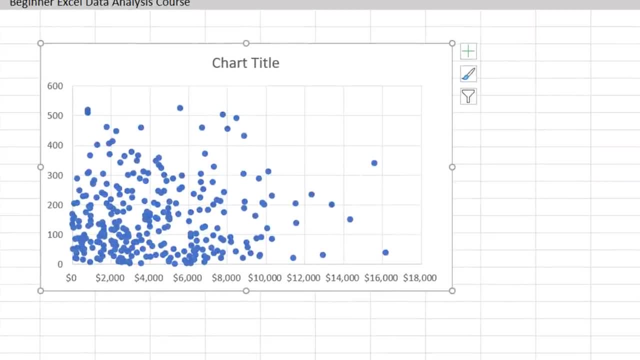 What this will do is it'll give you a data. It'll give you a distribution of the data. You can see that amount is on the X axis here, and on Y axis we have the units and you will see that in general they're kind of all over the place, but I would call some of these. 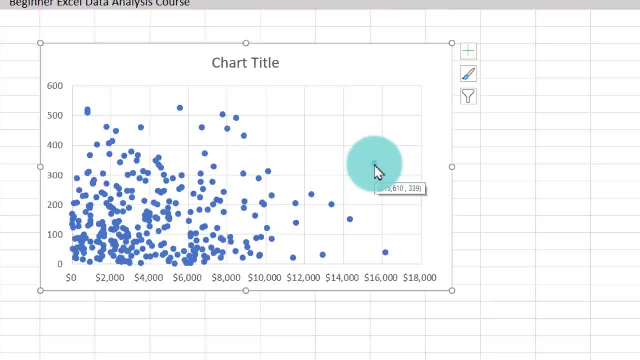 dots as anomaly Like, there is a amount of $15,610 selling 339 units, So a quite a high amount and high number of units, whereas this dot is also interesting- even 40 units. So likewise. here are some of the interesting examples. 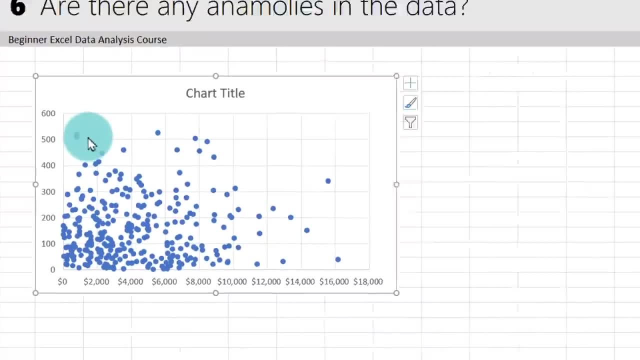 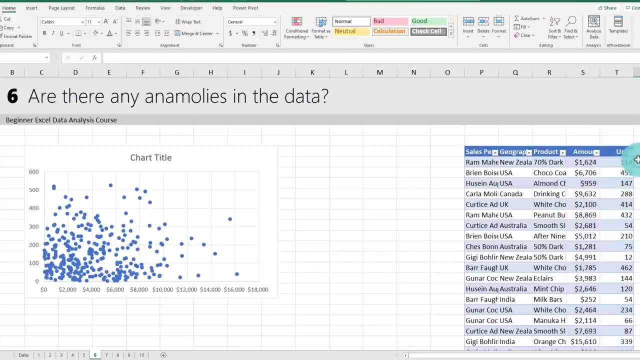 The only problem with this approach is you will have to do it manually. Like you will examine this, You will say, okay, these look interesting, That looks interesting, That looks interesting. Then you will have to go back to your data manually, tag those items for further followup. 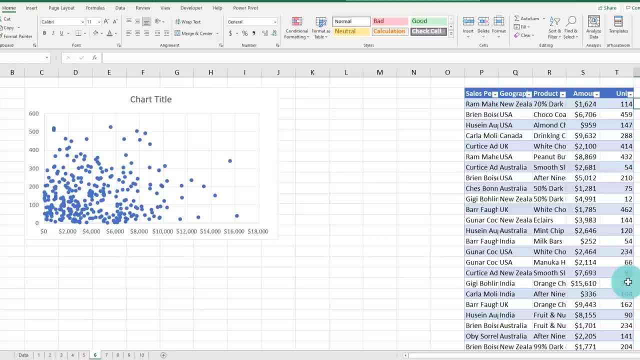 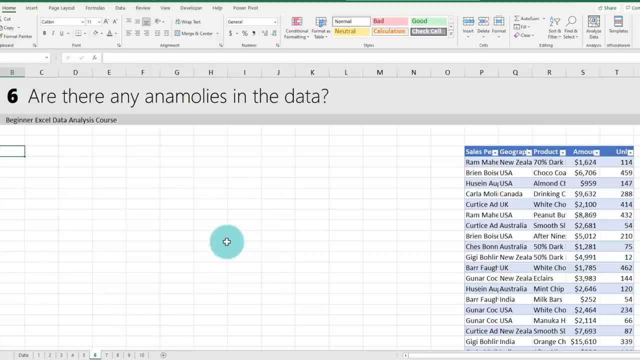 So there is no systematic way to immediately isolate and do it, but that this gives you one technique right: You just look at it and then you visualize. The second method is to understand the distribution of a column and then see if there is anything. 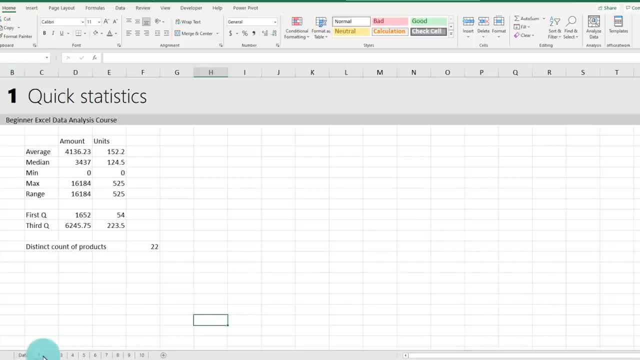 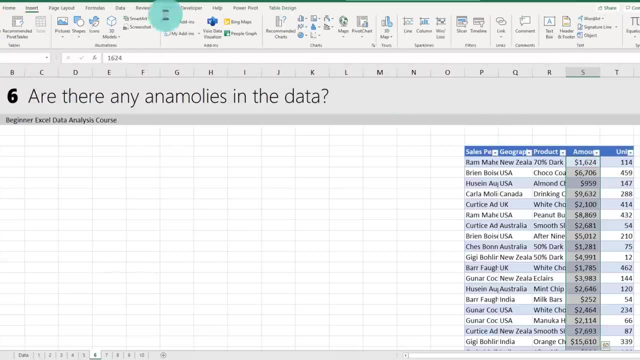 interesting happening, any numbers or outliers. This is kind of like a followup on the quick statistics analysis there. So let's pick the amount column and then we can go to insert. This will work in Excel 2016,, 365, Excel 2019, but in older versions you're not able to. 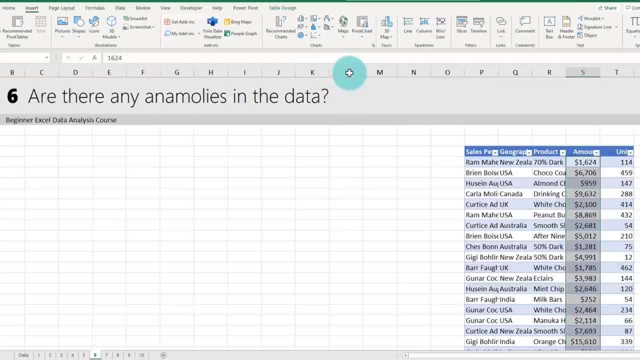 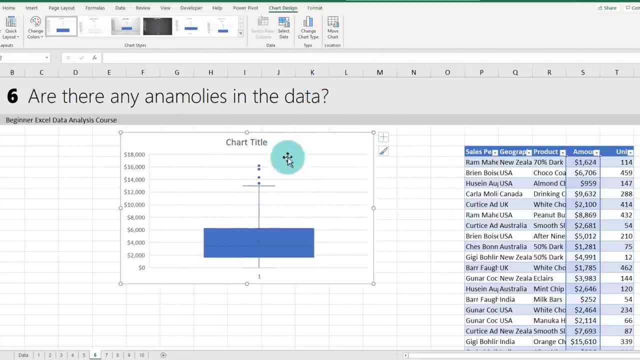 do this natively. So we want to insert a box plot to explore the distribution. And then there is a box- This is called the whisker plot, And here I can see that my amounts are distributed like this. There is um. the median amount is here: 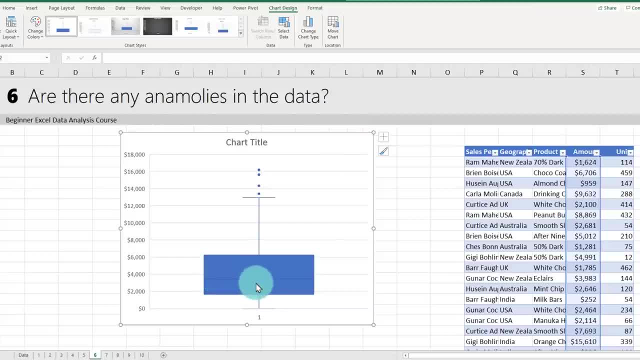 And then we have these values- averages at this place around $4,000.. And then there are some values here and these are my outliers. So there is no tool tip appearing here, but you can see that these amounts higher than 12,000, 13,000 are really kind of breaking the trend. 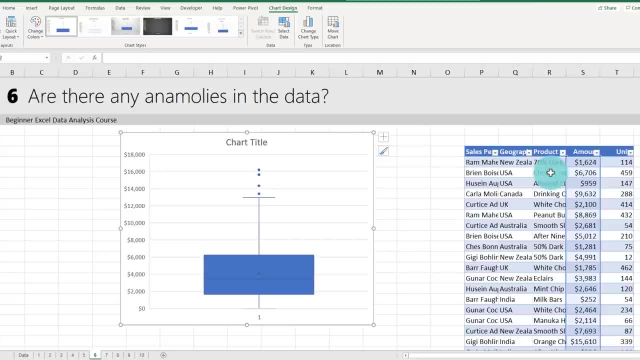 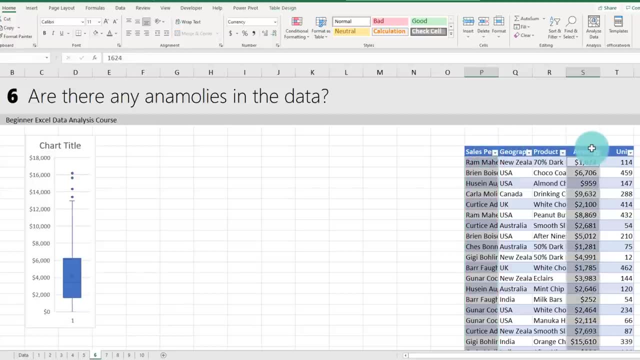 For all amount. But if I want to look this by individual, geography or salesperson, we could also do that: Select the salesperson column and then hold down the control key and select amount column. So we picked both because we have too many people. 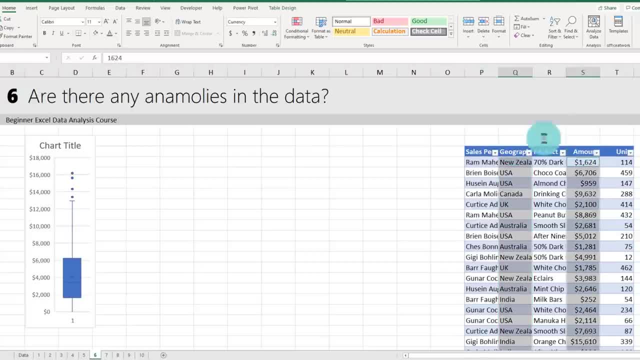 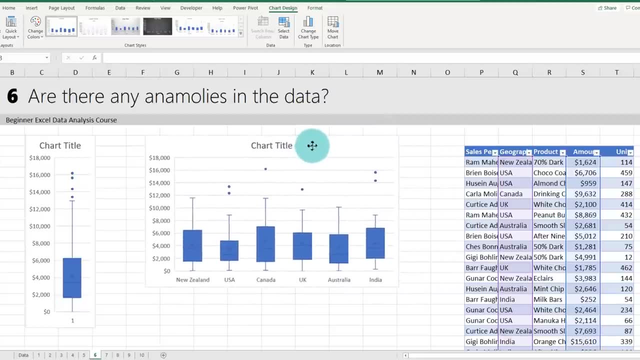 I'm just going to switch to geography and amount- that'll make it a smaller graph- and then insert a box and whisker. So now we are looking at the distribution by geography and this will tell you a completely different story. So you can see, for example, here: um, USA has a very tight. 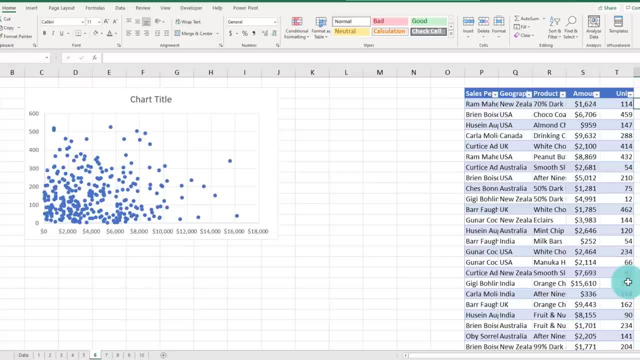 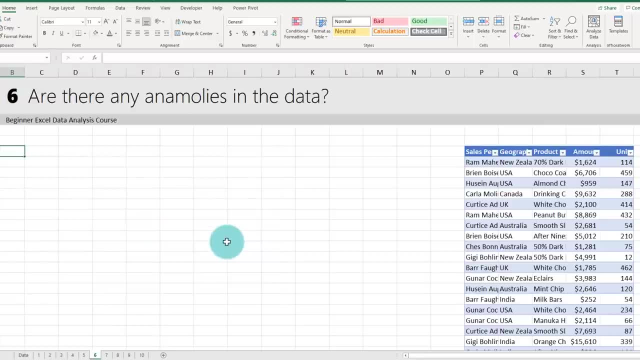 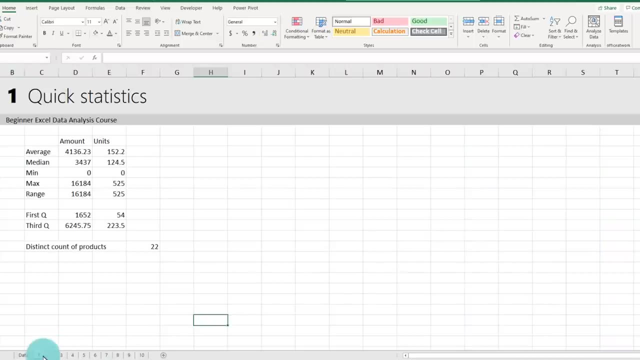 immediately isolate and do But that. this gives you one technique right: you just look at it and then you visualize. the second method is to understand the distribution of a column and then see if there is interest, anything interesting happening, any numbers or outliers. this is kind of like a follow-up on the quick. 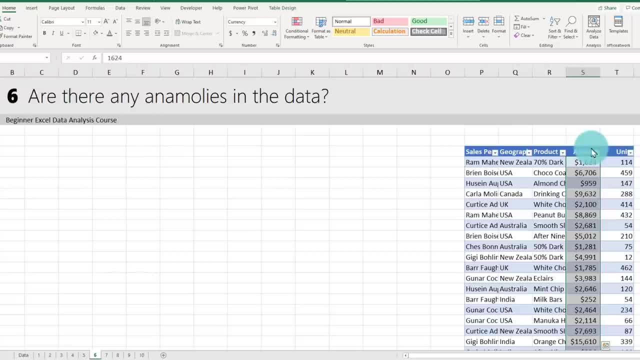 statistics analysis there. so let's pick the amount column and then we can go to insert. this will work in excel 2016, 365, excel 2019, but in older versions you're not able to do this natively. So we want to insert a box plot to explore the distribution, and then there is a box and whisker. 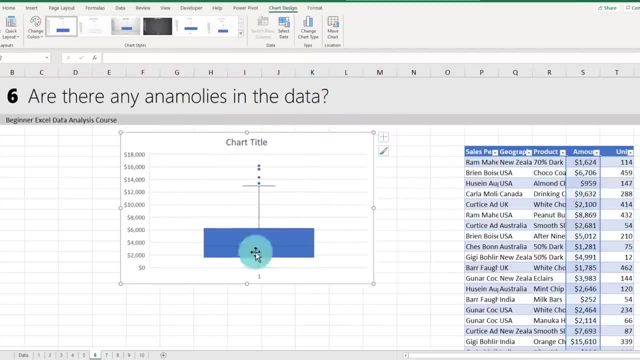 plot, and here I can see that my amounts are distributed like this: there is the median amount is here- and then we have these values- average is at this place around four thousand dollars- and then there are some values here and these are my outliers, so there is no tooltip appearing here. 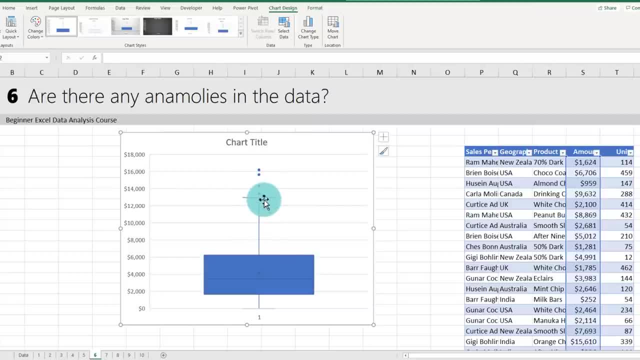 but you can see that these amounts higher than the outliers, and then there are some values here that are higher than twelve thousand. thirteen thousand are really kind of breaking the trend. this is my overall amount, but if I want to look this by individual, geography or salesperson, we 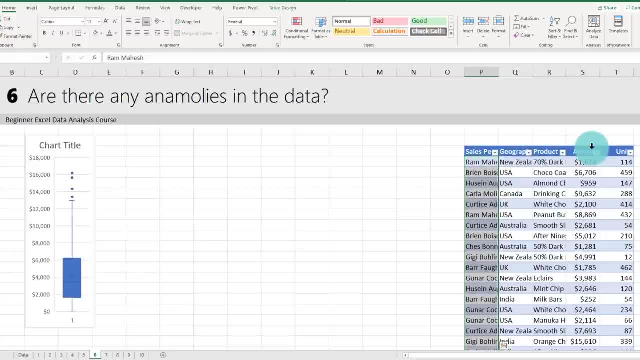 could also do that: select the salesperson column and then hold down the control key and select amount column. so we picked both, because we have too many people. I'm just going to switch to geography and amount. that will make it a smaller graph- and then insert a box and whisker. so now 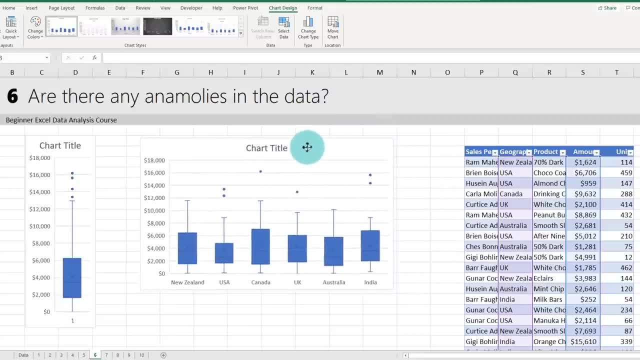 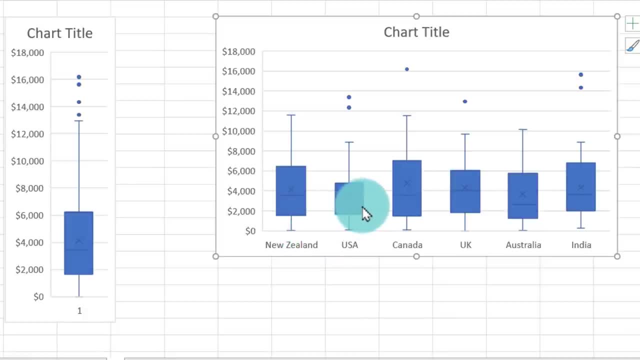 we are looking at the distribution by geography and this will tell you a couple of things about the distribution by geography, and this is a completely different story. so you can see, for example, here USA has a very tighter middle, indicating that most of the middle half of the 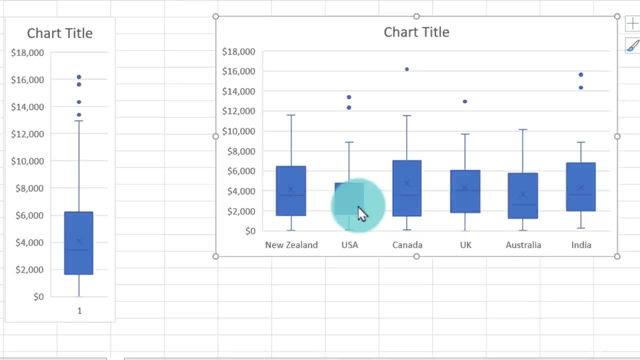 Um, The middle uh, indicating that most of the middle half of the 50 middle half of the sales are all happening in the bucket of about 15, $1,800 to $5,000, whereas the wider this box is, the wider there is a variation, uh, and also the number of dots on the top indicate. 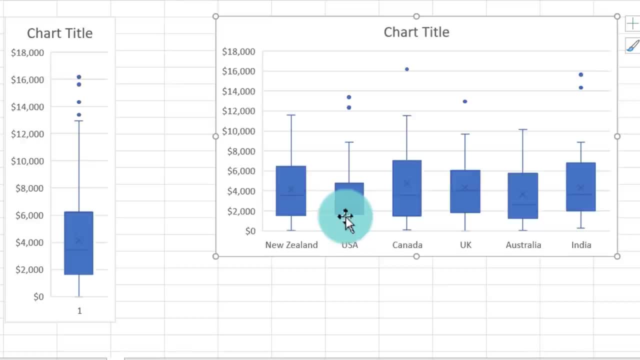 fifty middle half of the sales are all happening in the bucket of about fifteen, eighteen hundred dollars to five thousand dollars, whereas the wider this box is, the wider there is a variation, and also the number of dots on the top indicate like how many values are really out there and and 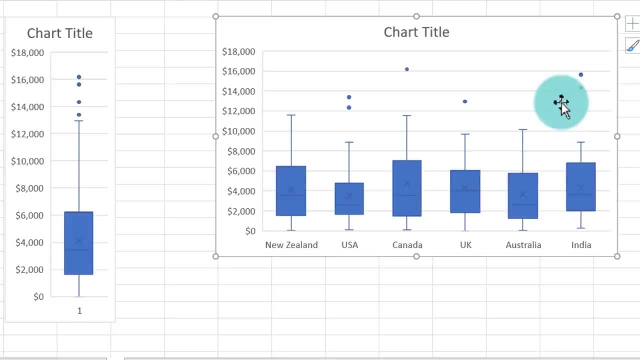 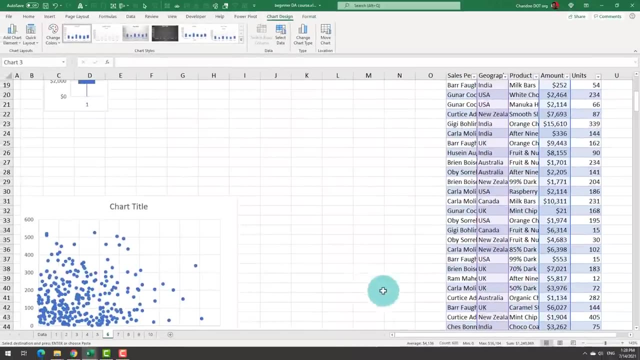 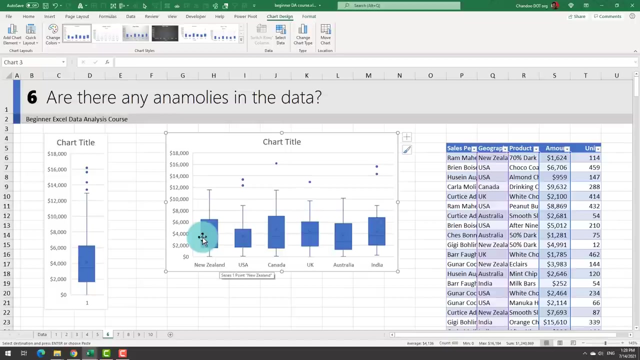 like: how many values are, uh, really out there, uh, and, and that'll give you a different picture. So using these two graphs, this box plot index By scatterplot, we are able to visually spot anomalies in the data and ask some more interesting. 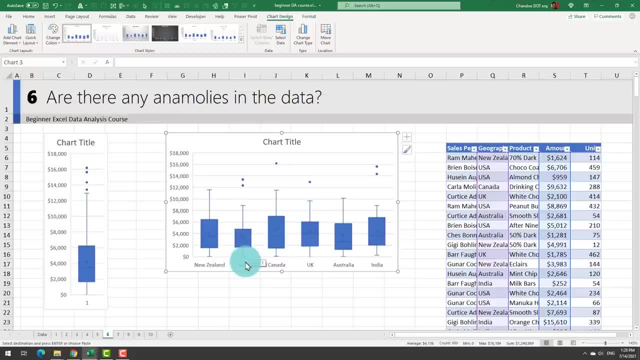 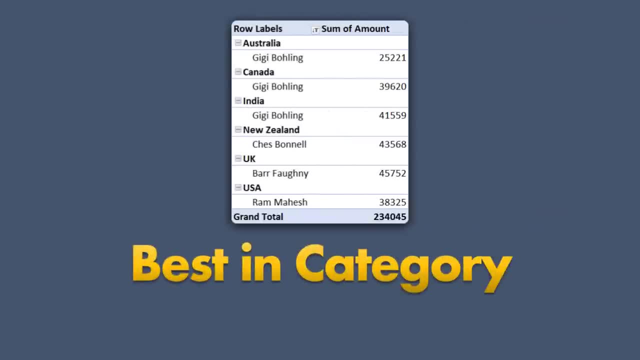 questions like: you know what's going on with the USA, like how come their sales are all more uniform um and and uh, and understand what is happening to the customers there. In this situation, we would like to look at who are our best performing sales persons. 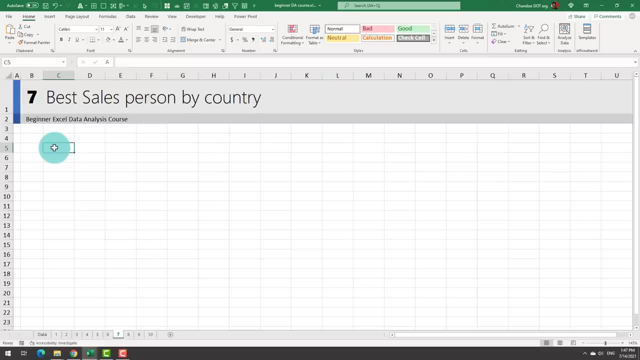 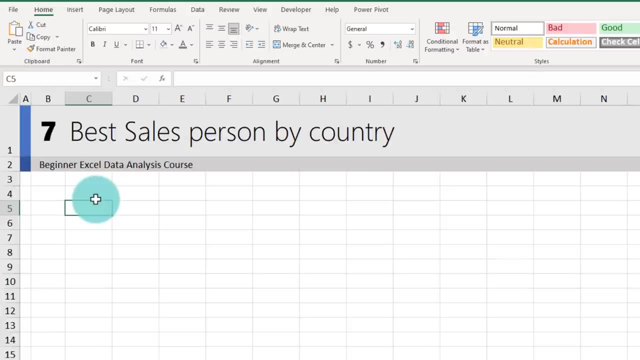 by country. We can take the same concept and look at either best or worst performing sales person or product, or any other combination for that matter. Again, in this situation, you can use both pivot tables or formulas to get the answer. I'm going to show you the pivot table technique because it is slightly simpler and faster. 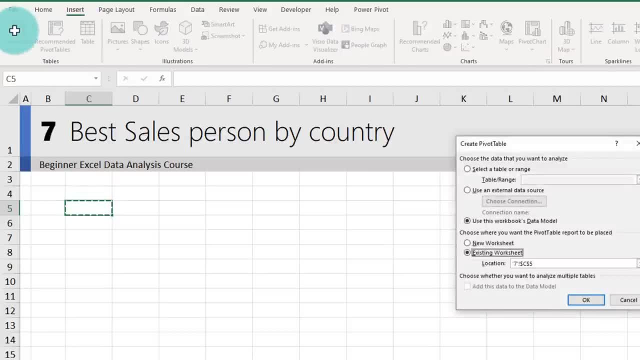 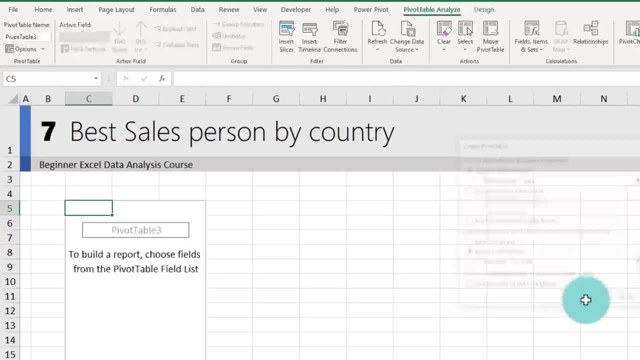 to get that result. So we insert a pivot table, select the table as a data- It doesn't matter whether you add it to the data model or not- and let's click okay Now, because we are interested in the country, we will start off by putting geography first. 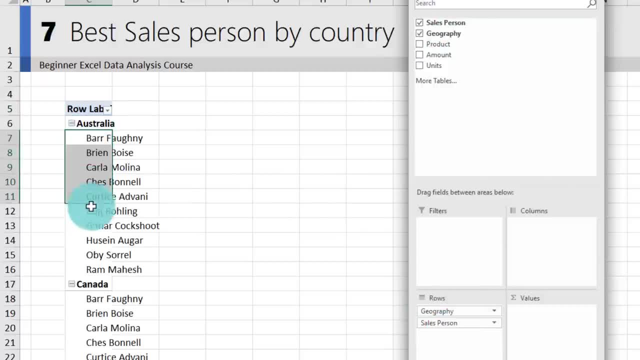 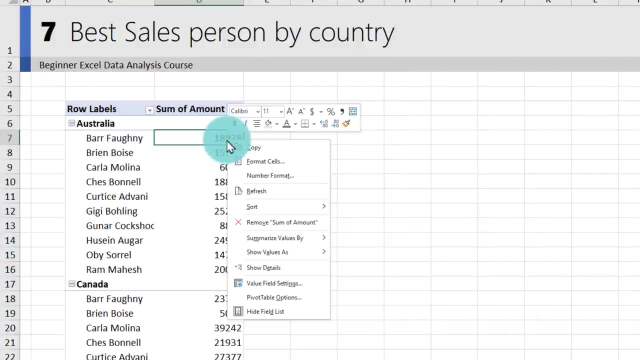 and then add salesperson Underneath. So we will have one row per sales person within each geography. Here I'm just going to assume that by best salesperson we mean the person who is selling most amount, So we will drag the amount column, put that there and right click on the amount sort. 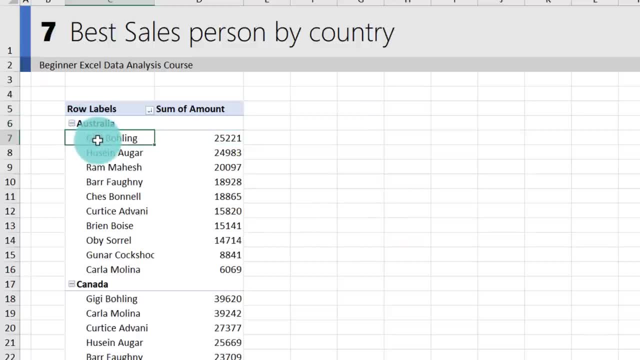 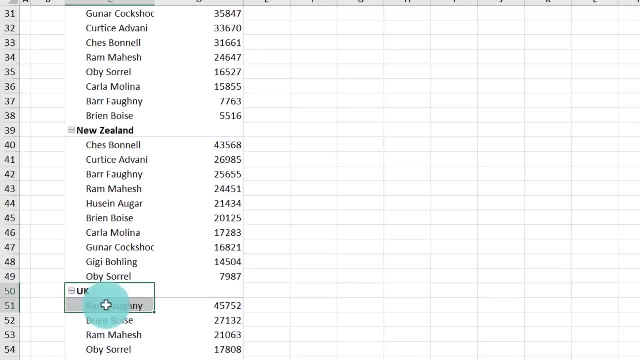 largest to smallest. So we can see: within Australia Gigi's name comes up, Canada Gigi again. India also Gigi. New Zealand chess and UK bar. How do I see only that name and none of these others? 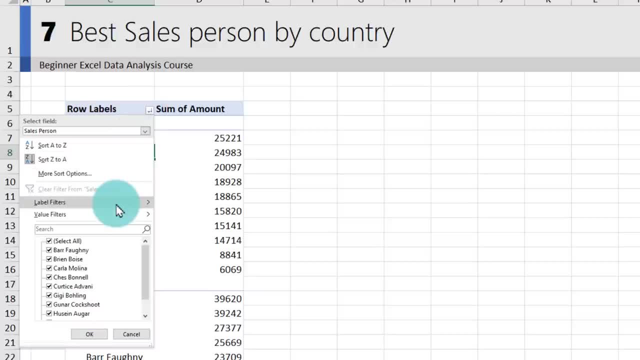 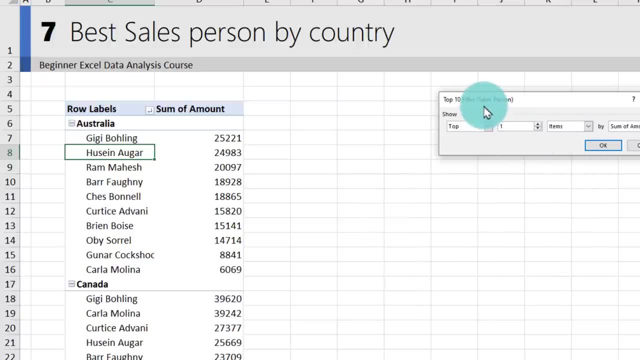 This is when we select one of these names, click on that button, value filter, top 10, and then simply say: I just want to see the top one item by the amount of within the salesperson column. This will kind of change the pivot table to show these amounts alone. 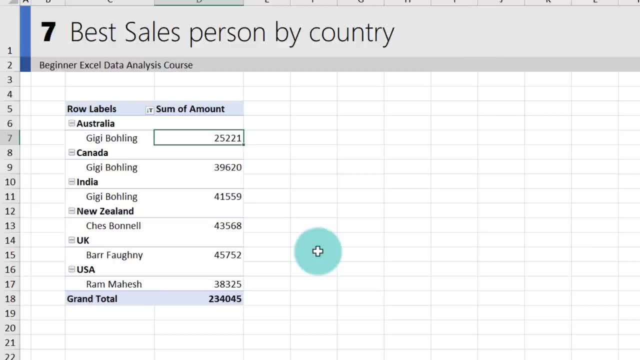 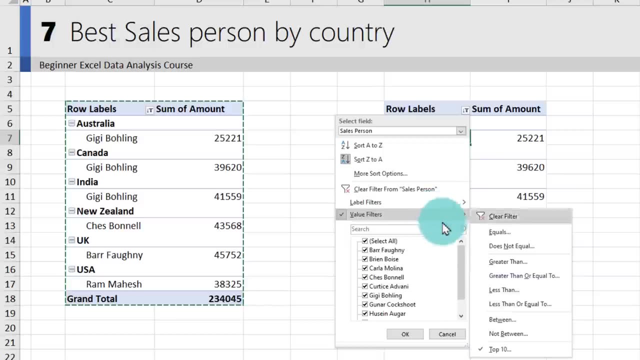 And there you go: Best salesperson by the country. How would we do the same for- but look at, the lowest performing salesperson? all we have to do is make a copy, Go back to the top 10 filter where it says top one, change this to bottom one and we. 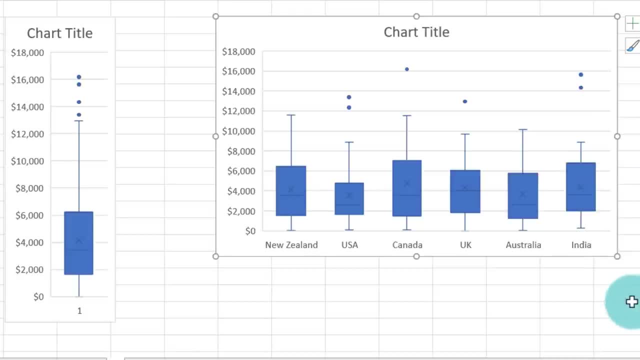 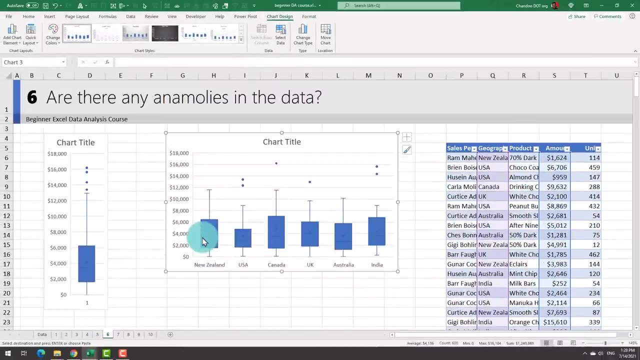 that will give you a different view of the distribution. so, using these two graphs- this box plot and the x- y scatter plot- we are able to visually spot anomalies in the data and ask some more interesting questions, like you know what's going on with the USA, like how come their sales are all more uniform, and understand what is happening to the customers. 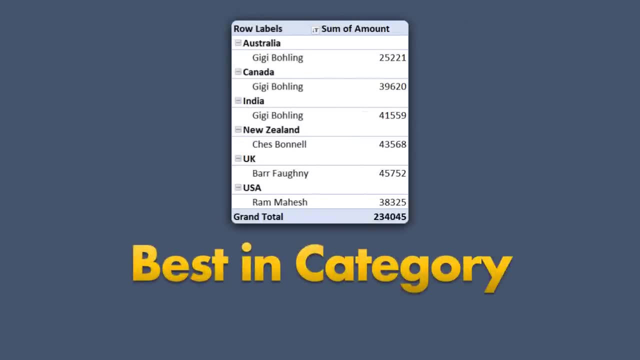 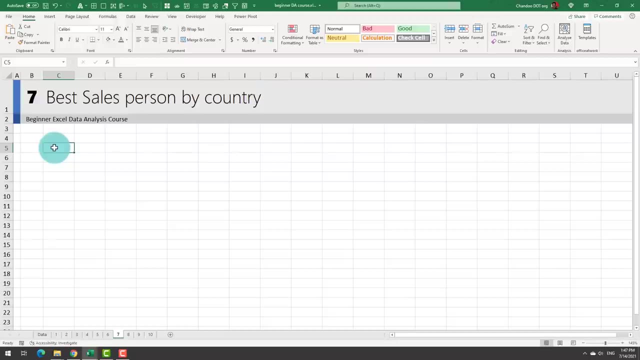 there. in this situation, we would like to look at who are our best performing sales persons by country. we can take the same concept and look at either best or worst performing sales person or product, or any other combination for that matter. again, in this situation, you can use both pivot tables or formulas to get the 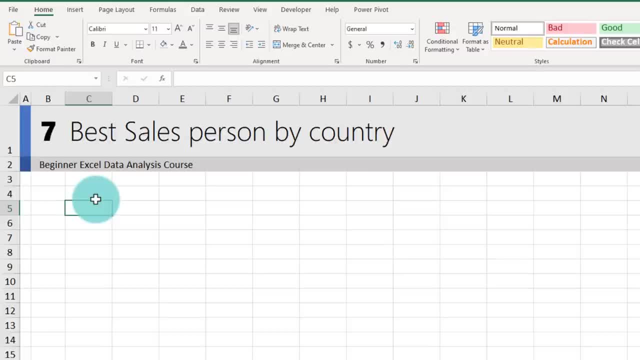 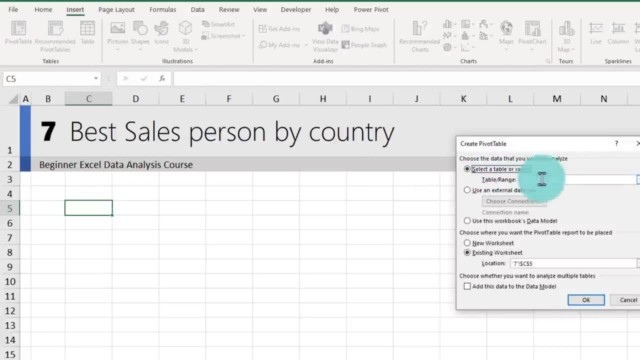 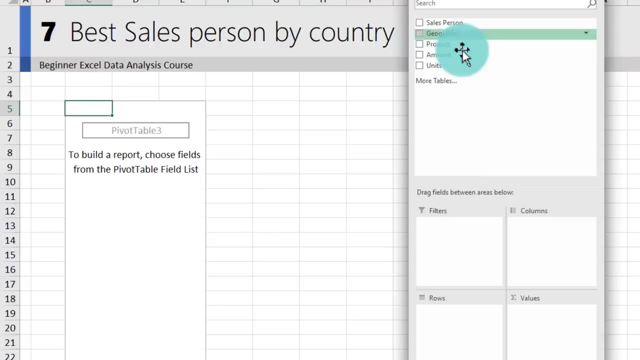 answer. i'm going to show you the pivot table technique because it is slightly simpler and faster to get that result. so we insert a pivot table, select the table as a data- it doesn't matter whether you add it to the data model or not- and let's click ok now because we're 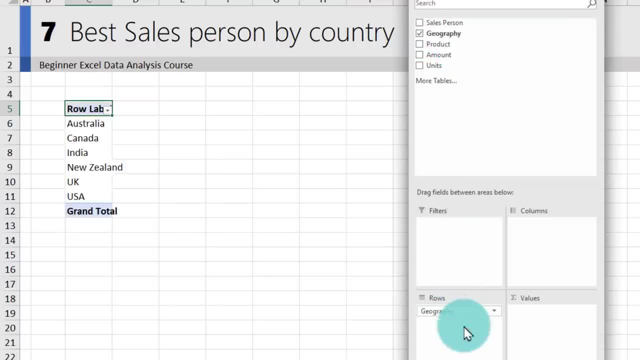 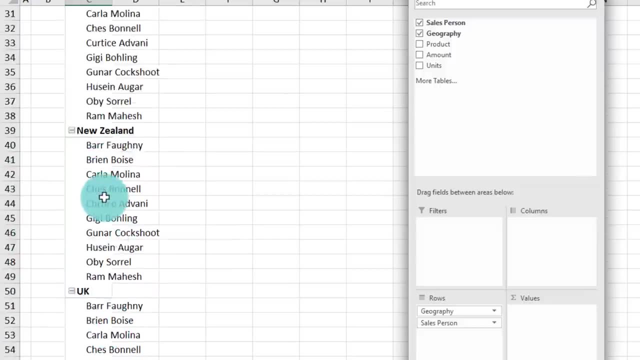 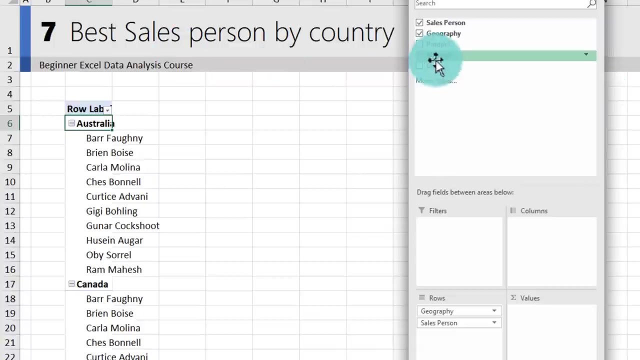 interested in the country. we will start off by putting geography first and then add sales person underneath, so we will have one row per sales person within each geography here. i'm just going to assume that by best sales person we mean the person who is selling most amount, so we will drag. 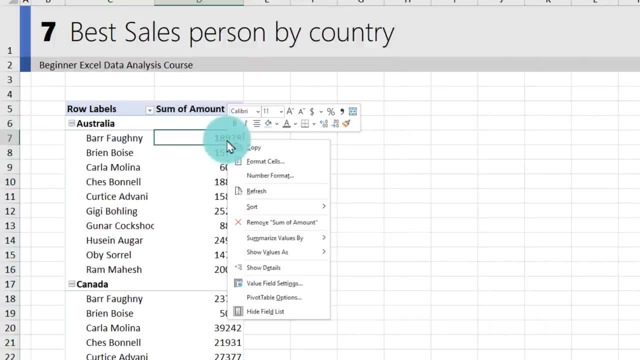 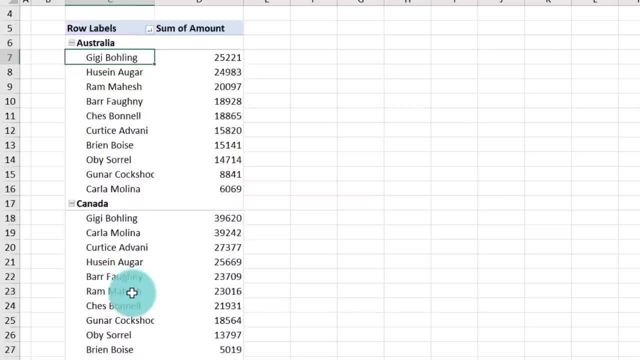 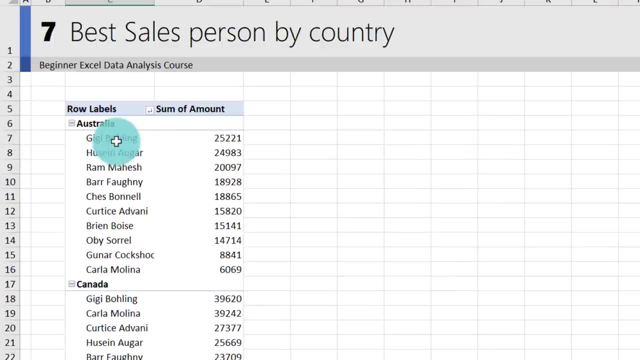 the amount column. put that there and right click on the amount. sort largest to smallest so we can see: within australia, gigi's name comes up. canada, gigi again. india also gigi. new zealand, chess and uk bar. how do i see only that name and none of these others? 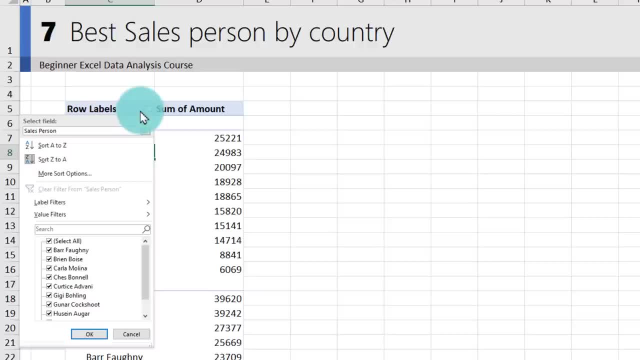 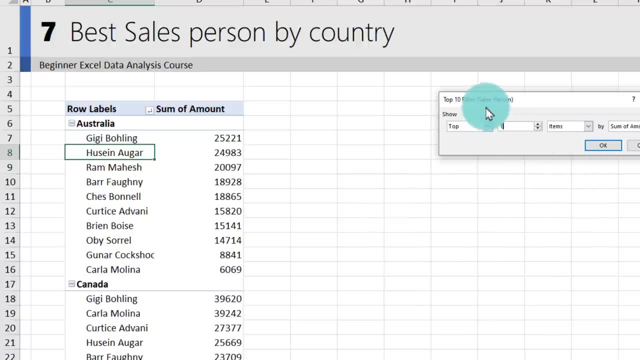 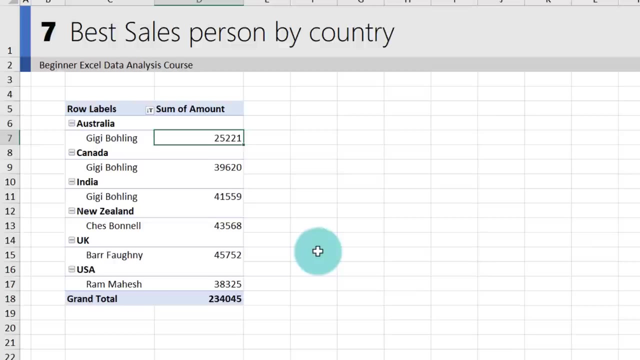 this is when we select one of these names, click on that button, value filter, top 10- and then simply say: i just want to see the top one item by the amount within the sales person column. this will kind of change the pivot table to show these amounts alone. and there you go, best sales person. 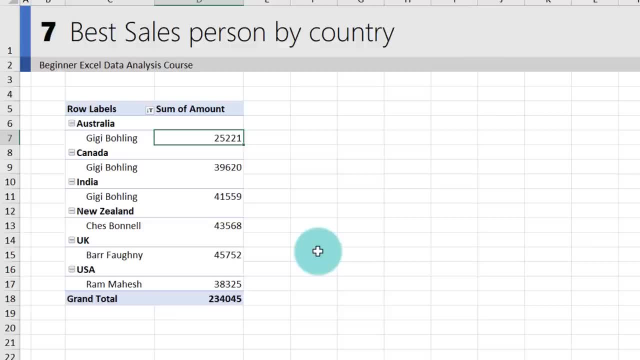 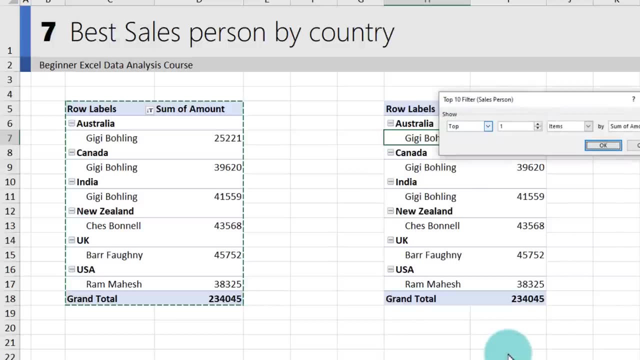 by the country. how would we do the same for- but look at- the lowest performing sales person? all we have to do is make a copy, go back to the top 10 filter, where it says top one, change this to bottom one and we will get the corresponding. 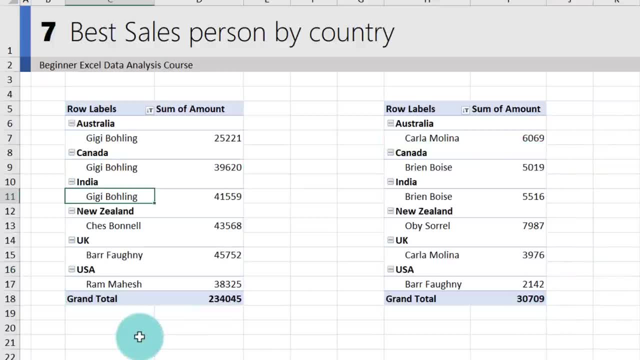 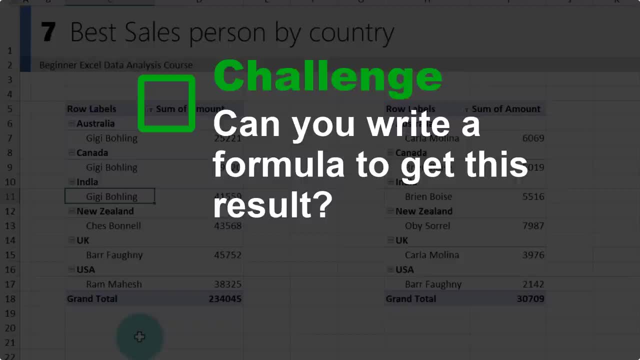 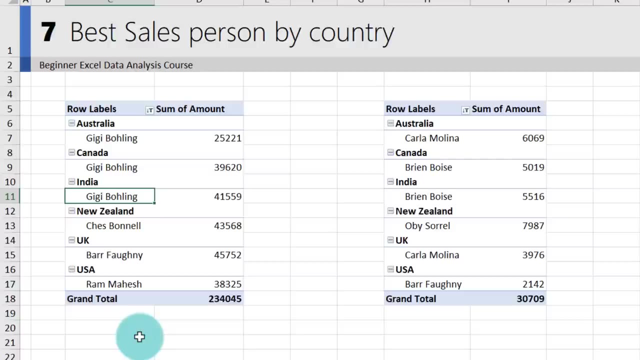 will get the corresponding person's name as well. Now here is a fun challenge for you. How would you get the similar result, but use Excel formulas? take it up as a challenge, write the formulas And if you either encounter some struggle or you come up with successful answers, share. 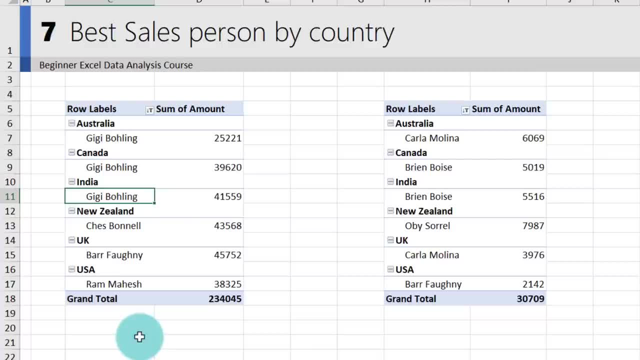 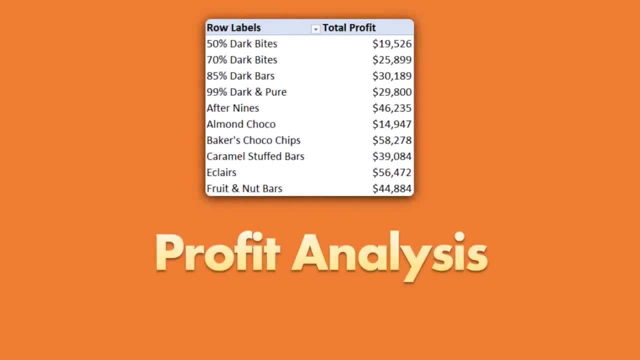 them in the video comments so that I can remark or I can talk about more If needed. all the very best for this example. we would like to look at profits by product, but obviously we don't have the profit information. We only know how much amount we are making. 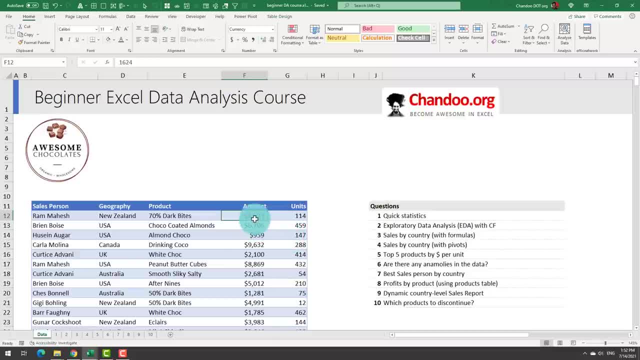 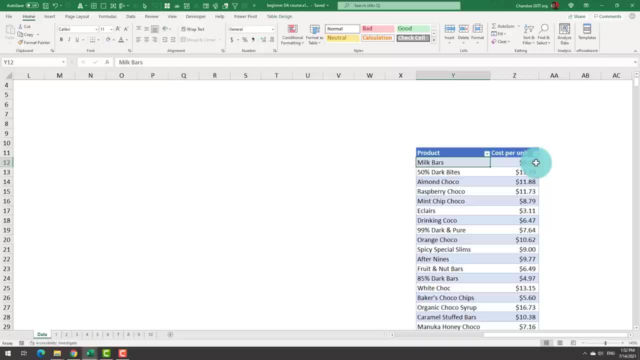 We do need to have a sense of what is the cost that we are incurring. when we generated this revenue For that purpose, I have a supporting table here. My product table tells me what is the cost per unit that we incur. We can combine this table and that table. 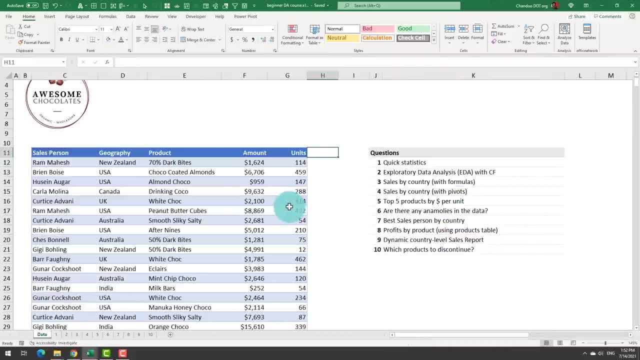 In a number of ways. in many times when you are doing the data analysis, such combination of data from two or three different tables is fairly common. I will show you one common Excel technique that we can use to combine data like this. It is to use the lookup formulas. 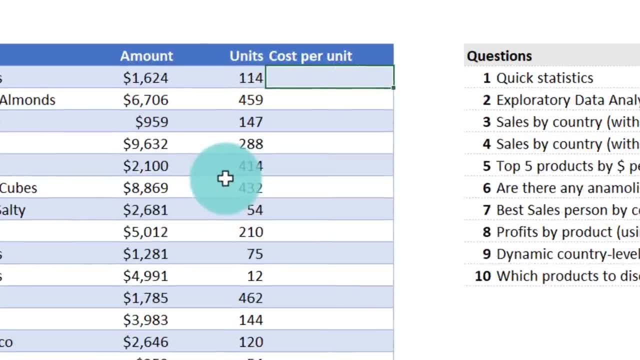 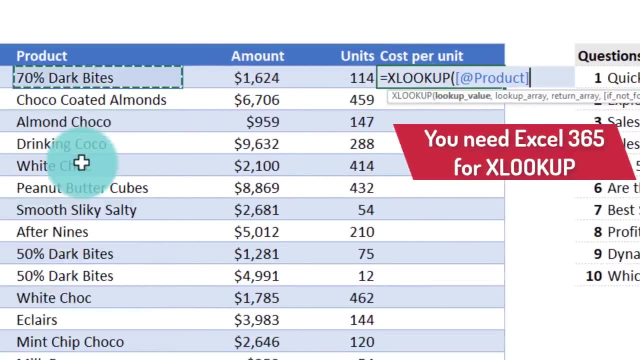 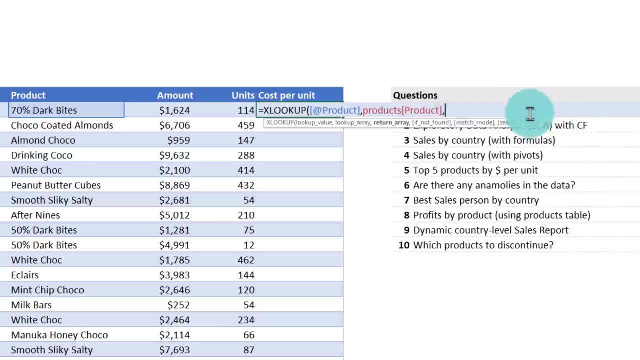 So I will say cost per unit here we will simply say XLOOKUP. You can also use VLOOKUP if you are using an older version of Excel. product name at the rate product, Then select the product column here and then specify the product's cost. 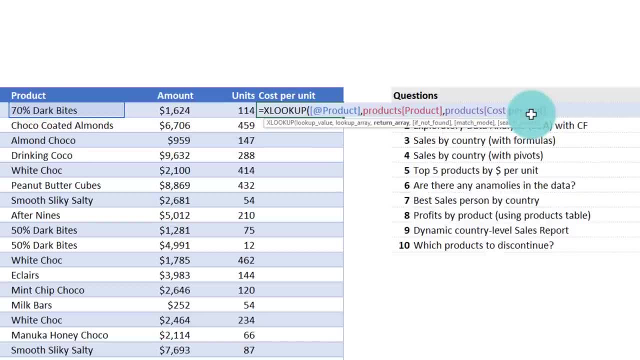 So I will say: products table cost per unit. So this XLOOKUP function, it will look up 70% dark bytes in the products table and then tell you what is the cost per unit. It will do so for all other items as well, because it is a table and you type formula. 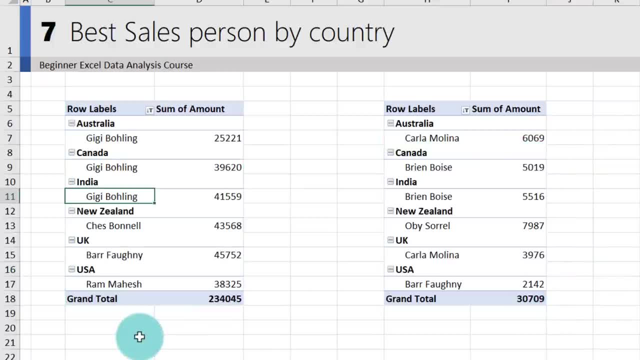 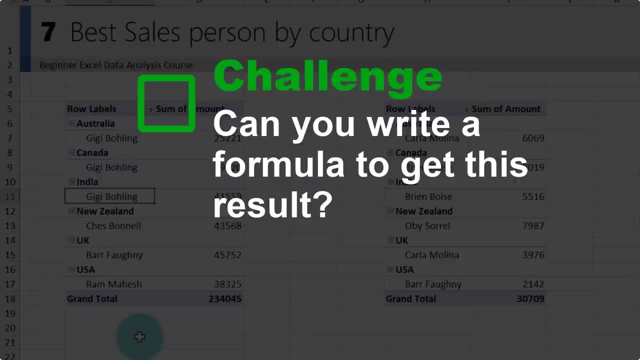 person's name as well. now here is a fun challenge for you. how would you get the similar result, but use excel formulas. take it up as a challenge, write the formulas and if you either encounter some struggle or you come up with successful answers, share them with your friends and family. 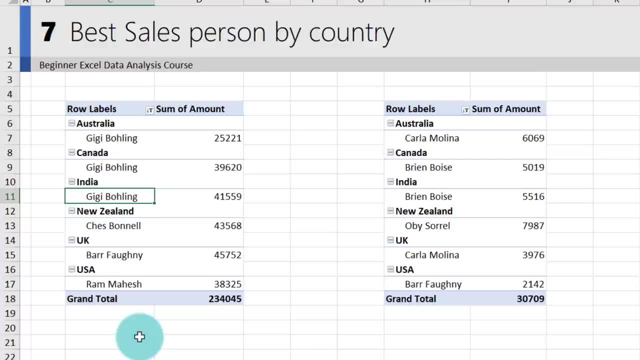 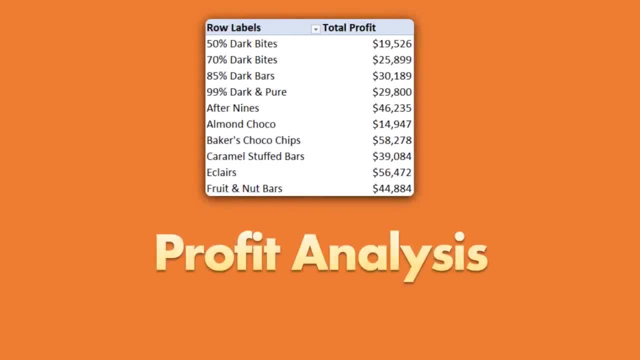 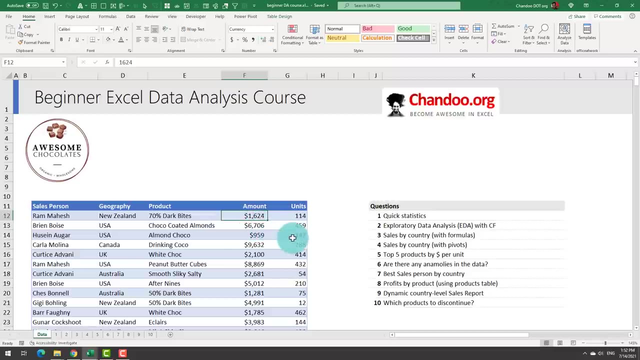 in the video comments so that i can remark or i can talk about more if needed. all the very best for this example. we would like to look at profits by product, but obviously we don't have the profit information. we only know how much amount we are making. we do need to have a sense of what is the 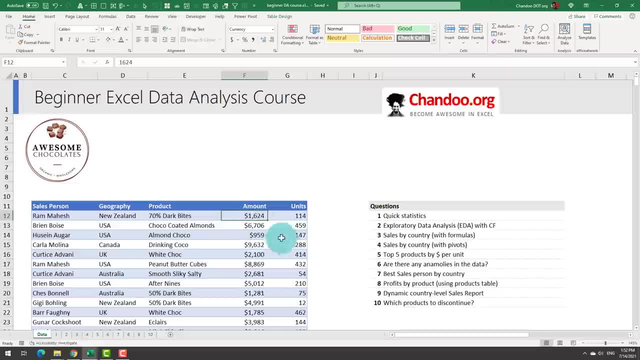 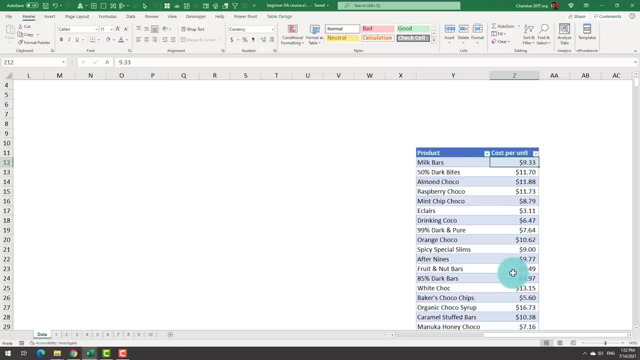 cost that we are incurring when we generated this revenue for that purpose. i have a supporting table here. my product table tells me what is the cost per unit that we incur. we can combine this table and that table in a number of ways. in many times when you 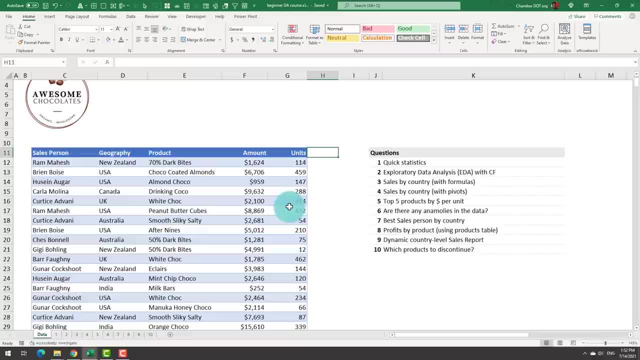 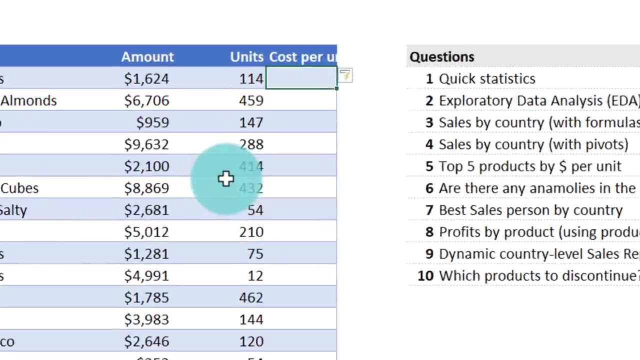 are doing the data analysis. such combination of data from two or three different tables is fairly common. i will show you one common excel technique that we can use to combine data like this. it is to use the lookup formulas, so i will say cost per unit here. we will simply say: 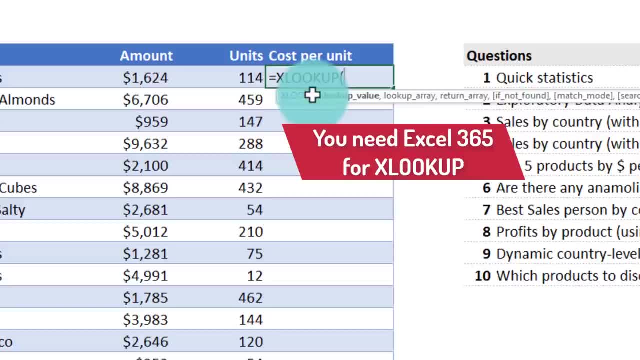 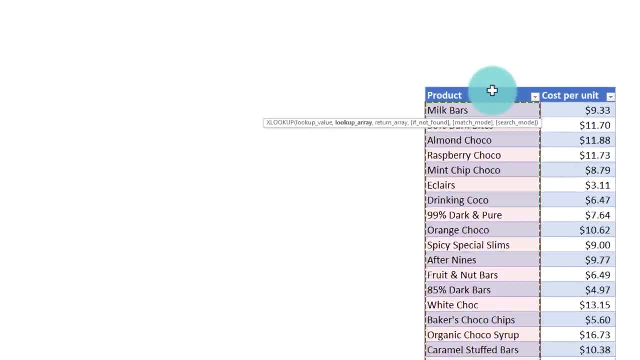 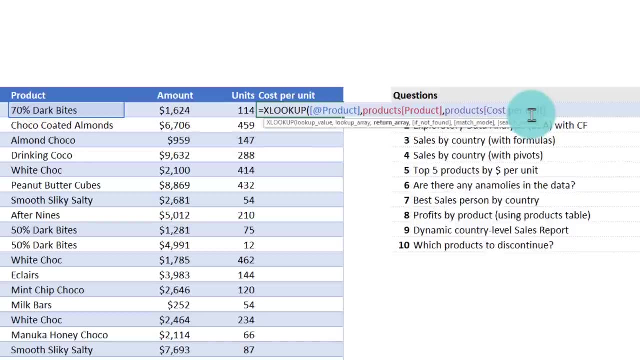 x lookup. you can also use vlookup if you are using an older version of excel. product name at the rate product and then select the product column here and then specify the product's cost. so i'll say products table cost per pro unit. so this x lookup function. 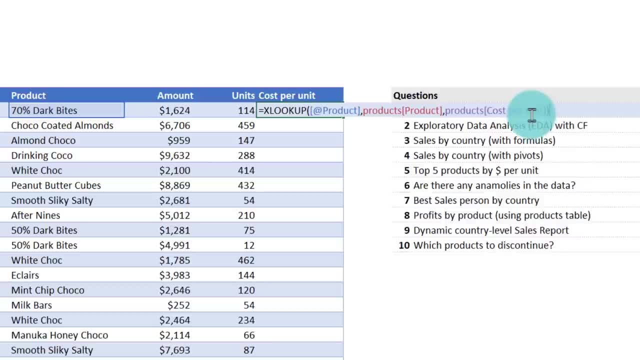 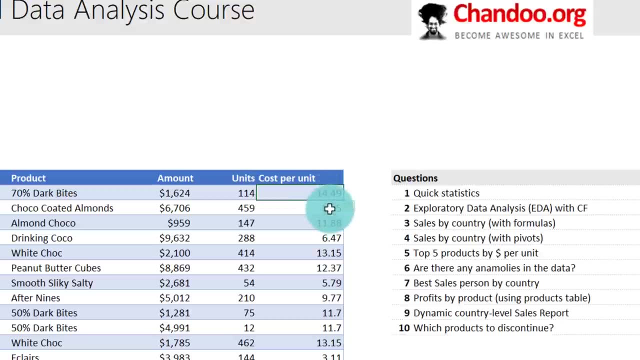 it will look up 70 dark bytes in the products table and then tell you what is the cost per unit. it will do so for all other items as well, because it is a table. when you type formula in one cell, excel will automatically fill the same formula all the way through. 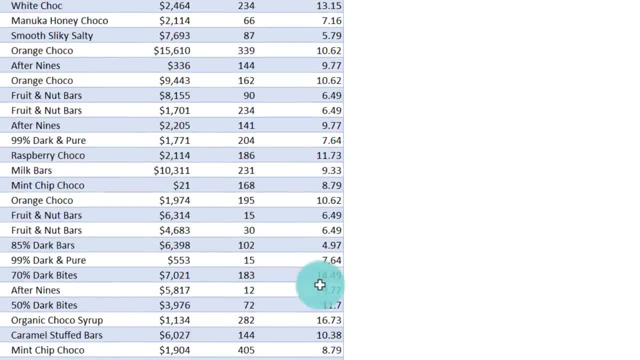 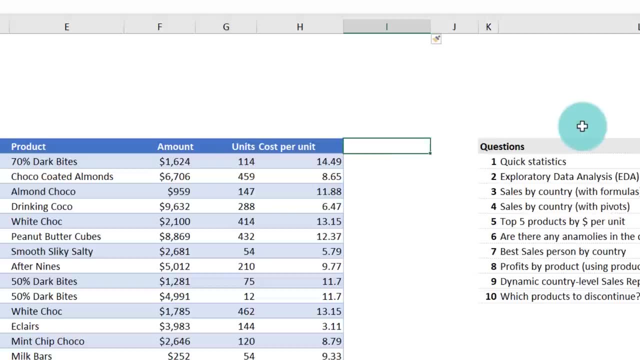 in one cell, Excel will automatically fill the same formula all the way through, giving you cost per unit everywhere. Let me insert a column here. I will calculate total cost. I will just call this as cost, which would be cost per unit times number of units. 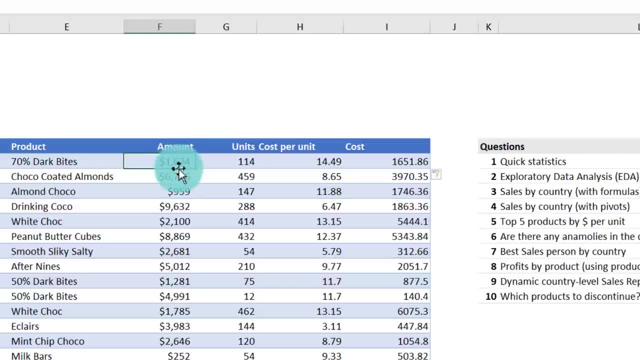 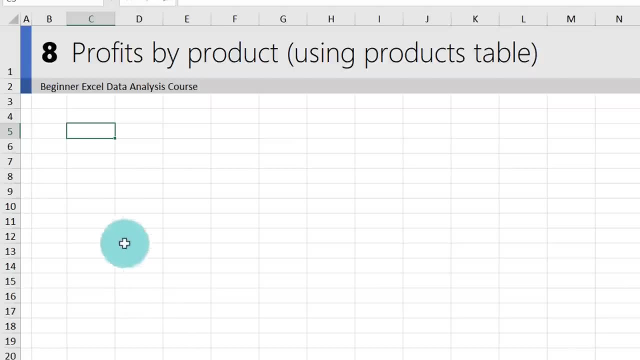 You can see that, for example, in this case our amount is 1624, but our cost is 1651. So we actually incurred a loss on this particular line. So let's go ahead and now calculate the total profit and then do the analysis. 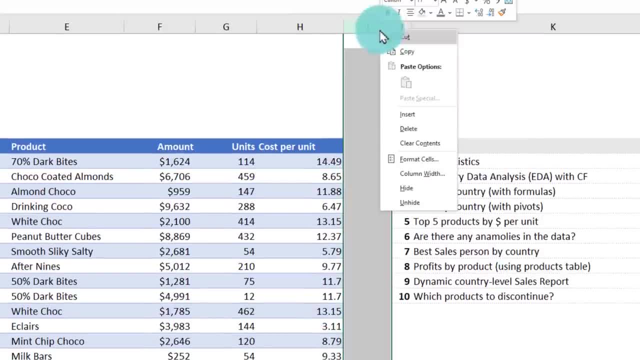 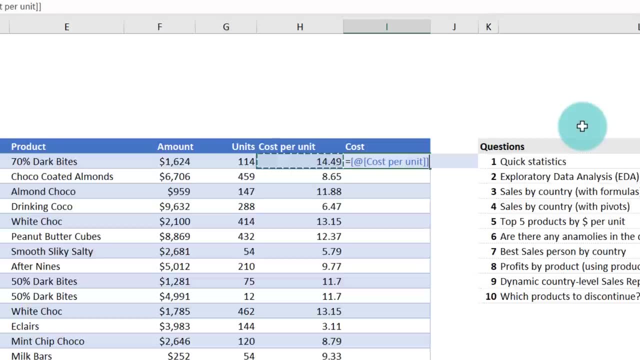 giving you cost per unit everywhere. we will now calculate. let me insert a column here. i'll calculate total cost. i'll just call this as cost, which would be cost per unit times number of units. you can see that, for example, in this case our amount is 1624, but our cost is 1651, so we actually 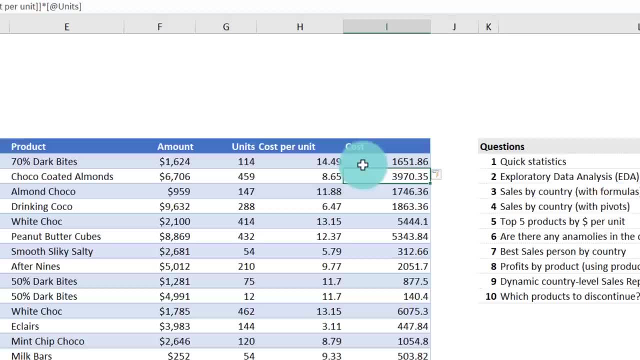 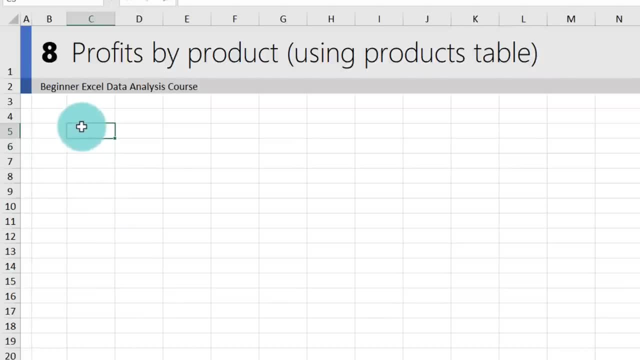 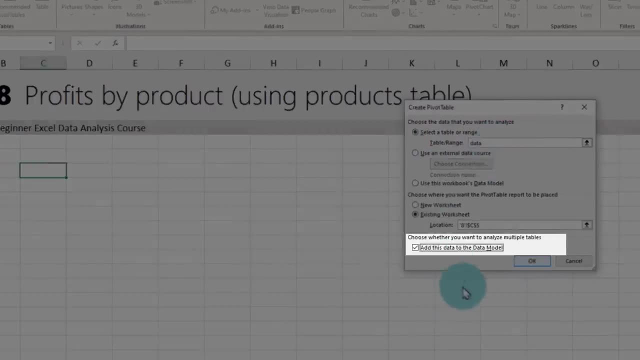 incurred a loss on this particular line. so let's go ahead and now calculate the total profit. so learnt from that data economy of excel itself and then do the analysis. so here i will just say: insert pivot table from my data. this time we need to add this to data model. 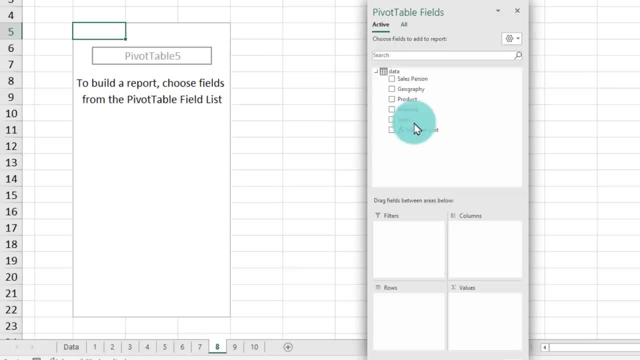 and we will get this nice little thing. you notice that here it doesn't show the cost columns. this is because when you insert a pivot table, if you have already done this a few times in the workbook, excel will not go back to the original data. it will kind of use a stale in memo function for this. 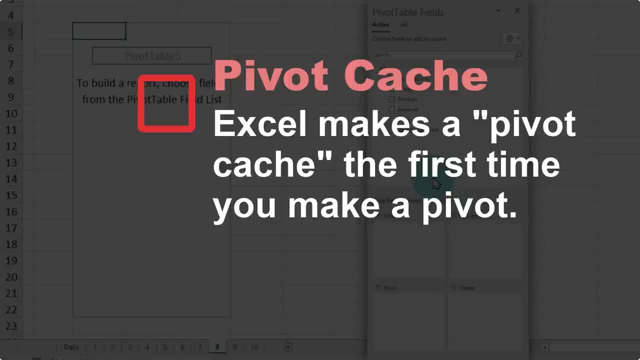 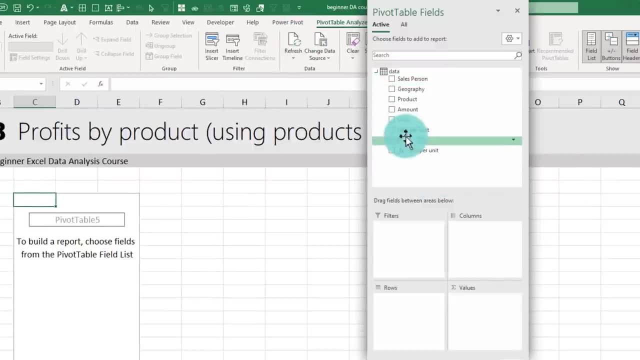 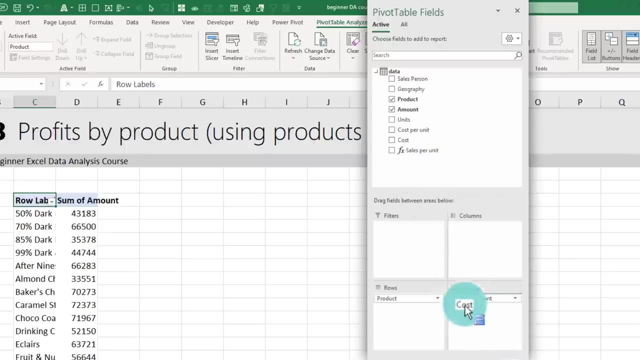 of use a stale in-memory copy of the data to build the pivot table for you. But to force Excel to reconsider all the fields, just hit the refresh and it will bring those additional fields for us. Now let's go and add product here, total amount, and then we will add cost as well. 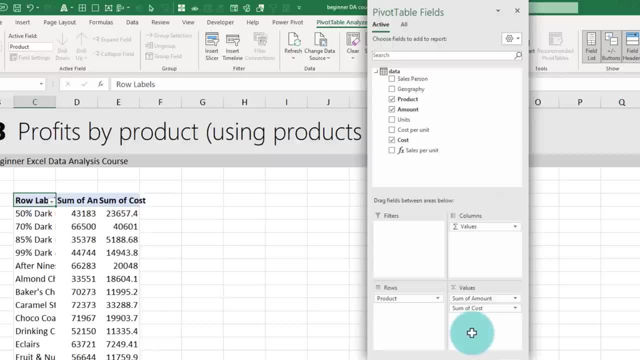 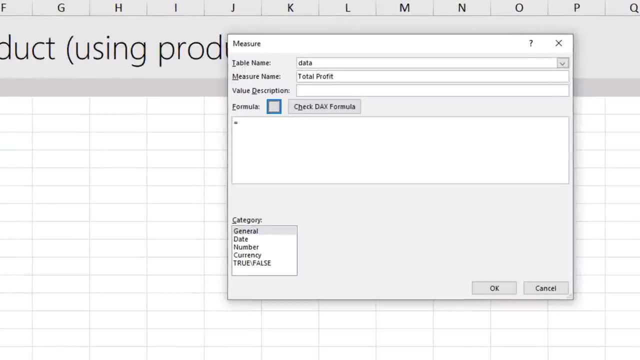 So amount and cost comes up Now. profit would be total amount minus total cost. So we will add that as a measure, add measure total profit And this is nothing but sum of amount minus sum of cost. And we will just say that should be a currency value and add the total. 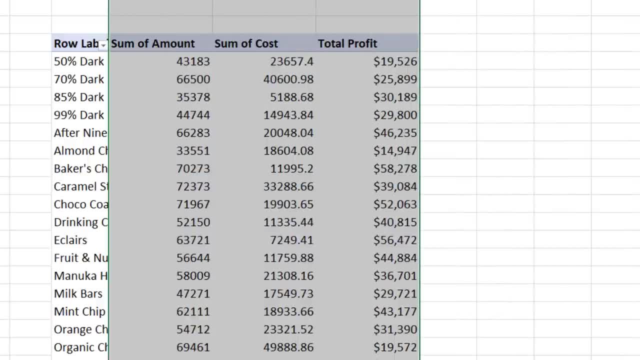 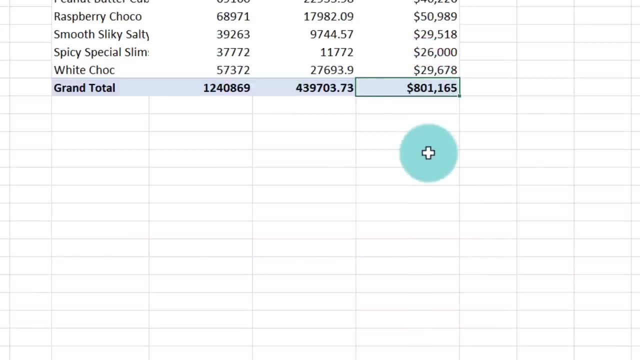 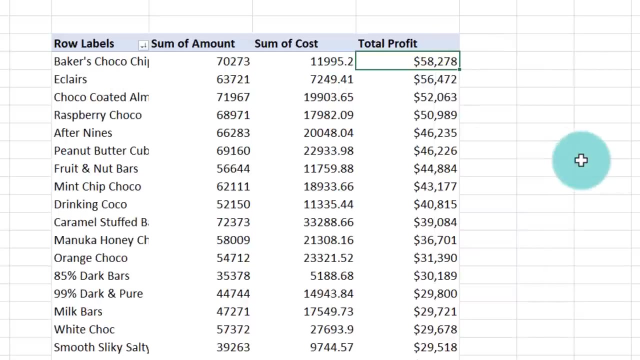 profit as well. So here I'll get a nice little report that shows me, by each of our product, what is the profit we are generating. So we made $800,000 profit total all, And this is how that is. I can apply some sort order on this to look at or most profitable products. 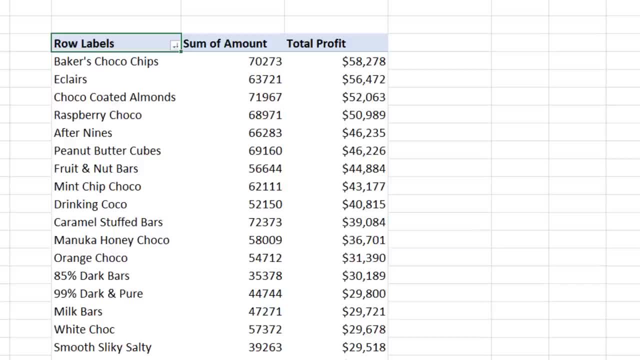 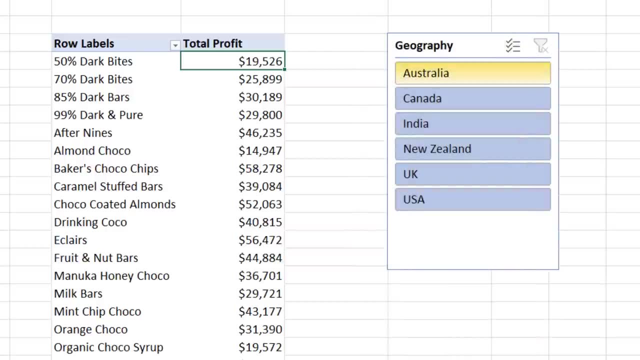 I can also drop these other fields because we're only interested in total profit. I can even add a slicer on a bond. These fields like geography, So I can look at it by India, New Zealand, Australia or all the countries. As you could see, when we go into one of these geographies, you will start to notice. 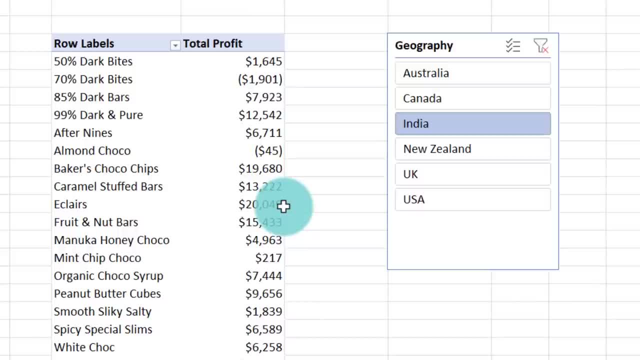 some of these items are making loss in that particular field right now. This isour profit And again we'll add the document at this point So we can also add depth geography, but at a grand total level we're not making loss at. 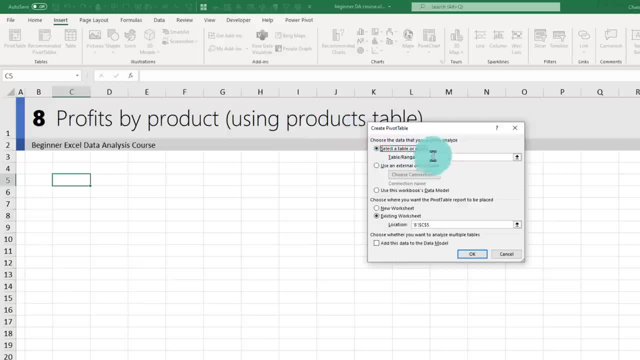 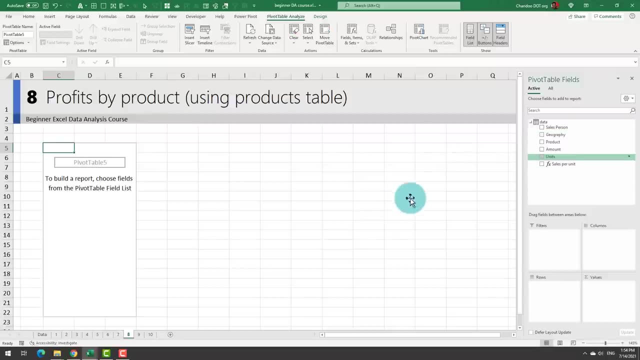 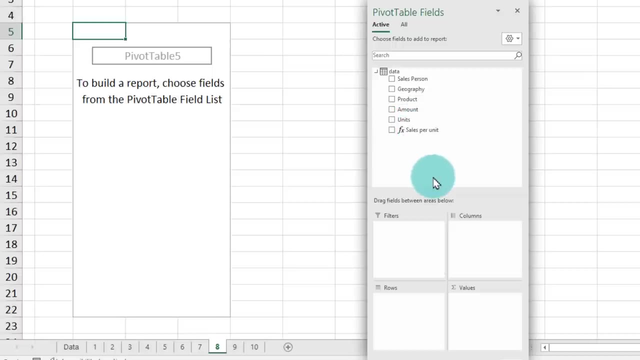 So here I will just say: insert pivot table from my data. This time we need to add this to data model and we will get this nice little thing. You notice that here it doesn't show the cost columns. This is because when you insert a pivot table, if you have already done this a few times, 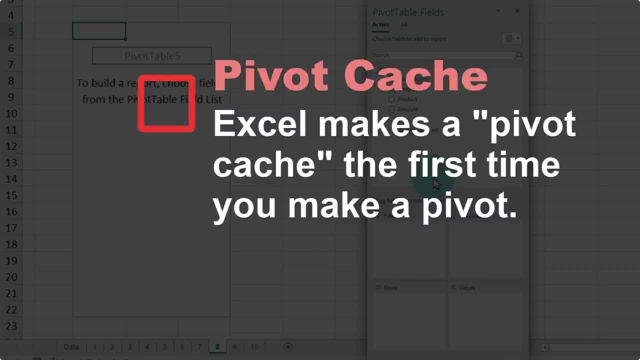 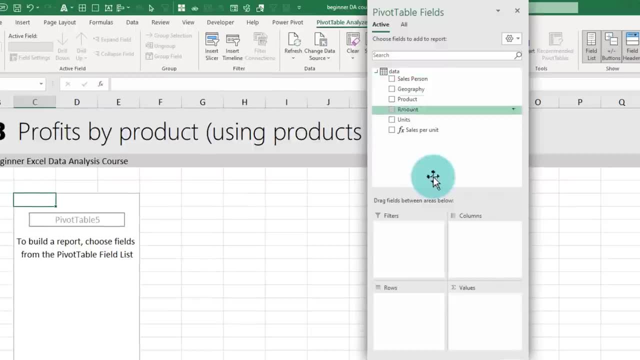 in the workbook. Excel will not go back to the original data. It will kind of use a stale in-memory copy of the data to build the pivot table for you. But to force Excel to reconsider all the fields, just hit the refresh and it will bring those. 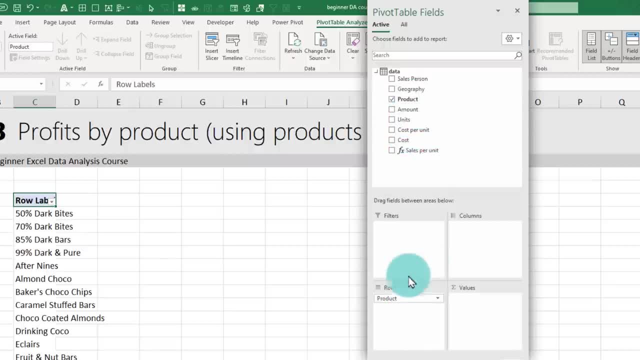 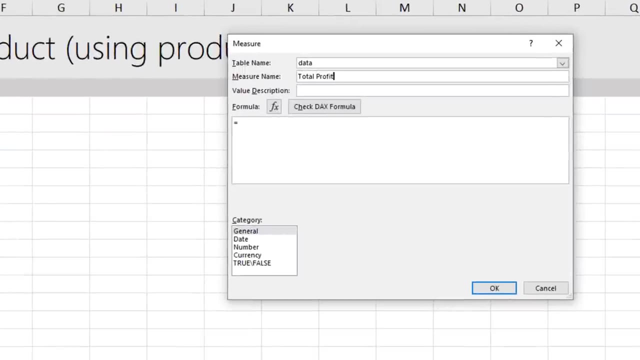 additional fields for us. Now let's go and add product here, total amount, and then we will add cost as well. So amount and cost comes up. The profit would be total amount minus total cost. So we will add that as a measure, add measure, total profit and this is nothing but sum. 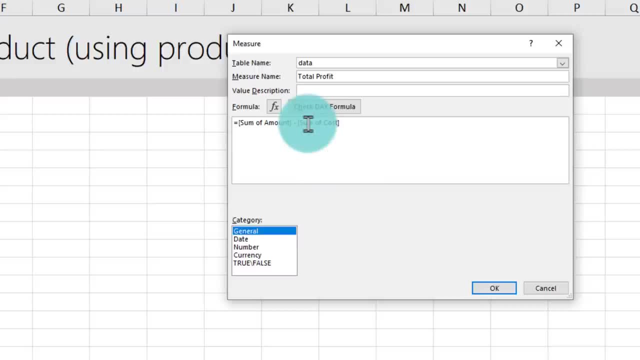 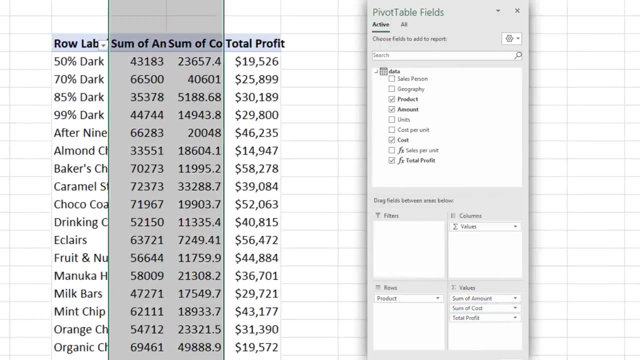 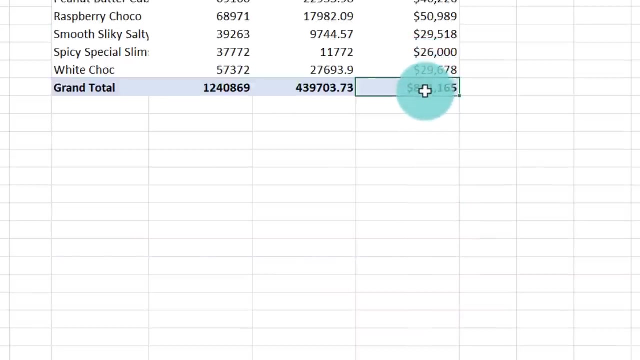 of amount minus sum of cost, And we will just say that should be a currency value and add the total profit as well. So here I'll get a nice little report that shows me, by each of our product, what is the profit we are generating. 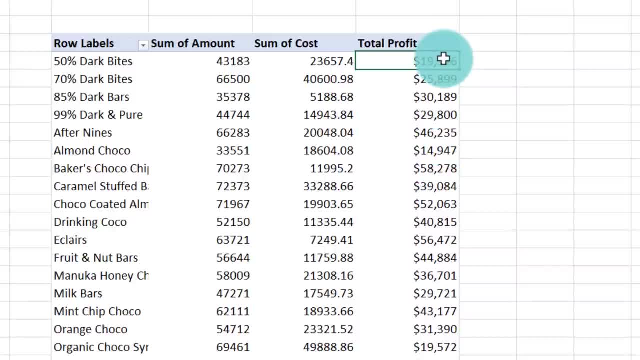 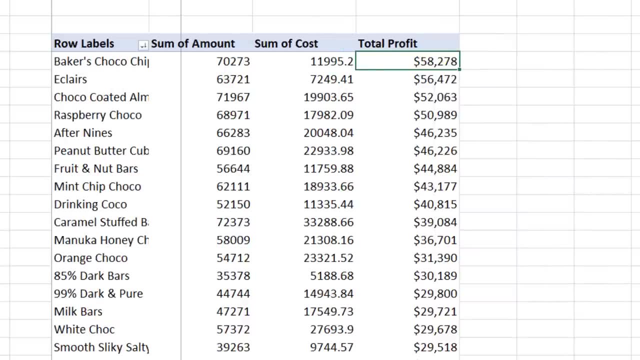 So we made $800,000 profit, total all, and this is how that is spread up. I can apply some sort order on this to look at our most profitable products. I can also drop these other fields because we're only interested in total profit. 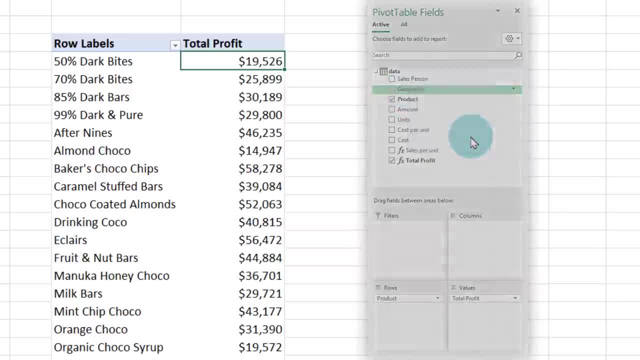 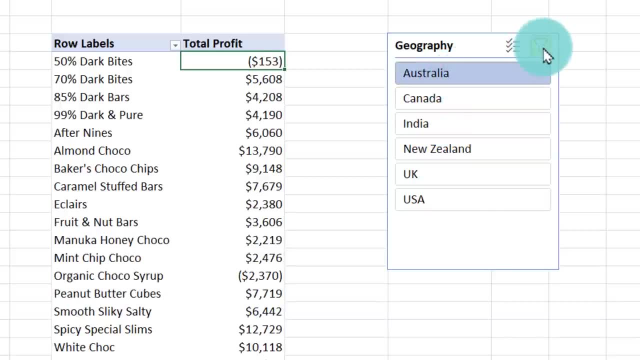 I can also drop these other fields because we're only interested in total profit. We can even add a slicer on one of these fields like geography, So I can look at it by India, New Zealand, Australia or all the countries. As you could see, when we go into one of these geographies, you will start to notice some. 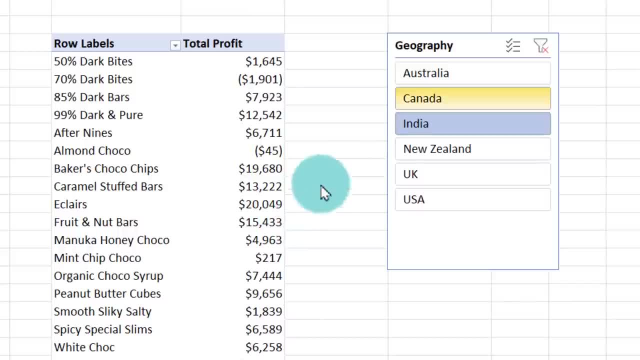 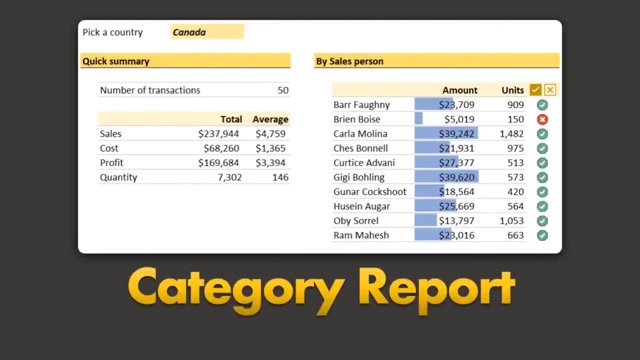 of these items are making loss in that particular geography, but at a grand total level we're not making loss for anything. For this example, we want to create a dynamic country level sales report. The focus here is to present what's happening within the country as a report to you. 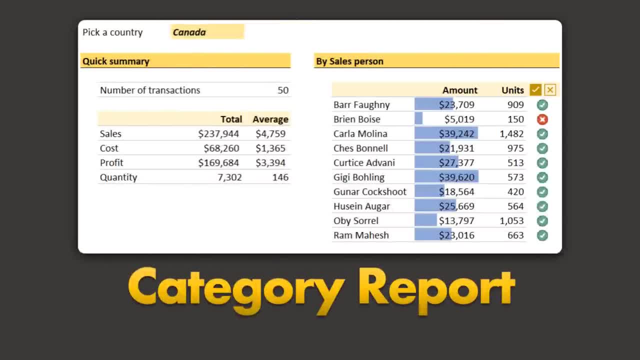 for anything. For this example, we want to create a dynamic country level sales report. The focus here is to present what's happening within the country as a report to you. Unlike the first eight examples, for this one I have chosen a different. 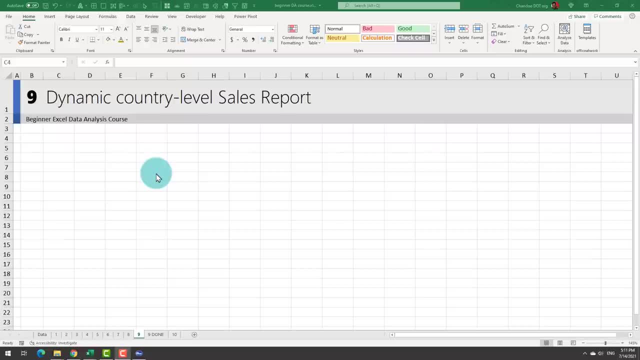 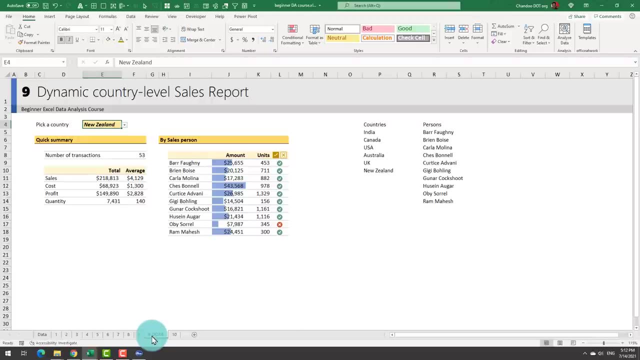 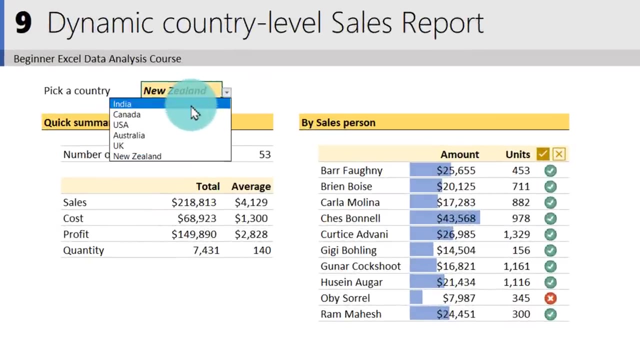 Unlike the first eight examples, for this one I have chosen a different route, where I have already finished the work and I will just walk through the process. but I want you to take this up as a challenge and try to do it yourself. So here I can pick a country, so I can, for example, select India, and then I can immediately. 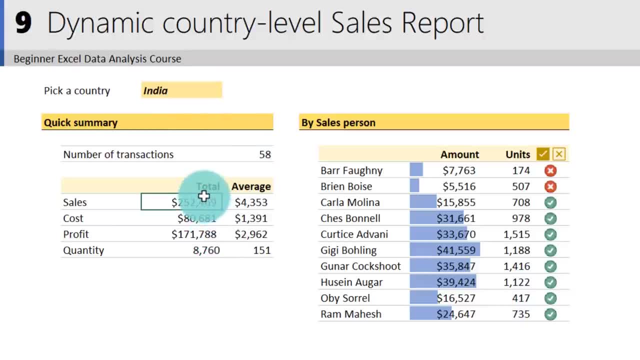 see how many transactions we had within India, What is the total sales Cost Profit, How much is the total quantity and what is the average level, As well as by salesperson, I can see how much amount we have generated, how many units. 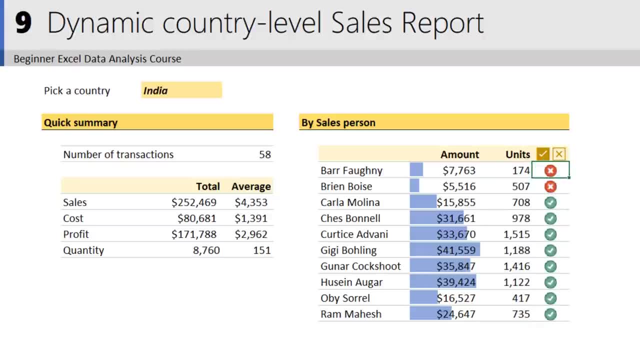 and if the salesperson has met the target of $12,000 within the country. If so, it will show a green tick mark, else a red X mark. So how do we do such a thing Now, before we actually proceed and learn the logic for doing it? 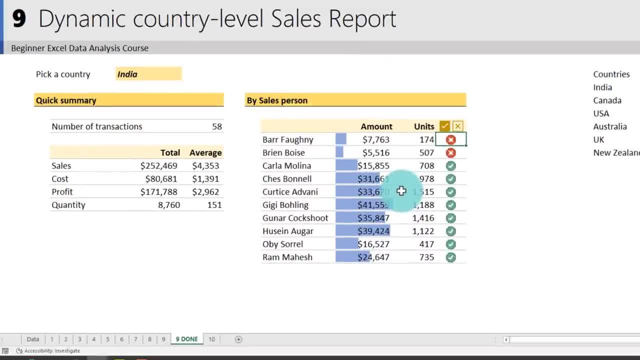 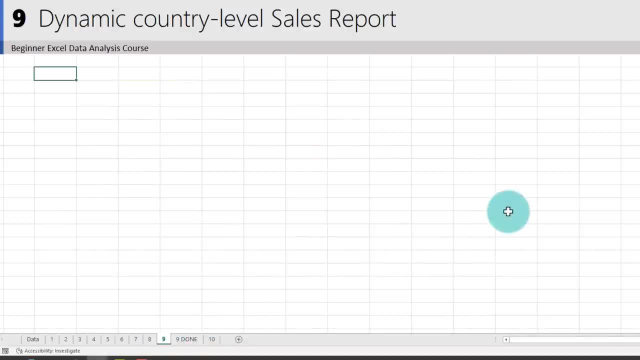 I just want to make a quick note that you would learn a lot more by trying to just take a snapshot of this and use the blank file to recreate it. This way, you will try to connect all the ideas that I have presented so far in the 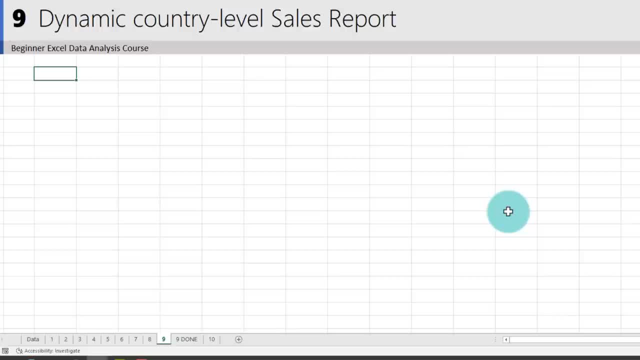 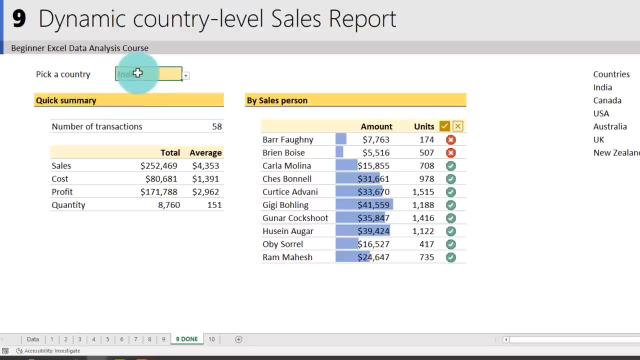 first eight examples and do it better. But if you need some help or you're in a hurry and you just want to know how this is done, Let's see how this works In order to select the country. this kind of thing is called data validation. 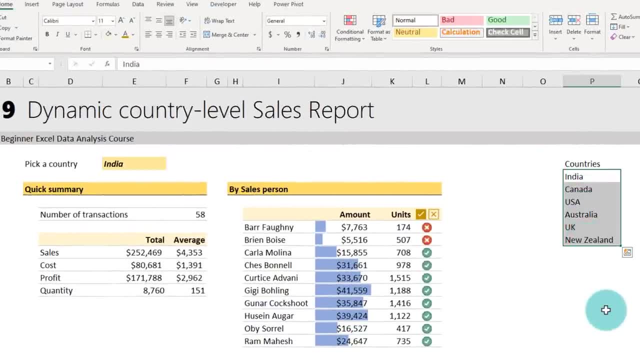 So what we need is we need A list of all the values listed somewhere on the spreadsheet. It doesn't have to be on the same page, It can be in a separate tab as well. So once these values are there, you select the cell, you go to data, click on data validation. 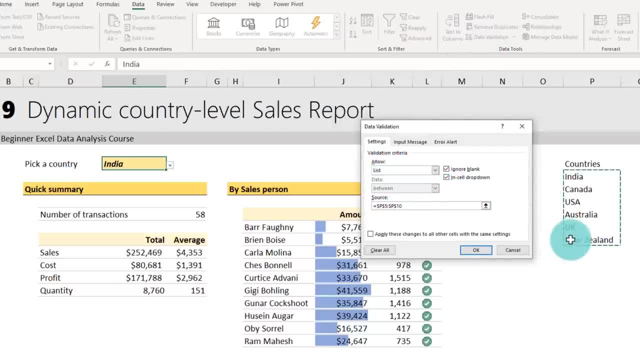 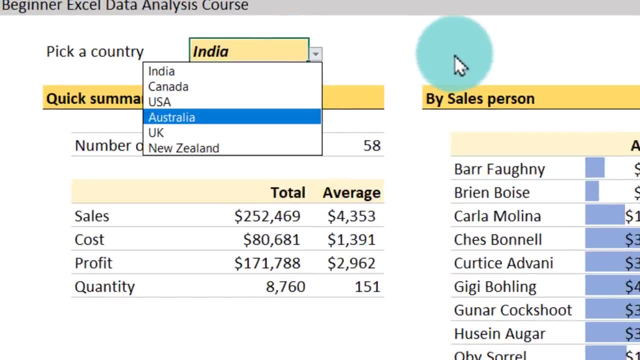 specify a list type of validation and point to the range where your values are. This will now give you a small drop down within the cell from where I can pick a country. So notice this cell: It is E4.. This is where we are selecting the country to see the number of transactions within the 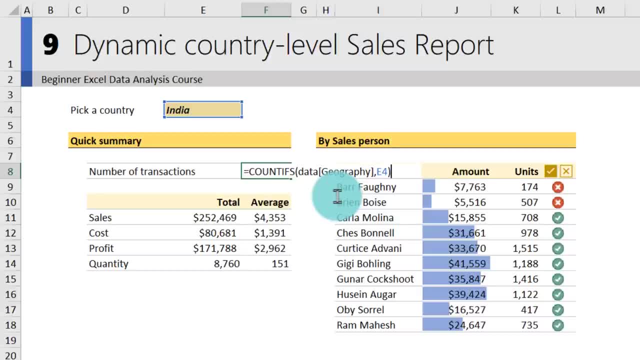 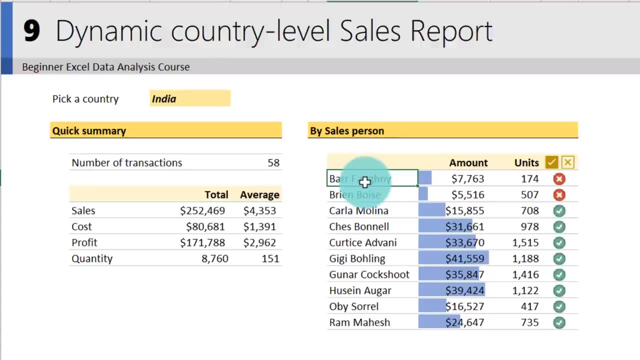 country. We can use the count ifs formula and just count how many times the geography that is in E4 has appeared, And to see totals and averages we simply use some ifs or average ifs formulas. What about this part of the report? Here again, we just need to list all the people. 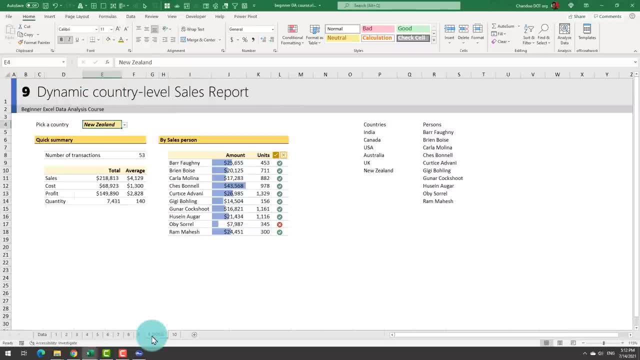 route where I have already finished the work and I will just walk through the process. but I want you to take this up as a challenge and try to do it yourself. So here I can pick a country, So I can, for example, select India, and then I can. 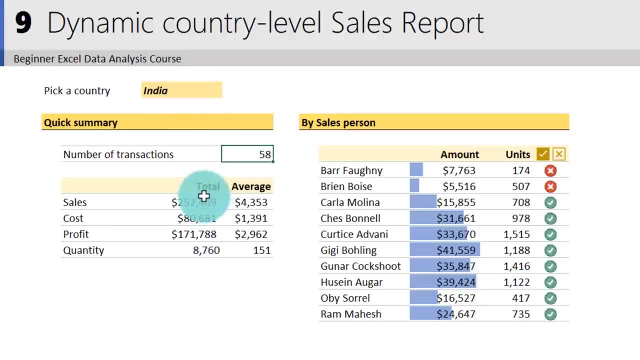 immediately see how many transactions we had within India, what is the total sales cost profit, how much is the total quantity and what is the average level, as well as by salesperson. I can see how much amount we have generated, how many units, and if the salesperson has met the target. 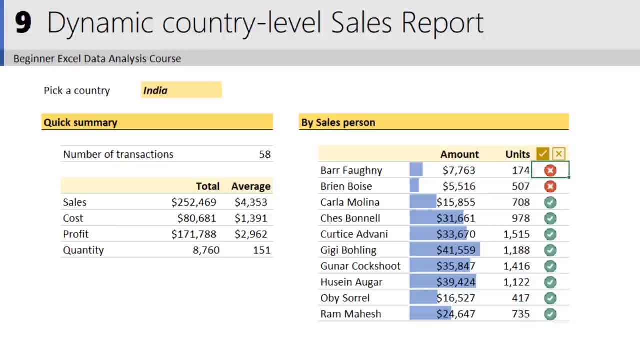 of twelve thousand dollars or within the country. If so, it will show a green tick mark, else a red X mark. So how do we do such a thing? Now? before we actually proceed and learn the logic for doing it, I just 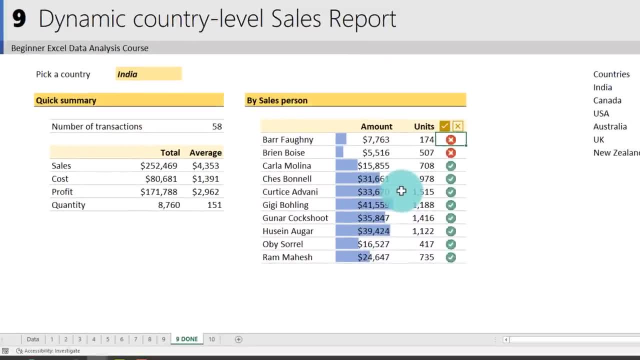 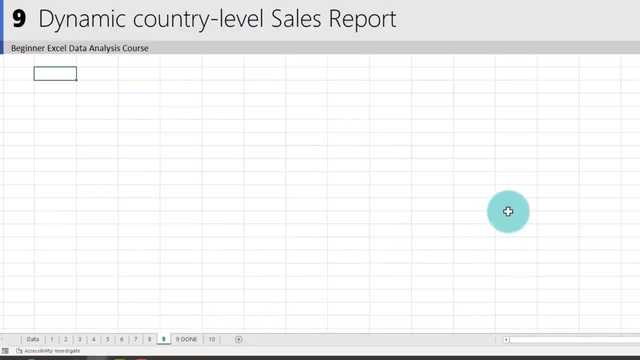 want to make a quick note that you would learn a lot more by trying to just take a snapshot of this and use the blank file to recreate it. This way, you will try to connect all the ideas that I have presented so far in the first eight examples. 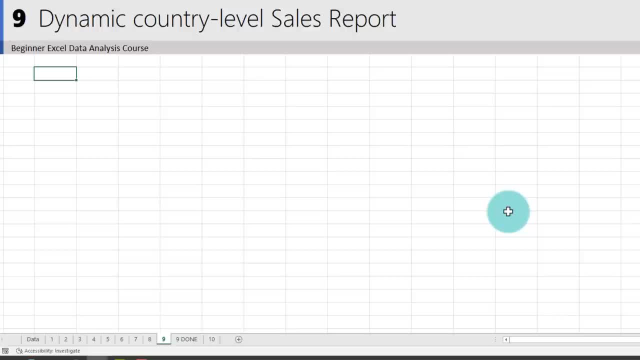 and do it yourself. So let's get started, Let's go ahead and do it better, But if you need some help or you're in a hurry and you just want to know how this is done, let's see how this works In order to select the country this kind of thing is. 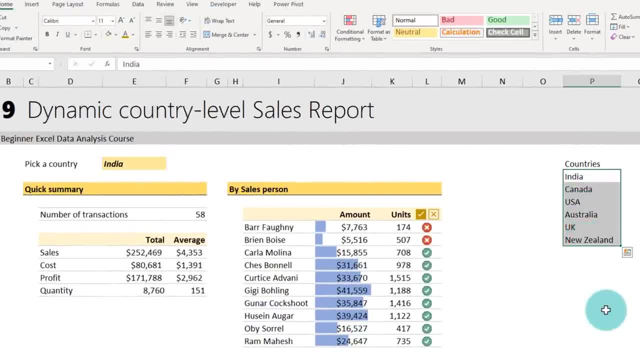 called data validation. So what we need is we need a list of all the values listed somewhere on the spreadsheet. It doesn't have to be on the same page, It can be in a separate tab as well. So once these values are there, you select the cell, you go to data. 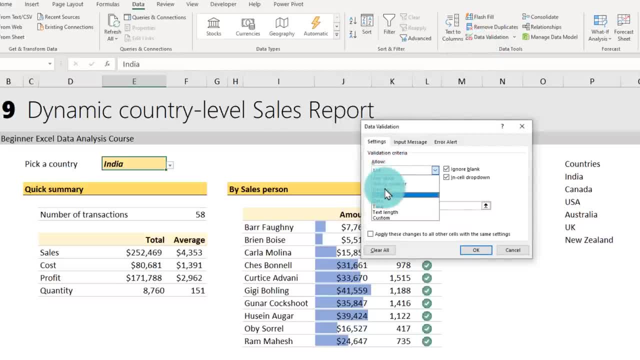 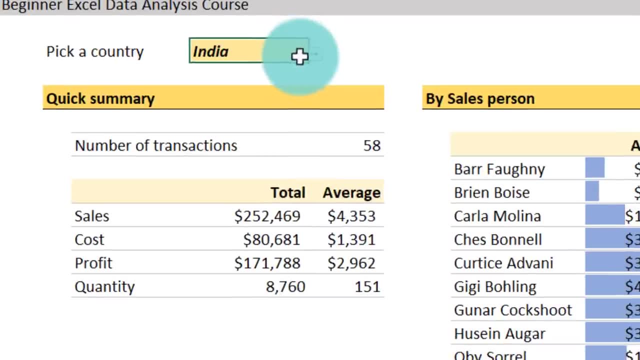 click on data validation, specify a list type of validation and point to the range where your values are. This will now give you a small drop down within the cell from where I can pick a country. So notice this cell. it is E4 where we are. 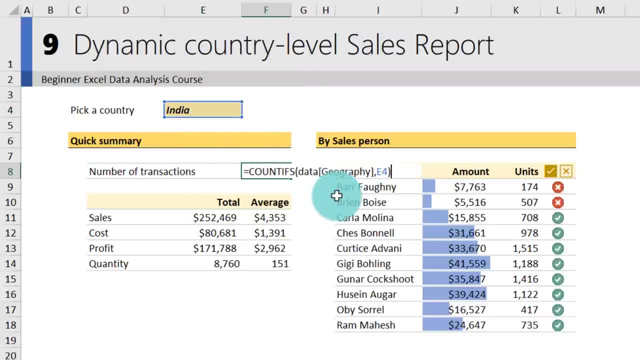 selecting the country. To see the number of transactions within the country, we can use the count ifs formula and just count how many times the geography that is in E4 has appeared. And to see totals and averages we simply use some ifs or average ifs formulas. 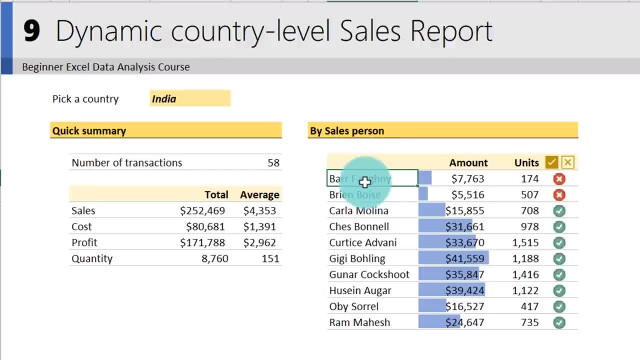 What about this part of the report? Here again, we just need to list all the people. I have listed them in the alphabetical order. We only have 10 people, so I kind of pasted the values here, removed duplicates and sorted And the amount is some. 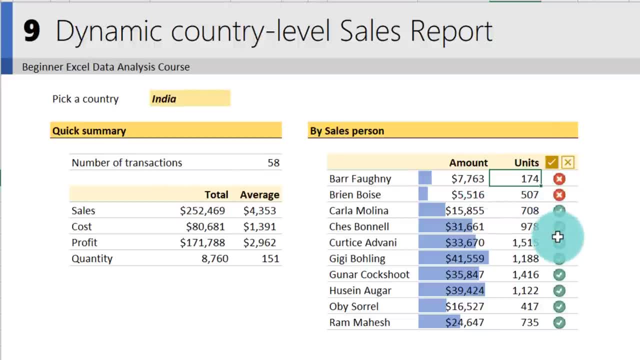 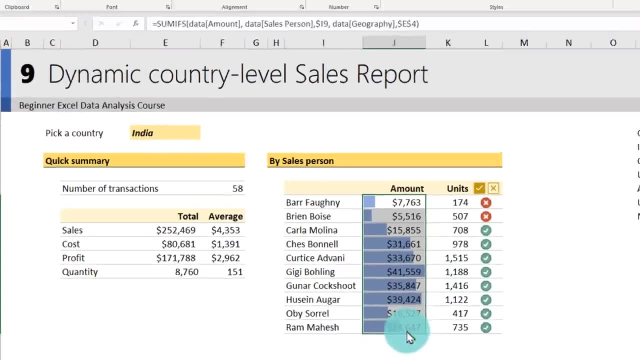 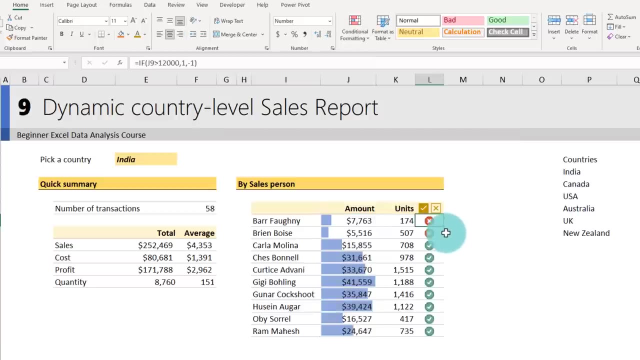 ifs with additional conditions. units is again some ifs on the units column with some extra condition And once these values are here, we just select this, go to home conditional formatting data bar and add a solid data bar. Next, for the check on whether somebody has met the target of 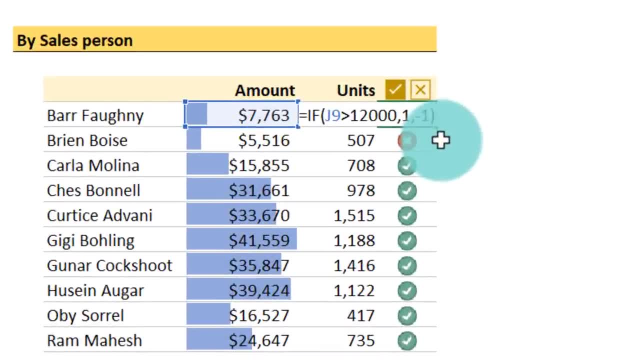 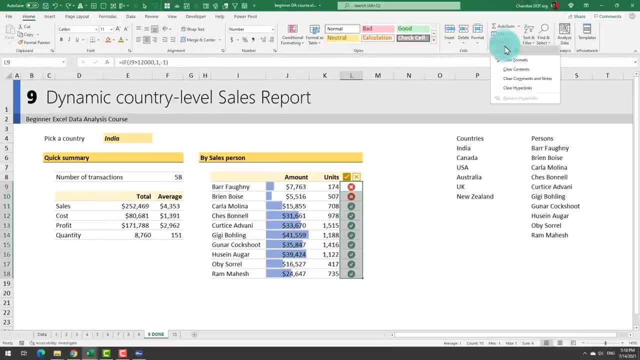 $12,000 or not. I'm using a if formula. If the amount is greater than 12,000, I want one, else I want negative one, And then I select all of these cells. I'm just going to clear the formats. 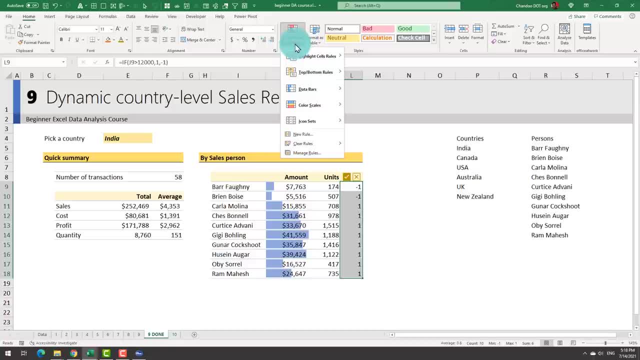 here to show you how the conditional formatting done. So then we go to conditional formatting icon, pick the indicator of this tick mark and X mark And that will give you that We go to manage rules, select and edit, And then we go. 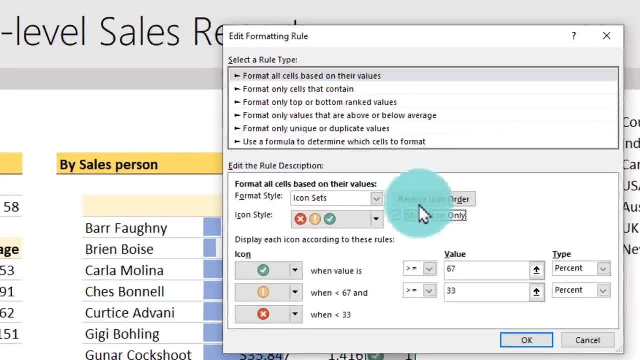 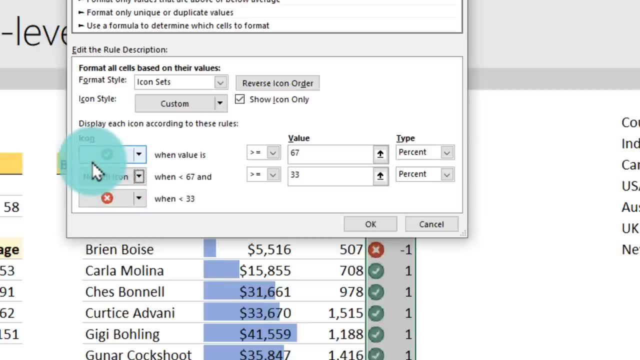 to select and edit the rule And from here enable show icon only because we don't need to see that number And we don't want anything in the middle. So we'll just say this needs to be no cell icon, So we just want green tick and X mark and green. 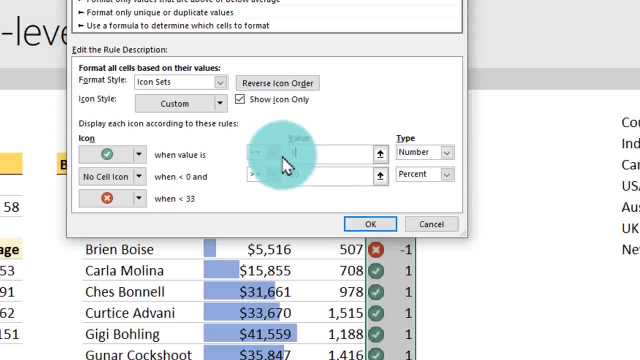 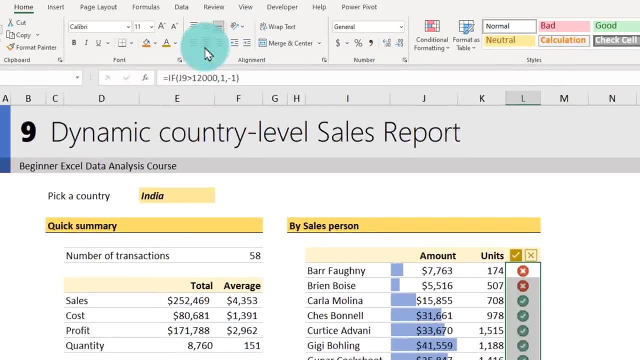 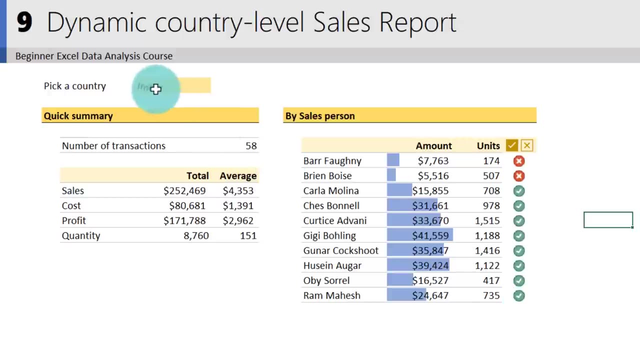 tick when the value is greater than or equal to one, and red one when the value is less than zero. So it is negative one. Set that up and then we can just center align these icons and we'll get this nice little indicators to show what's happening, Because all of these formulas depend on that. 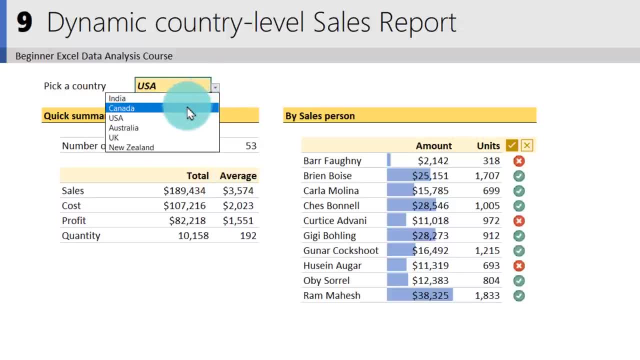 cell Anytime it changes. so I go to USA or I go to Canada, I can see my report by that country. So that is how you can create a dynamic country level sales report. If you are up for more challenge, what I recommend is try to create a completely. 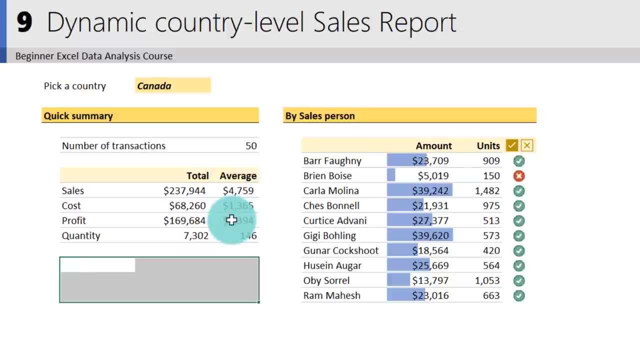 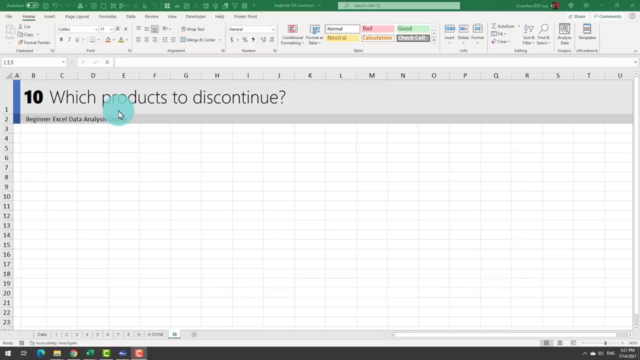 different report that showcases what is happening within the country by some other different criteria or some other different metrics. Take it up as a challenge and again share with me in the comments what you try to do. Now for our 10th example. let's go again with an open ended question: The product. 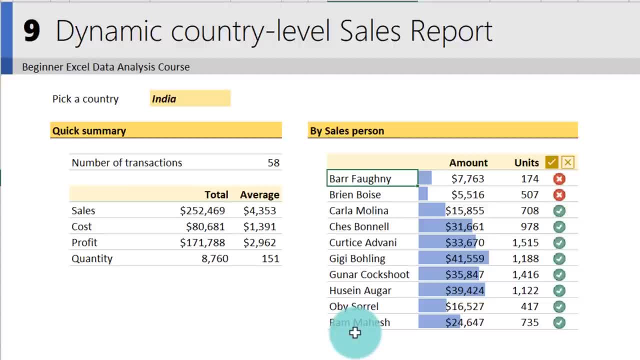 I have listed them in the alphabetical order. We only have 10 people, So I kind of pasted the values here. Remove duplicates Sorted And the amount is some ifs with additional conditions Units is again some ifs on the units column with some extra condition. 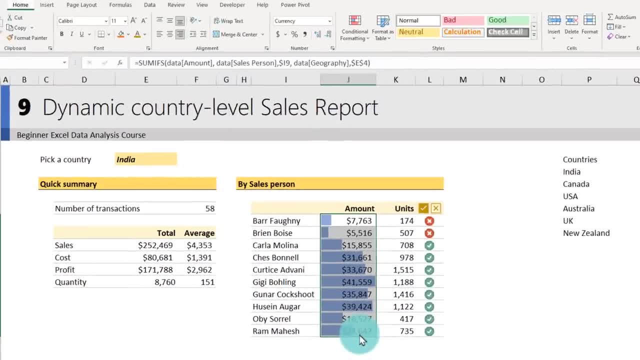 And once these values are here, we just select this, Go to home conditional formatting data bar and add a solid data bar. Next, for the check on whether somebody has met the target of $12,000 or not, I'm using a if formula. 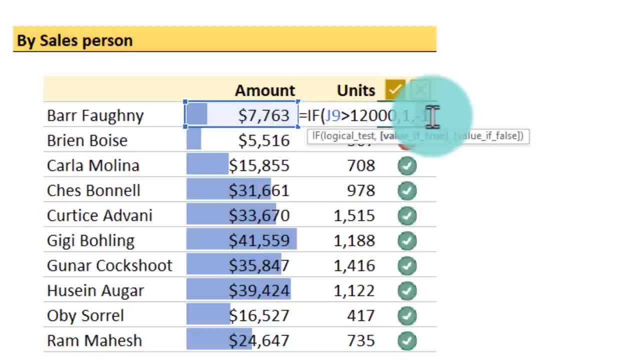 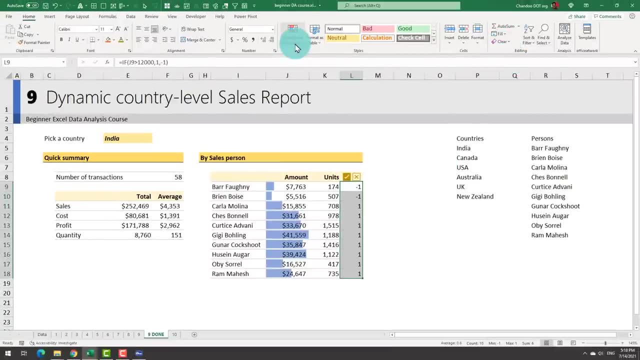 If the amount is greater than 12,000, I want one, else I want negative one, And then I select all of these cells. I'm just going to clear the formats here to show you how the conditional formatting done. So then we go to conditional formatting icon. 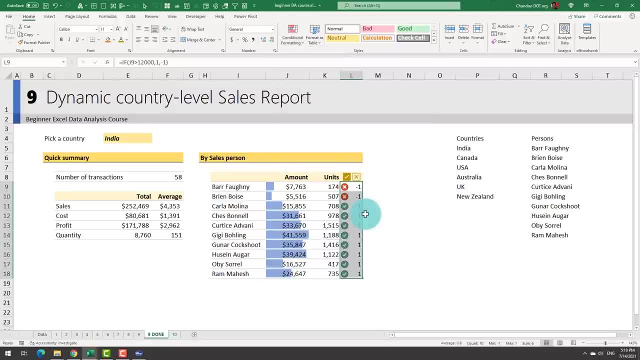 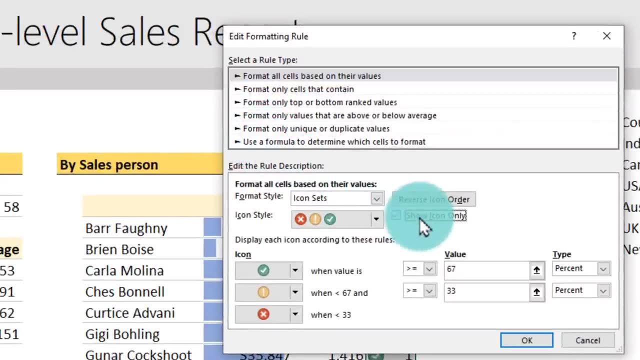 Pick the indicator of this tick mark and X mark and that will give you that. We go to manage rules, select and edit the rule And from here, enable show icon only because we don't need to see that number and we don't. 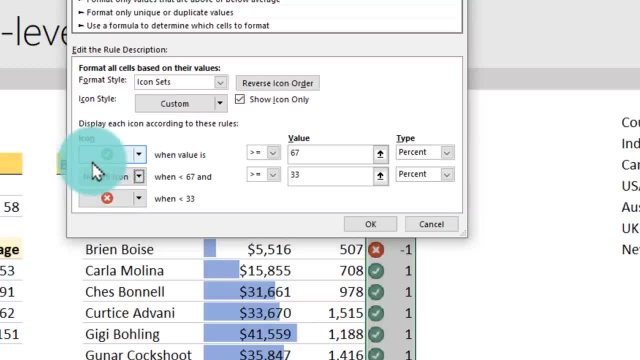 want anything in the middle, So we'll just say this needs to be no cell icon. So we just want green tick and X mark, And green tick when the value is greater than or equal to one and red one when the value is less than zero. 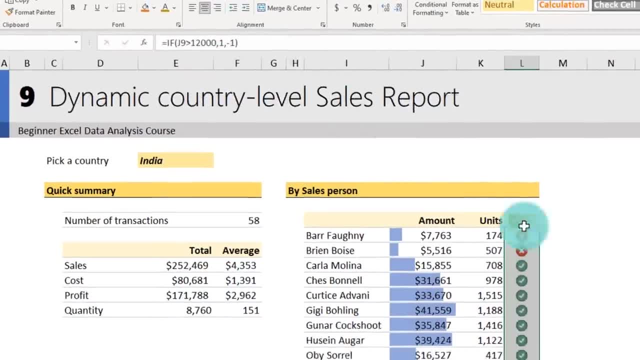 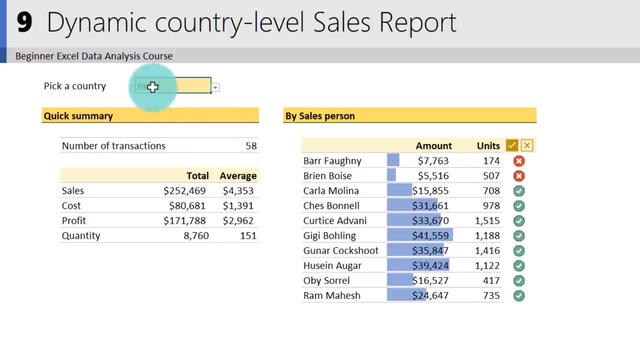 So it is negative one. Set that up and then we can just center align these icons and we'll get this nice little indicators to show what's happening, Because all of these formulas depend on that cell anytime it changes. so I go to USA or 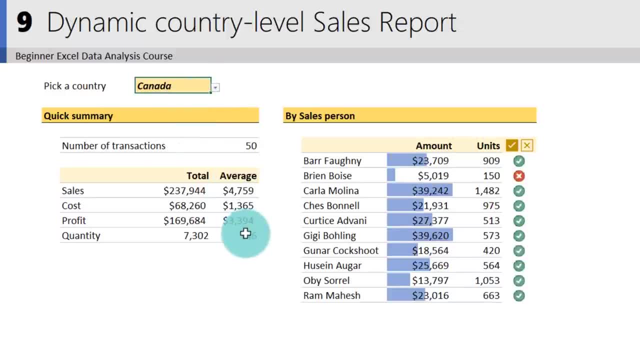 I go to Canada, I can see my report by that country. So that is how you can create a dynamic country level sales report. If you are up for more challenge, what I recommend is try to create a completely different report that showcases what is happening within the country by some other, different criteria or 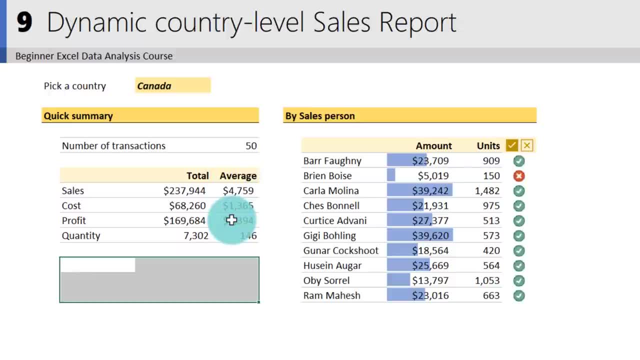 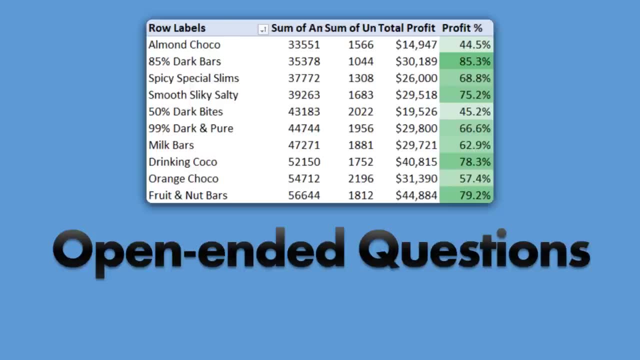 some other different metrics. Take it up as a challenge and again share with me in the comments what you're trying to do. Now for our 10th example, let's go again with an open ended question. the product manager of awesome chocolates. 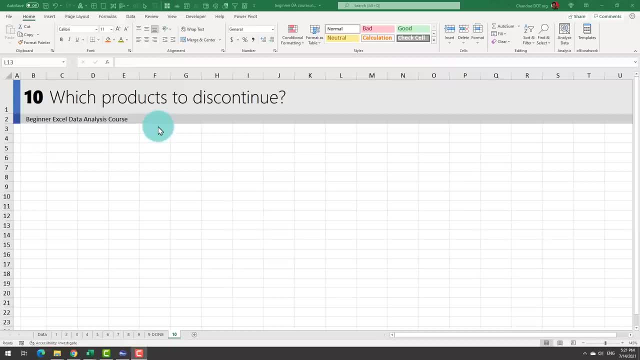 manager of Awesome Chocolates asked you which products to discontinue. She wants to know, among all the 20 odd products that we sell, if there are some really dull ones that we should probably discontinue or use that effort to work on something else. When you get a question like this, it can be fairly. 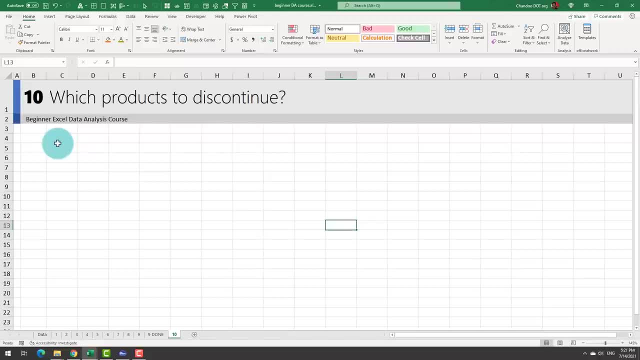 daunting to figure out how to answer it, But if you have a question you can answer it. So we will try doing it in a few different ways so that you can form some arguments and then you can go and see that result. So let's start off by asking the 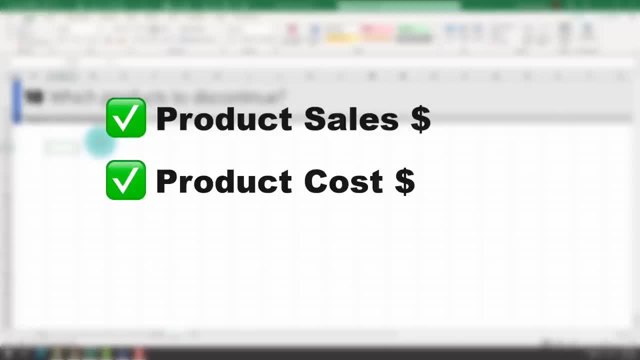 question on how much money we are bringing in for each of these products, How much is the cost that we are incurring, What is the number of units we are selling and what is the total profit we are making. And we will use all these four numbers. 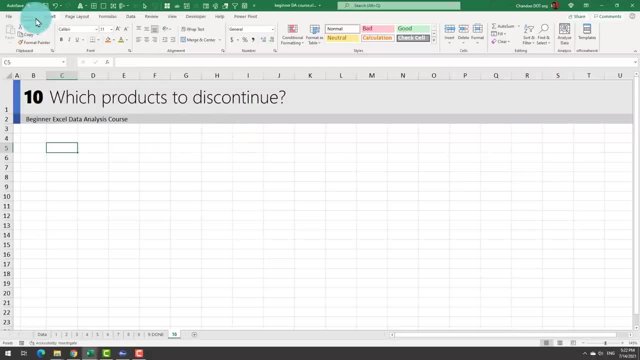 to make our decision on whether to discontinue a product or not. We will do this in any number of ways, but I'm going to use pivot table because this will give you a little more flexibility to quickly do something If you're not happy. 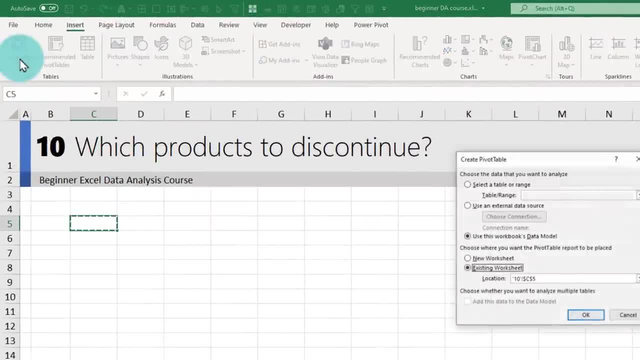 you can kind of switch back and do something else with the data. So we'll do a pivot table on the data and we will use the data model so that we can capitalize on our profit measures and other things. So we'll create this and I'm just gonna put my product. 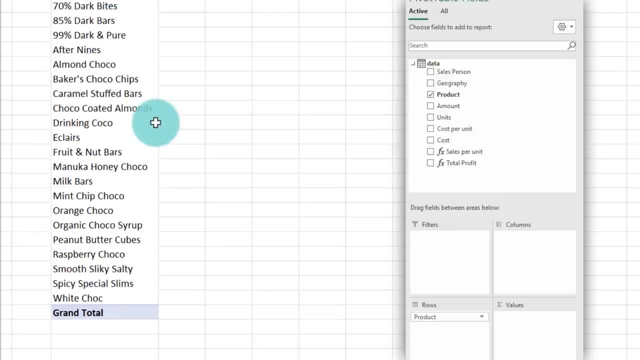 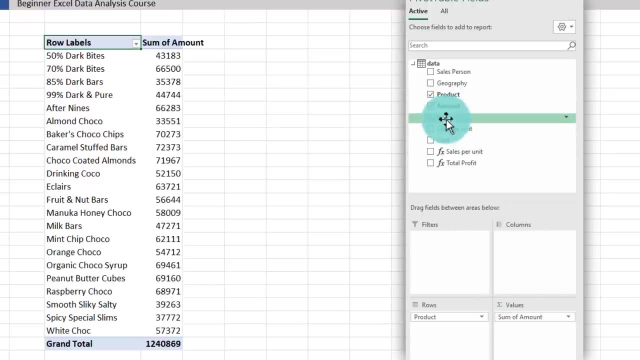 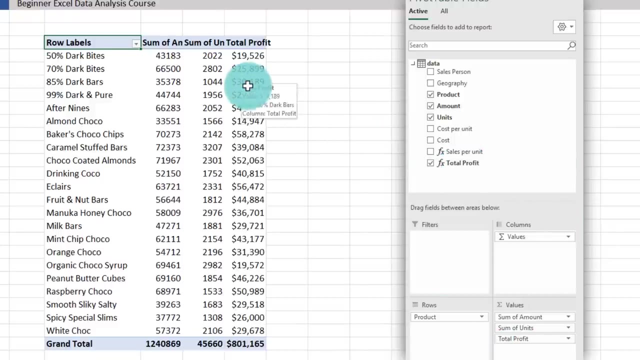 here. This will list one row per product, so we can see that all that products are there, and for each of these products I want to see total amount, total units and then total profit. Let's start by asking the question of which are our least selling products? 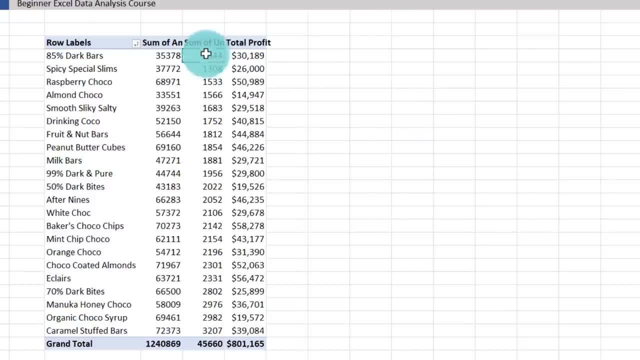 So we can go and sort this from smallest to largest. you can see that 85% dark bars is one of our least selling products and we only sell 1000 units of that. But you can see that it does have fairly high profit amounts of $30,000 profit out of $35,000. 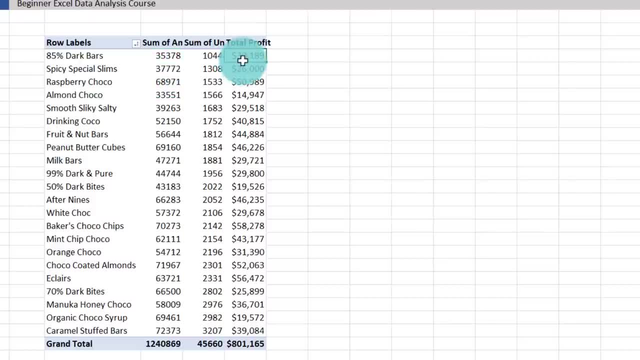 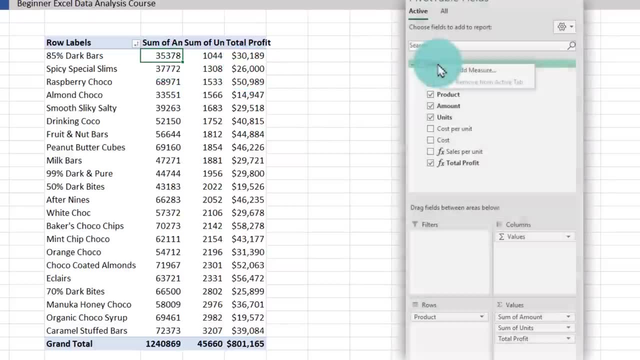 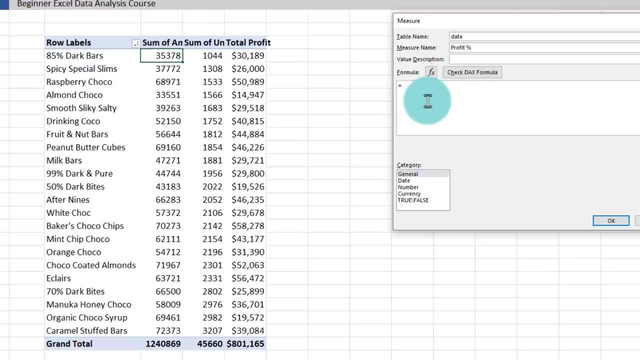 sales. So the profit is fairly high. But because we are kind of comparing different numbers, looking at these alone is hard, So I'm going to add a new measure. right click add measure. This is my profit percent. This will make it easy for us to compare one with another at an absolute level. 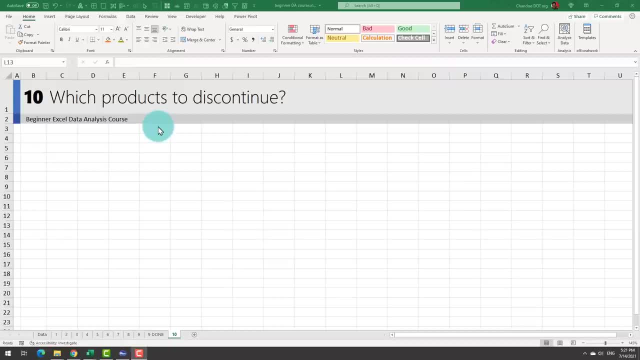 Ask a deal which products to discontinue. She wants to know, among all the 20 odd products that we sell, if there are some really dull ones that we should probably discontinue or use that effort to work on something else. When you get a question like this, it can be fairly daunting to figure out. 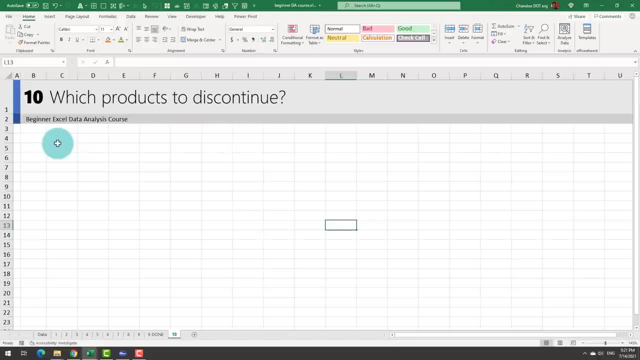 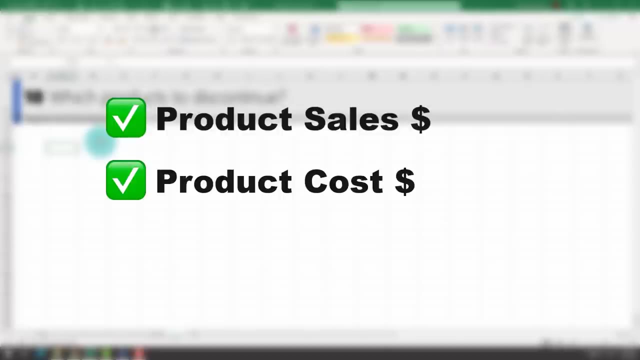 how to answer it. So we will try doing it in a few different ways so that you can form some arguments and then you can go and see that result. So let's start off by asking the question on how much money we are bringing in for each of these products. How much is the cost that we 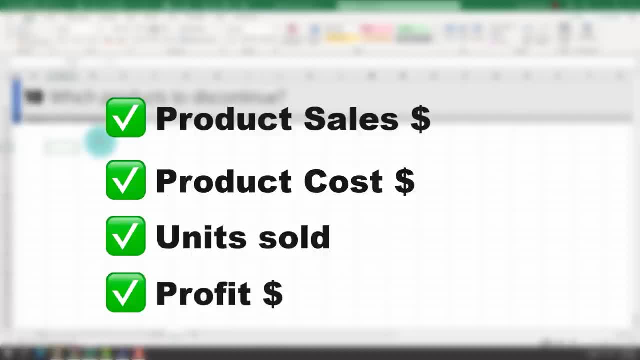 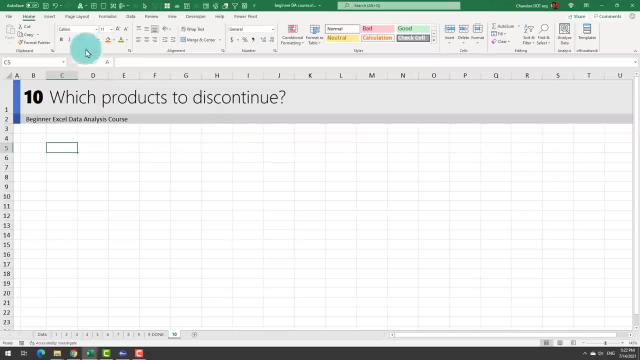 are incurring, What is the number of units we are selling And what is the total profit we are making, And we will use all these four numbers to make our decision on whether to discontinue a product or not. We could do this in any number of ways, but I'm going to use pivot table. 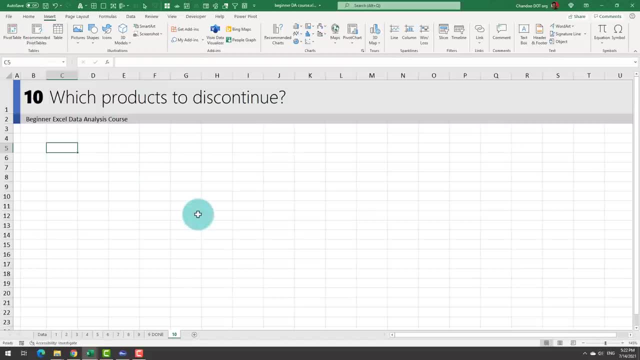 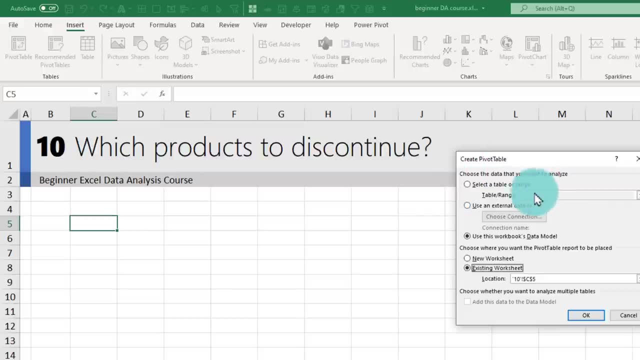 because this will give you a little more flexibility to quickly do something. If you're not happy, you can kind of switch back and do something else with the data. So we'll do a pivot table On the data And we will use the data model so that we can capitalize on our profit measures. 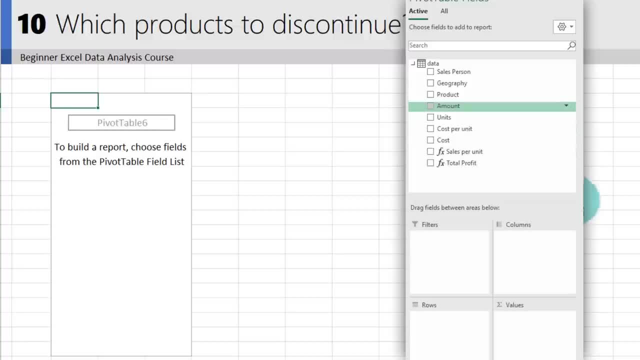 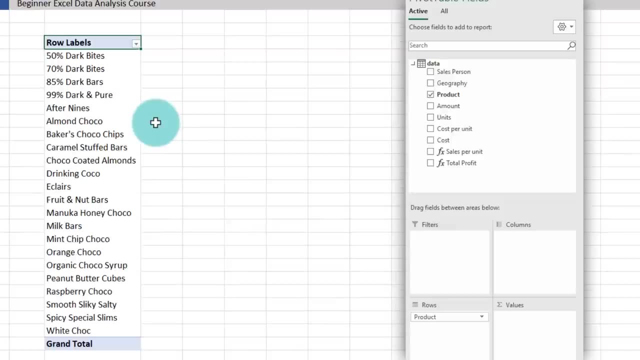 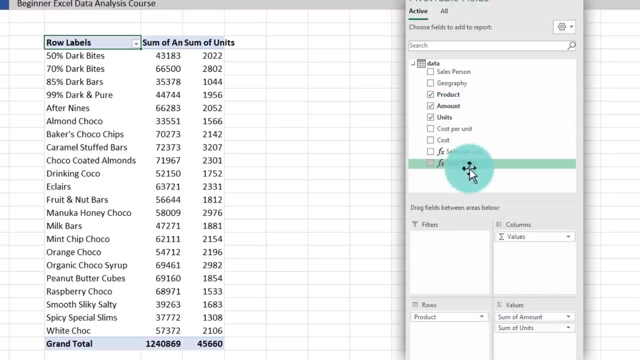 and other things. So we'll create this and I'm just going to put my product here. This will list one row per product, So we can see that all the 22 products are there, And for each of these products I want to see total amount, total units and then total profit. Let's start by 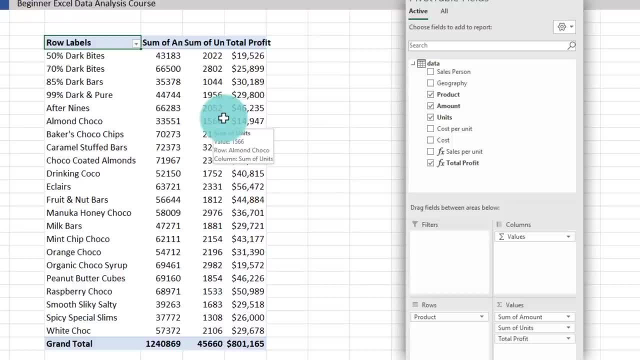 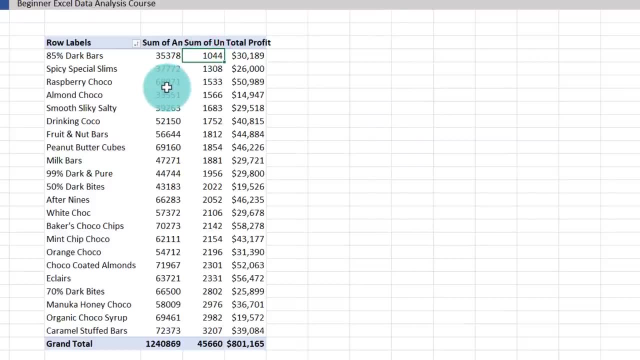 asking the question on how much money we are bringing in for each of these products. How much money we are bringing in for each of these products, So we can go and sort this from smallest to largest. You can see that 85% dark bars is one of our least selling products. 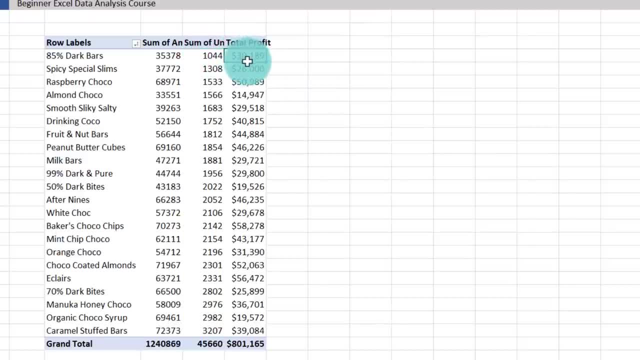 And we only sell 1000 units of that. But you can see that it does have fairly high profit amounts: a $30,000 profit out of $35,000 sales. So the profit is fairly high. But because we are kind of comparing different numbers looking at each of these products, we are 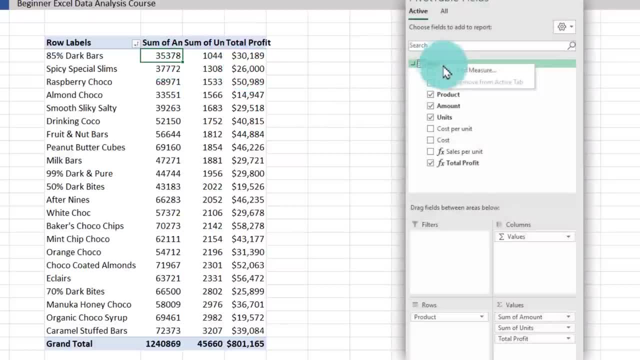 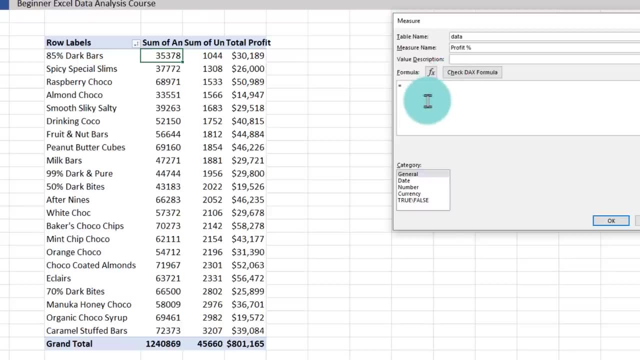 looking at these alone is hard, So I'm going to add a new measure. right click add measure. This is my profit percent. This will make it easy for us to compare one with another at an absolute level. This is nothing but taking my total profit and divide that with 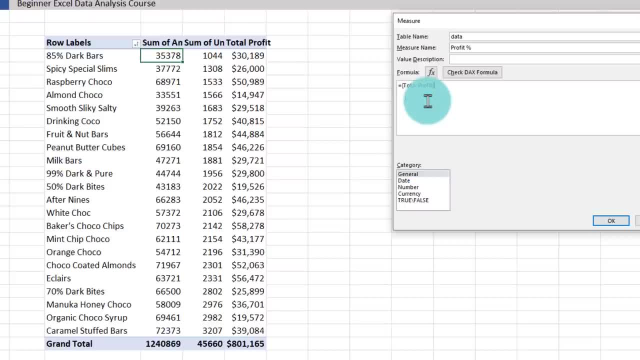 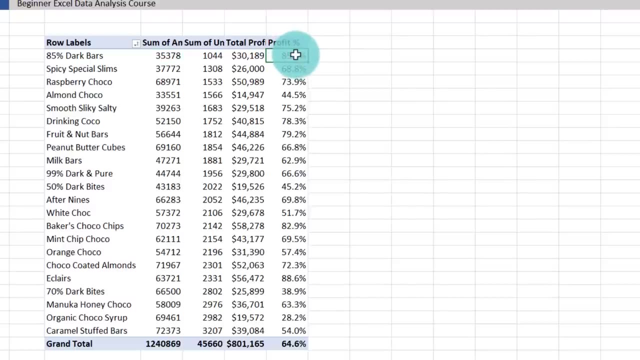 This is nothing but taking my total profit and divide that That with sum of amount, and we will just set this as a number percentage, one decimal point. Let's add that and you can clearly see that this has 85% profit. So if you want to cut this particular product, you would be really giving up one of your. 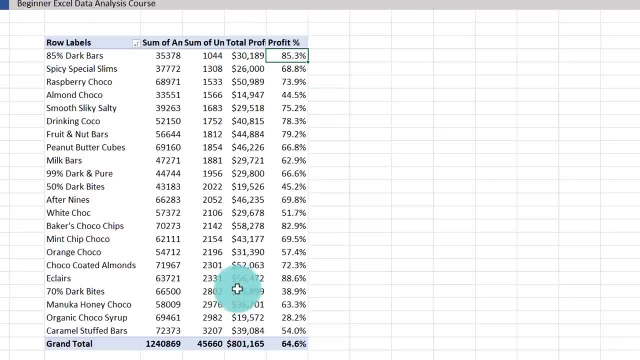 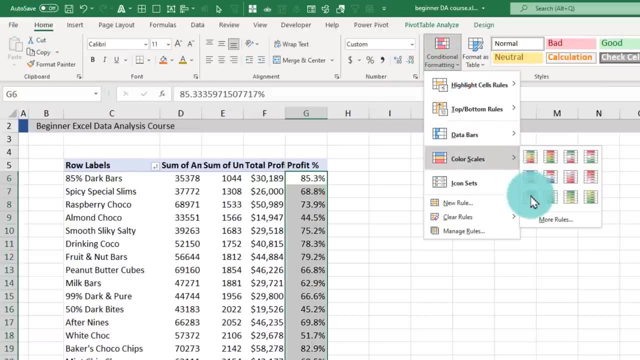 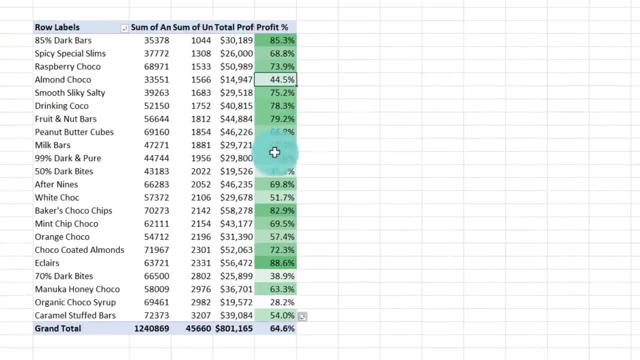 highly profitable products. You can again double check. We only have 22, so we can eyeball and see. But if you have hundreds of products, you can select all of this, go to home. conditional formatting and quickly A color scale to see that you know this one is fairly green, whereas one of these 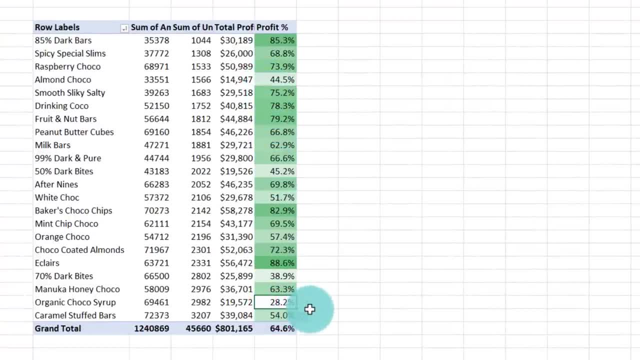 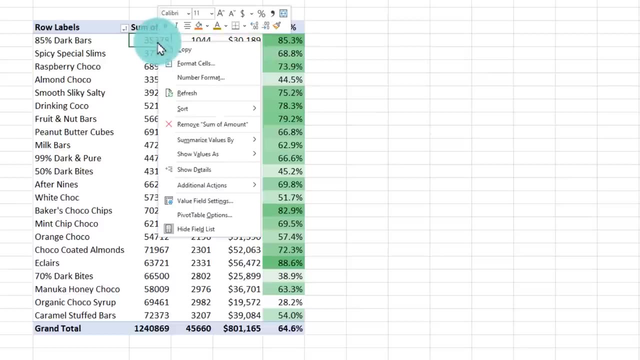 would be a better choice. like this, one has only 28% profit, So probably that's a good way to kind of let go. So this gives you an indication of what to do now. because number of units is not a good indicator, Maybe let's go and sort this by amount. 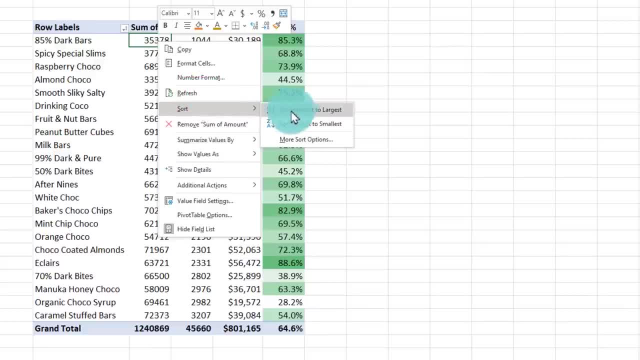 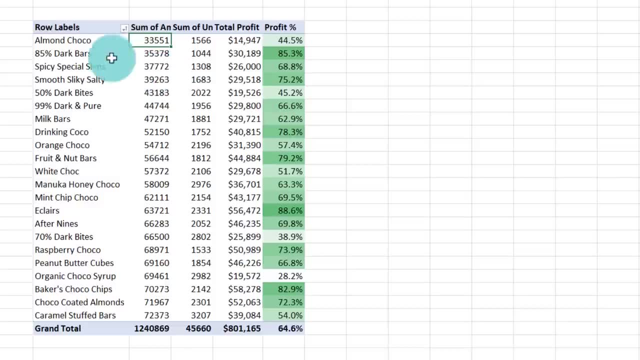 So we'll see which ones are actually bringing in least amount for us. So we'll go smallest to largest. You can see that Almond Choco is one of the smallest products that we sell in terms of revenue And it also happens to have not not a very great profit percentage- 44%- in contrast with 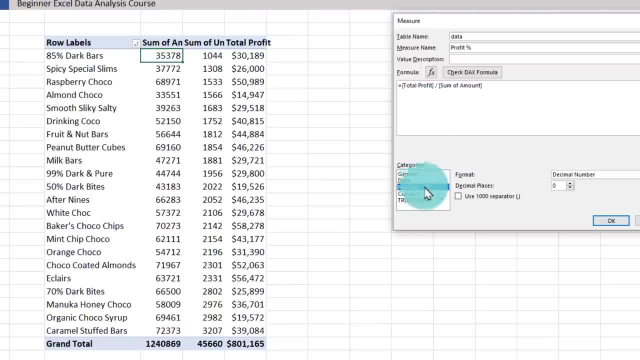 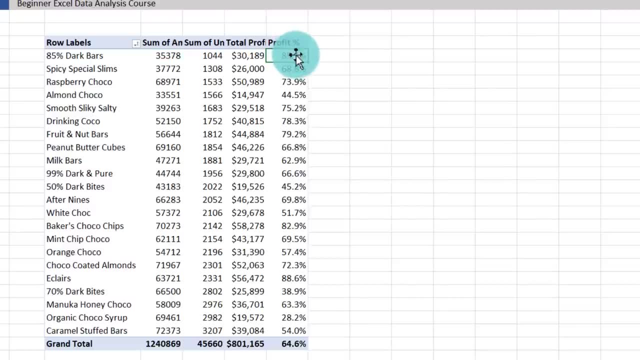 sum of amount, And we will just set this as a number, percentage, one decimal point. Let's add that And you can clearly see that this has 85% profit. So if you were to cut this particular product, you would be really giving up one of your highly profitable products. 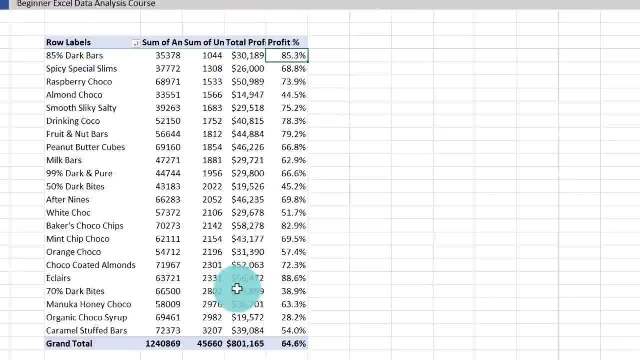 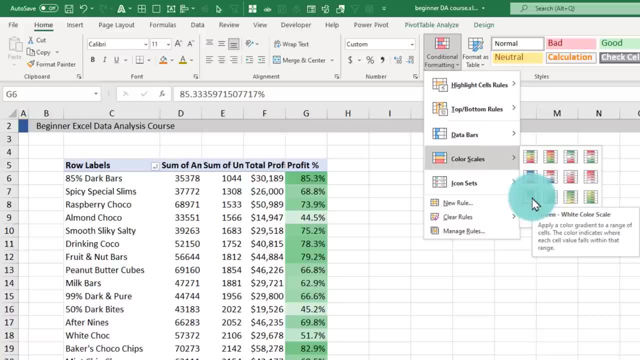 You can again double check. we only have 22. So we can eyeball and see. But if you have hundreds of products, you can select all of this, go to home conditional formatting and quickly put a color scale to see that you know. this one is fairly green, whereas one 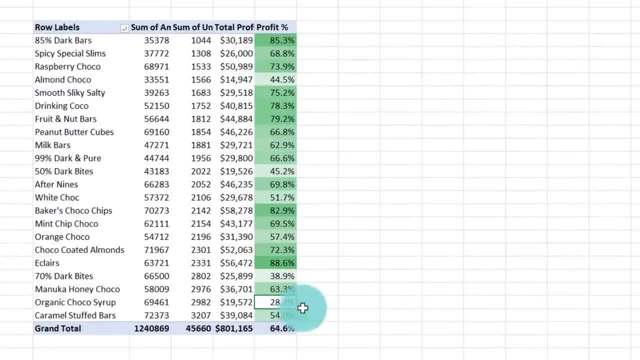 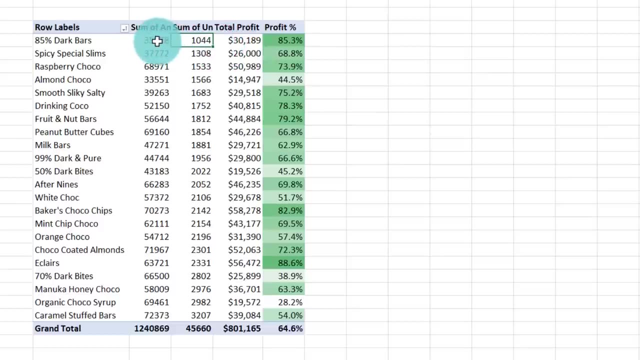 of these would be a better choice. like this, one has only 28% profit, So probably that's a good way to kind of let go. So this gives you an indication of what to do Now, because number of units is not a good indicator, Maybe let's go and sort this by amount So we'll see which ones are actually. 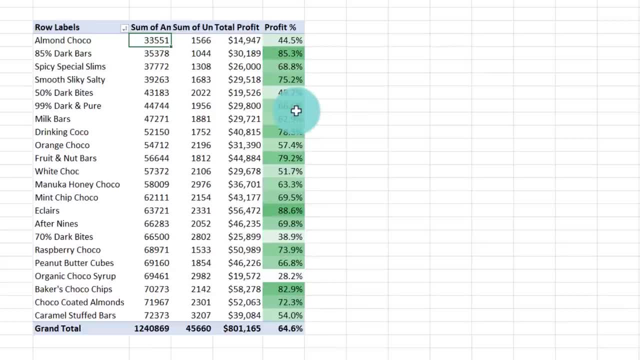 bringing in least amount for us. So we'll go smallest to largest, And you can see that almond Choco is one of the smallest products that we sell in terms of revenue And it also happens to have not not a very great profit percentage: 44%. 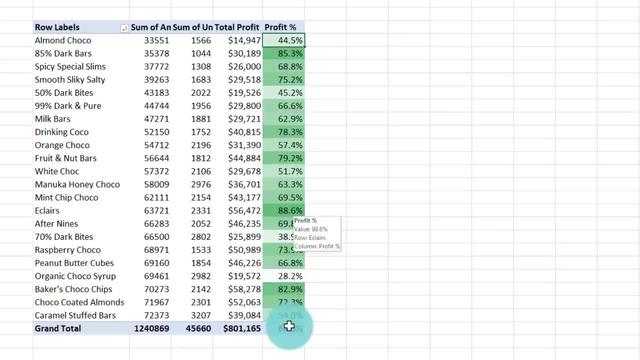 In contrast with some of these very high numbers in 60s and 80. So if I want to drop this one, we are not gonna really, you know, take a huge hit on our bottom line or top line and we will still be fairly good. So this is one of the products that we can definitely drop. 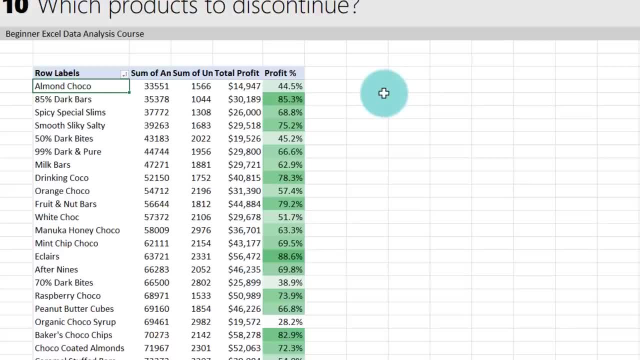 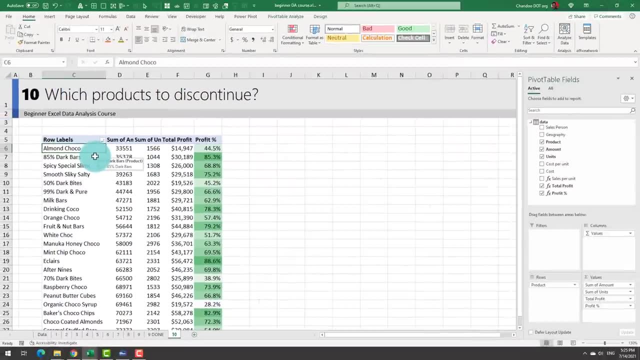 based on our criteria of looking at amounts and looking at total units and total profit percentage. But if you want to take this to the next level, we could then say wait a sec, maybe we can discontinue the products by geographies To add that layer of detail. 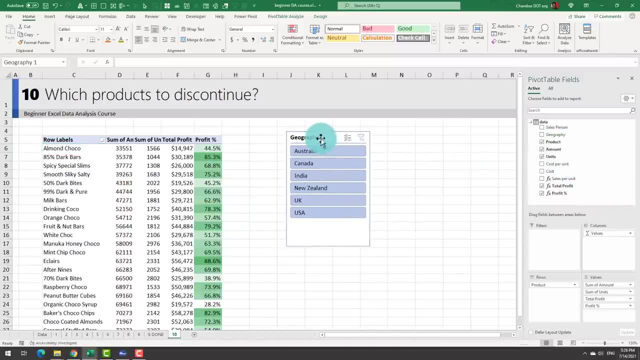 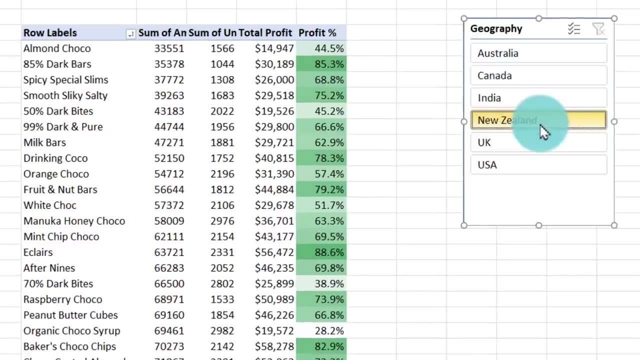 you can add a slicer on on the country And then you can pick the country where you want to, for example, test your discontinuation process. So let's go with New Zealand. Within New Zealand, you can see that almond Choco is actually one of our loss making products. 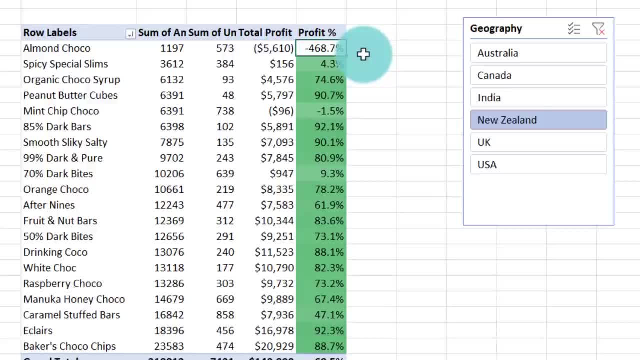 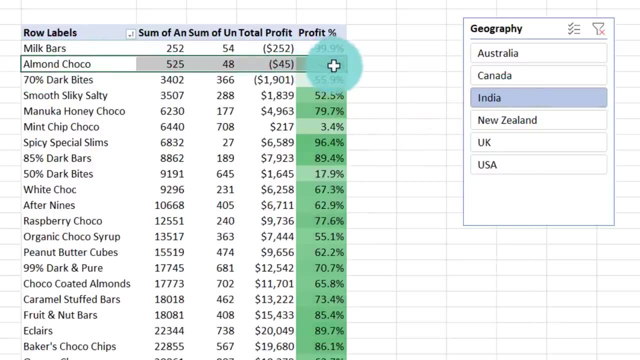 It is giving you negative 468% loss. So this is not good right? This is this again. Reeky confirms our belief that almond choco is probably the one to drop. let's see what is happening within india. within india, almond choco again ranks fairly high. it is making loss, but it we have also. 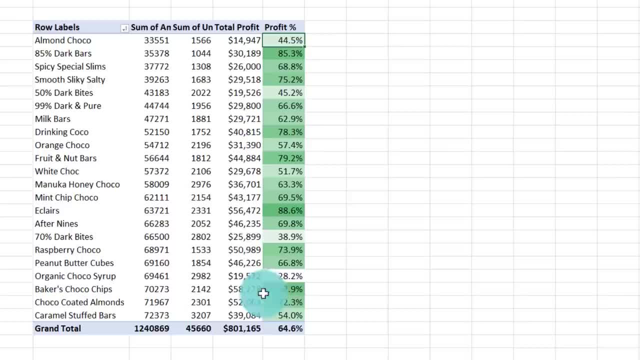 some of these very high numbers in 60s and 80. So if I want to drop this one, we are not gonna really, you know, take a huge hit on our bottom line or top line and we will still be fairly good. 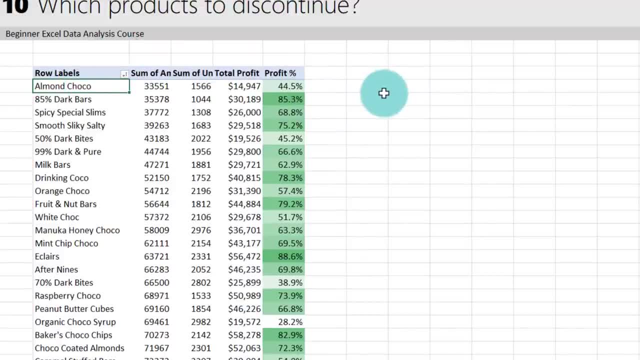 So this is one of the products that we can definitely drop, based on our criteria of looking at amounts and looking at total units and total profit percentage. But if you want to take this to the next level, we could then say wait a sec, maybe we can. 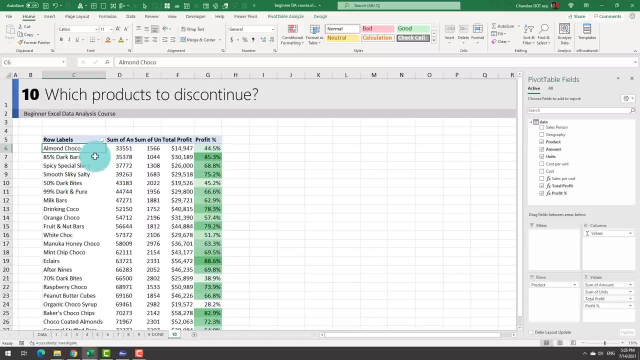 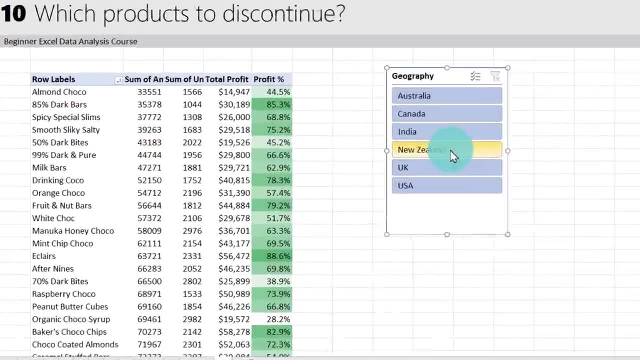 discontinue the products by geographies. To add that layer of detail, you can add a slicer on on the country And then you can pick the country where you want to, for example, test your discontinuation process. So let's go with New Zealand. 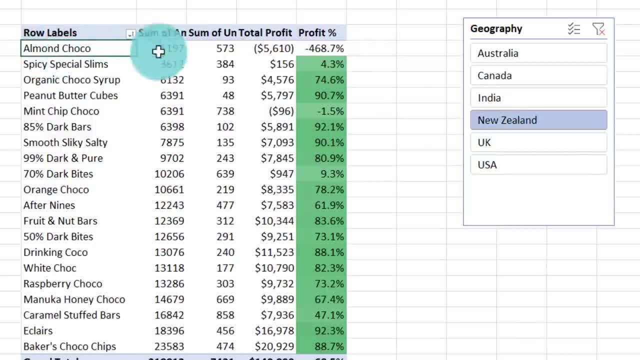 Okay, And within New Zealand, you can see that Almond Choco is actually one of our loss making products. It is giving you negative 468% loss, So this is not good right? This again reconfirms our belief that Almond Choco is probably the one to drop. 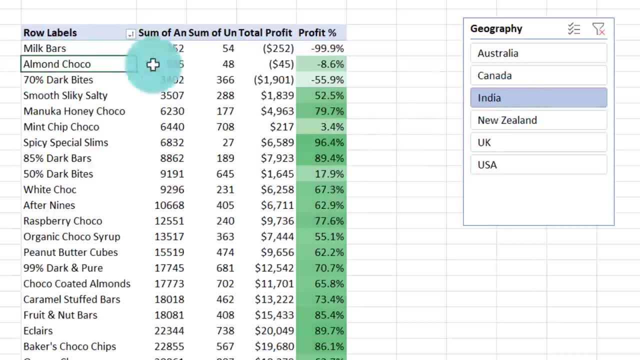 Let's see what is happening within India. Within India, Almond Choco again ranks fairly high. It is making loss, but we have been also making losses on the milk bar, but we don't really make much money- only $252.. 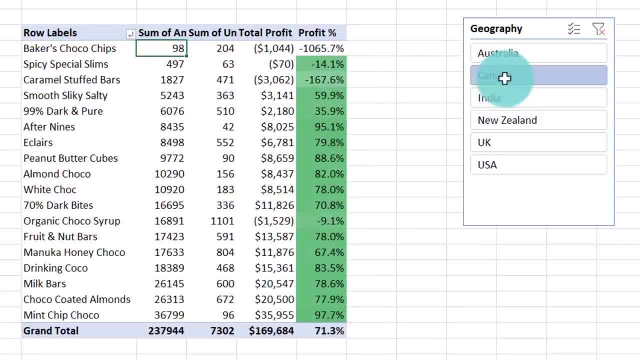 So it's not a big deal. To look at Canada, Almond Choco is one of the more profitable ones within Canada market, So probably not a good idea to drop Almond Choco for Canada, But this is Baker's Chocolate Chips is a good candidate: $98, 204 units. 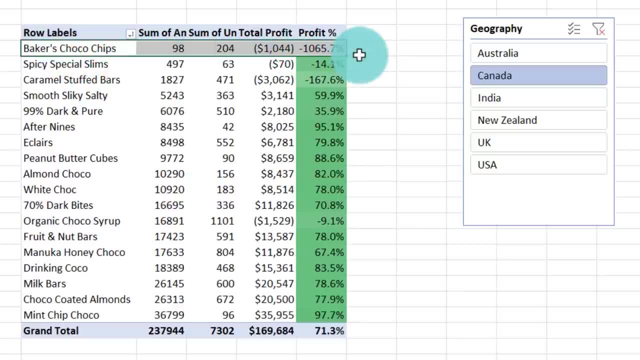 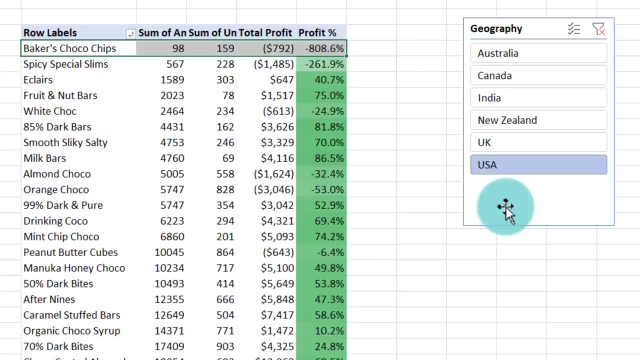 And we incur a massive loss on that, probably because we have to ship those things all the way to Canada. So this is how you can make the decision. You can at least give some solid arguments saying, hey, when we look at these individual cross sections across multiple things, I'm noticing that Almond Choco, Baker's Choco. 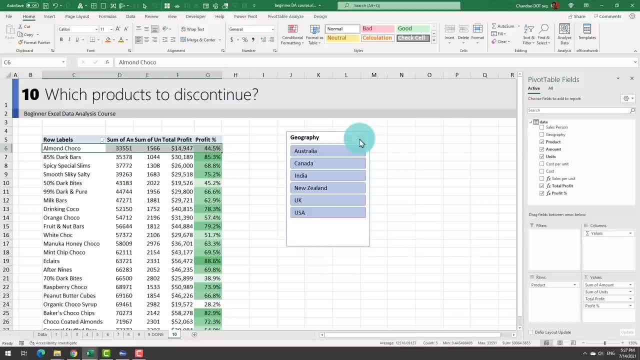 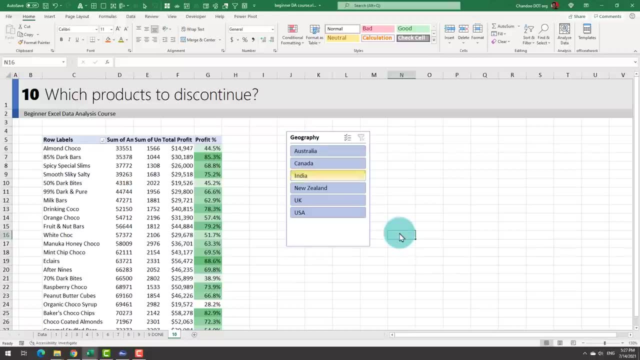 Chips appear all the time. So probably those are some of the solid starting candidates for us to drop, And you can see that when you deselect everything. Almond Choco is still at the top, but Baker's Choco Chips is somewhere at the bottom. 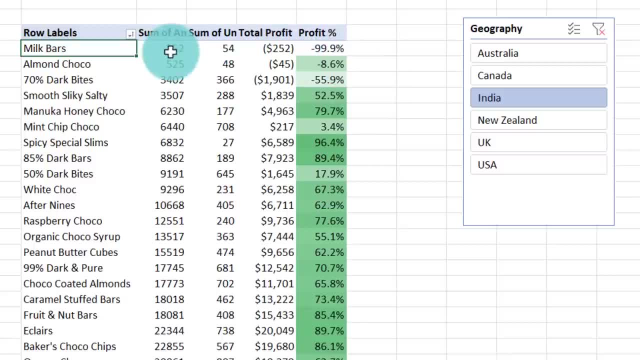 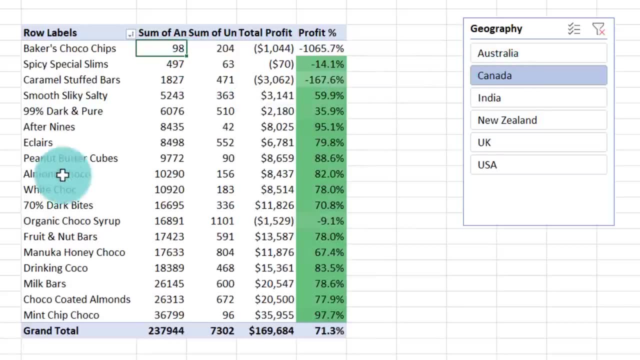 may we have been also making losses on the milk bar, but we don't really make that much money- only 252 dollars- so it's not not a big deal. to look at, canada almond choco is one of the more profitable ones within canada market, so probably not a good idea to drop almond choco for canada. 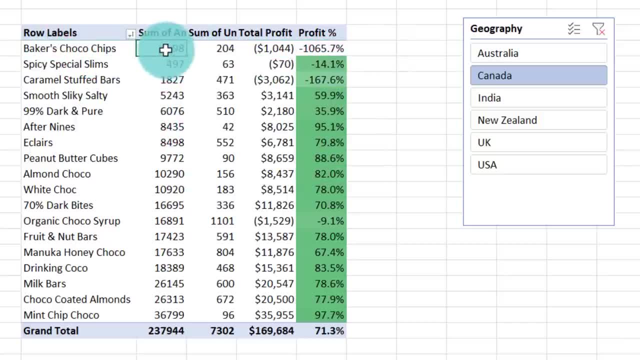 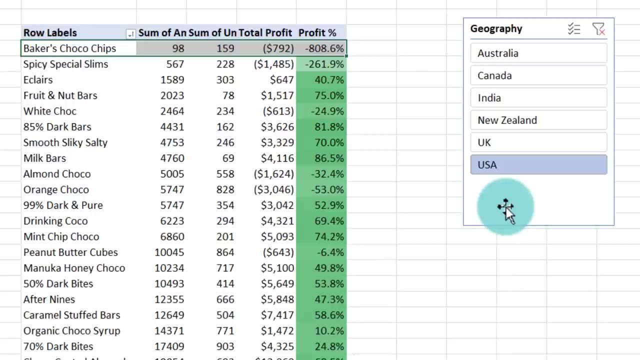 but this is baker's chocolate chips is a good candidate: 98 dollars, 204 units, and we incur a massive loss on that, probably because we have to ship those things all the way to canada. so this is, uh, how you can make the decision. you can at least give some solid arguments saying: 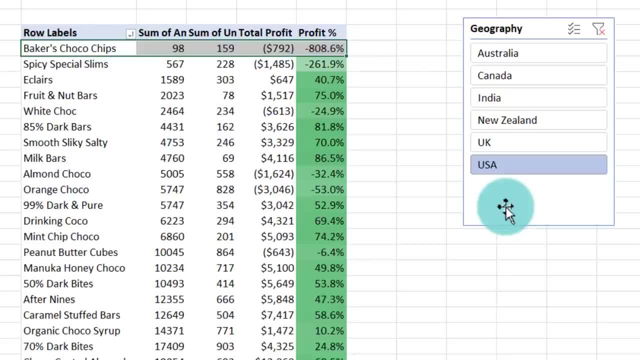 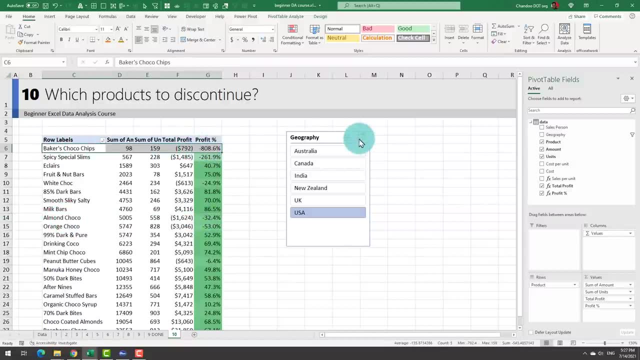 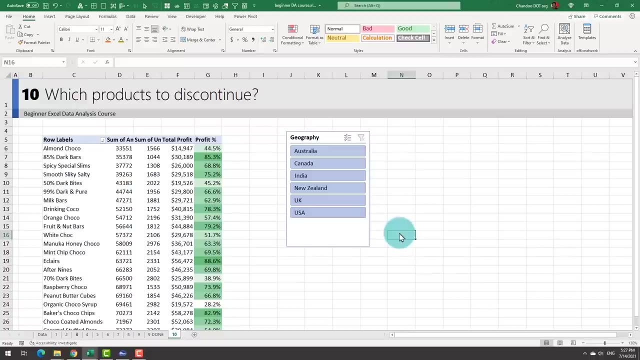 hey, when we look at these individual cross sections across multiple things, i'm i'm i'm noticing that almond choco baker's choco chips appear all the time, so probably those are some of the solid starting candidates for us to drop, and you can see that when you deselect. 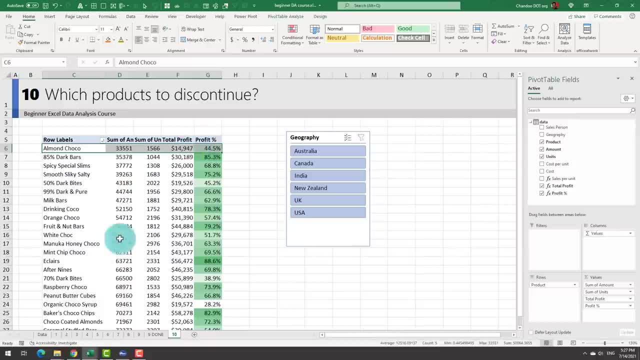 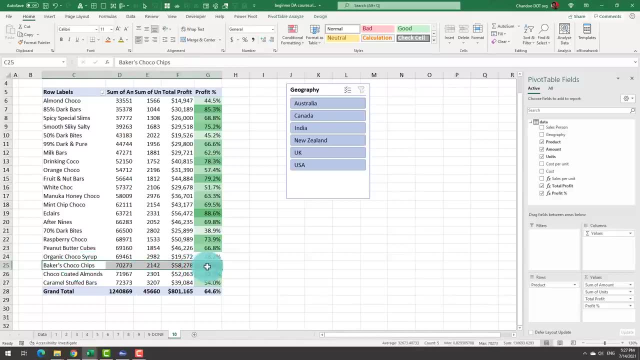 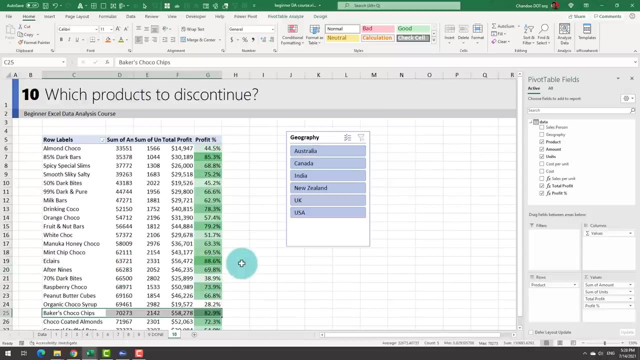 everything almond. choco is still at the top, but baker's choco chips is somewhere at the bottom with the very high profitability ratio. so probably not a good idea to drop this one straight away, but only discontinue it for certain geographies. so this is how you can go and come up with that recommendation to say that product almond. 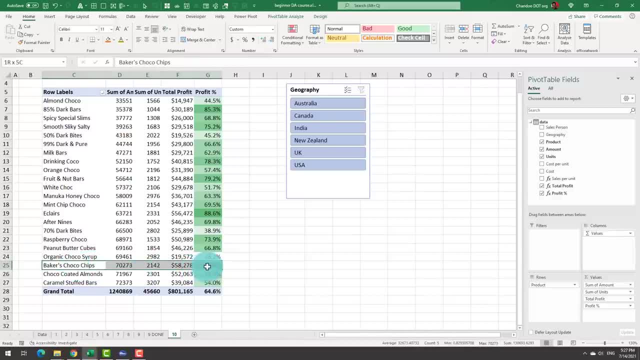 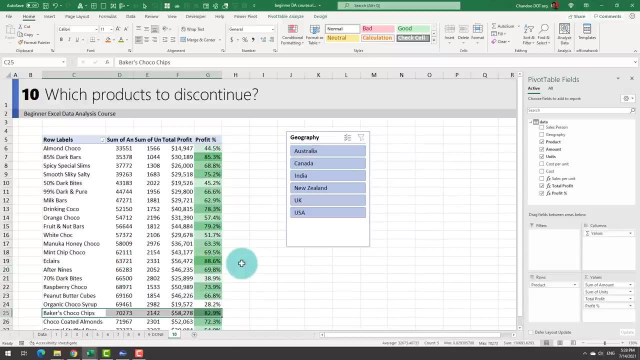 With the very high profit Profitability ratio. So probably not a good idea to drop this one straight away, but only discontinue it for certain geographies. So this is how you can go and come up with that recommendation to say that product Almond. 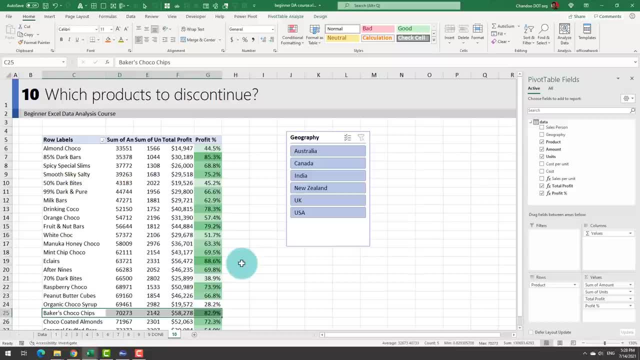 Choco need to be discontinued across the board. Baker's Choco Chips only for geographies A, B and C, like that. So that will give your managers or your clients more confidence that, yes, you've looked at the data. You've now come up with some valuable things. 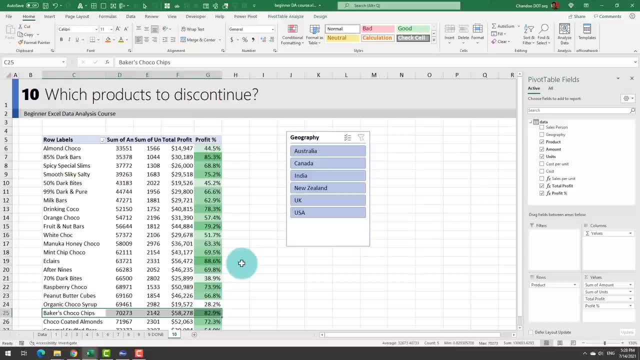 choco need to be discontinued across the board. baker's choco chips only for geographies a, b and c, like that. so that will give your managers or your clients more confidence that, yes, you've looked at the data. you've now come up with some valuable things. now here is a question back to you. 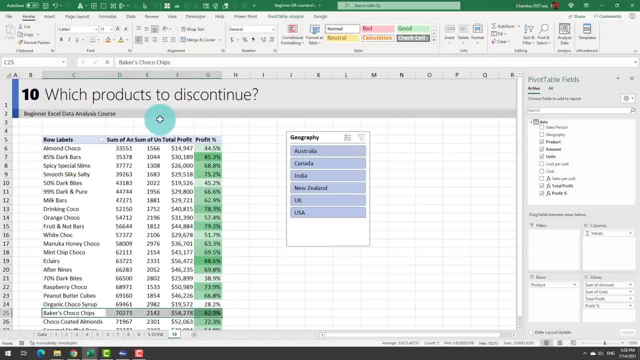 how would you decide which products to discontinue? what other additional things or metrics or indicators would you use Or what logic would you use? Tell me in the comments, because I'm very keen to learn from you and your experience as well. So if you find anything interesting that I missed, 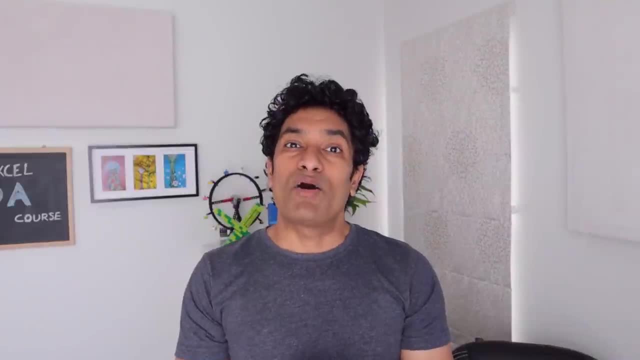 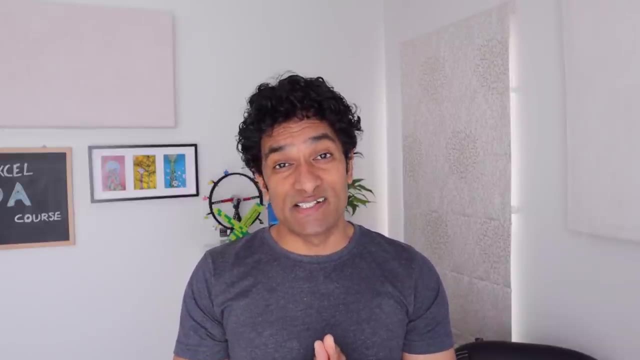 tell me, and then we can all benefit from that. I hope you found that video very useful. Don't forget to download the sample files so that you can right away practice these skills before you forget them Now. if you are looking to improve your data analyst skills, I highly recommend. 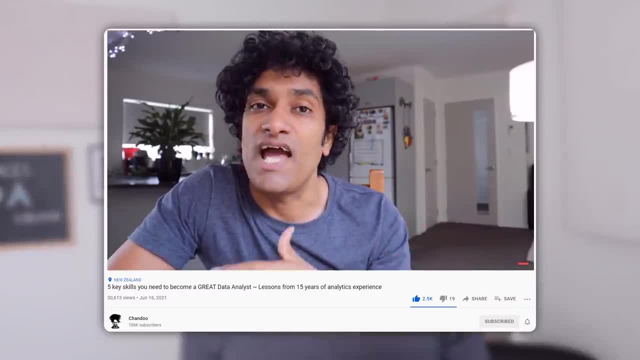 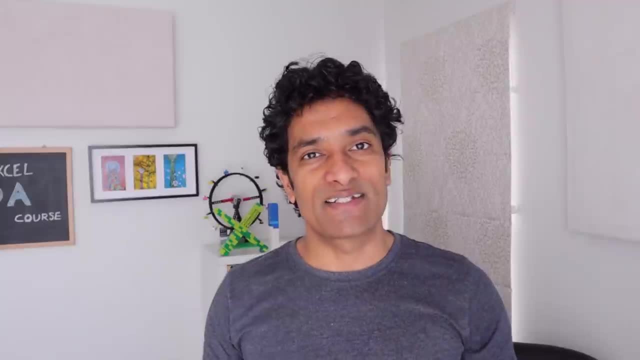 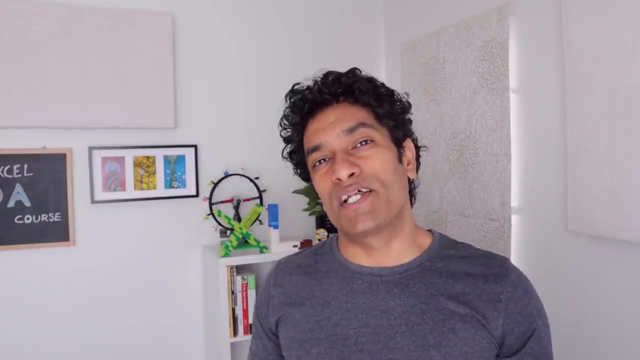 checking out my recent video. It talks about five key data analyst skills that you should develop if you want to be a great data analyst. Check it out- It is linked somewhere up on the screen For more data analysis videos using Excel. check out my playlist on the data analysis things here.